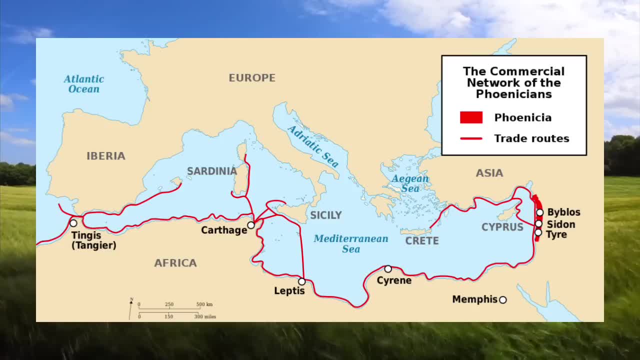 on the North African coast Near present-day Tunis, Tunisia. the Phoesians, a Semitic-speaking people known for their seafaring skills, established colonies and trading posts throughout the Mediterranean, and Carthage became a powerful maritime empire, Dominating regions such as North 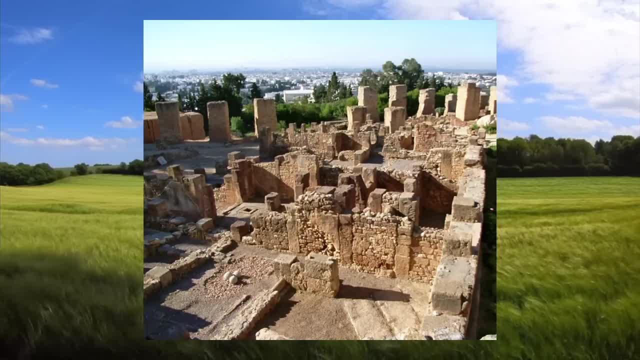 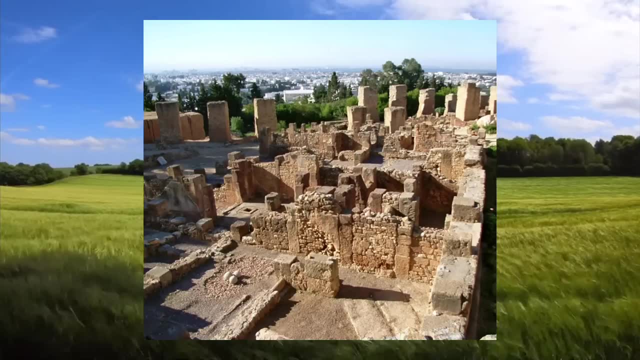 Africa, Sicily and the Mediterranean. Carthage became a powerful maritime empire, Sardinia, Corsea and parts of Spain. The rivalry between Carthage and Rome culminated in the Punic Wars, a series of conflicts spanning from 264 BCE to 146 BCE, The Second Punic War in particular. 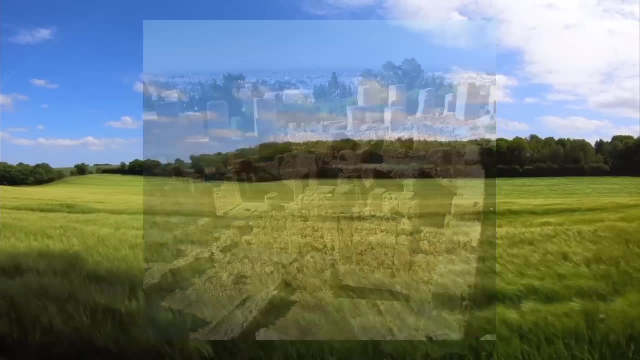 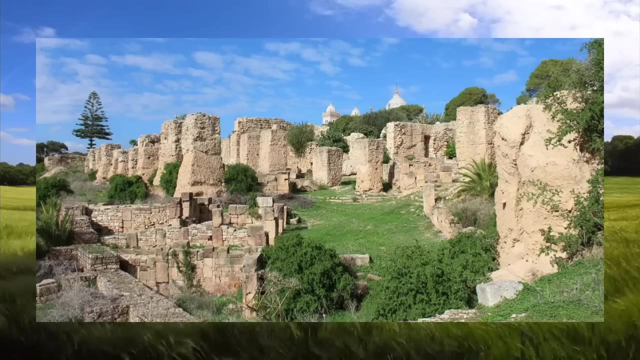 gained historical prominence with the brilliant military campaigns led by Carthagin General Hannibal, including the famous crossing of the Alps with elephants. Despite Hannibal's notable victories, Rome ultimately emerged triumphant, culminating in the destruction of Carthage in 146. 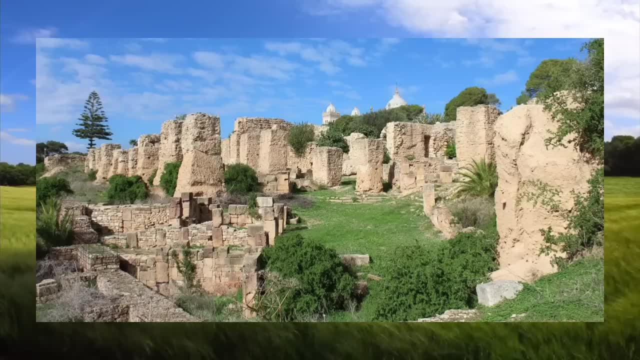 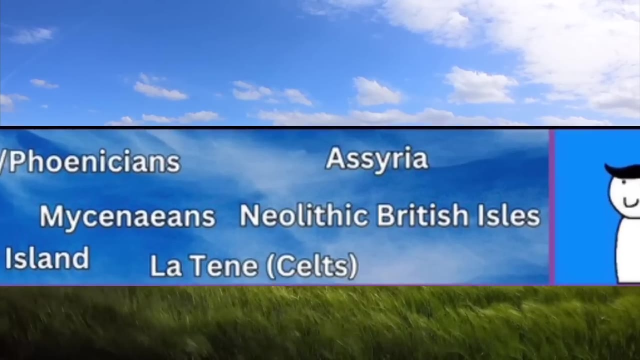 BCE Around the Third Punic War. the legacy of the Phoesians and Carthaginians endures in various different aspects. Their contributions to maritime technology, trade and culture left a lasting impact on the ancient Mediterranean world. Assyria, an ancient Mesopotamian civilization. 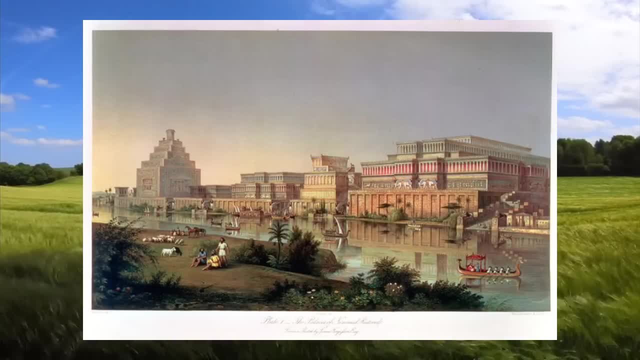 thrived from the 25th century BCE to the 7th century BCE in the northern part of Mesopotamia. It encompassed regions of modern-day Iraq, Syria, Turkey and Iran, with the Tigris River flowing through its heart. The empire had several capital cities. including Ashur, Nimrud and Nevin. The latter became one of the largest and most influential cities in the ancient world. Renowned for their military prowess, the Syrians developed advanced tactics, siege warfare techniques and a highly organized army, Iron weapons and a standing army. contributed to their military dominance. The Syrian empire reached its end under rulers like Ashurprinural II, Shalmaneser III and Shalmaneser III. The Syrians were the first to reach the Tiglath-Pileser III, Sargon II and Senecherbi, spanning from the Persian Gulf to the Mediterranean. 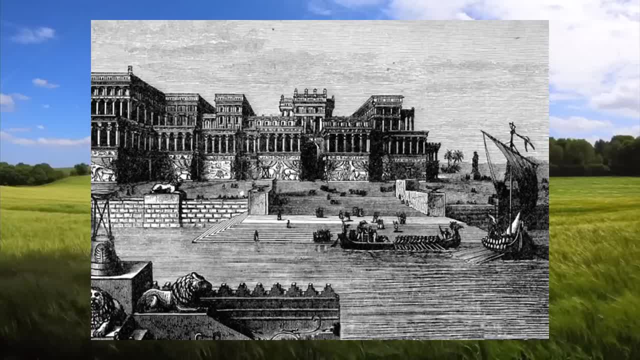 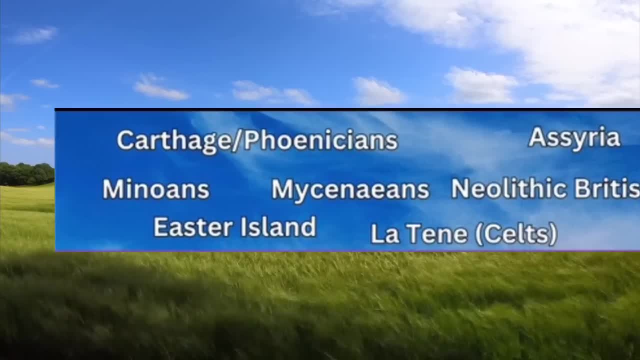 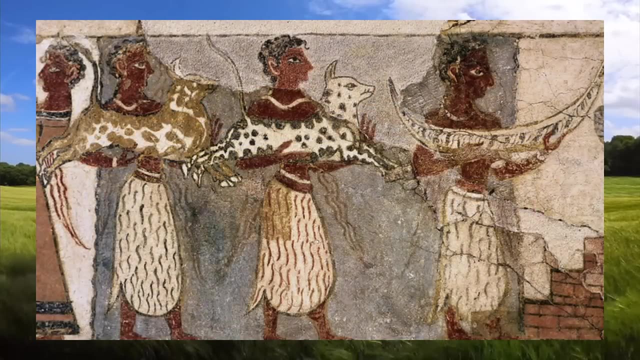 and from Antolia to Egypt. Culturally, Assyrians made significant contributions to art and architecture Minoans. The Minoans, a fascinating ancient civilization that thrived on the island of Crete from approximately 2700 BCE to 1450 BCE, left an enduring legacy in the annals of Mediterranean. 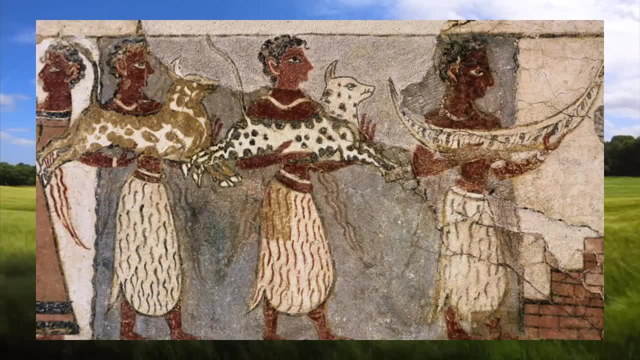 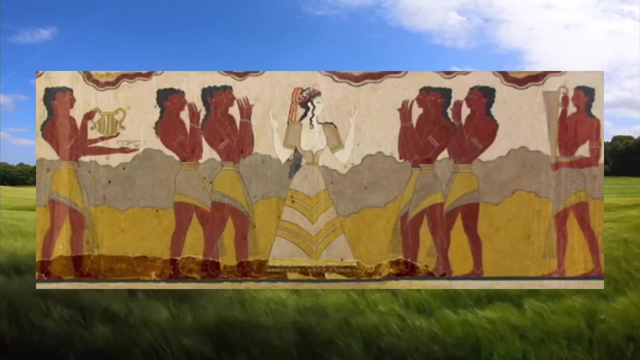 history, The Minoans were the first to reach the Mediterranean, and the Minoans were the first to reach the Tiglath-Piles for the third time in their long history, a few hundred years before the inhabitants of size more unknown ones in other parts of the world later on down the iceberg. But anyways. centered around major cities like Knos, Vesitios, Malia and Zakros. the Minoans are renowned for their elaborate palace complexes, with the Palace of Knos standing out as a prime example. These multi-story structures featured intricate layouts, courtyards, storage rooms, residential areas. 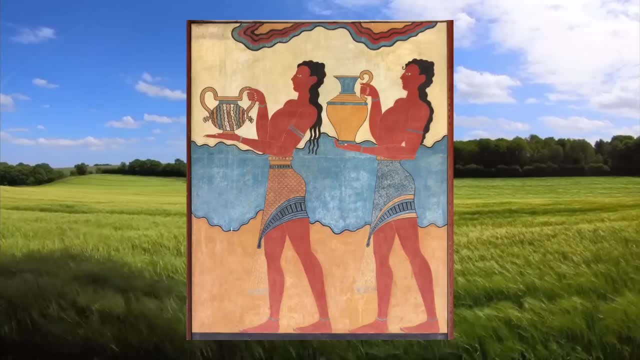 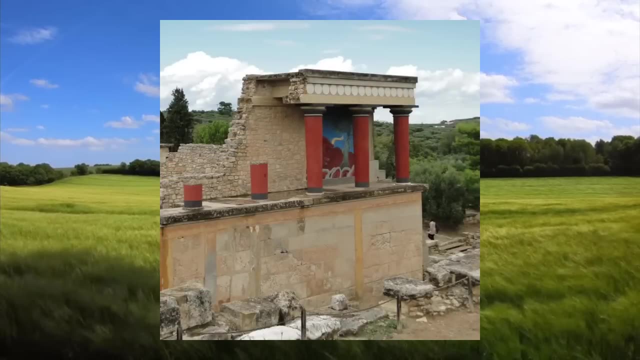 and religious sanctuaries, providing insights into the sophistication of Minoan urban planning. Artistically, the Minoans displayed a vibrant and naturalistic style in their frescoes, capturing scenes of daily life, nature and religious rituals which helped us see into their 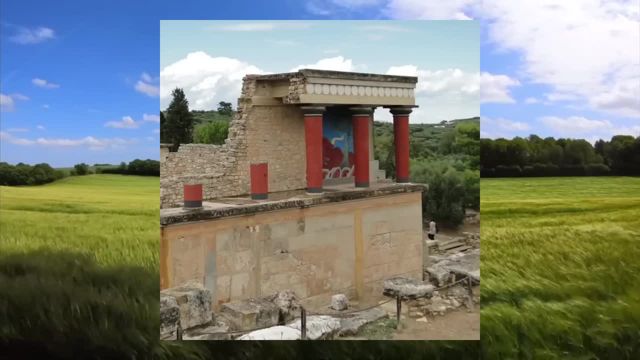 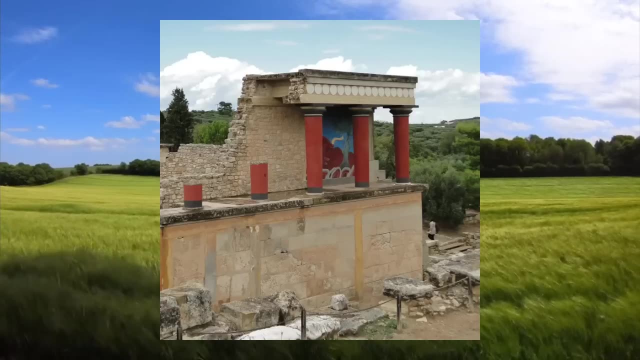 kind of lives so many years back then. The famous depictions of bowl leaping showcase the Minoans' athletic and ceremonial pursuits. The Minoans employed a writing system known as Linear A, although its meaning remains undeciphered, adding an area of mystery to the linguistic. 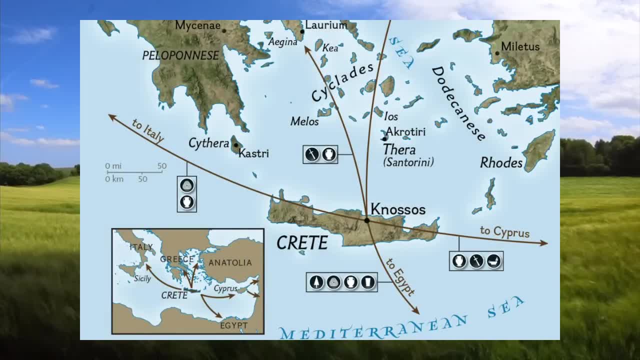 achievements. A defining aspect of the Minoans' artistic and cultural heritage is the fact that the Minoan civilization was its maritime prowess and extensive trade networks. The Minoans were adept seafarers engaging in commerce with other Mediterranean cultures, including Egypt and the 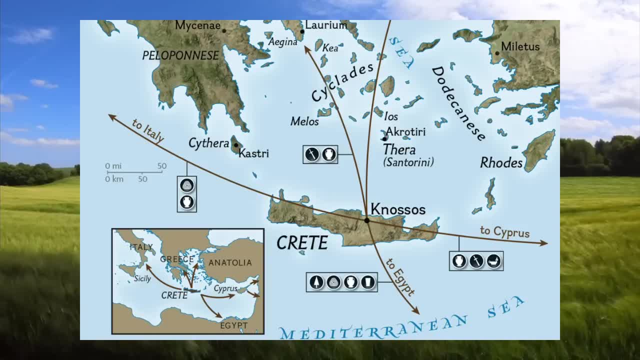 Silitic Islands. Their influence reached far beyond Crete, marking them as a significant player in regional interactions. The Minoans' religious practices were intricate, featuring a complex patheon of diades and rituals. Bowl symbolism played a prominent role, suggesting 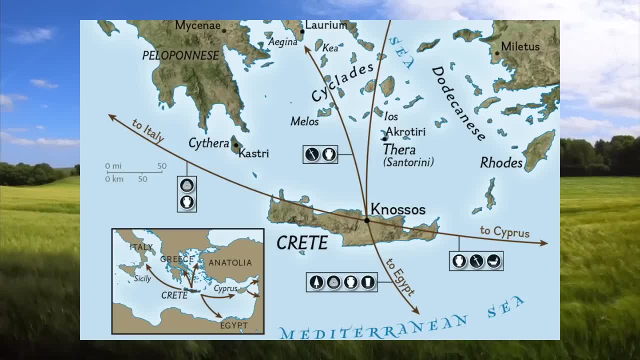 connections to themes of fertility and power. Despite their cultural and cultural heritage, the decline of the Minoan civilization around 1450 BCE remains unknown. Natural disasters such as earthquakes and the eruption of Thera volcano and the invasion of Mycenaeans from 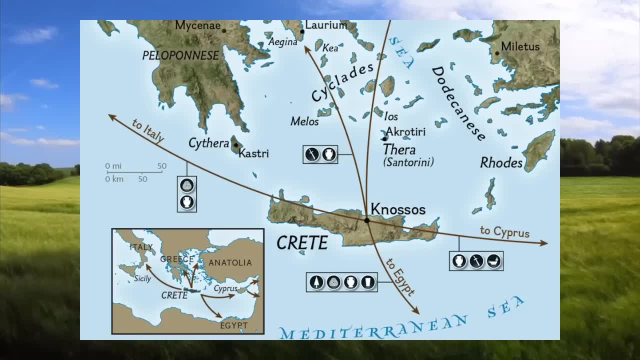 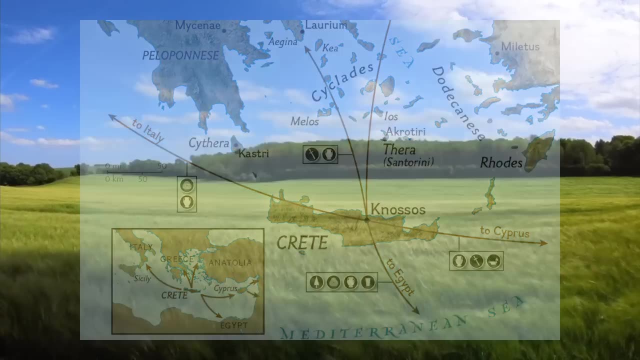 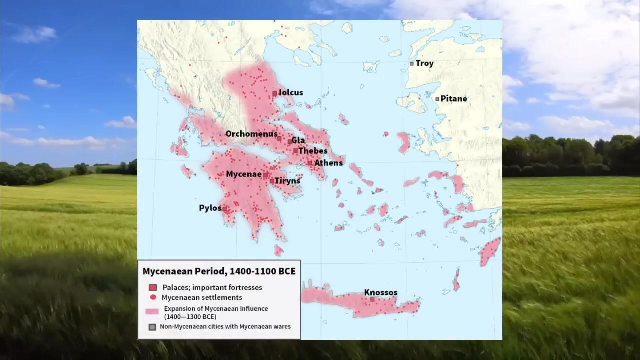 the mainland Greece are proposed factors contributing to their downfall. The legacy of the Minoans persists through their contributions to art, architecture and seafaring activities. Mycenaeans- The Mycenaeans, an ancient Greek civilization flourishing from approximately 1600 BCE to. 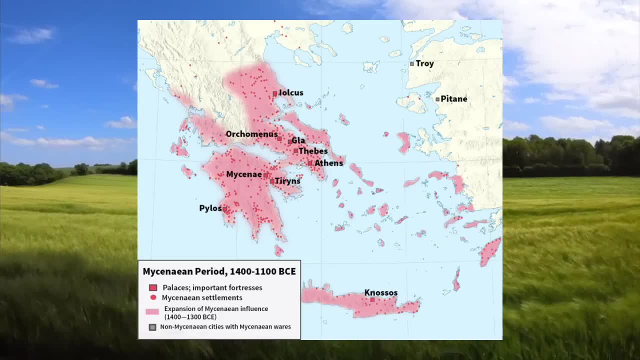 1100 BCE left an indelible mark on the history and culture of ancient Greece. Situated on the Greek mainland, their major centers, including Mycenaean, Tyrenes, Pylos and Athens, were characterized by fortified palace complexes that served as administrative, economic and. 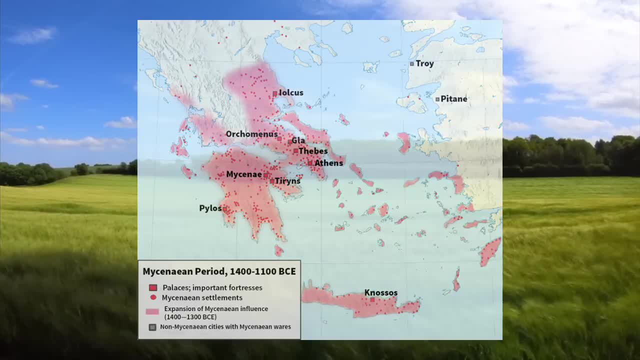 potentially religious hubs. Notable among these was Mycenaean, which was the most important of the Mycenaean civilizations. The Mycenaeans were also known as the Mycenaeans of the Mycene, distinguished by the iconic lion gate and associated with legendary figures. 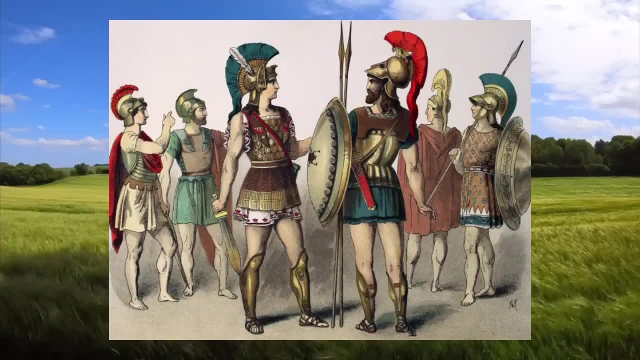 like Agamemnon and Achilles in the Tales of the Trojan War recounted by Homer, The Mycenaeans utilized the Linear B script, of opposite from the Linear A script, A syllabic writing system deciphered in the mid-20th century, primarily for administrative and economic. 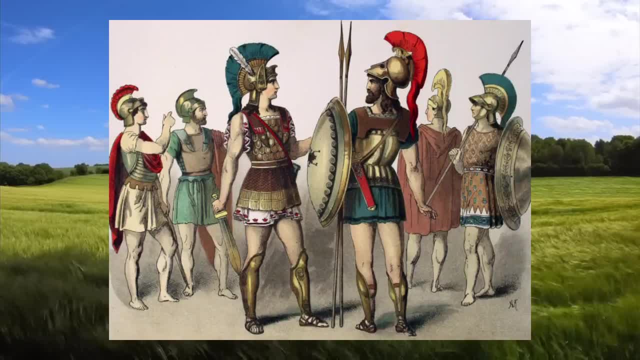 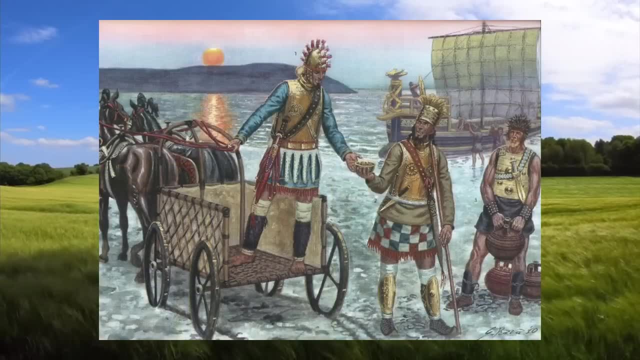 purposes reflecting a warrior culture. Mycenaean cities were fortified with defensive walls and their art, such as the renowned Mycenaean, was a symbol of the Mycenaean culture. The famous Mycenaean warrior vase paintings depicted scenes of battle and military life. The Mycenaeans 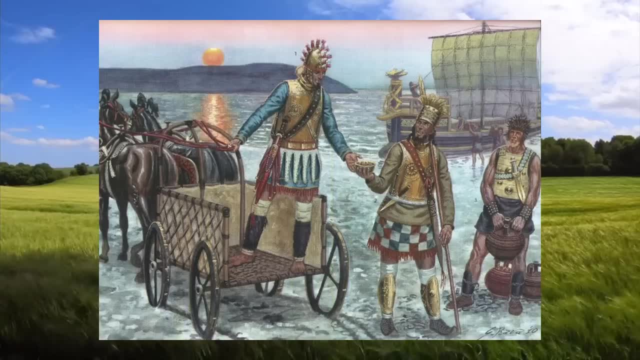 engaged in active trade, establishing connections with cultures across the Mediterranean, including the Minoans, as we just covered, and the Invalidum regions, as far as Sicily and the eastern Mediterranean. The legendary Trojan War, a central theme in Homer's epics, is often associated with Mycenaean leaders like Agamemnon, contributing to the rich tapestry of Greek mythology. However, this historical accuracy of the Trojan War remains a topic of debate. The decline of the Mycenaean civilization around 1100 BCE marked the end of this era. 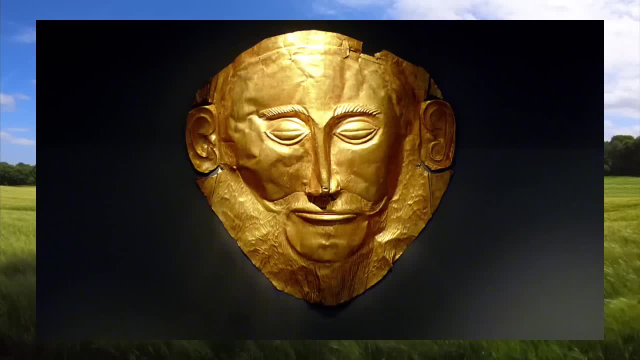 With factors such as internal unrest, invasions and socioeconomic changes playing a role in the complex process. despite their eventual decline, the Mycenaeans left a lasting legacy. They were their cultural and artistic contributions. in fact, The older Mycenaeans were the second. 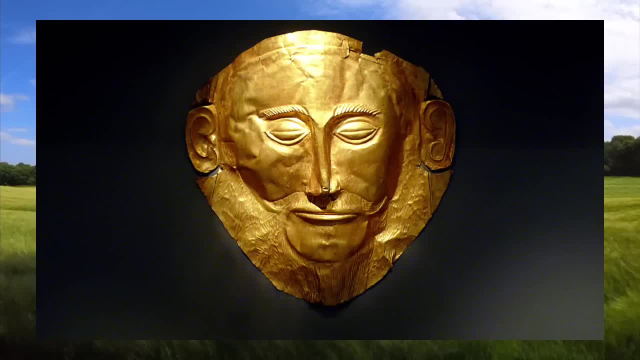 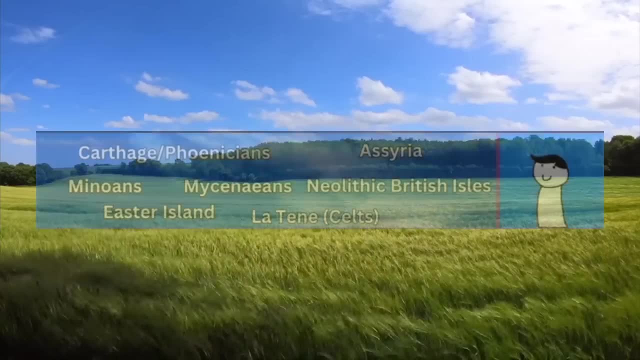 to reach this status By the time their Chartres were following the rest of the Roman territory. Warrior ethos and trade networks laid the foundations for classical Greek civilization, providing a crucial bridge between the Bronze Age and the subsequent Classical Era- Neolithic British Isles. The Neolithic period in the British Isles, spanning roughly from 4000 BCE to 2000 BCE, marked a pivotal era characterized by transformative developments in human society. One of the defining features was the adoption of agriculture, leading to settled communities engaged in cultivating crops and domesticating animals. 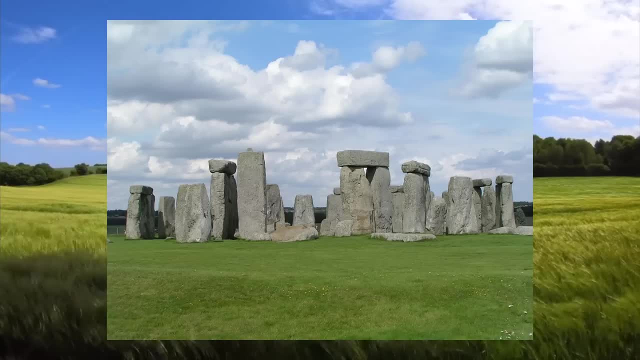 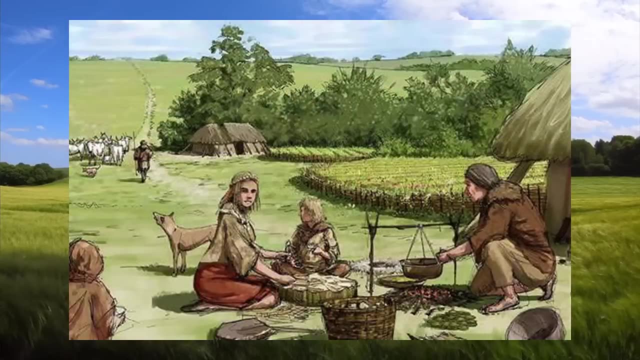 This shift from a hunter-gatherer lifestyle to settled agriculture laid the foundation for significant societal changes. During the Neolithic, the construction of megalithic monuments became a prominent aspect of the British Isles' landscape: Stone circles, hinges and chambered tombs, exemplified by sites like Stonehenge and Avebury. 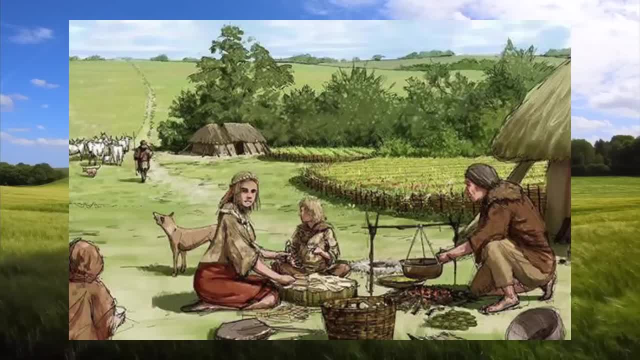 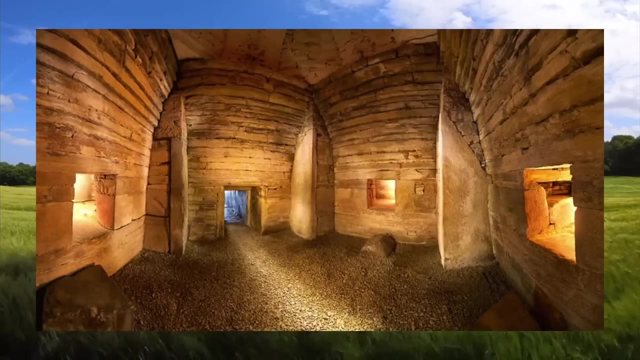 reflected the community's engagement in religious, ceremonial and possibly astronomical activities. The mystery and grandeur of those structures continued to captivate modern imaginations. Burial practices also evolved during this period with the construction of long barrows. These elongated earthen mounds served as communal burial sites. 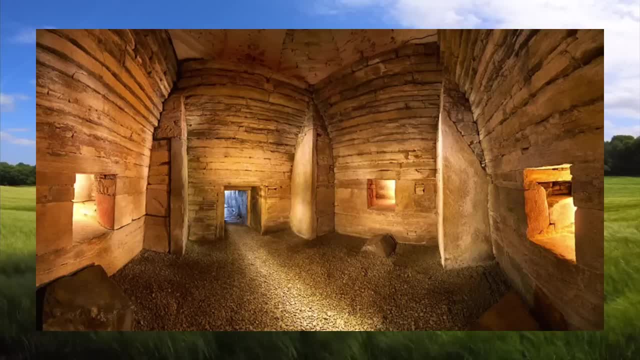 often accompanied by grave goods, providing insights into Neolithic beliefs regarding the afterlife and spirituality. Advancements in pottery technology were evident in the Neolithic material culture. Pottery vessels became more sophisticated, showcasing the artistic and functional capabilities of these early communities. 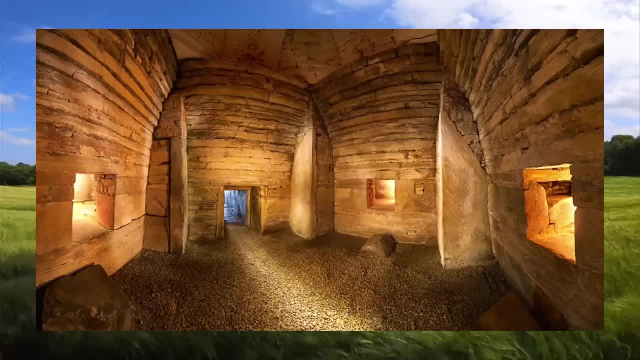 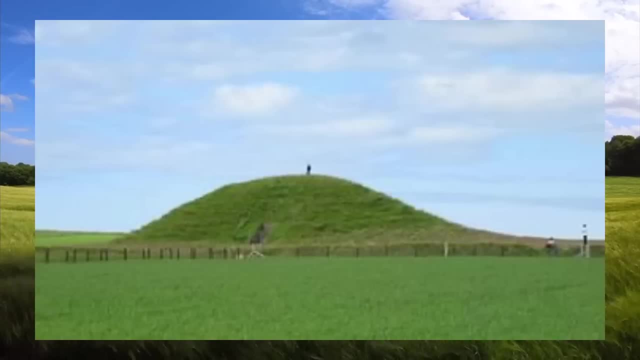 The prolific tarion and polished stone tools, flint, arrowheads and decorative items further characterized the artifacts of this era. Trade networks played a crucial role in connecting Neolithic communities, facilitating the exchange of good over considerable distances. This interaction contributed to the cultural diffusion and the sharing of raw materials. 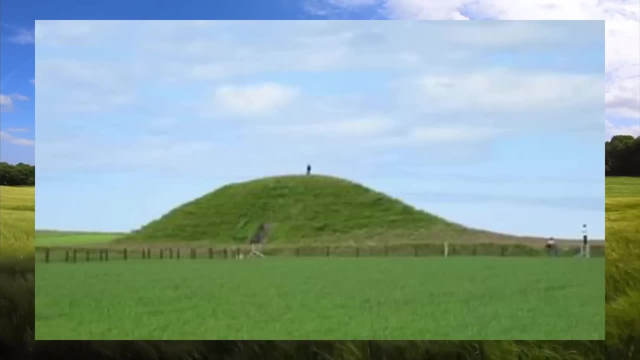 enhancing the diversity of material culture. environmental changes and the impact of early agricultural practices shaped the landscapes of the British Isles during the Neolithic. The complex relationship between human activities and the environment influenced both ecosystems and the availability of resources. As agriculture practices became more established, social structures likely became. 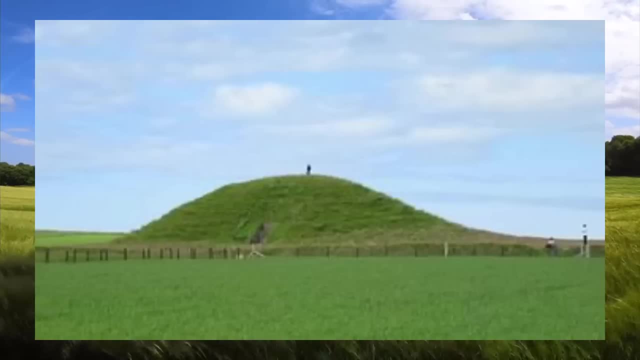 more complex, reflected in the communal endeavors such as the monument construction and burial rituals. This period of societal evolution laid the groundwork for subsequent cultural developments, including the transition to, once again, the Bronze Age. So this was before, which was like the Stone Age to the Bronze Age, another big shift marked by the introduction of metalworking and the use 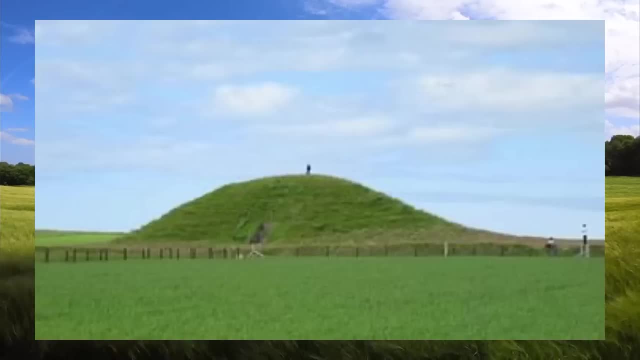 of bronze tools and weapons. In summary, the Neolithic period in the British Isles was a dynamic and transformative era that witnessed the emergence of settled agricultural communities, the construction of impressive megalith monuments and the establishment of new social and cultural practices. 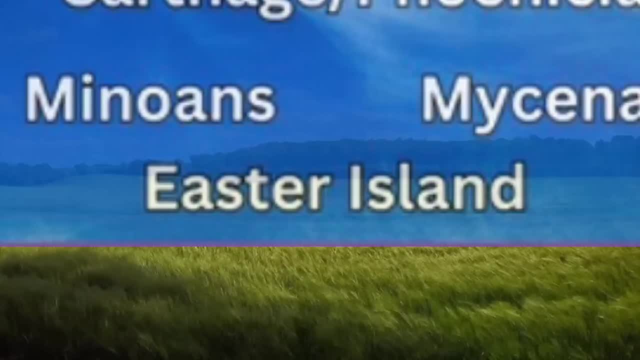 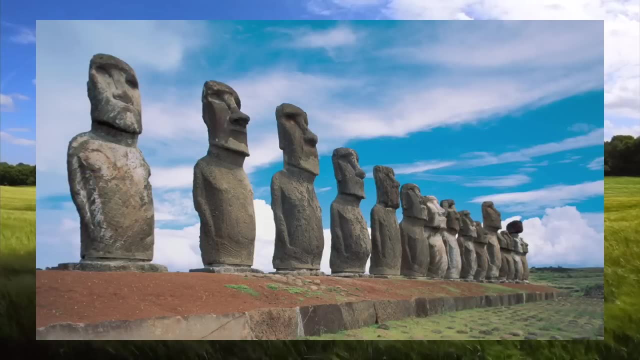 Easter Island. Easter Island, situated in the vastness of the southeastern Pacific Ocean, stands as a testament to the ingenuity of the indigenous people, the Rapa Nui. Central to its cultural identity are the iconic Maui statues, colossal stone figures with distinctive elongated features scattered across. 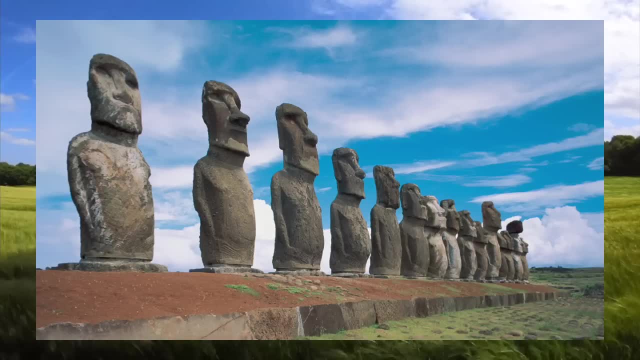 the island, Carved from compressed volcanic ash. these statues are a remarkable feat of ancient craftsmanship and engineering. The construction and transportation of the Maui remains subject to scholarly debate. No one really knew how they moved these huge, colossal stones weighing about several tons each. 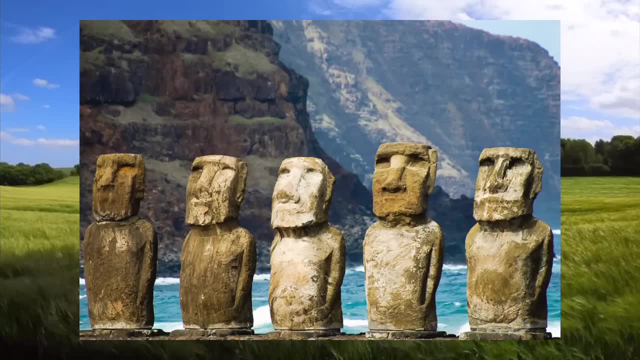 so, like I just said, these things are huge- were transported across the island to ceremonial platforms known as a Hu, showcasing the advanced skills and organization of the Rapa Nui people, The mystery of how they accomplished this feat using basic tools, sledges and ropes. 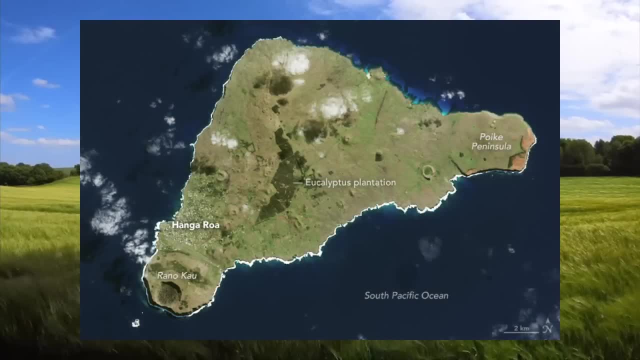 adds to the intrigue surrounding the Easter Island. The island's environmental history is also marked by significant deforestation events believed to be linked to the resources required for Maui construction. Once covered in palm trees, Easter Island's ecosystem suffered, potentially contributing to societal decline. This environmental degration 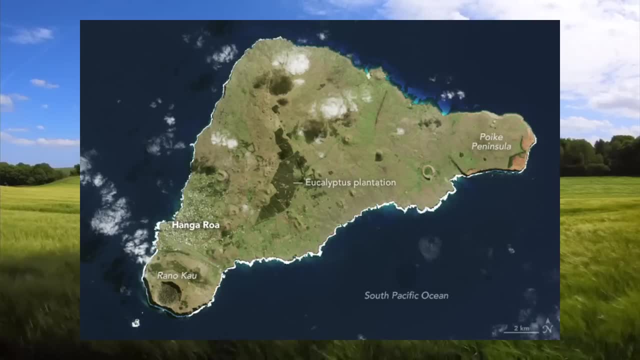 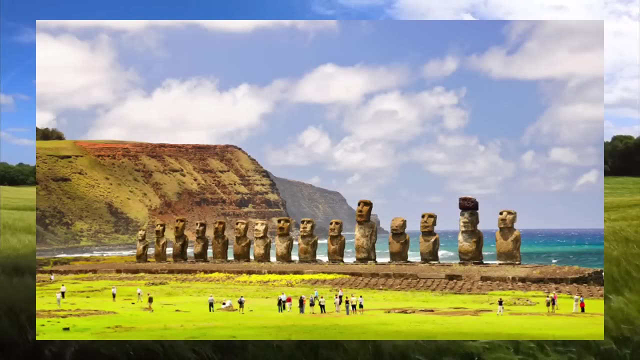 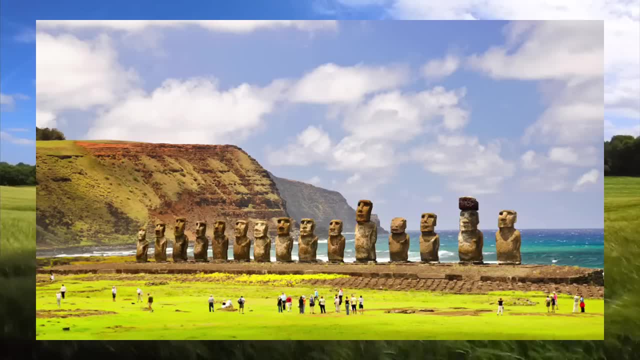 population. The island, annexed by Chile in the late 19th century, faced challenges related to land rights, cultural perservation and modern economic development. Today, Easter Island remains a source of fascination and UNESCO World Heritage Site, drawing visitors and researchers eager to unravel the mystery of its past: The Endurgen legacy of the Maui. 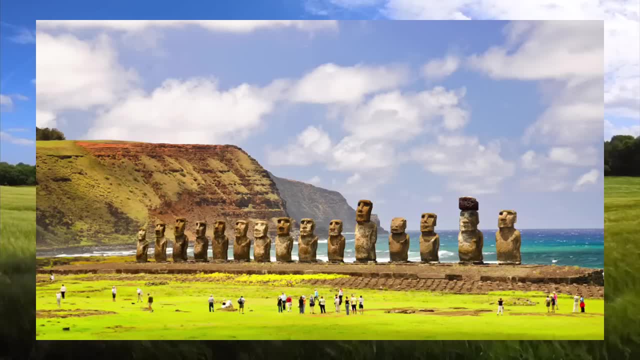 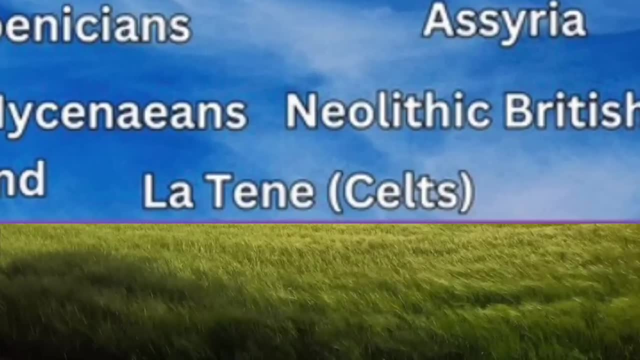 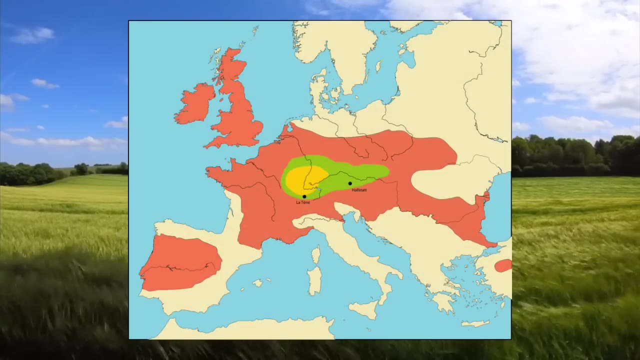 statues and the lessons embedded in the island's environmental history continue to resonate with people today. La Tène, or the Celts, The La Tène culture flourishing across Europe from approximately 450 BCE to the 1st century BCE, represents a significant chapter in the history of the Celts. 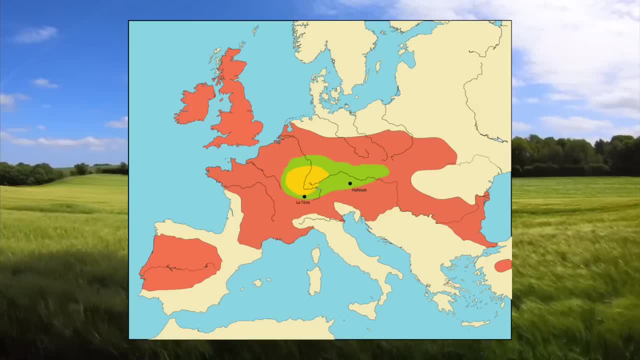 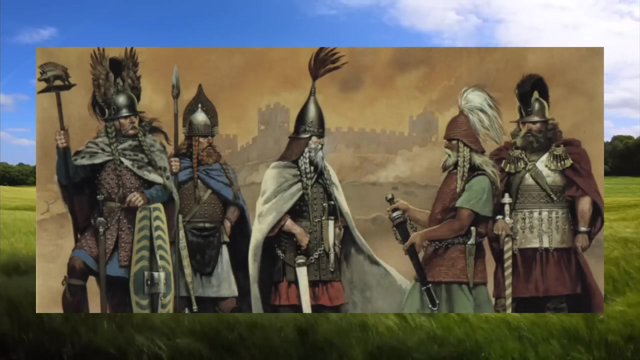 Named after the archaeological site of La Tène in Switzerland. this Iron Age culture showcased a distinctive artistic style characterized by elaborate metalwork, including intrinsically designed weapons, jewelry and everyday objects. The swirling motifs, geometric patterns and animal imagery displayed on these artifacts 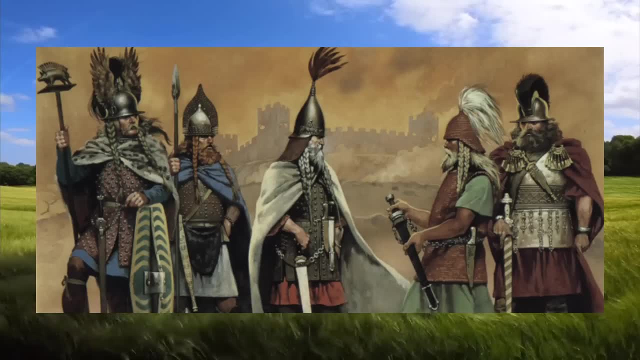 reflect the Celts' advanced metalworking skills. Geographically, the La Tène culture spanned a vast territory stretching from present-day France, Switzerland and Germany to the British Isles, the Iberian Peninsula and the Balkans. The Celts associated with the La Tène culture were adept to constructing hill forts and fortified settlements, such as a notable example of Broquet in France. These all served as central hubs for political, economic and cultural development. The Celts engaged in extensive trade and cultural interactions, establishing connections with neighboring regions and the Mediterranean world. While their religious practices during the La Tène period are not extensively documented, 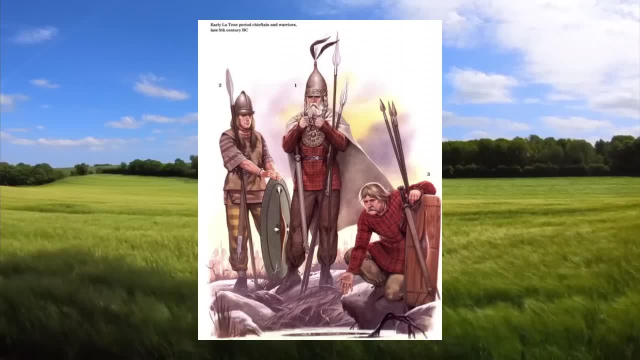 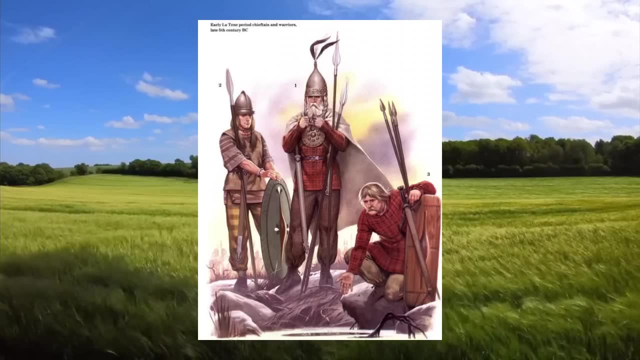 archaeological evidence suggests a polytheistic belief system with a focus on nature and deities associated with the elements. The decline of the La Tène culture coincided with the expansion of the Roman Empire. The Roman conquest of Gaul in the 1st century BCE marked a pivotal moment in the history. 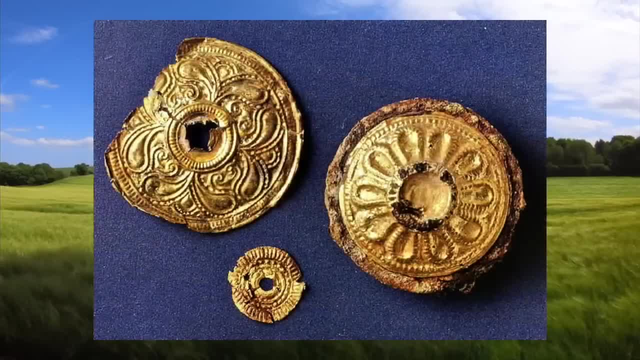 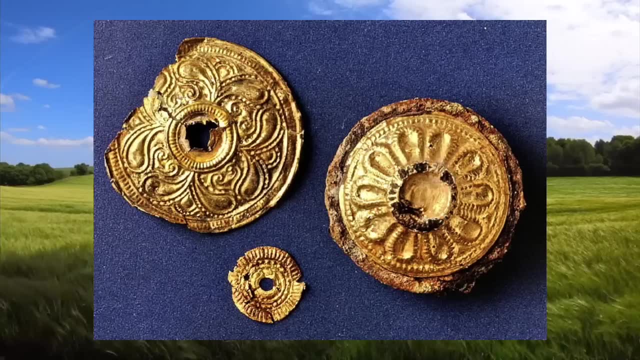 of the La Tène culture, Leading to the assimilation of Celtic territories into the Roman world. Despite the decline, the Celts' resistance across and against the Roman expansion and their artistic achievements have left an enduring legacy. The Celtic language, although diminished, survived in some regions today and elements 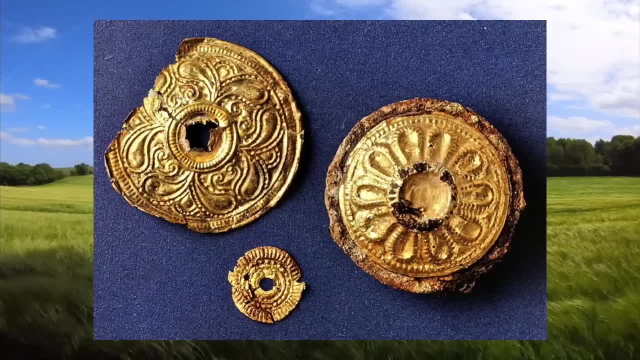 of Celtic art continue to influence contemporary design and cultural expression. The La Tène period stands as a testament to the rich cultural diversity and contributions of the Celtic culture. It was a time of great interest to the Celtic people in the complex tapestry of European 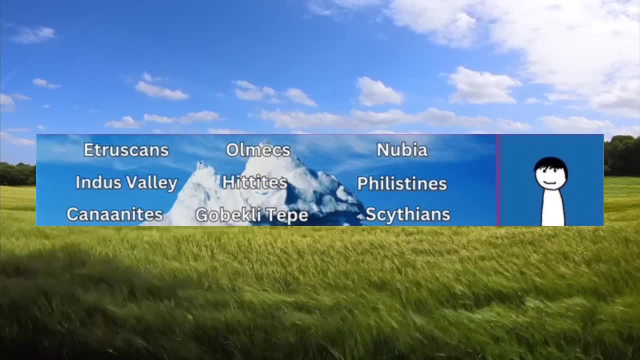 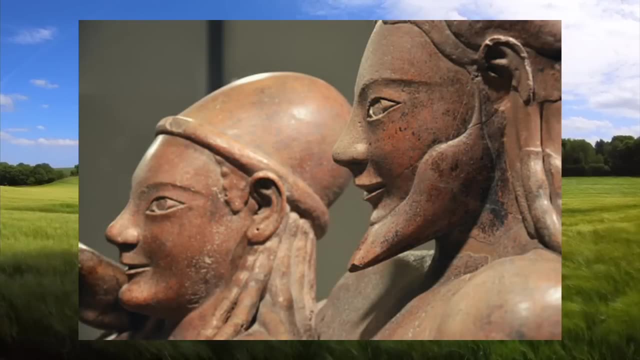 history All right. now onto tier 2, starting off with the Etruscans. The Etruscans, an ancient civilization in central Italy from the 8th to the 3rd century BCE, are characterized by a rich cultural heritage that significantly influenced the 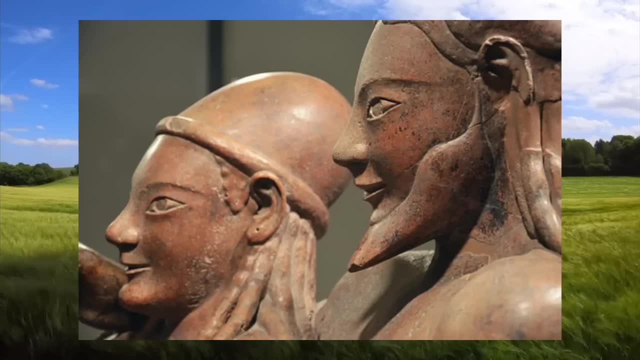 development of the region. Originating in the central Italian territories in Tuscany, Umbria and Lazalo, the Etruscans' established a network of city-states known for advanced urban planning, monumental architecture and sophisticated infrastructure, including drainage systems and roads. 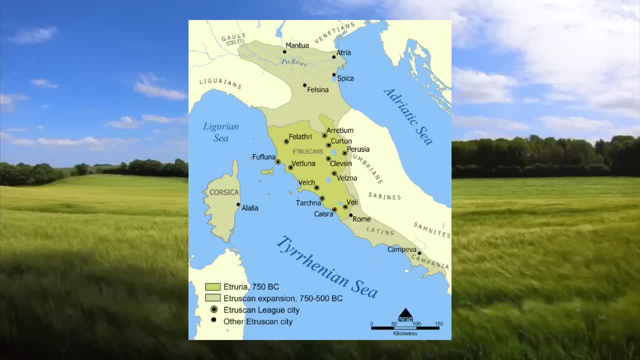 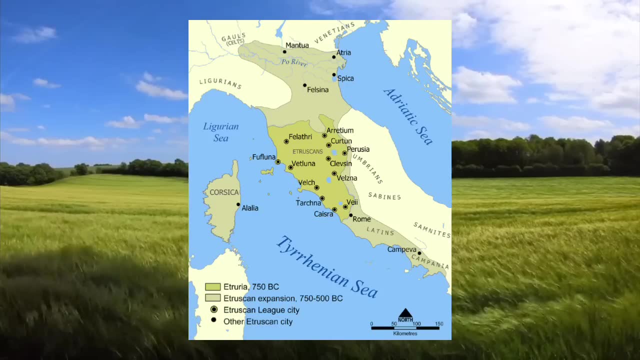 They, Czarnica and Cerveti, are among the prominent Etruscan cities that flourished. The enigma of the Etruscan language persists as it remains unclassified, without any known language families. although deciphered to some extent, their written records often 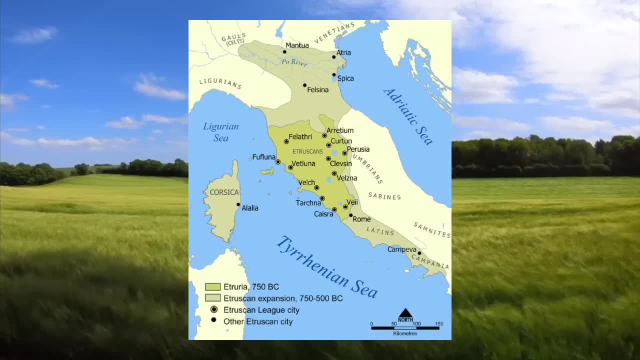 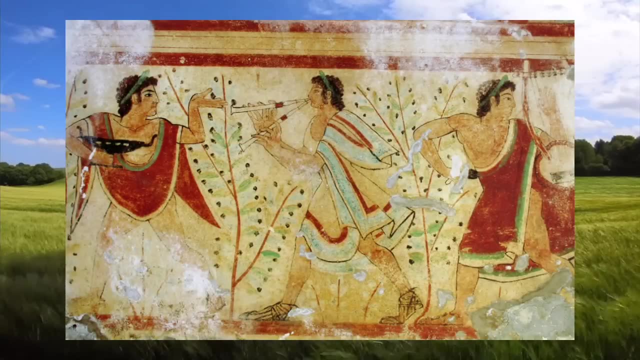 inscribed in a script distinct from the Latin alphabet, still pose challenges to comprehensive translation. Etruscan art, characterized by vibrancy and intricate details, encompassed frescoes, sculptures and pottery reflecting their cultural prowess. Active participants in Mediterranean trade, the Etruscans engaged in commerce with Greeks. and other neighboring cultures. Their influence on early Rome is pretty significant, contributing to cultural exchange and leaving a lasting impact on Roman art, religion and urban planning. Etruscan religious practices were polytheistic, featuring divination and a strong emphasis. 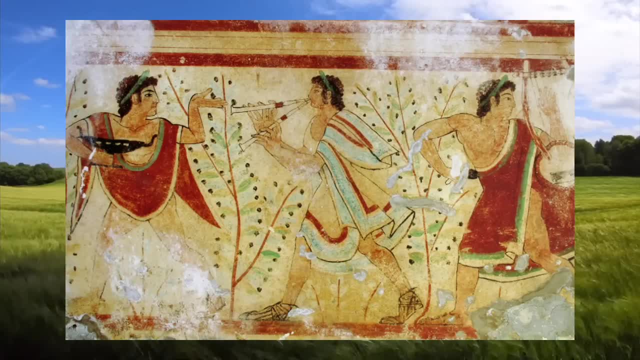 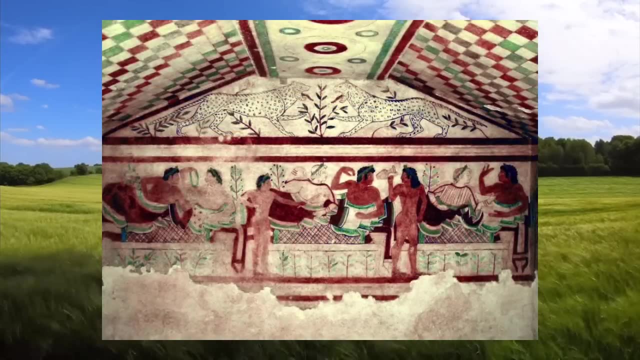 on the religious and religious traditions of the region. The Etruscans, however, were not the only ones to insist on interpreting omens and auspices. Etruscan tomes stand as a testament to their unique architectural designs. Timuli chamber, tomes and Necropolises were adorned with elaborate frescoes depicting scenes 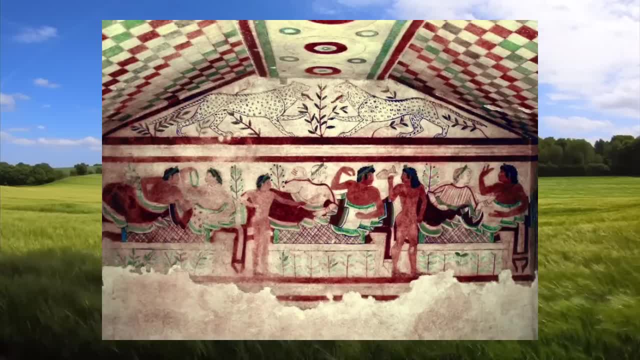 of daily life, religious rituals and beliefs about their afterlife. The decline of the Etruscan civilization is attributed to factors such as military conflicts, internal strife and eventual absorption into the expanding Roman Republic by the end of the 3rd century BCE. 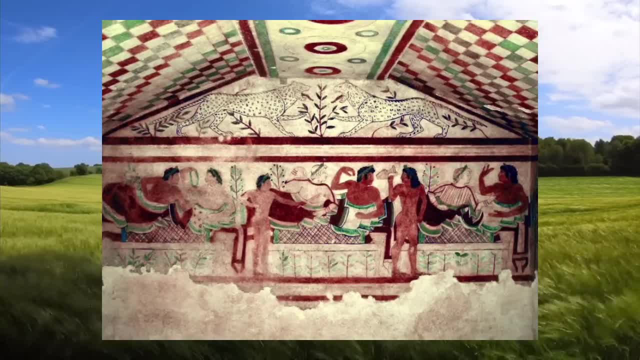 Despite the limited direct relationship between the Etruscans and the Roman Empire, the Etruscans have a long history. Their legacy endures through the profound impact on early Roman civilization. Elements of Etruscan art, religious practices and urban planning became integral to the 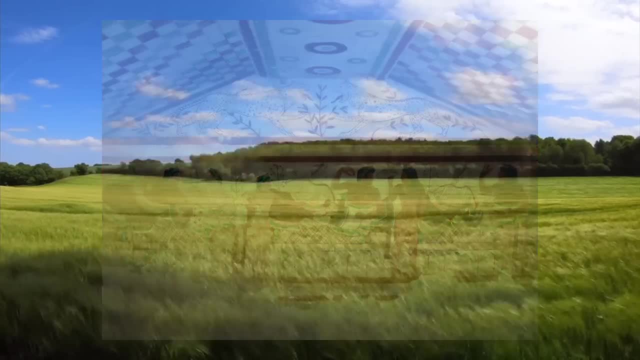 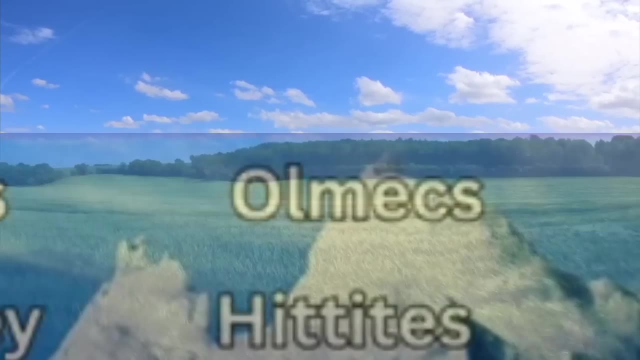 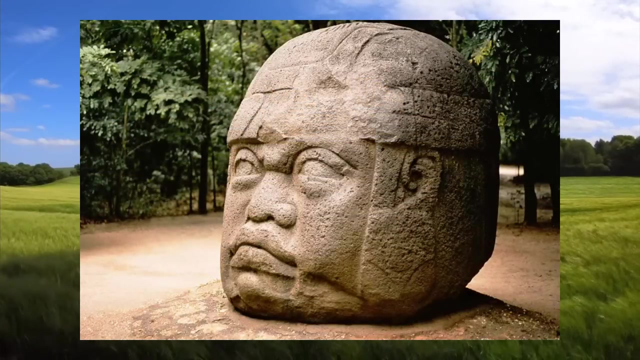 fabric of ancient Italy and the subsequent Roman Empire Olmics. The Olmics, an ancient Mesoamerican civilization, emerged along the Gulf Coast of present-day Mexico from around 1400 BCE to 400 BCE, establishing themselves as the cradle of Mesoamerican civilization. 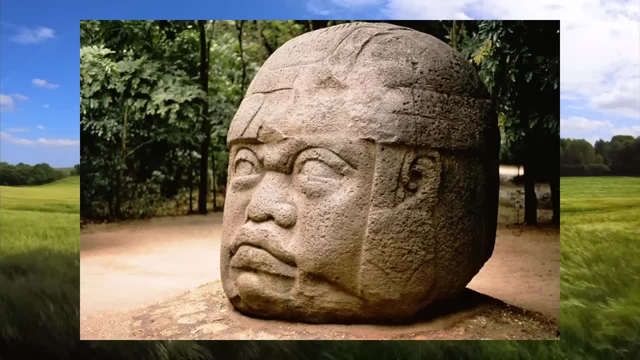 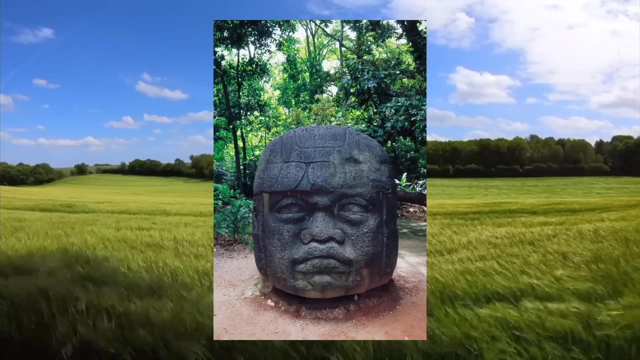 Flourishing in tropical Lao lands of Veracruz and Tabasco, the Olmics created a distinctive cultural legacy that influenced subsequent Mesoamerican cultures, including the Maya and the Aztecs, which were pretty, really famous civilizations Renowned for their colossal heads carved from basalt. the Olmics showcased advanced sculptural. 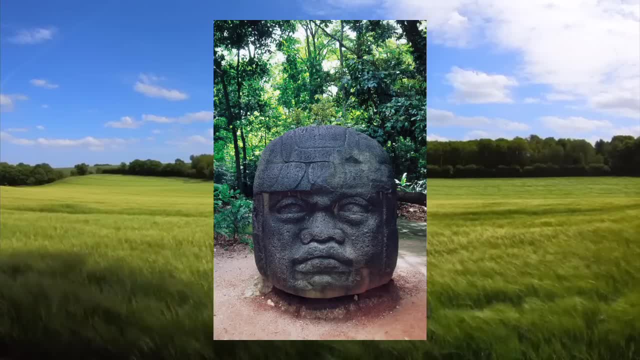 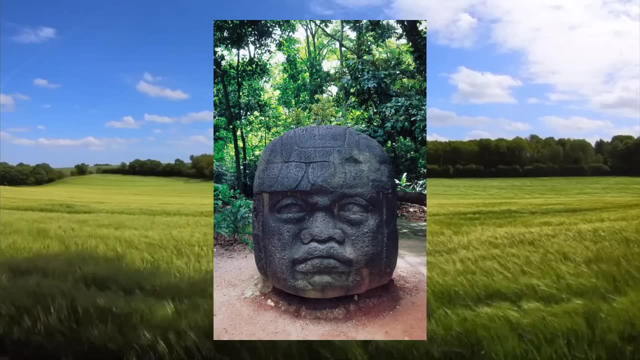 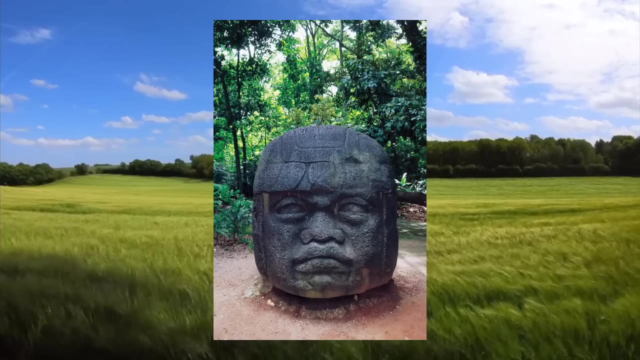 skills. The massive stone representations believed to depict Olmics rulers remain iconic symbols of their civilization. The ceremonial central of La Venta, featuring earthen mounds, pyramids and intricate draining systems, provide insight into the Olmics' architectural and engineering prowess. 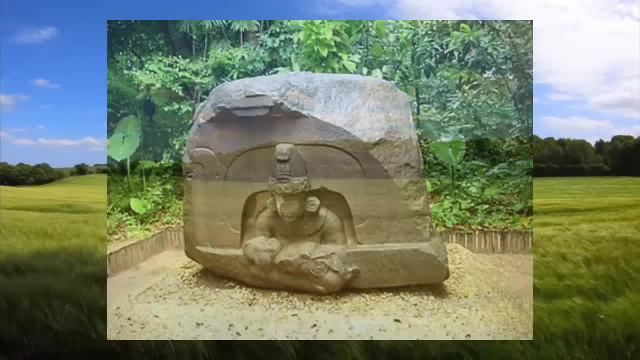 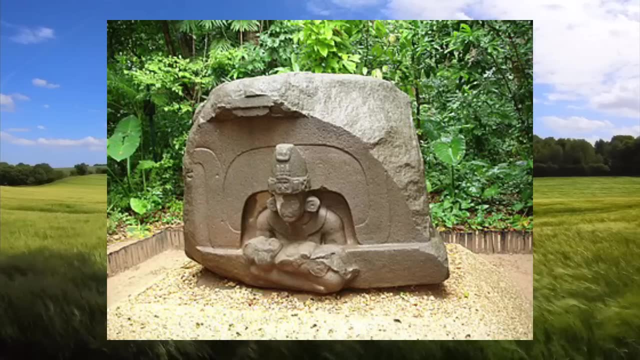 The Olmics emerged in agriculture, cultivating staple crops like maize beans and squash. Their society exhibited a complex societal structure with elite rulers, and their trade networks connected them with neighboring Mesoamerican cultures. While the Olmics are believed to have used a riding system, it remains undeciphered. 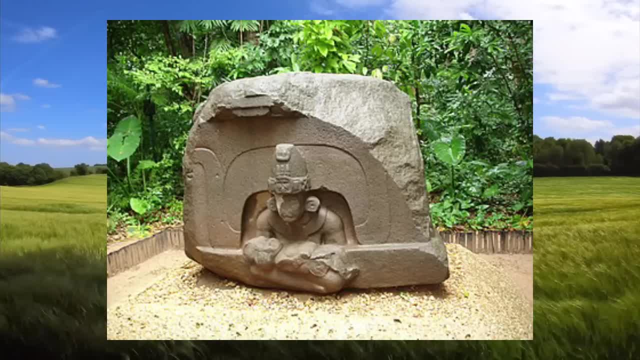 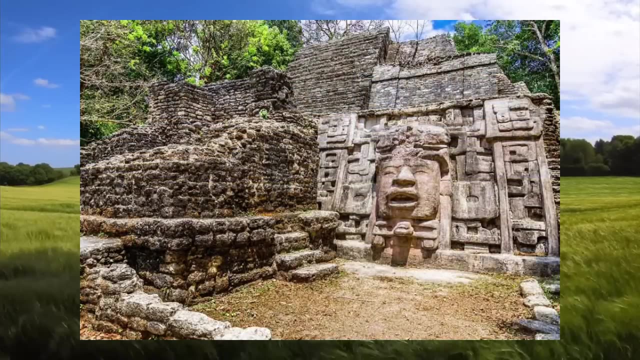 Necessitating a reliance on architectural discoveries for insights into their history and their culture. Around 400 BCE, the Olmics' civilization experienced a decline, and the reasons for this remain speculative Factors such as environmental changes possibly induced by volcanic activity or shifts in 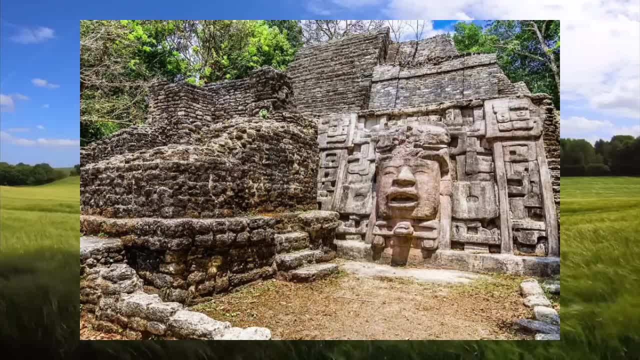 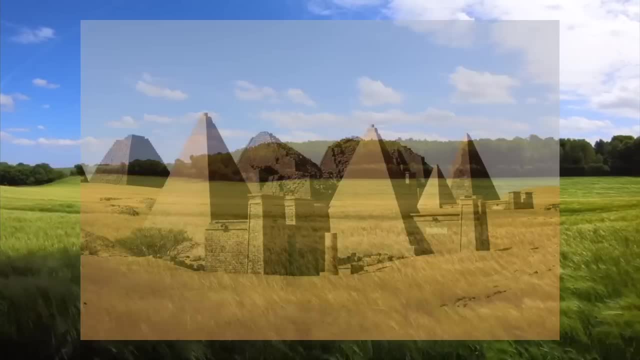 The Olmics were the first to establish the Olmics' cultural heritage. How did they establish their cultural heritage? First there is the Olmics Nubia. Nubia, an ancient region situated along the Nile River, holds a multifaceted history. 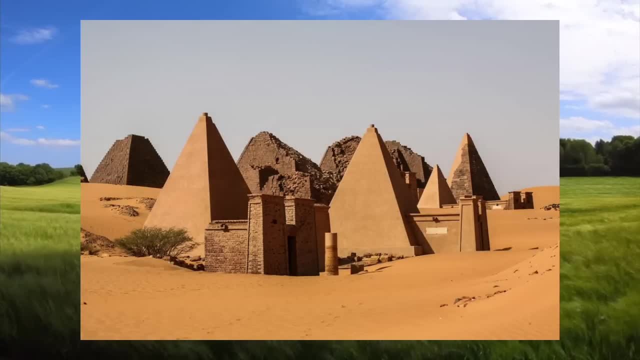 that spans millennia, Stretching from the first cataract in southern Egypt to the sixth cataract near Qahum, Sudan. Nubia served as a vital cultural and economic bridge between ancient Egypt and sub-Saharan Africa. The region's significance lies in its role as a trade hub for valuable commodities like 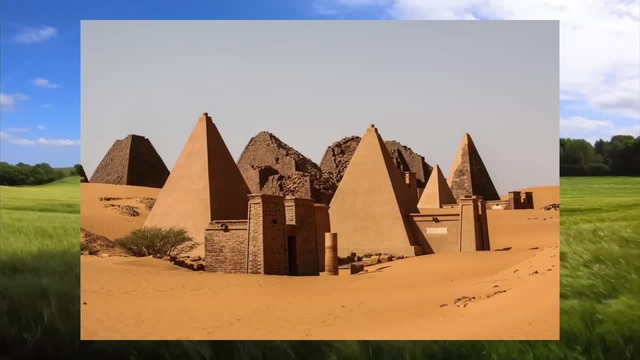 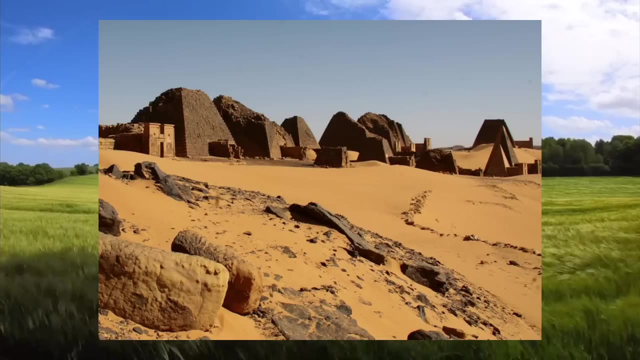 gold, ivory and ebony Since the Aztec period. the Olmics are important assets to bear, fostering cultural exchange beyond diverse civilizations. The early Kerma culture, dating all the way back to around 2500 BCE, marked one of the 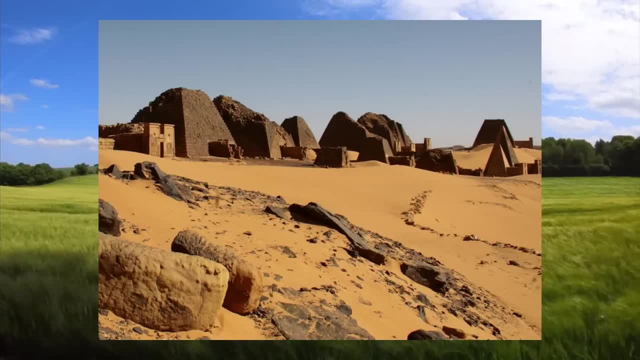 earliest complex societies in Nubia, Characterized by agricultural practices, pottery production and trade. subsequently, the Kingdom of Kush emerged around 1070 BCE, becoming a powerful state with its capital as Napata. During the 25th Dynasty, Kushanite kings even ruled over Egypt. 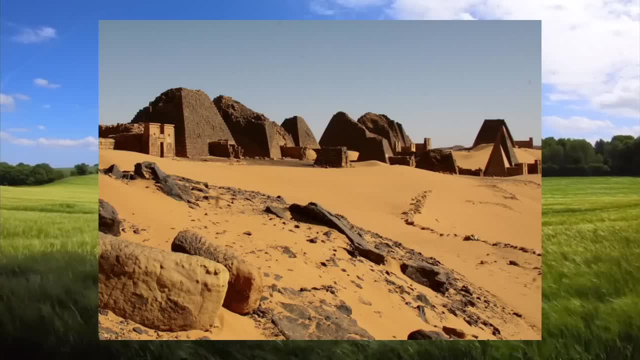 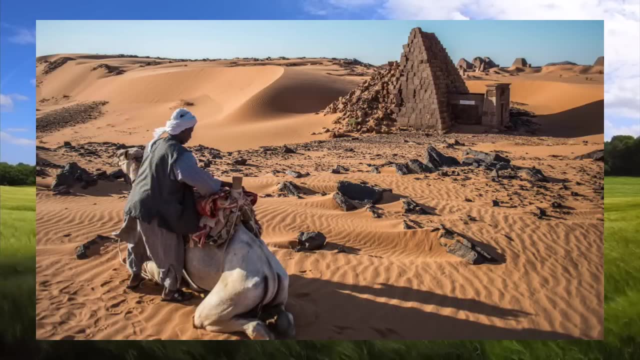 The Kingdom of Kush reached its 10th during the Metric Period when the capital shifted to Meroe. The Meroeic Strip, unique to the kingdom, remains one partially deciphered, adding an air of mystery to the historical record. 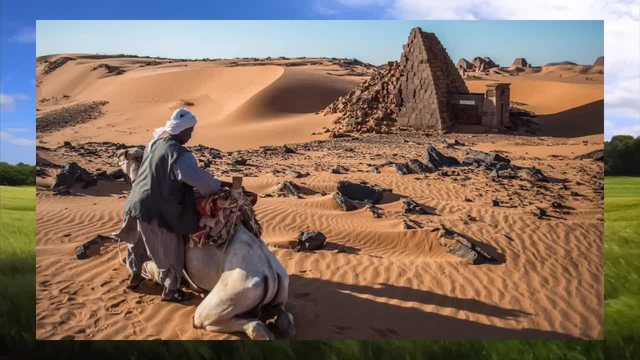 However, the decline of Kush occurred around the 4th century CE, influenced by changes in trade routes and the ascent of the Kingdom of Kumsum in Ethiopia. Nubia's historical trajectory continued as it underwent Christianization in the later centuries, becoming a significant center of Christianity. 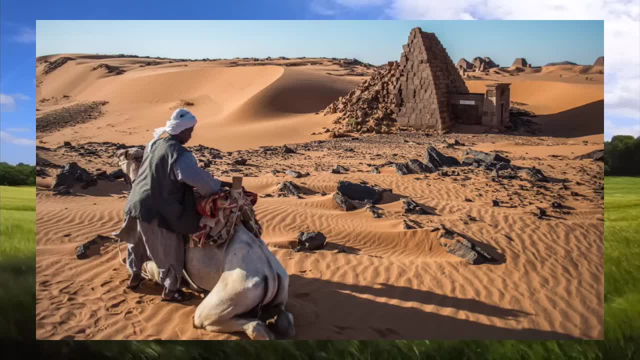 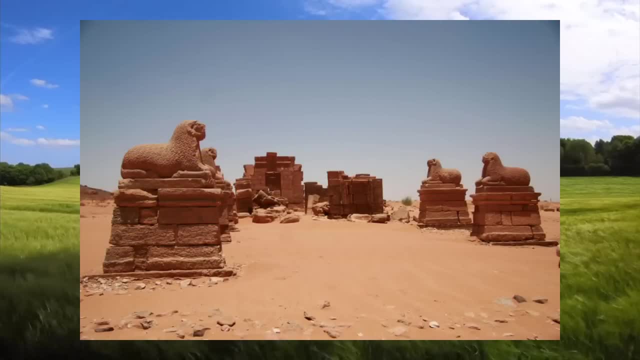 In Africa. the Christian Nubian kingdoms of Makuria and Alida maintained connections with both Byzantium and the Islamic world during the Medieval Period. Nubia's architectural sites, such as those at Kerma, Napata and Meroe, have provided. 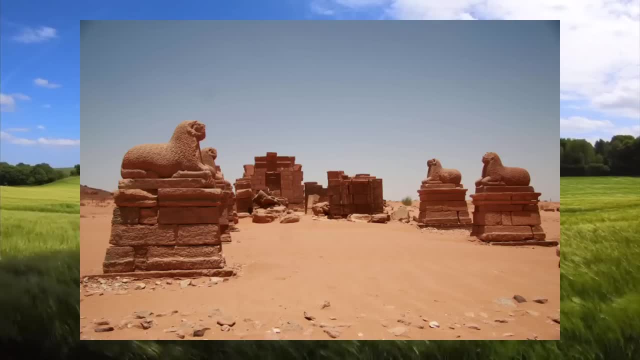 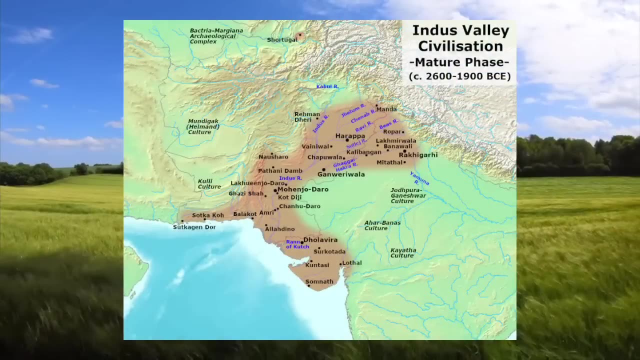 invaluable insights into the complexities of the ancient civilizations Indus Valley. The Indus Valley civilization, emerging in the 3rd millennium BCE, stands as one of the earliest urban civilizations in the world. It was founded in the northwestern part of the Indian subcontinent, encompassing a vast 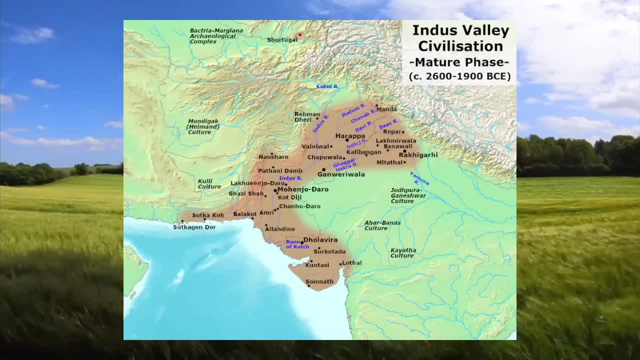 region that includes present-day Pakistan, India, Afghanistan and Iran. Its hallmark cities, such as Harappa and Mohenjo-Dario, exemplified remarkable urban planning and infrastructure in the once-ancient city. Streets laid out in grid pattern and an advanced drainage system showcased the civilization's 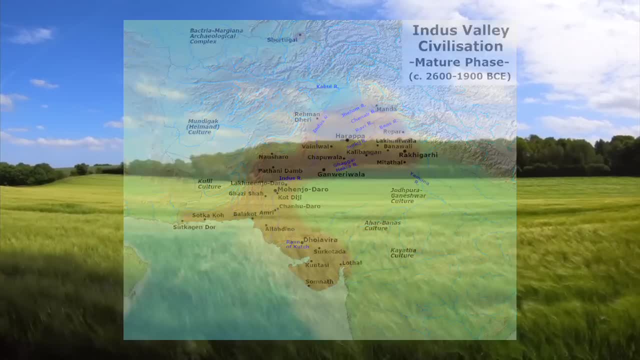 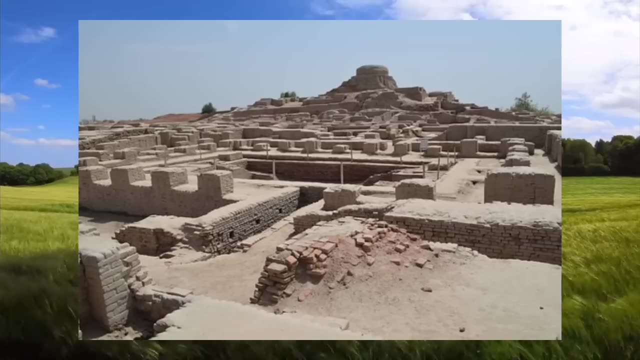 sophisticated approach to urban living, with the iconic Great Bath and Monero-Daro serving as a testament to their engineering prowess. One of the most enduring mysteries of the Indus Valley civilization lies in the undeciphered writing system. Despite the presence of a script on seals and artifacts, the absence of bilingual text, 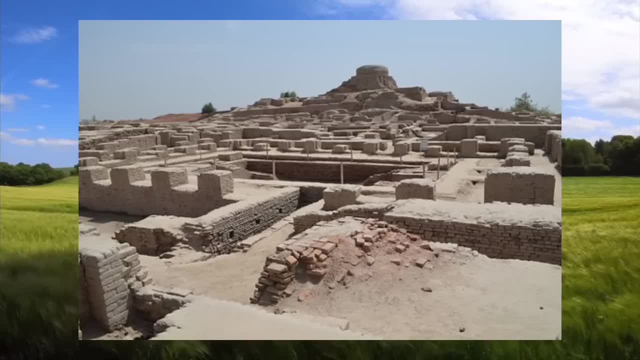 has hindered efforts to interpret this ancient writing. The civilization engaged in extensive trade connecting with distant regions like Mesopotamia. Architectural evidence points to a well-developed economic system, including standardized weights and measures, built upon an agricultural foundation. 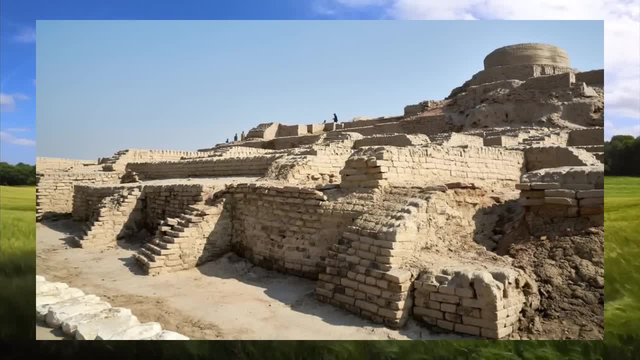 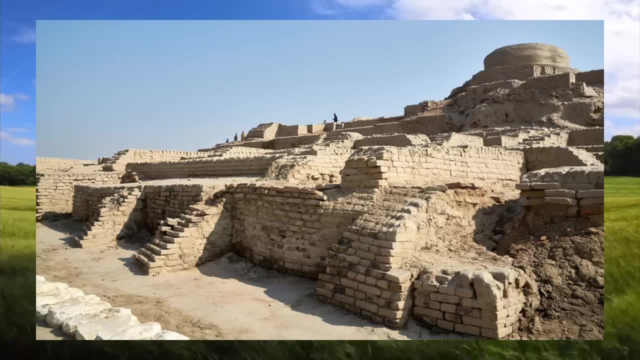 tered around 1900 BCE, and the exact cause remains speculative. Proposed factors include environmental changes, such as alterations in the course of the Indus River, alongside potential social, economic or political factors. The legacy of the Indus Rally: civilization endures. 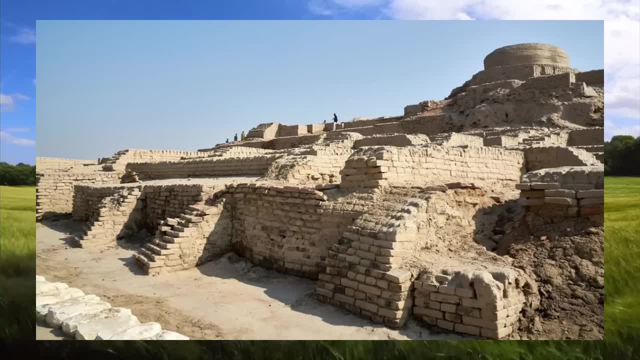 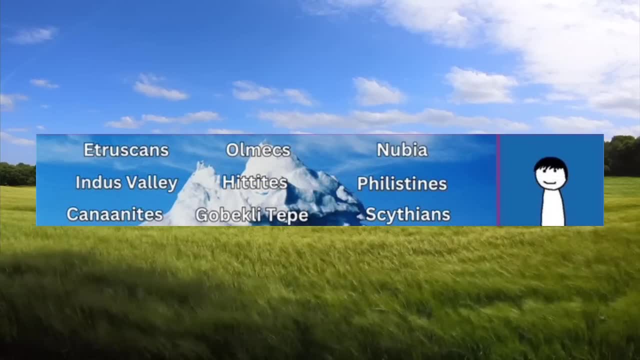 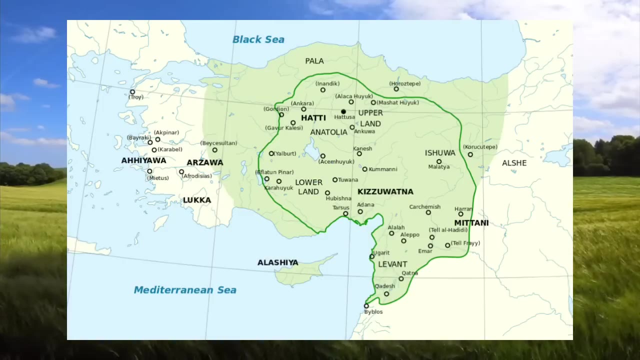 with its contributions to urban planning, trade and agriculture, laying the foundations for subsequent cultures in the Indian subcontinent. 7. Hittites The Hittites, an ancient Indo-European people, left an indelible mark on the history of the ancient Near East, Flourishing in Antolia, which is modern-day. 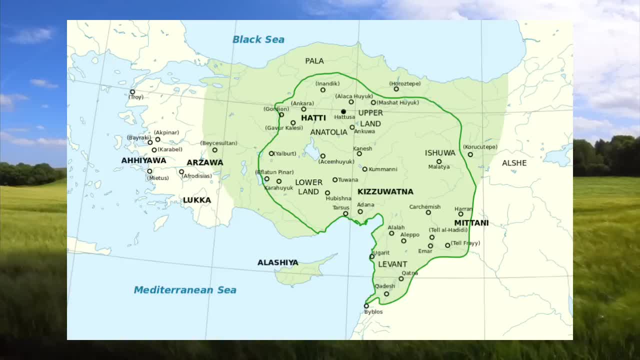 Turkey. the Hittites rose to prominence in the 17th century BCE during the Hittite Old Kingdom. Notable rulers like Hittites. I expanded Hittite territories, setting the stage for their power under Suplemia I and Merlissi II in the 14th century BCE. 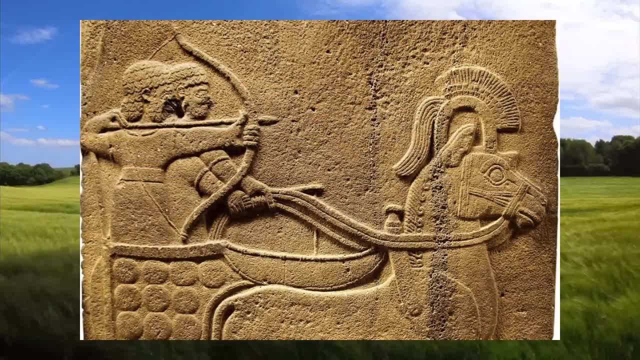 The Hittites were formidable empire builders, extending their influence into northern Syria and conquering Babylon. Their legal code, often referred to as the Laws of the Hittites, reflected a commitment to justice covering various different aspects of daily life and social interactions Engaged in conflicts with the Mitaini Kingdom. 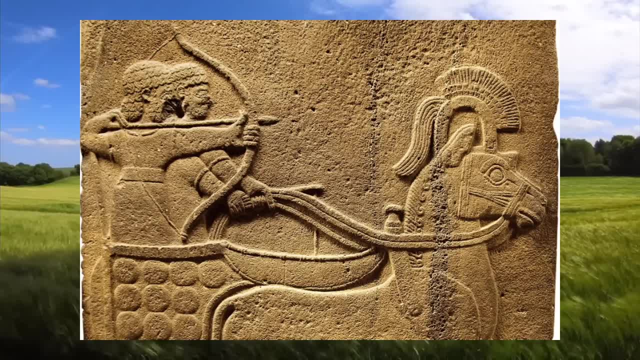 the Hittites were also party to the Treaty of Kadesh, one of the earliest surviving peace treaties signed with the Egyptians in the 13th century BCE. The Hittites' practice of the Hittites was a great success and the Hittites' practice of the Hittites' practice. 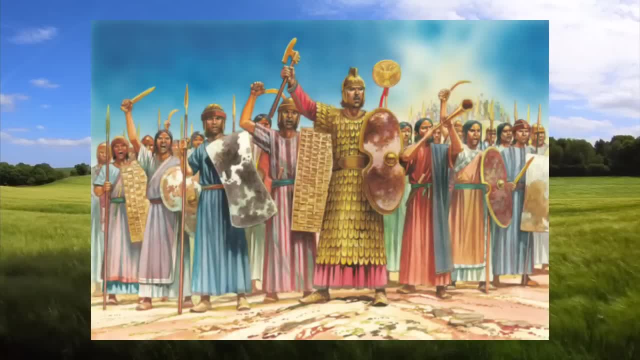 polytheistic religion worshipping deities in Teteshtub and Arniti. Their religious rituals involved elaborate ceremonies and offerings. After a period of decline, the Hittites experienced a resurgence in the 13th century BCE, known as the Hittites' New Kingdom, under King Suplemia II. 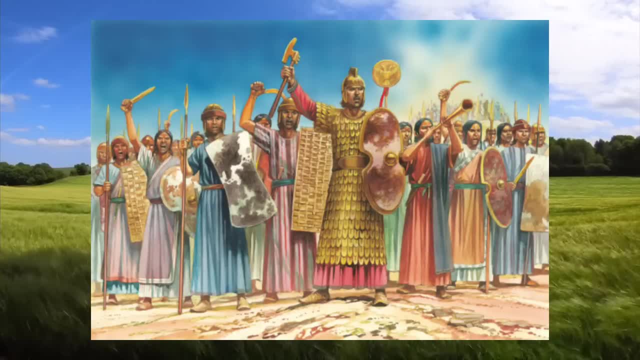 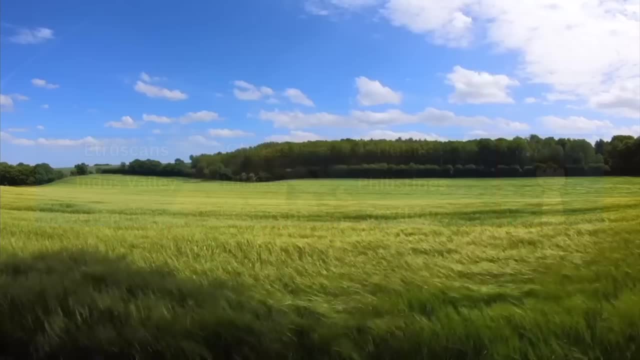 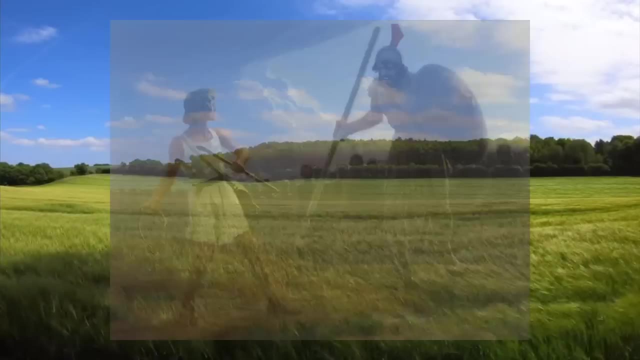 However, their empire ultimately collapsed around 1100 BCE during the Late Bronze Age, collapse attributed to internal strife, external invasions and broader disruptions. Philistines- The Philistines originating from the Aegean region migrated to the southern coast of Canaan. 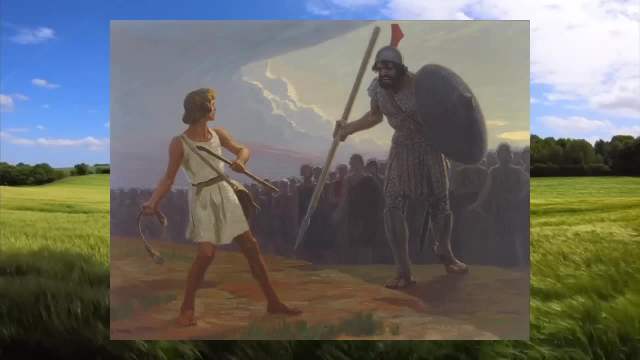 around the 12th century BCE, establishing a confederation of five major city-states: Ashkelon, Ashdod, Ekron, Gath and Gaza. Their prominence is vividly depicted in the biblical narrative, particularly in the context of conflicts with the Israelites, The Philistines. 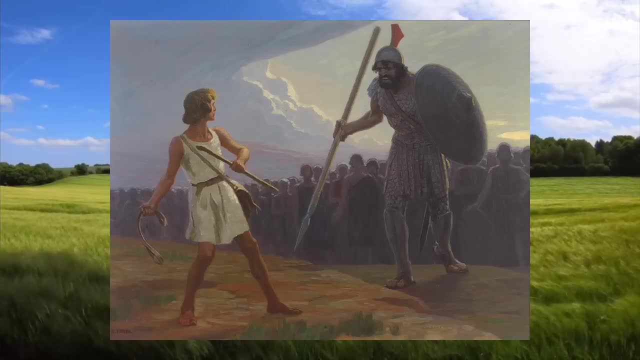 played a central role in episodes such as the Battle of Ephek and the capture of the Ark of the Covenant. Becoming architects of the Ark of the Covenant, the Philistines were the first to be architectural foes, With figures like the giant warrior Goliath symbolizing their formidable 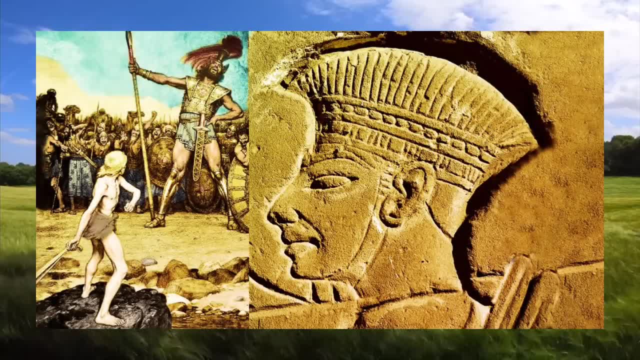 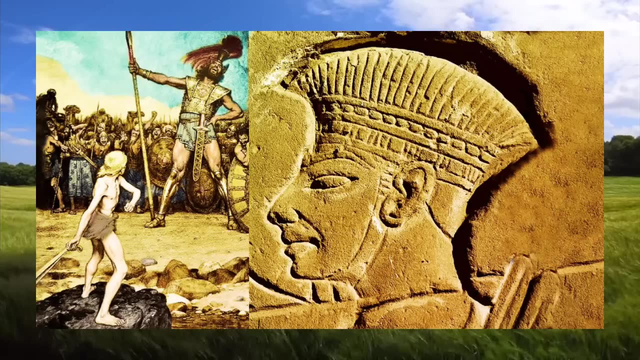 presence. known for their distinctive material culture, the Philistines left a tangible archaeological footprint, especially in pottery adorned with unique motifs. The cities they founded were centers of daily life, and excavations have uncovered evidence of houses, tools and religious practices. Despite their adversarial relationship with the Israelites, 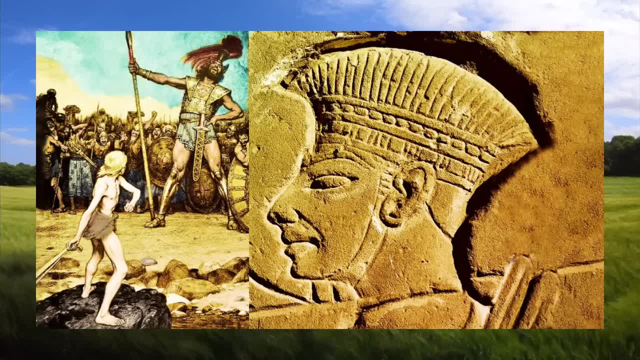 there was cultural exchange, as seen in the adoption of certain Philistine pottery styles and iconography influencing Israelite art. The biblical story of Samson, a judge renowned for his strength, is entwined with the Philistines, featuring episodes of conflict and intrigue with each other, including Samson's relationship with Delilah. However, the power of the Philistine city-states waned in the 7th century BCE due to the expansion of the Neo-Asryan Empire. Cities like Ashkelon faced destruction by the Assyrians in 604 BCE, marking the decline of the Philistine. 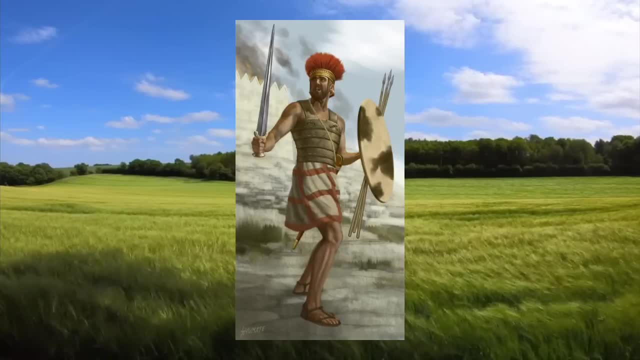 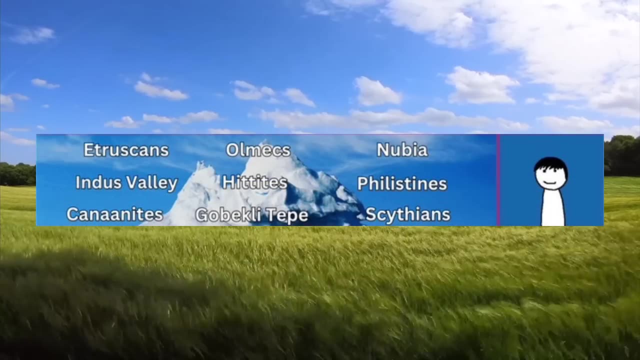 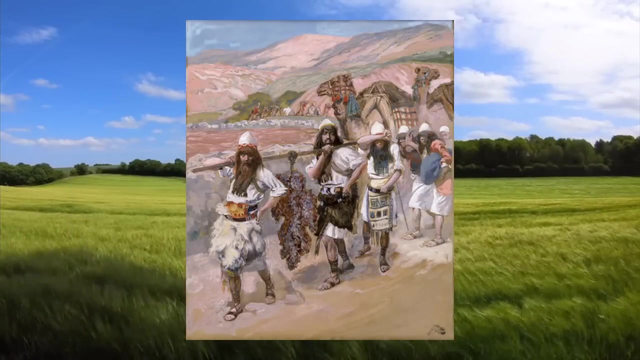 influence. The legacy of the Philistines is much more important than the history of the Philistines, as it is a cultural and historical tapestry of the Eastern Mediterranean CANONITES- The Canonites, an ancient Semitic-speaking people, occupied the land of Canaan, a strategic region. 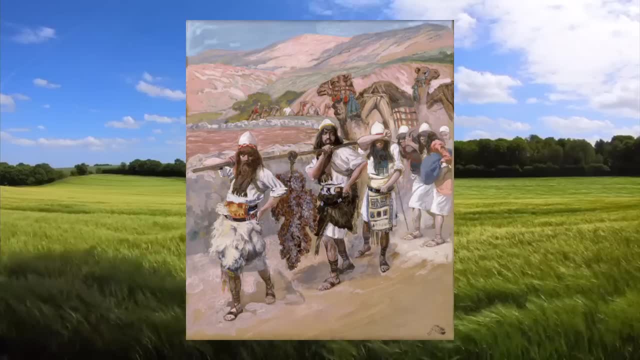 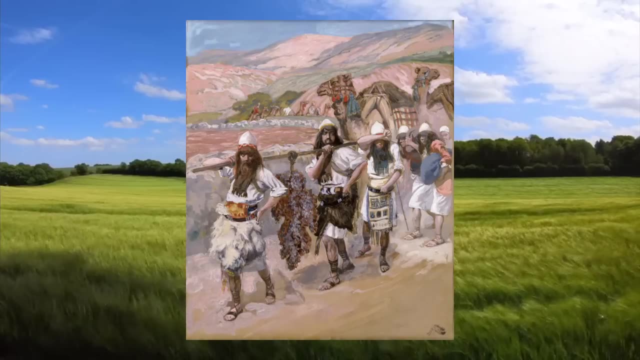 connecting Egypt and Mesopotamia, Organized into city-states with distinct rulers and local deities. prominent cities like Irrigate, Biblios, Tyre and Sidon flourished. Known for their active trade, the Canonites engaged with neighboring civilizations such as the Scythians. the Scythians, the Scythians. 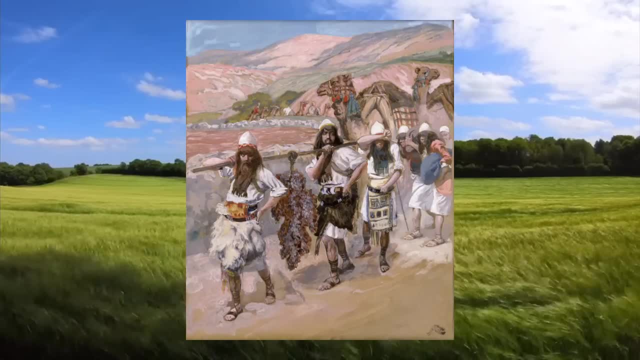 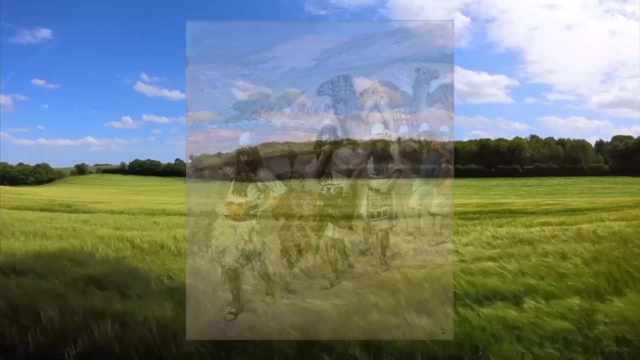 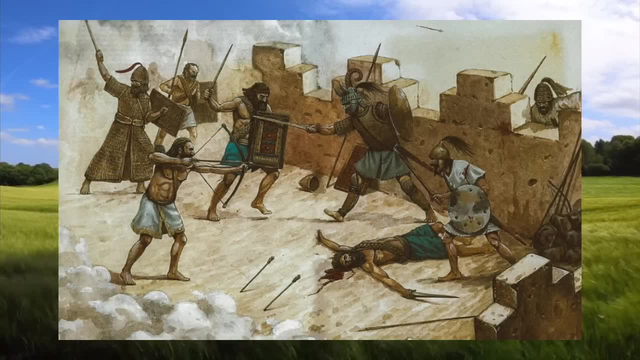 incorporating fertility rites and animal sacrifices. Culturally, the Canonites made significant contributions, including the development of an early alphabetic writing system that influenced later scripts. Biblical narratives portrayed the Canonites as inhabitants of the Promised Land, setting the stage for conflicts with the Israelites, the Scythians, the Scythians and the. 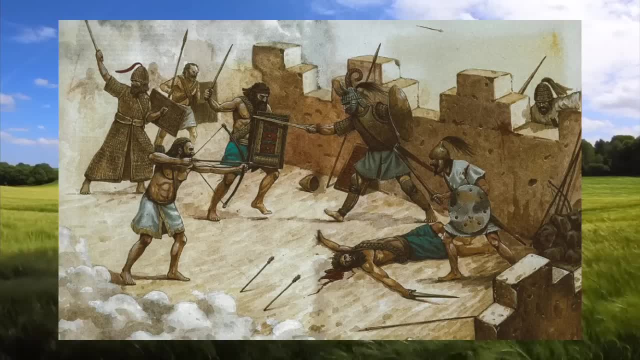 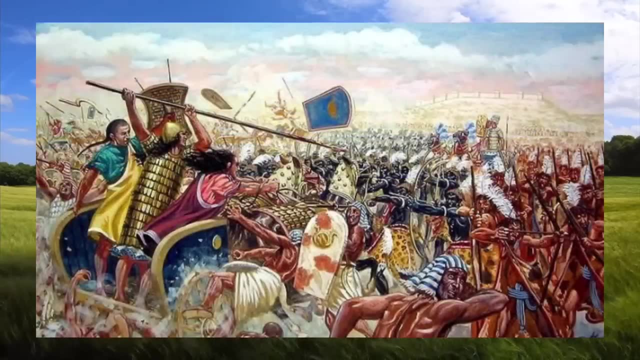 Israelites. The Bible, particularly the Old Testament, highlights the conquest of Canaan as a central theme in Israelite history. The decline of the Canaanites unfolded over centuries, influenced by external invasions, conflict with neighboring powers and shifts in trade routes. 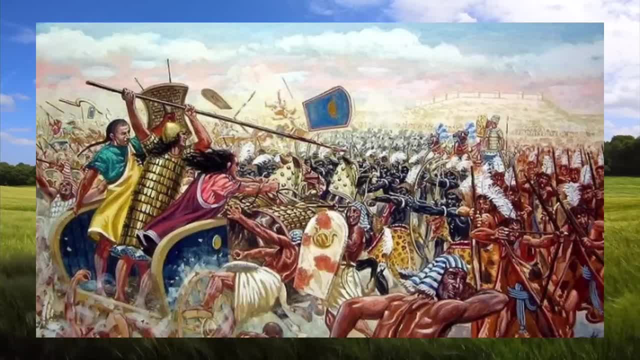 Despite the political decline, their culture and religious influence persisted through subsequent civilizations. The Bohesians, considered descendants of the Canaanites, played a crucial role in maritime trade and colonization, leaving a lasting impact on the Mediterranean world. Architectural excavations in the region have unearthed Canaanite artifacts. 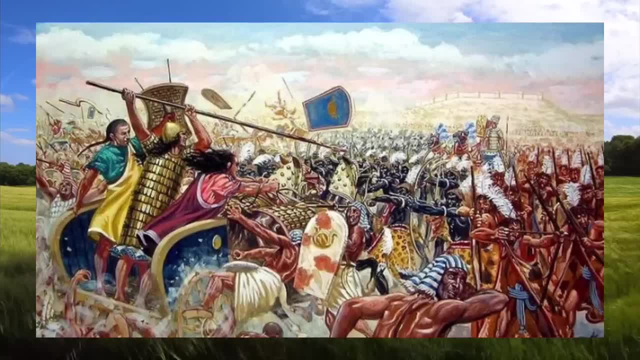 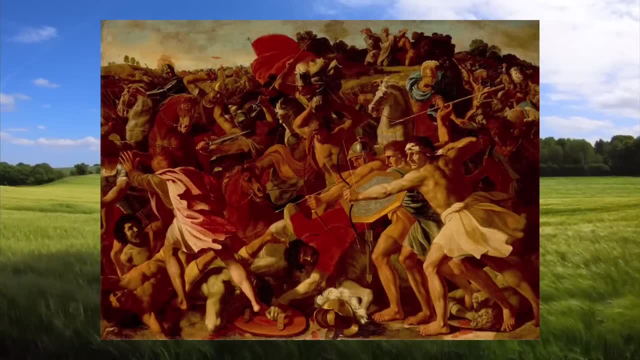 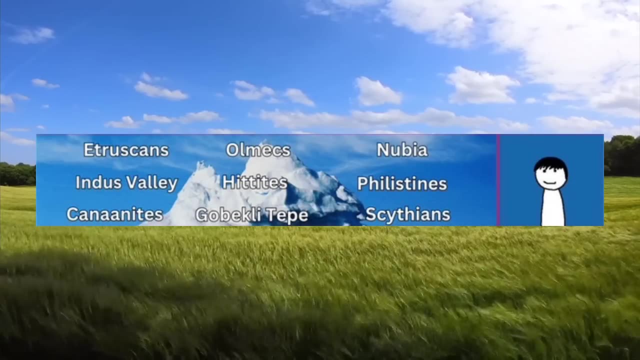 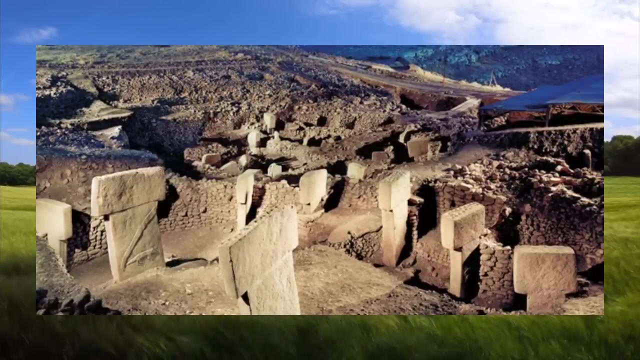 providing insights into their daily life, religious practices and material culture. The Canaanites, situated at the crossroads of ancient civilizations, played a pivotal role in shaping the cultural, religious and historical shape of the eastern Mediterranean. Gobekli Tepe, situated in southeastern Turkey, stands as a testament to the ancient Greek civilization of the Middle East. It is believed that the Canaanites, the Canaanites and the Canaanites were the first to establish the ancient Injuidity of its builders, Dating all the way back to the 10th and 9th millennium BCE. it ranks among the world's 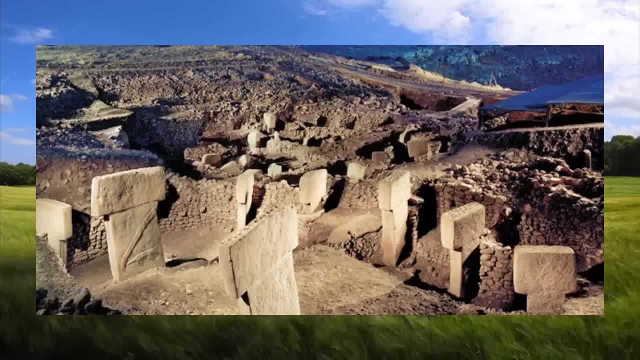 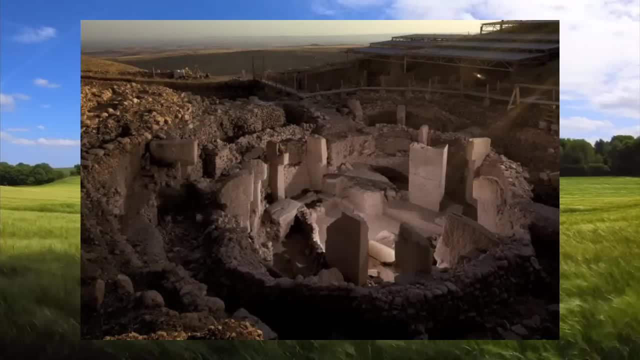 oldest monumental structures, comprising circular and oval-shaped structures with massive limestone pillars adorned with intricate carvings of animals and symbols. Gobekli Tepe challenges conventional notions about the capabilities of ancient hunter-gatherer societies. The purpose of Gobekli Tepe remains a subject of scholarly inquiry, with the prevailing consensus that it 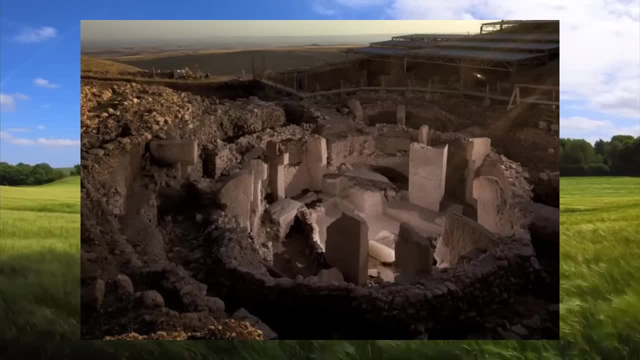 served as a ceremonial and cultural center for the Canaanites. The Gobekli Tepe, which is a symbol of civilization, is a symbol of the ancient civilization of the Middle East. Its alignment with celestial events suggests a possible astronomical connection, While the 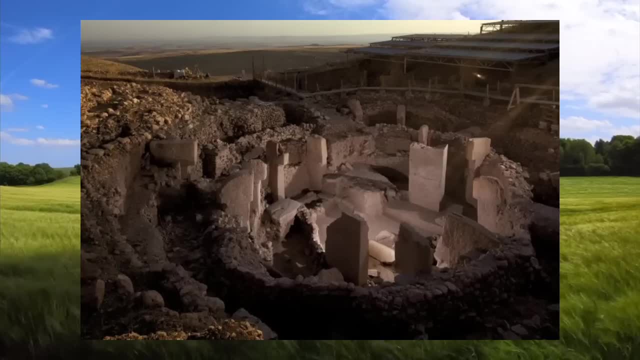 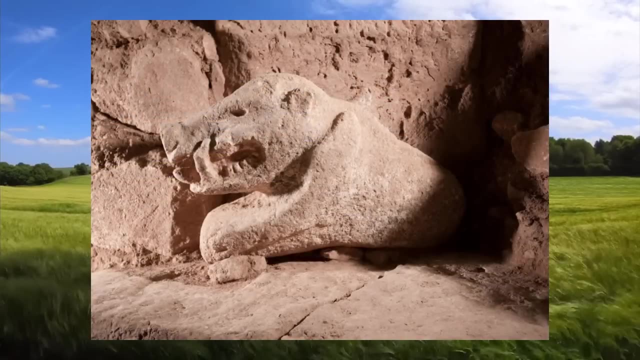 carvings of animals and abstract symbols on the pillars provide glimpses into the religious or symbolic beliefs of its builders. constructed by a community of hunter-gatherers, the site's complexity and scale underscores a high level of organization and communal effort. Its discovery in 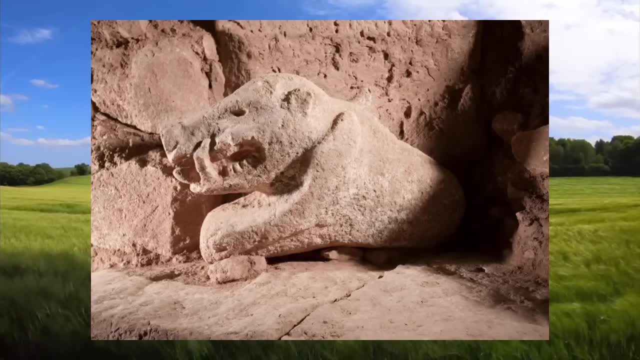 the 1990s, followed by the excavations led by Klaus Schmidt, has reshaped our understanding of early human history. The site's history is a great example of how the Gobekli Tepe was built and how it was built. The significance of Gobekli Tepe lies in its challenge to establish 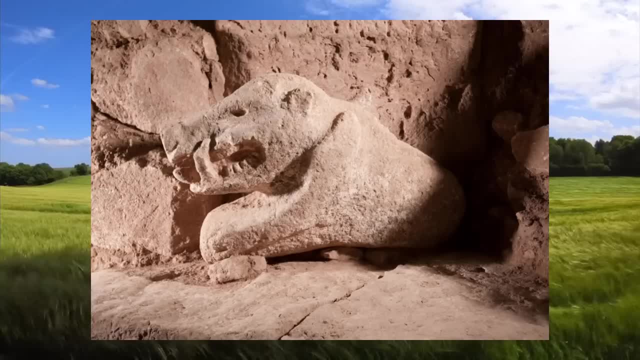 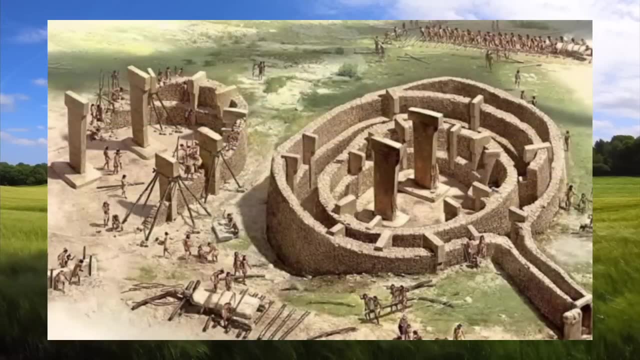 narratives about the development of complex societies and the relationship between agriculture and monumental architecture in early humans. The deliberate burial of Gobekli Tepe raises intriguing questions about the reasons for its abandonment and why they buried it, or who even buried it. It stands as a World Heritage Site and ongoing research continues. 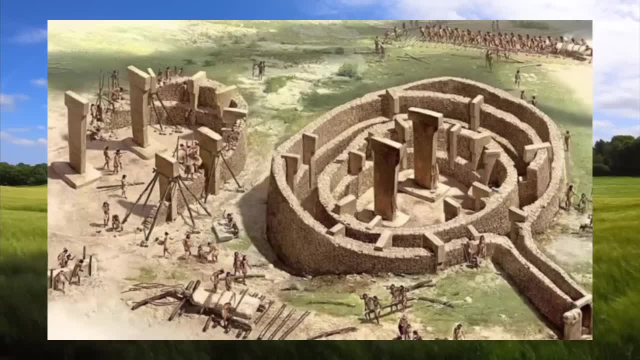 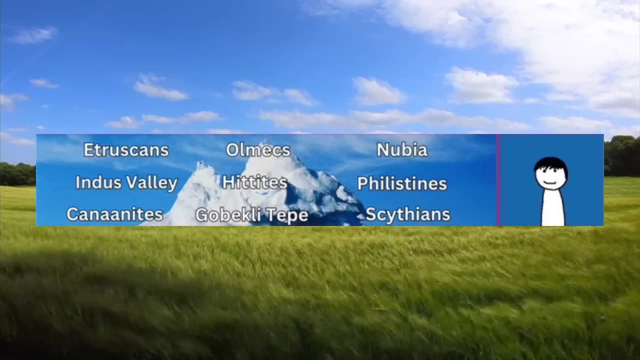 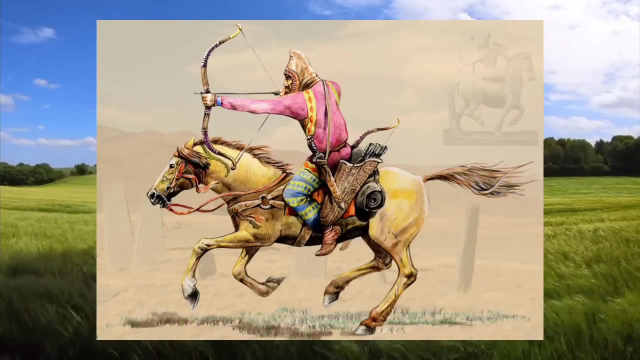 to unravel the mysteries surrounding this ancient marvel. Gobekli Tepe has become a focal point for understanding the social, religious and technological dynamics of a distant epoch, offering profound insights into the evolution of human civilization and where it really started. The Scythians, an ancient group of Iranian nomads, held sway over the vast Eurasian steppes from the 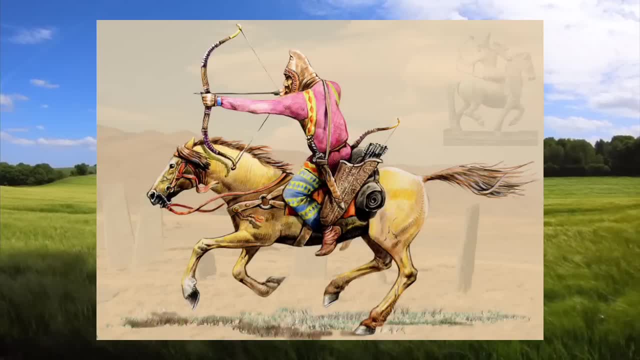 7th century BCE to the 3rd century CE. Originating in the regions around the northern Black Sea, they were nomadic pastoralists Adept at horse breeding and herding. their distinctive lifestyle, characterized by mobility and seasonal migrations, played a crucial role in shaping their identity. Renowned for their 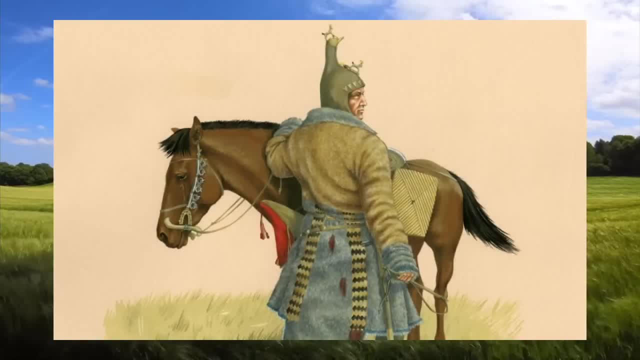 formidable warrior culture. the Scythians were particularly skilled in mounted archery, utilizing composite bows to shoot arrows from horseback. This prowess made them a formidable force in the eyes of their contemporaries, including the Greeks and the Persians. Ancient writings, such as those by Herodotus, provide insights into their nomadic existence. 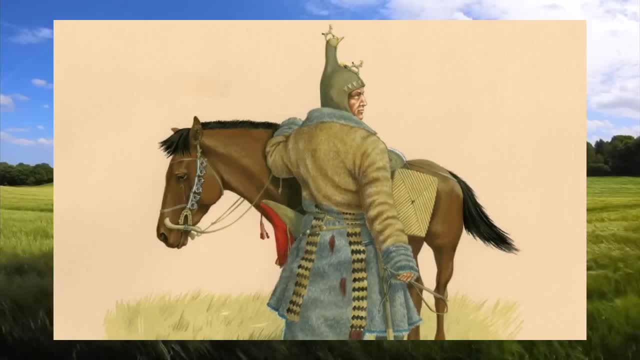 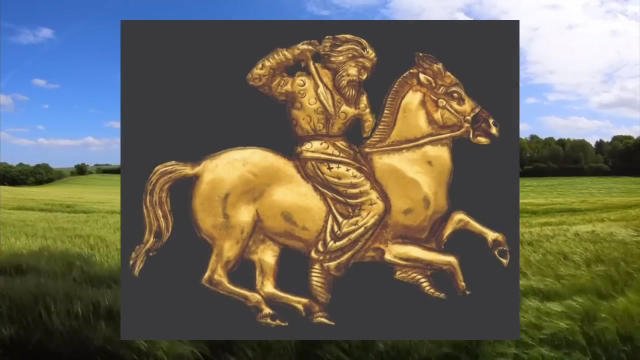 and martial achievements. The architectural record of the Scythians is marked by their distinctive burial practices, notably the kurgans or burial mounds. These sites, rich in grave goods, offer a glimpse into their material culture and customs. The Peseric burials in the Atalaya Mountains, featuring well-preserved mummies and elaborate 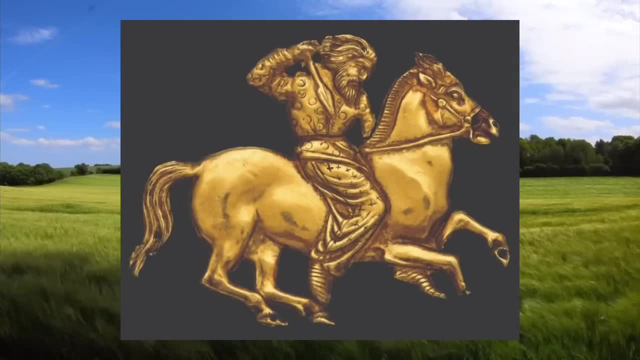 artifacts are particularly significant for understanding Scythian traditions. Interacting with neighboring civilizations, the Scythians left an imprint on their cultural landscape. Their legacy extends to the Scythians who were the first Scythians to be born. They were the first. Scythians to be born. They were the first Scythians to be born. They were the first Scythians to be born to art, mythology and military tactics influencing subsequent civilizations. The Scythians were part of a broader cultural group that included the Saka and the Sirmashans. 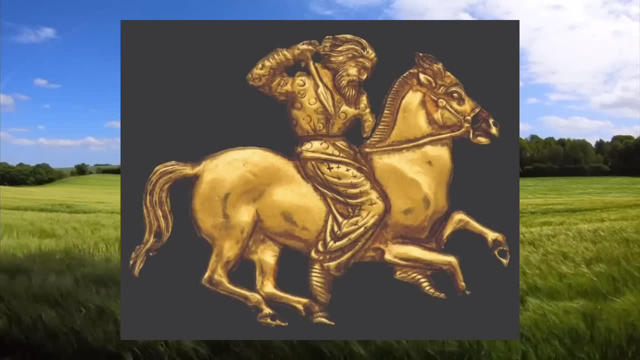 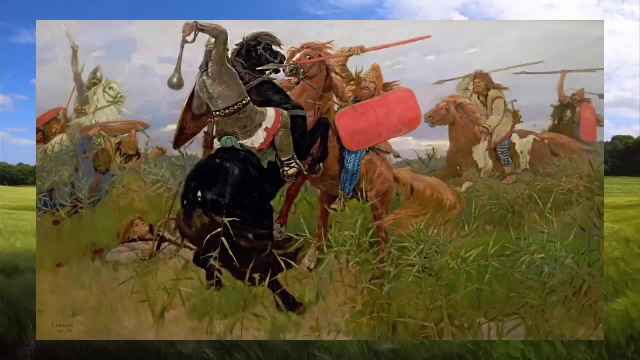 collectively known as the Scytho-Siberian cultures. Despite their cultural and military prowess, the Scythians faced decline due to various different factors, including pressure from other nomadic groups, conflicts with settled societies and environmental changes in the Eurasian steppes. Archaeological discoveries in the 20th and 21st centuries have played a crucial 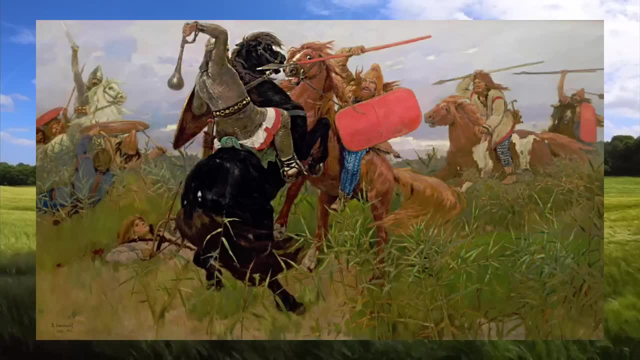 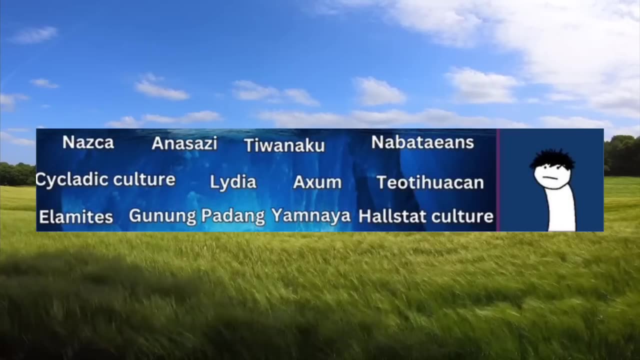 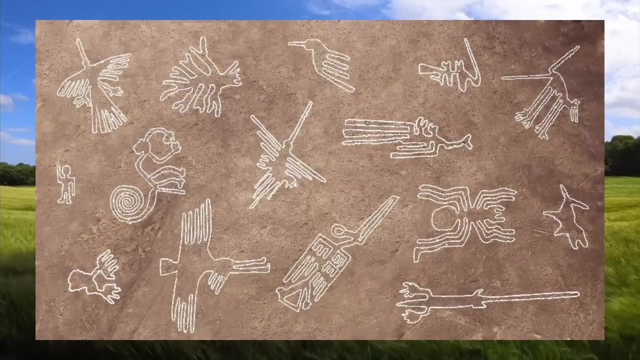 role in unraveling the mystery of the Scythian culture. The Scythians were part of a broader of the Scythian history, providing modern scholars with valuable artifacts and insights into their complex and dynamic civilizations. Tier 3. Nazca: The Nazca civilization flourishing along the arid coastal region of southern Peru. 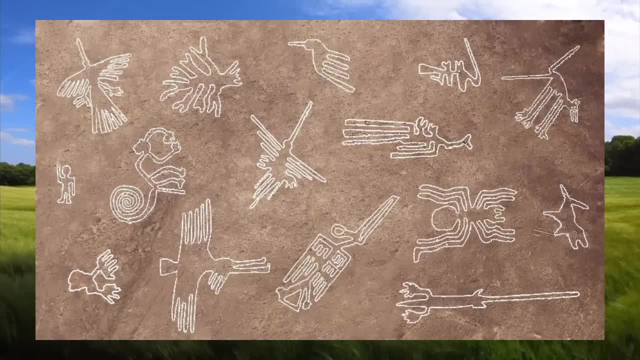 from 200 BCE to 600 CE, is best known for the enigmatic Nazca lines, colossal geoglyphs etched into the desert floor. These lines featuring animals, plants and geometric patterns spark speculation and their purpose, with theories ranging from 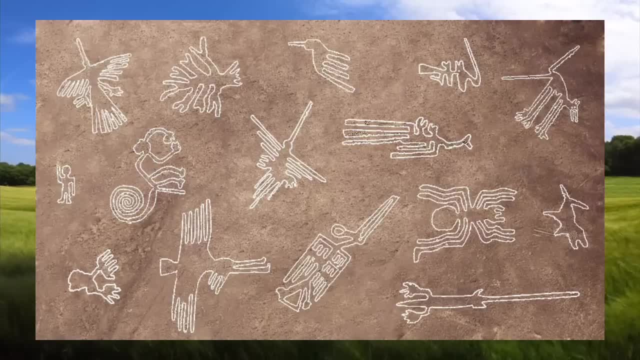 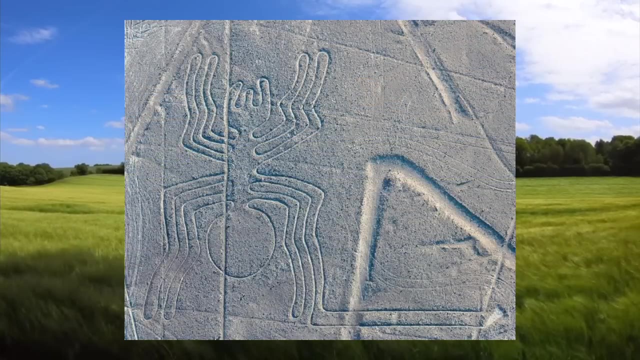 religious and ceremonial significance to alignments with astronomical phenomena. The Nazca people, adept at harnesting water in their arid environment, engineered sophisticated underground aqueducts, known as puquillos, to support agriculture. Artistically, the Nazca were accomplished poet-editors and weavers These ceramics. 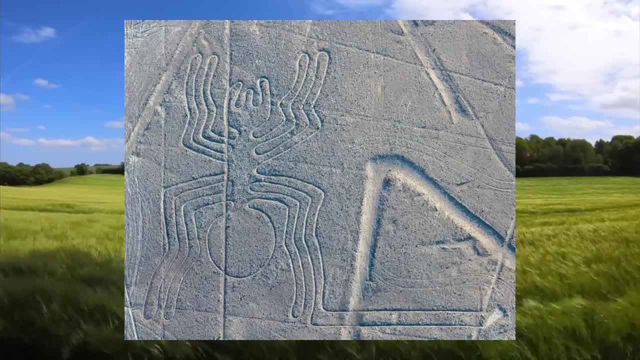 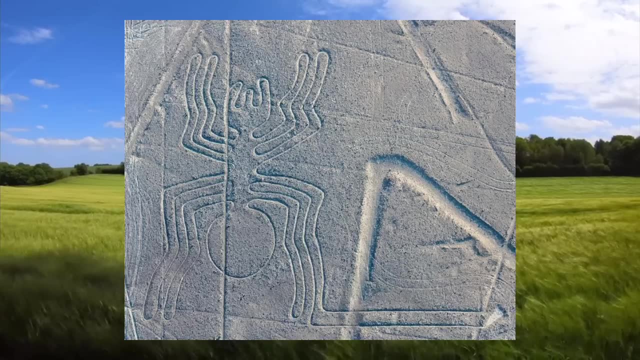 exhibited intricate designs and polychrome decorations, often depicting mythological and religious beliefs. The Nazca people were also known for their artistic and cultural themes. Nazca textiles, renowned for their complexity and vibrant colors, featured images of animals, plants and mythical beings. Ceremonial centers like Cahuji, which is an adobe pyramids. 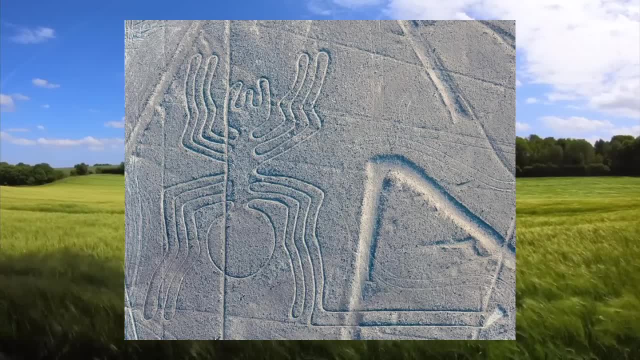 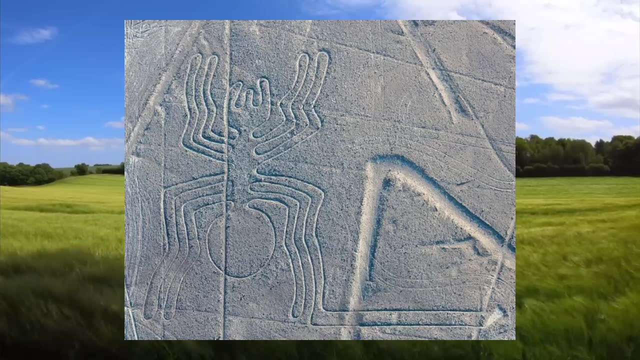 and platform mounds played a central role in Nazca religious rituals and administration. The decline of the Nazca civilization around 600 CE remains a puzzle and no one really knows what happened to them, with factors like environmental changes and social shifts likely contributing to. their end. The Nazca civilization, flourishing along the arid coastal region of southern Peru, is best known for their artistic and cultural themes. The Nazca people adept at harnesting water in the holy land of the island are often followed by physicists and sculptors. The Nazca people 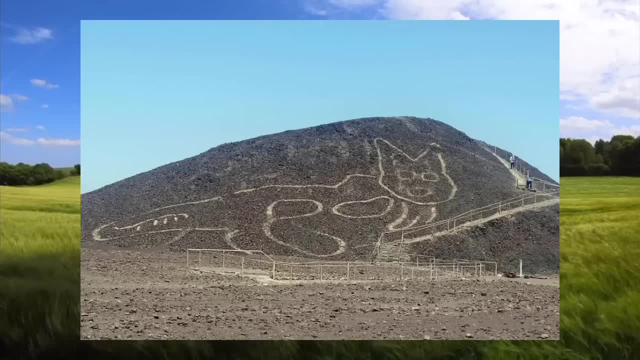 are among the most זalim in our region, but have always been usually as unique as the Arcoo people. This is due to their unique style in the area, including the Kiloa culture, which is often the most traditional and modern mani culture. 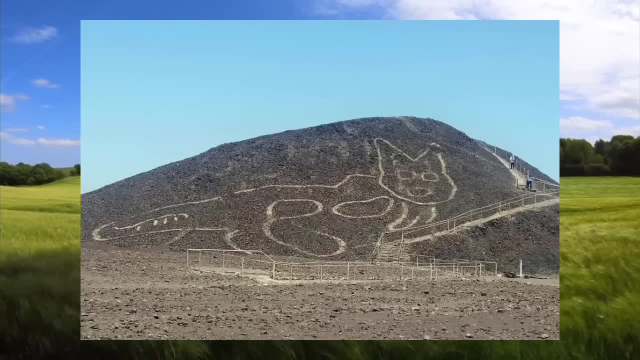 Ongoing architectural research, including excavations at sites such as Cahuji, continues to unravel the mysteries surrounding the Nazca people, shedding light on their daily lives, their cultural practices and technological advancements that then the natives would know. Anasazi. 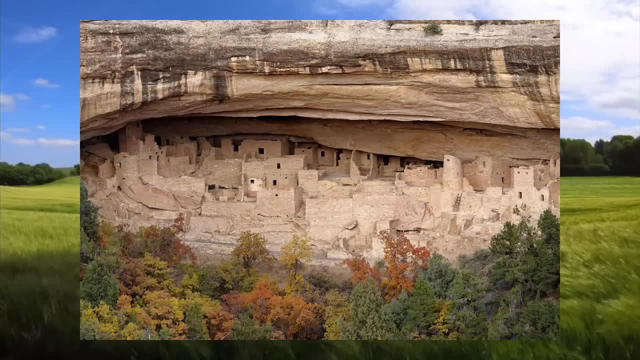 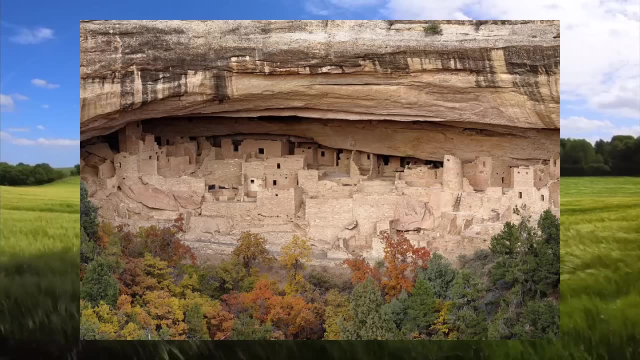 The ancestral Puebloans, commonly known as the Anasazi, were an ancient Native American culture that thrived in the Four Corners region of southwestern India, United States. Renowned for their distinctive architecture, they left a lasting mark with cliff. 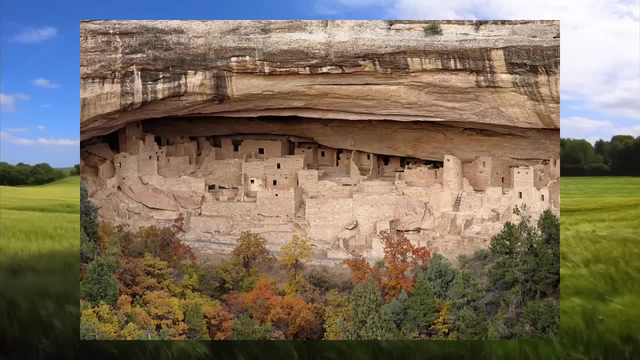 dwellings and multi-story pueblos, particularly notable at sites like Mesa Verde, Chaco Canyon and Canyon de Chile. This cultural evolution of the ancestral Puebloans, including periods like the Basketmaker and Pueblo, with advancements in construction techniques and pottery, evident. 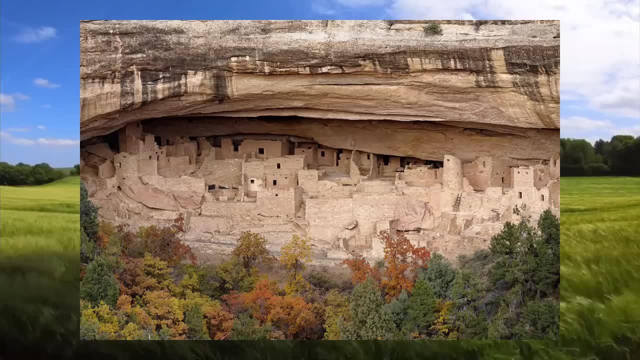 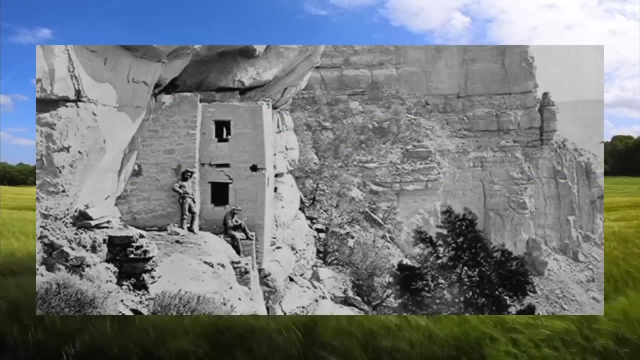 in the latter, Archiculturally adept, the ancestral Puebloans cultivated maize beans and squash, developing sophisticated water conservation methods in the arid environment. Trade networks centered around hubs like Chaco Canyon facilitated the exchange of goods, including turquoise shells and pottery. The construction of cavaz subterranean ceremonial 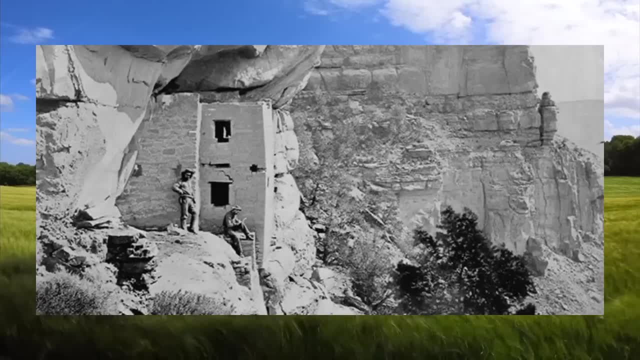 structures reflected their complex belief systems and participation in rituals linked to the agriculture, celestial observations and community cohesion. By the late 1200s, the ancestral Puebloan population declined, possibly due to environmental changes, resource depletion and other social factors. Some communities migrated southward. 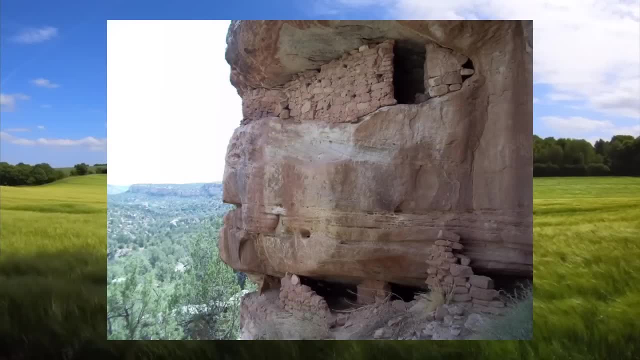 contributing to the formation of modern Puebloan tribes. The rock art left behind, including pedioglyphs and pictoglyphs, serves as a testament to the cultural richness and spiritual expressions And I think these things look so cool and it's crazy how they even built. 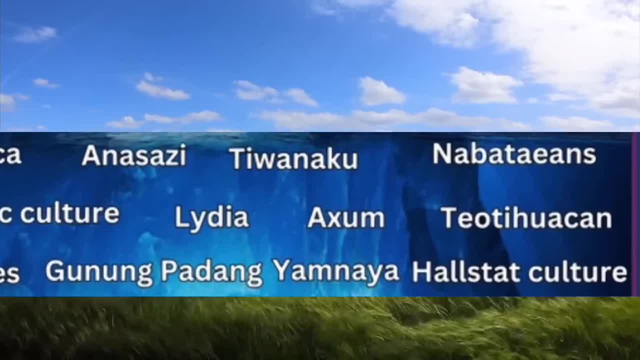 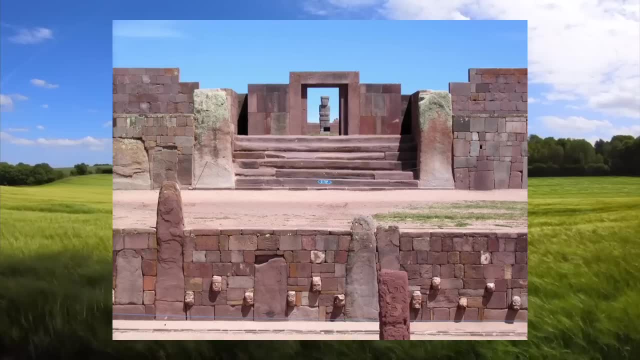 them. Tawenaku, the capital of the ancient Tawenaku civilization, is situated on the Bolivian Alley. Tawenaku is the capital of the ancient Tawenaku civilization and is located on the Tapano near Lake Titicaca. Thriving around 300 BCE to 1100 CE, Tawenaku served as a significant 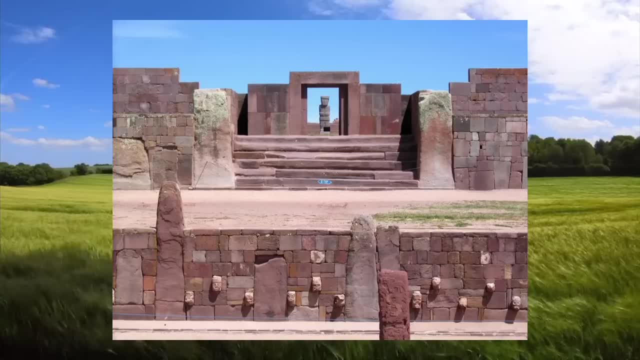 cultural and economic hub, influencing the Andean region's religious, artistic and architectural practices. The site's strategic location facilitated agriculture through sophisticated water management systems, showcasing the Tawenaku people's adeptness at cultivating crops in the high-altitude environment. Architecturally, the Tawenaku is renowned for its monumental structures. 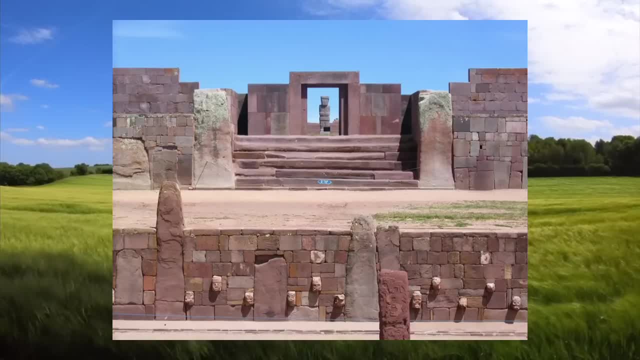 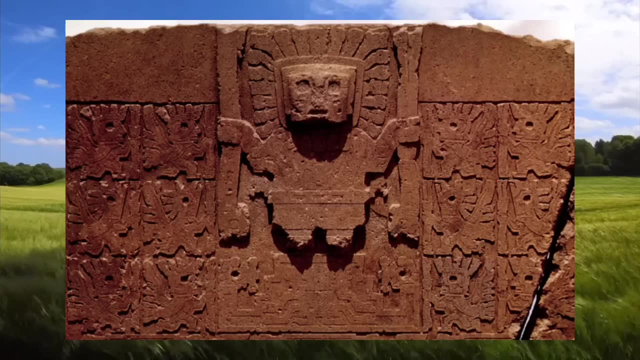 including the Kanapa Pyramid and the Poma-Panku Complex. These showcase advanced engineering skills, precision, stone-cutting and the use of massive stones. The site's religious significance is evident in features like sunken courts, terraces and the iconic Gateway of the Sun, adorned with 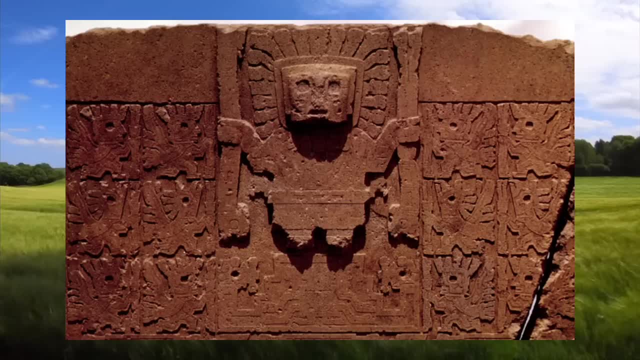 intricate carvings linked to ceremonial and religious practices. Tawenaku art reflects distinctive iconography featuring human-like figures with elaborate headdresses and animal motifs, providing insights into the civilization's religious and cultural values. The site's historical and archaeological heritage is a symbol of the Tawenaku people's religious and 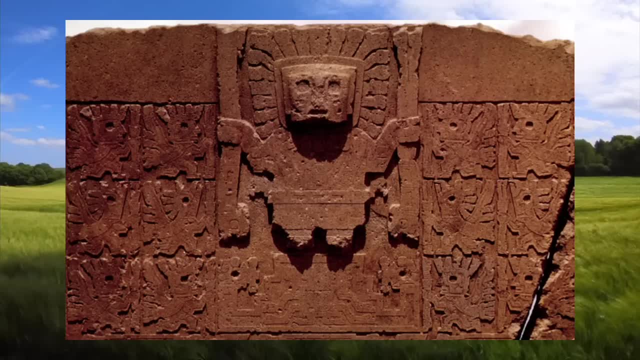 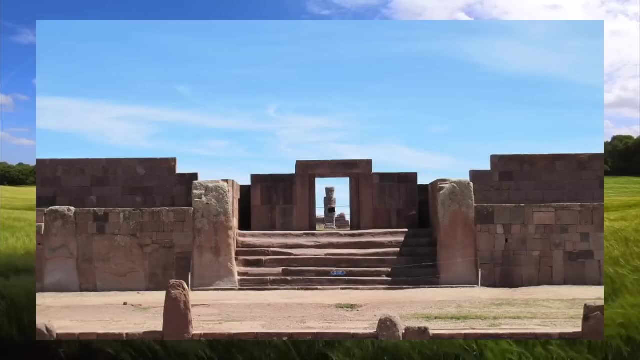 theological beliefs. Despite its decline around the 11th century, Tawenaku's legacy endured through subsequent Andean cultures. The Inca, in particular, held Tawenaku in reference, incorporating elements of its agriculture and other art into their structures. The reason for Tawenaku's decline: 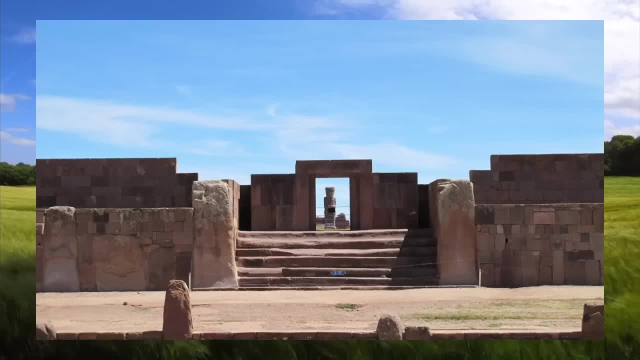 remains complex, possibly involving environmental changes, resource depletion and internal factors. Ongoing architectural investigations continue to unveil new discoveries, enriching our understanding of the Tawenaku civilization. In its contributions to the cultural tapestry of the Andean region, Tawenaku stands as a testament. 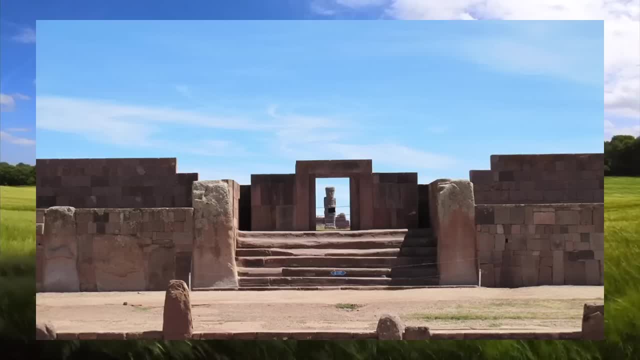 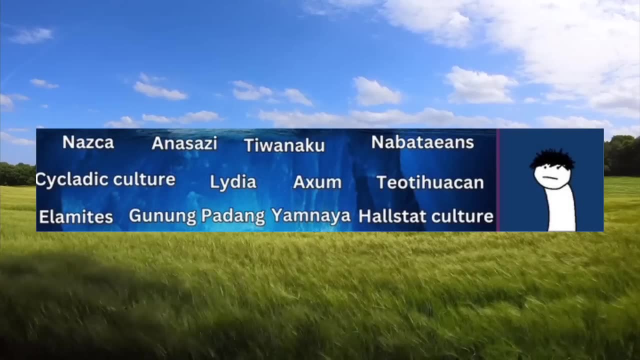 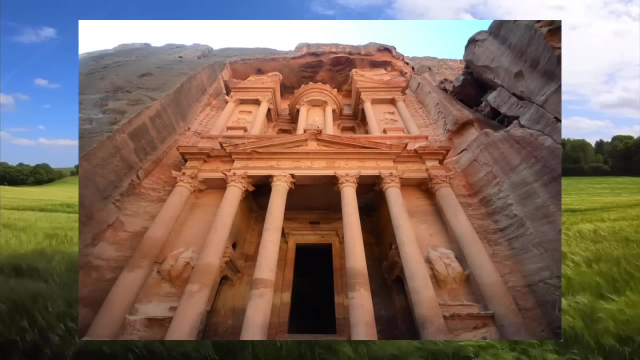 to the ingenuity and the cultural achievements of ancient Andean societies, leaving an impact on the archaeological and historical landscape of South America. Nabateans- The Nabateans, an ancient Arab people, thrived in the crossroads of northern Arabia and southern Levant, establishing a prominent kingdom with Petra as its capital. Petra, the jewel of Nabatean architecture, is renowned for its rock-cut structures, including the iconic alkanauts and the monastery. The Nabateans capitalized on their strategic location along major trade routes. 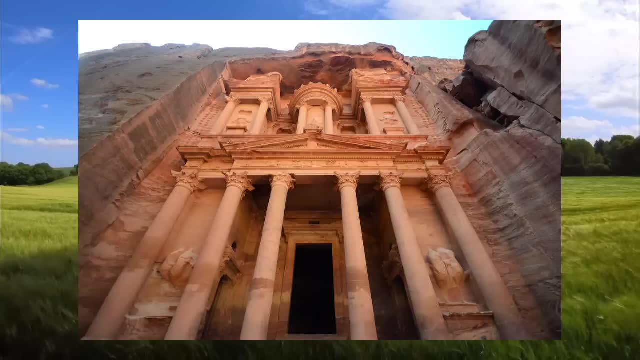 notably the incense route, facilitating the exchange of valuable goods between southern Arabia and the Mediterranean. Skilled merchants, they played a crucial role in the transportation of spices, incense and myrrh. One of the most notable aspects of Nabatean engineering was their. advanced water management systems, essential for sustaining life in the semi-arid arid region. Petra's survival hinged on dams, cisterns and underground channels that effectively captured and stored water. The Nabateans developed a distinctive culture with influences from Arabian, Hellenistic and local traditions. Their religious practices. 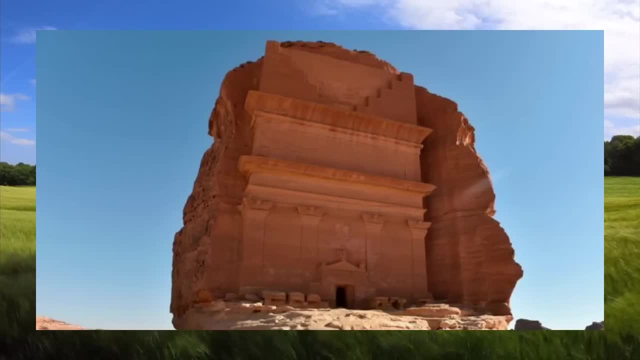 involved a pathion of deities, and inscriptions in an evolving Arabic script prove insights into their linguistic and religious heritage. In the early 2nd century CE, the Nabatean kingdom was annexed by the Roman Empire, leading to the fall of the Roman Empire. The Nabateans' 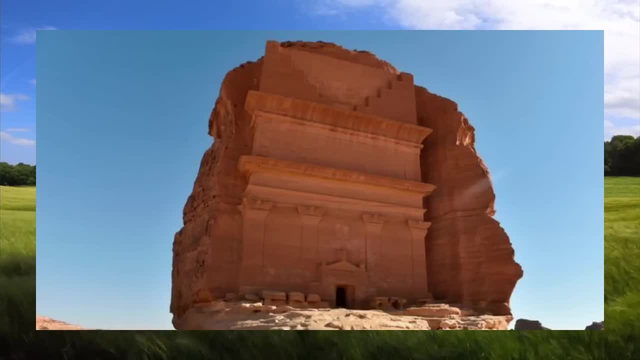 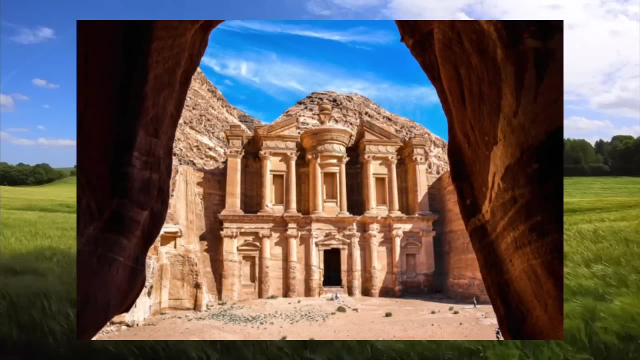 influence in the region. the decline of Petra and the Nabatean culture ensued, influenced by shifts in trade routes, economic dynamics and the waning importance of the incense trade. Petra was eventually abandoned and the city's rediscovery in the 19th century fueled architectural interest. 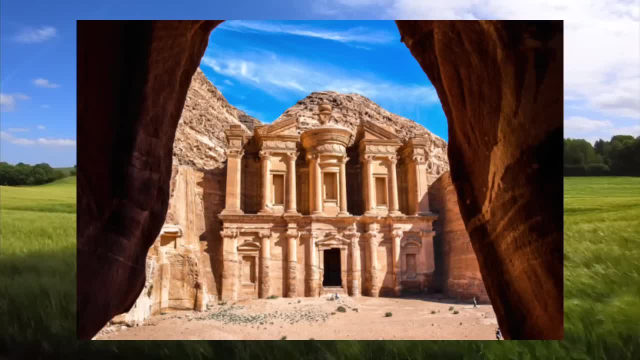 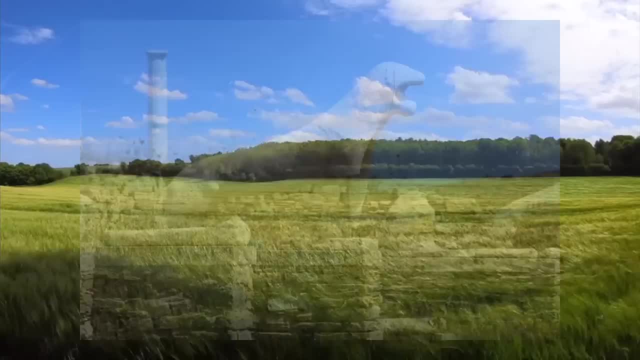 The legacy of Nabateans endures through the architectural marvels of Petra. Cycladic Culture- The Cycladic culture flourishing in the Aegean Islands during the early Bronze Age. The Cycladic culture flourishing in the Aegean Islands during the early Bronze Age is characterized. 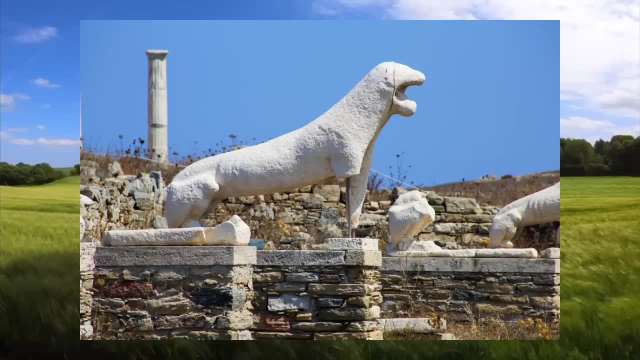 by its unique artistic expression and the maritime society Spread across islands like Delos, Mykonos and Santorini, the Cycladic people engage in seafaring, fishing and trade, connecting them with their neighboring cultures. Notably, their distinctive art is exemplified by: 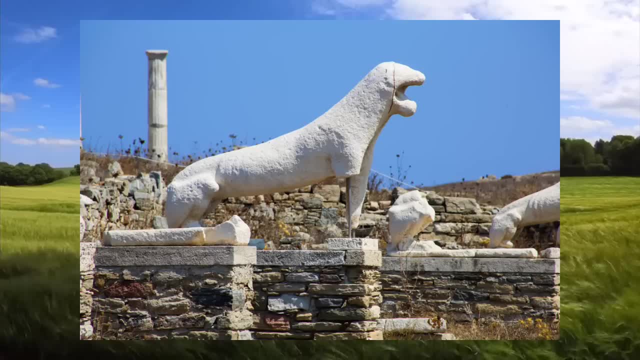 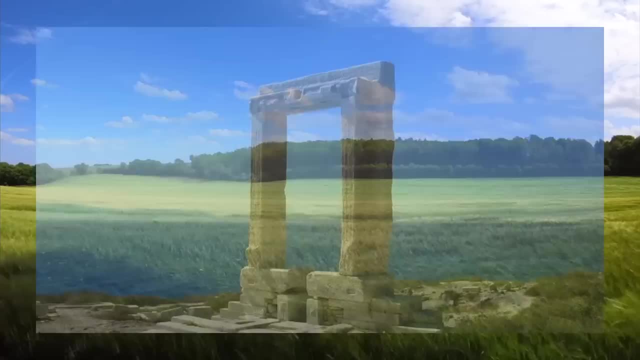 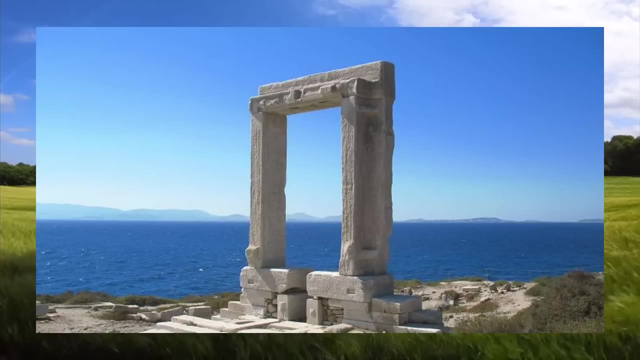 marbles figurines depicting abstracted and nude human forms. These figurines, often found in burials, suggest a ritual significance, providing a glimpse into the spiritual beliefs of the Cycladic people. Burial practices were integral to understanding their culture, with graves containing offerings. 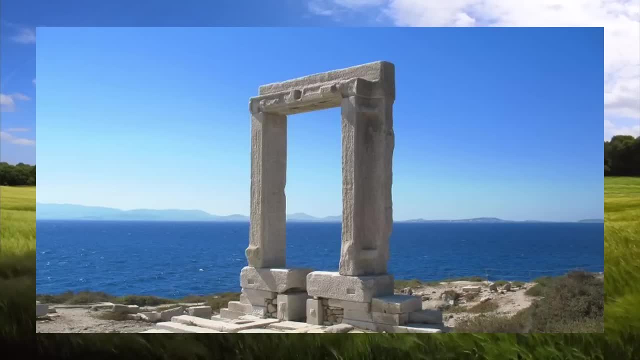 and sometimes featuring cis graves or tombs. The Cycladic people maintained interactions with contemporaneous civilizations, including the Minoans or Crete, and mainland Greek cultures, influencing artistic styles and material culture. Active participation in trade networks facilitated the exchange of goods like obsidian metals and marble, contributing to the cultural vibrancy of. 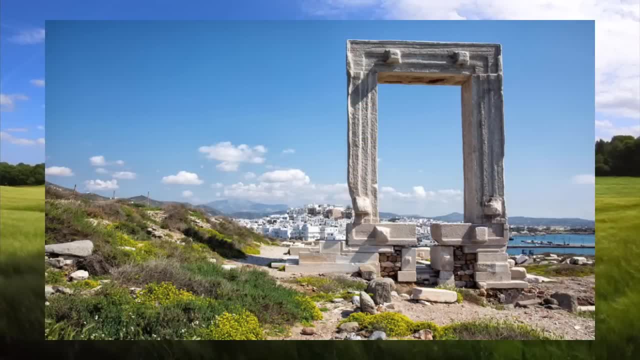 the Cyclads. The decline of the Cycladic culture led to the decline of the Cycladic culture. The decline of the Cycladic culture led to the decline of the Cycladic culture. The decline of the Cycladic culture led to the decline of the Cycladic culture. The decline of the Cycladic culture occurring around. 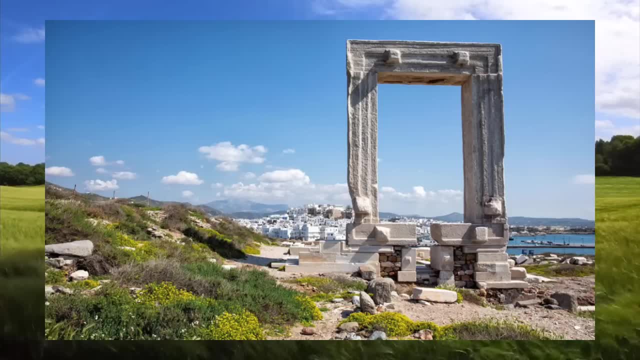 the transition to the Middle Bronze Age remains shrouded in some mystery. Factors such as environmental changes, resource depletion or external influences may have played a role. Notably, the eruption of Thera had broader implications for the Aegean region, Though its specific impact on the Cycladic culture is a subject of debate. 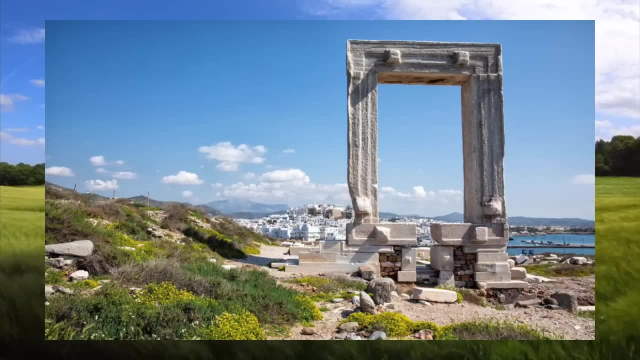 archaeological excavations on various Cycladic islands have unearthed a wealth of artifacts, including the iconic marble figurines, pottery and tools. These findings contribute significantly to our understanding of Cycladic daily life, their burial practices and the interconnectedness of ancient Aegean cultures. 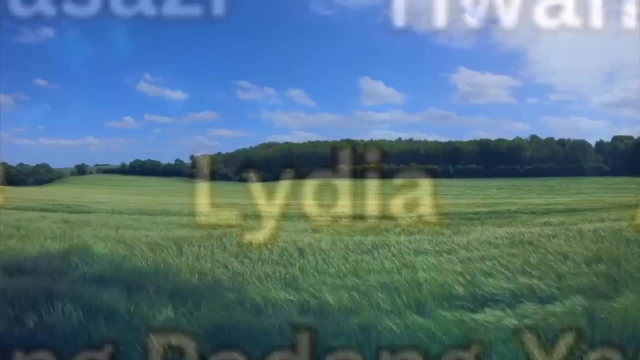 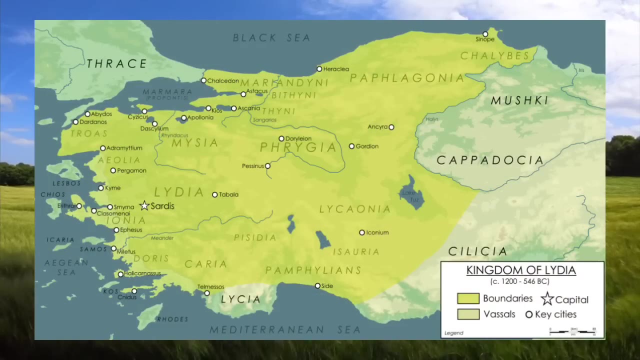 Lydia. Lydia, an ancient kingdom in western Asia Minor, occupied a strategic region along the Aegean Sea in what is now western Turkey. Its capital, Sardis, situated on the western Hermes River, became a thriving cultural and economic center, with legendary wealth associated with the. 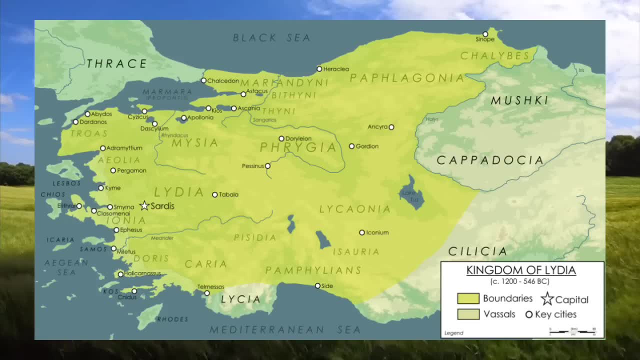 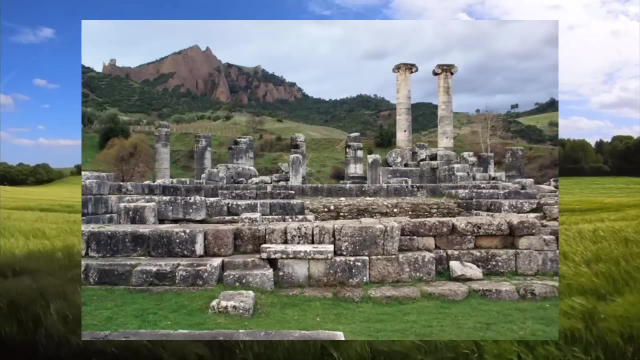 Picatulis River Renowned for its adoption of coinage. Lydia played a pivotal role in shaping early monetary systems and how money came into use in early civilizations, Using the natural alloy eclodium for minting coins. the Lydians had cultural ties with both Greek and Anatolian. 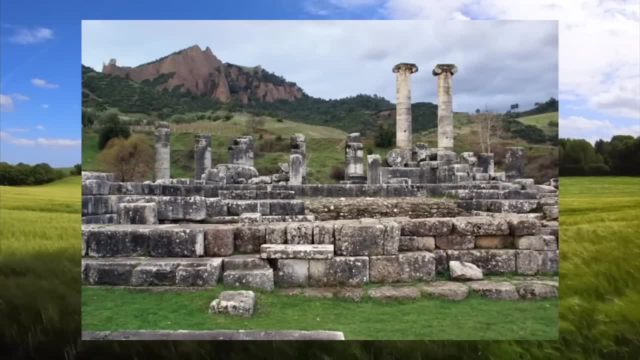 civilizations, blending influences to enrich their own cultural heritage, The Lydian kingdom gained historical prominence, which led to the formation of the Aegean Kingdom. The Aegean Kingdom was the capital of the Aegean Kingdom, with legendary figures like King Gyades and notably King 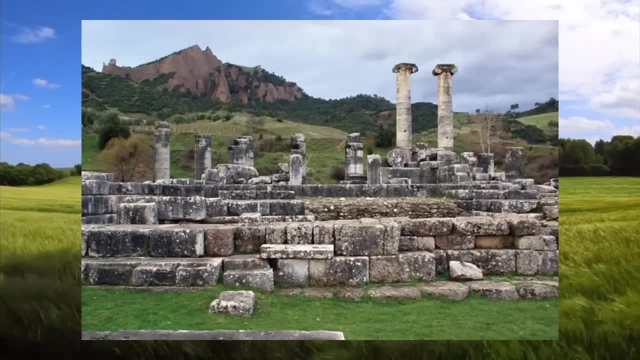 Crossinus, famed for its wealth. However, the wealth and power of Lydia faced a turning point in the mid-6th century BCE when it was conquered by Cyrus the Great, marking Lydia's incorporation into the Persian Empire. Herodotus, the ancient Greek historian, provided valuable insights into 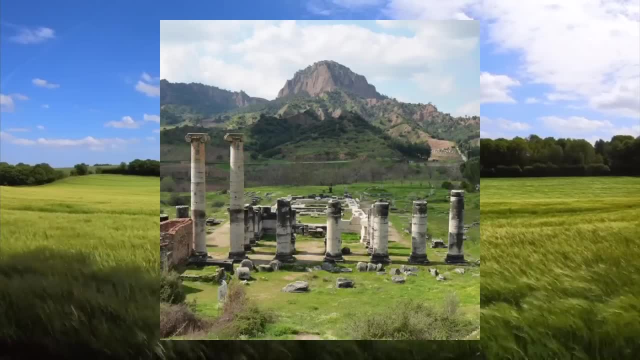 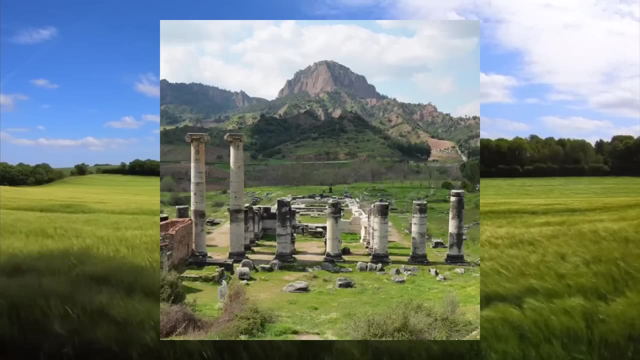 Lydia's history, customs and their notable events. Despite Lydia's absorption into larger empires, including the Persian and later the Hellenistic realms, its legacy endured. The Lydians' contribution to the introduction of coinage had a lasting impact on trade and economic systems. Architectural excavations at Sardis have unearthed artifacts. 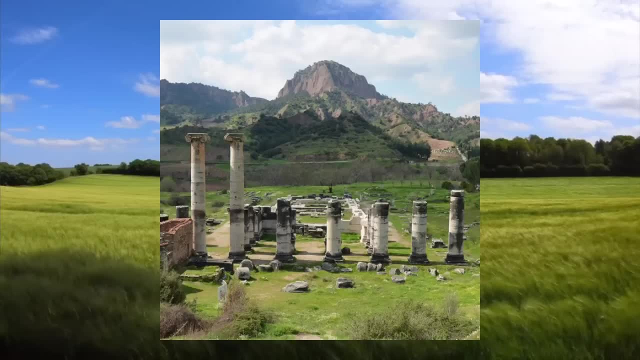 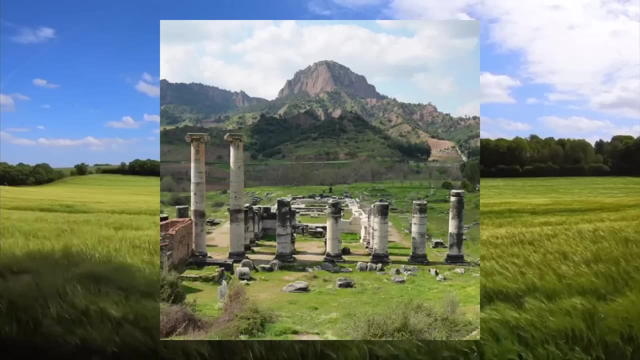 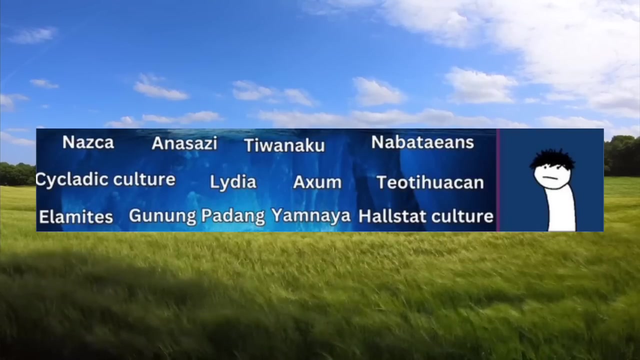 including the Temple of Artemis, offering glimpses into Lydia's architectural achievements and daily life. Lydia, with its blend of wealth, cultural exchange and historical transitions, remains a significant chapter in the rich tapestry of ancient Anatolian civilizations. Aksum, Aksum, an ancient kingdom. located in the Horn of Africa, specifically in present-day Ethiopia, and held a strategic position along the Red Sea that facilitated extensive trade and cultural exchanges. The capital city of Aksum, a thriving center for commerce, politics and religion, was adorned with monumental obelisks, including the famous Obelisk of Aksum. 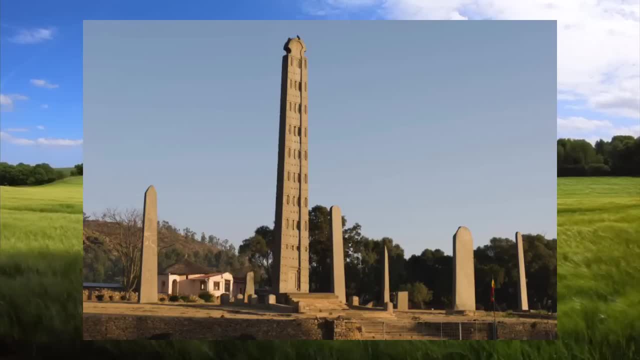 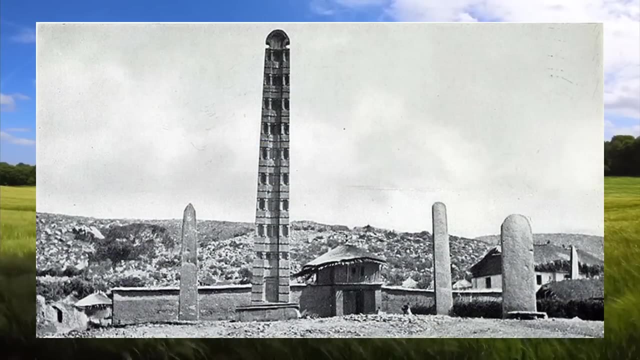 which has become an emblematic symbol of the kingdom. Prospering from its participation in trade routes connecting Africa, the Arabian Peninsula and the Mediterranean, Aksum's wealth was fueled by the exchange of valuable goods such as ivory, gold, spices and exotic animals. 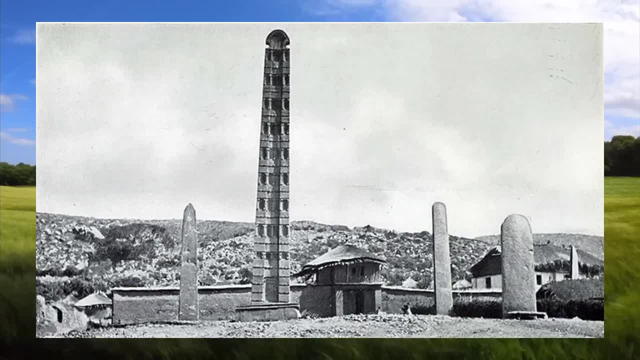 One of Aksum's most significant historical contributions is its early adoption of Christianity, with King Ezna converting to Christianity in the 4th century CE. The Church of St Mary of Zion in Aksum is believed to house the Ark of the Covenant. 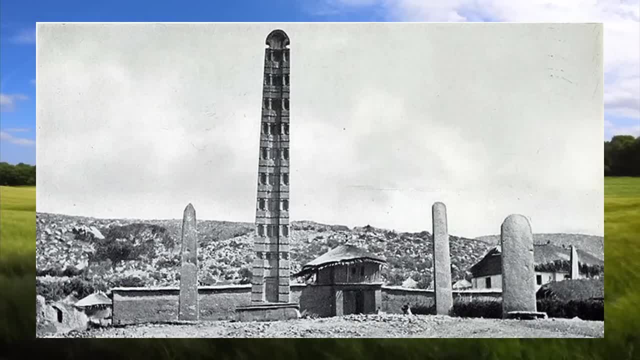 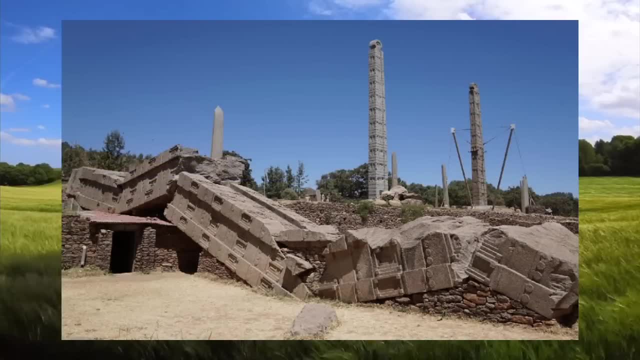 Adding to the kingdom's religious importance. Aksum's towering obelisk, crafted as a funerary monument, or markers of significance, reflect the kingdom's cultural and architectural achievements. The decline of Aksum's influence began in the 7th century, attributed to factors 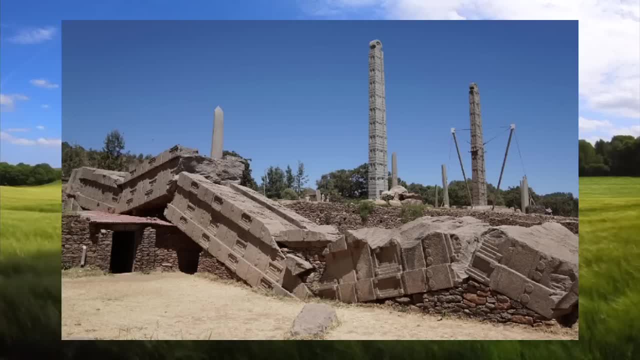 such as the rise of Islam and shifts in trade routes. Despite this decline, Aksum's historical significance endures and the kingdom is associated with the biblical Queen of Sheba and the Solomonic dynasty. Aksum's archaeological sites, including the obelisks, royal tombs- 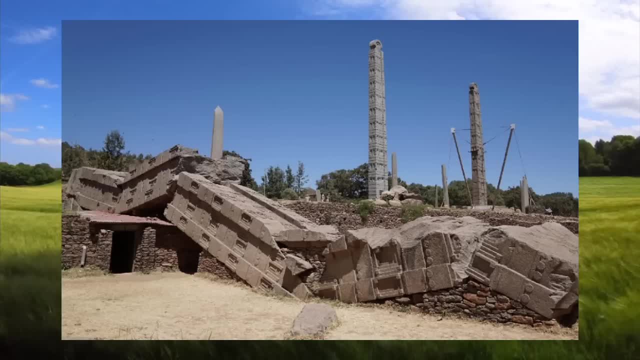 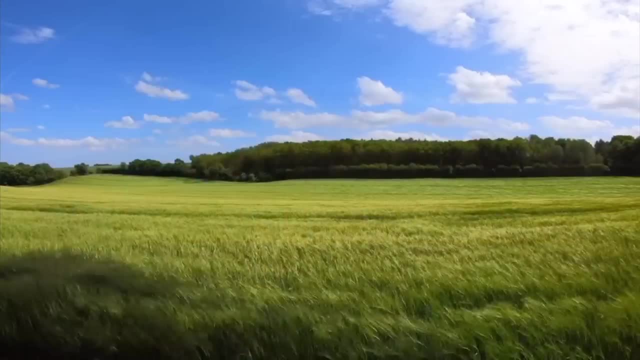 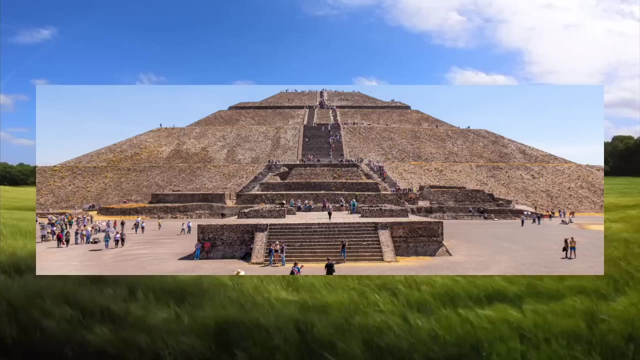 and ancient structures provide a tangible link to the kingdom's rich history. Teotihuacan. Teotihuacan, situated in the Basin of Mexico, emerges as one of the most significant archaeological sites from ancient Mesoamerica. Its well-preserved urban layout features a 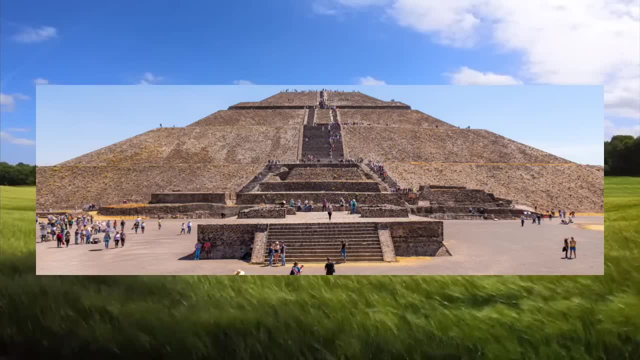 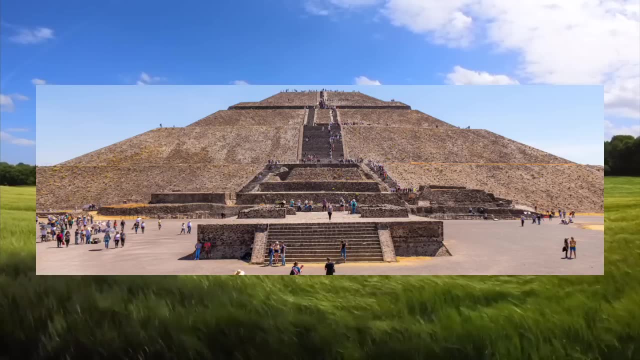 distinctive grid plan, with the iconic Avenue of the Dead serving as the central ceremonial axis. Dominating the landscape are the massive Pyramid of the Sun and the Pyramid of the Moon, both integral to the city's religious and ceremonial functions. Teotihuacan's allure extends beyond its 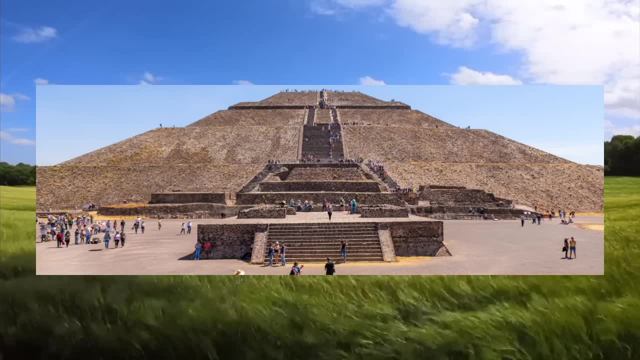 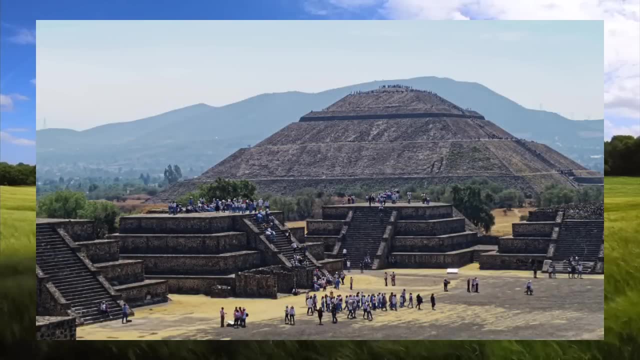 grandeur, encompassing a multicultural population and a blend of residential and ceremonial spaces. The multicultural nature of Teotihuacan is evidenced by its diverse population, incorporating various Mesoamerican groups. The residential areas, characterized by apartment-like compounds adorned with vibrant murals, provide glimpses into the daily life. 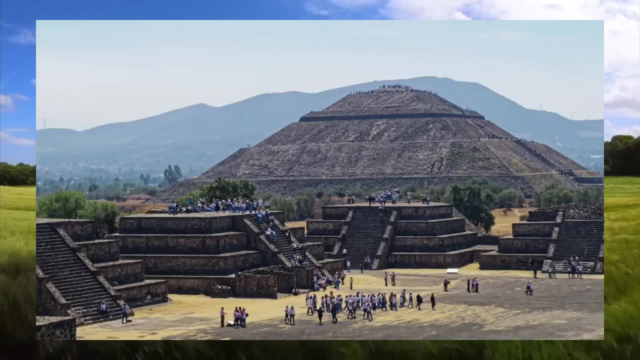 and the religious beliefs. Notable among these murals are those found in the Feathered Serpent Pyramid, depicting deities and mythological narratives with remarkable artistic skill. Despite its grandeur, the decline of the Teotihuacan remains shrouded in mystery. 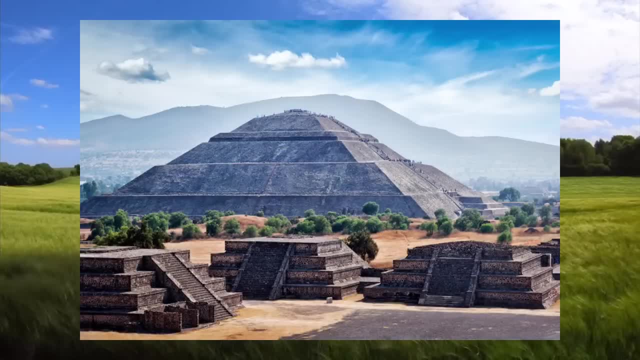 with theories ranging from social unrest to environmental changes. Abandonment around the 7th or 8th century CE. in the city's enigmatic legacy endured through its profound influence on subsequent Mesoamerican cultures, notably the Aztecs. Teotihuacan's imagery and symbolism. 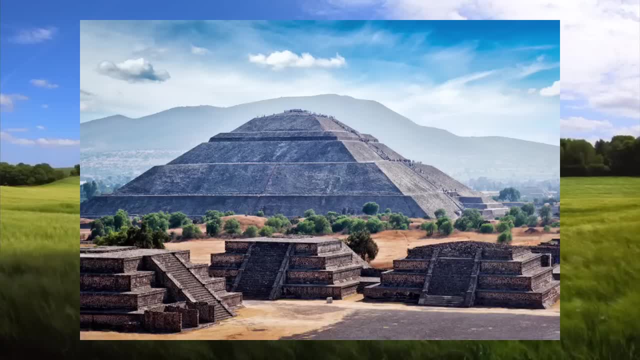 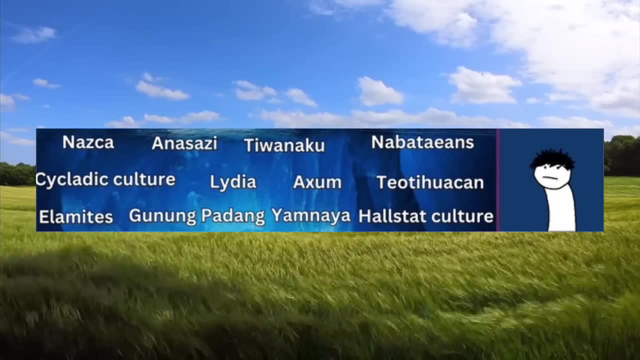 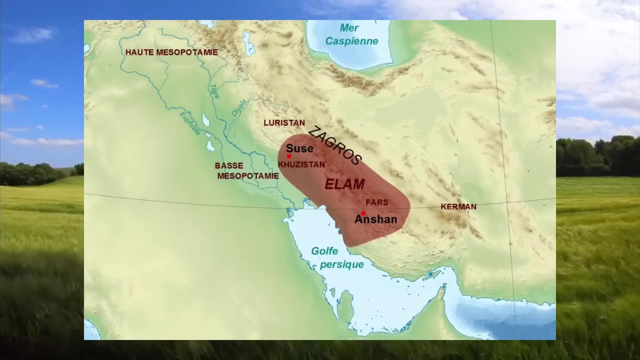 found resonance in Aztec religious beliefs, affirming its enduring cultural impact and how much it influenced Aztec culture. Elamites- The Elamites, inhabitants of the ancient region of Elam in what is now southwestern Iran, formed a distinctive civilization that emerged around the 3rd millennium BCE. 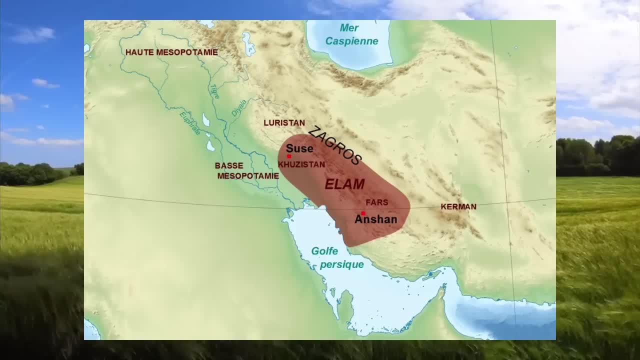 Geographically situated between the Tigris and Karan rivers, Elam held strategic importance due to its proximity to Mesopotamia. Unlike centralized states, Elam comprised a collection of city-states with evolving political structures, Experiencing periods of both independence and subjunction to foreign rule. the Elamite civilization is associated. 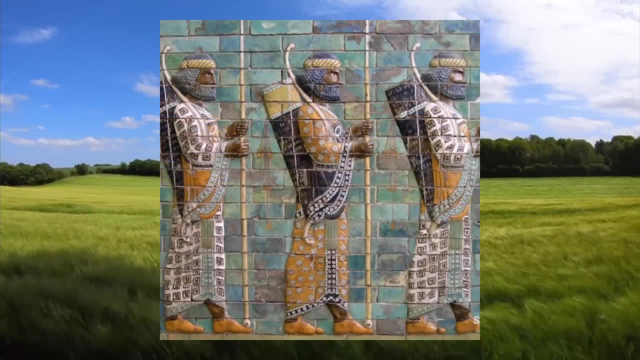 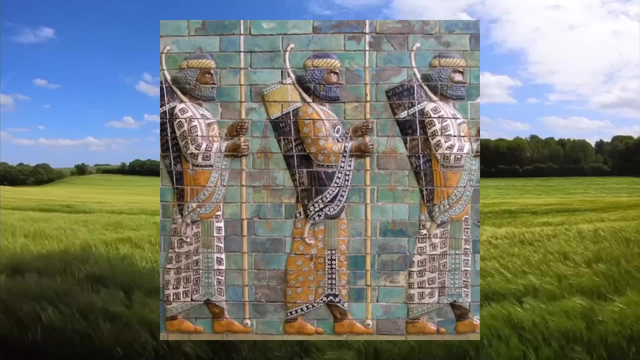 with the Elamite language, which remains largely undeciphered in the use of scripts such as linear Elamite and later the cuneiform writing system adopted from Mesopotamia. Throughout its history, Elam had complex relations with neighboring Mesopotamian civilizations engaging in trade. 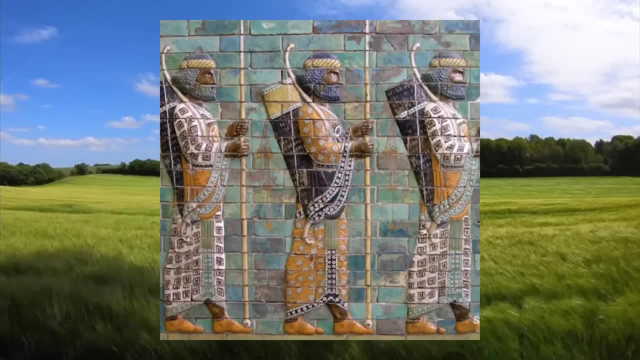 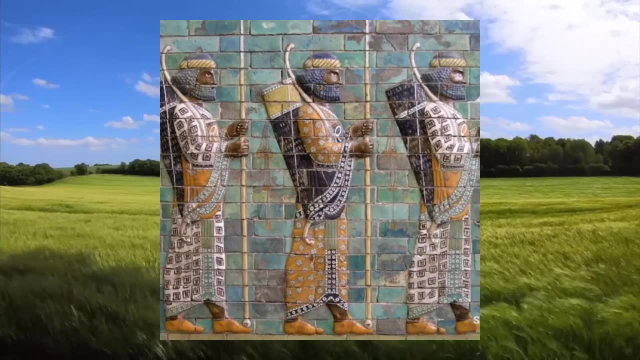 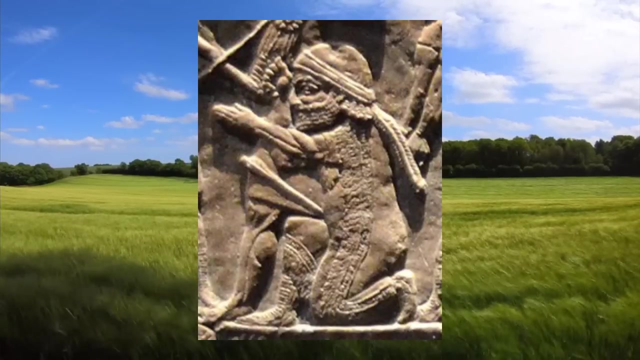 and conflicts with Sumer and Akkad. Elamite art and architecture bear a distinctive style, exemplified by structures like the Ziggurat at Kohar and Zannibal. This archaeological site provides valuable insights into Elamite religious practices and the urban planning that went along with it. 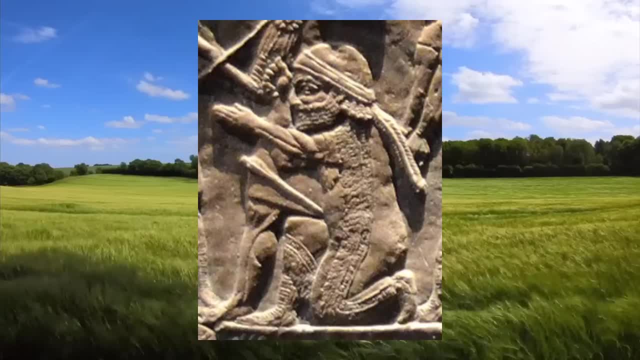 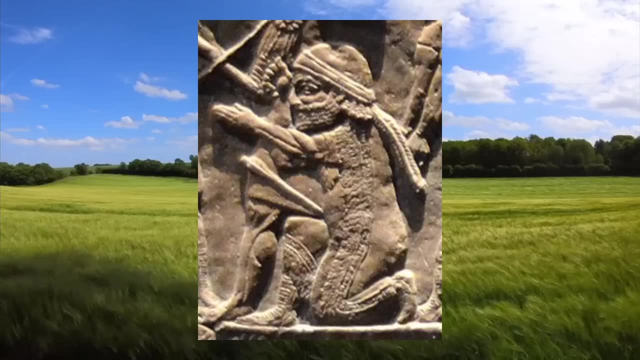 The Elamites were known for their military prowess, launching successful campaigns and, at times, invading Mesopotamia. The Ziran conquest of Elam in the 7th century BCE marked the end of Elamite political independence. However, elements of Elamite culture endured, influencing the 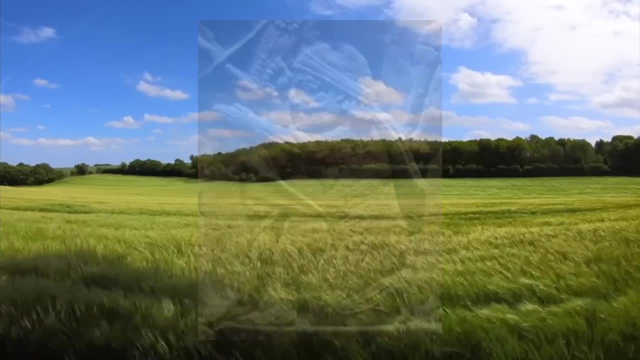 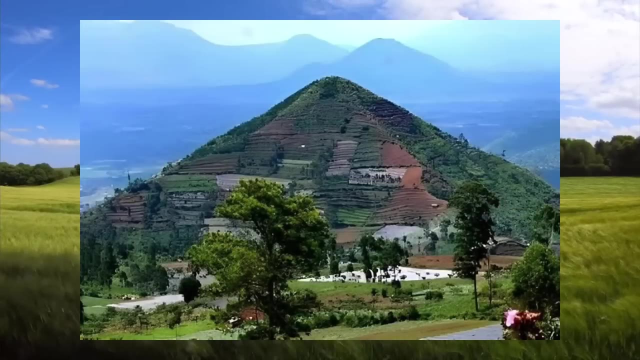 broader cultural landscape of the ancient Near East. GANANG, PADANG, Ganang Padang, located in West Java, Indonesia, has become a site of fascination and speculation due to its unique geological features and the possibility that it may be an ancient man-made structure. Positioned on a volcanic mountain, the site exhibits a stepped pyramid-like 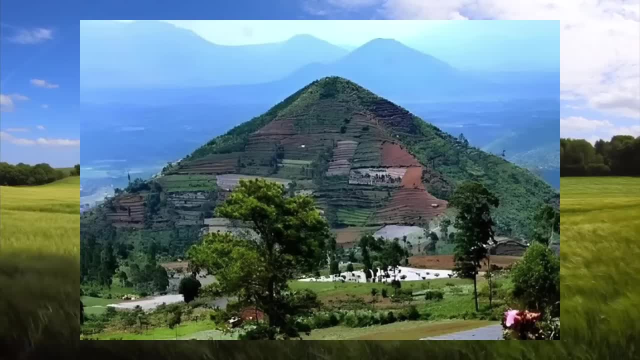 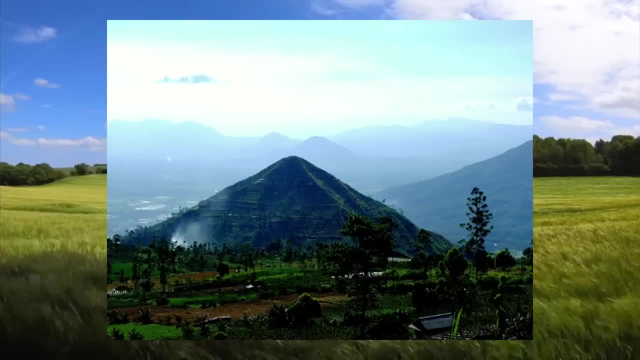 formation, prompting discussions about its potential as one of the world's oldest man-made structures. The controversy surrounding Ganang Padang revolves around its age, with claims suggesting it could date all the way back to the 9th century BCE. However, it is not known for its 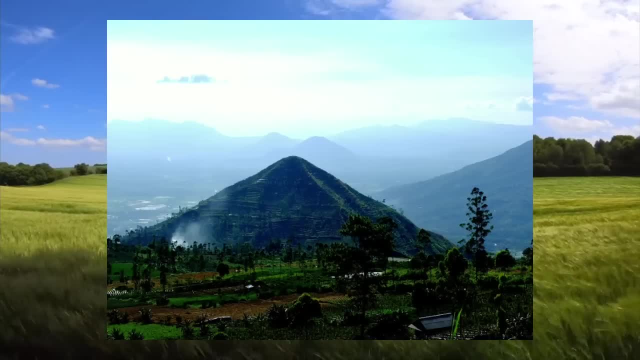 age. The site is believed to date back thousands of years, making it a candidate for one of the earliest known human constructions. The megalith structures at Ganang, Padang consist of terraces, stone columns and basalt slabs, contributing to the speculation that it might be a man-made. 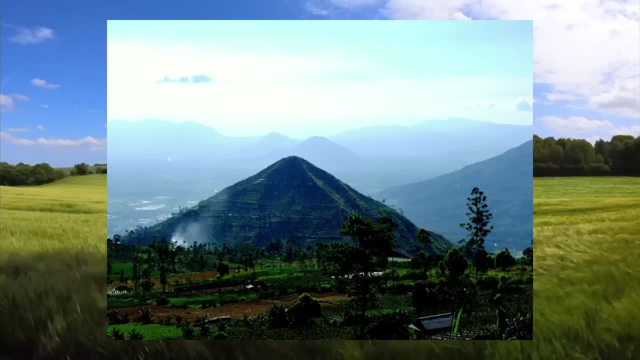 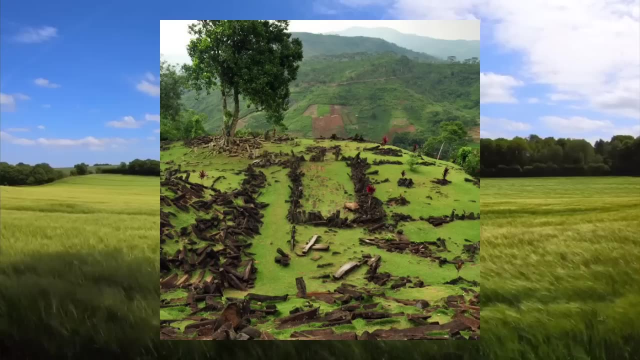 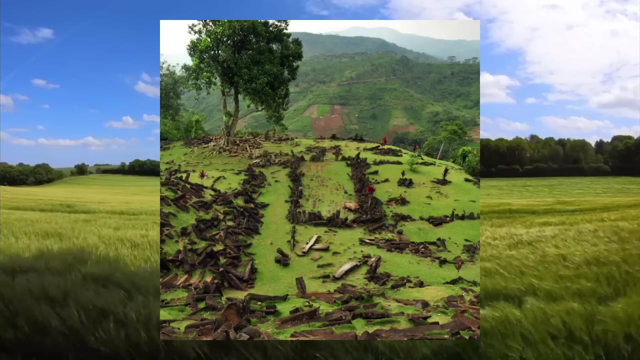 pyramid. Archaeological excavations have been conducted to unravel the site's history and the significance along with it, and ongoing research is attempting to establish its age and the cultural context. Despite these efforts, the mainstream archaeological community remains cautious about it and claims of Ganang Padang being an ancient pyramid or 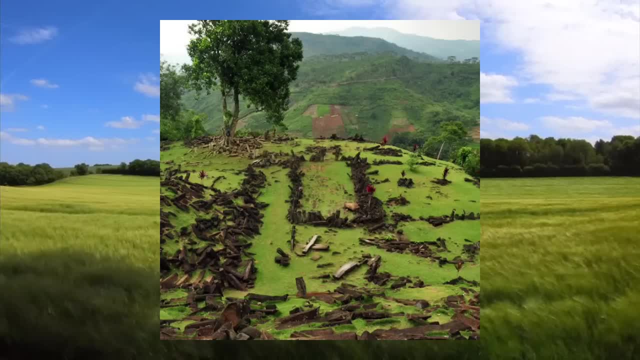 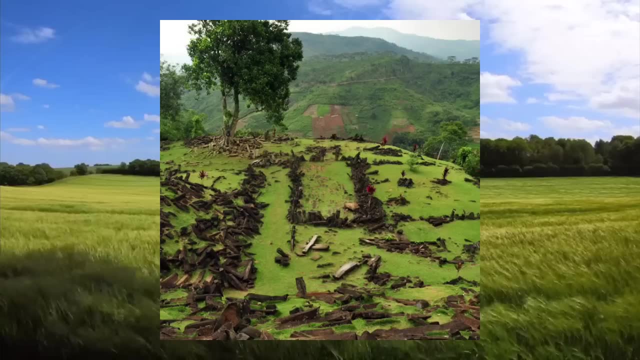 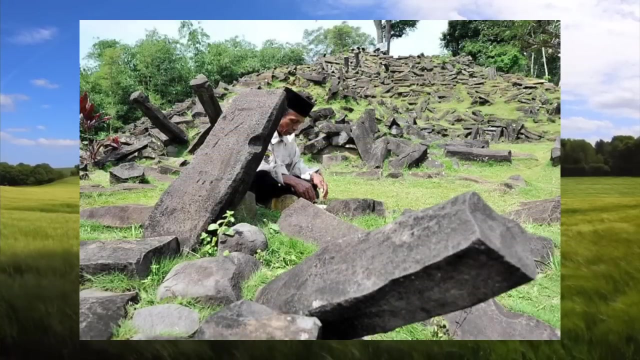 remnant of an advanced prehistoric civilization are highly controversial. The Indonesian government has supported research at Ganang, Padang, involving institutions like the National Research Center for Archaeology. Additionally, this site holds cultural and spiritual importance for the local Sudanese people, leading to rituals and ceremonies. 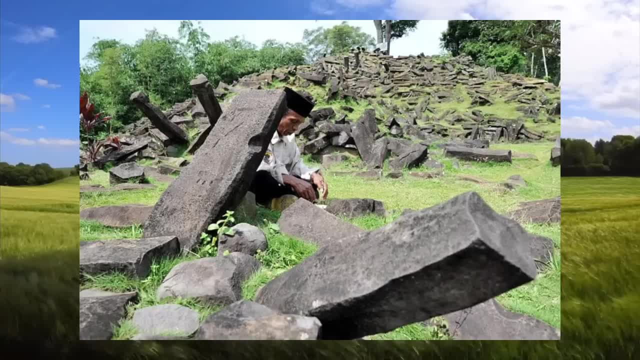 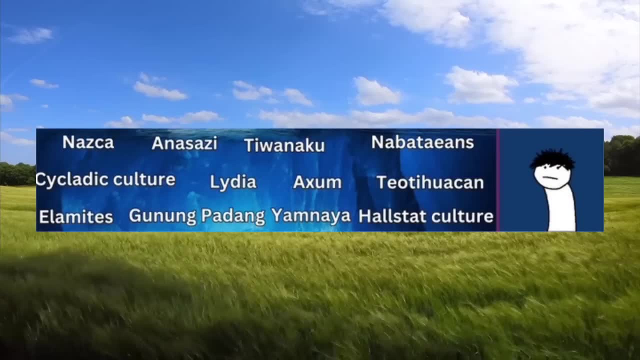 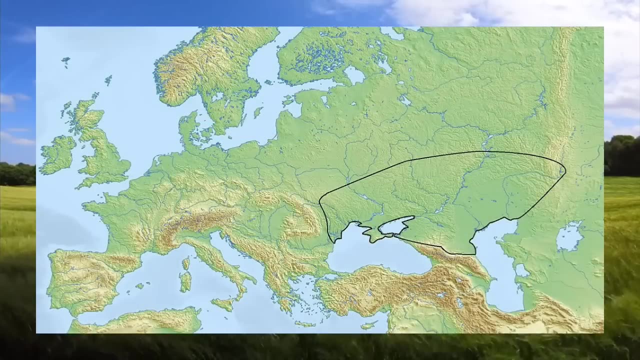 being conducted at the location. Ganang Padang stands as a complex archaeological puzzle, With its true nature and historical significance yet to be definitively determined. Yamnaya, The Yamnaya culture flourishing on the Panacaspian steppe during the Late Copper Age and 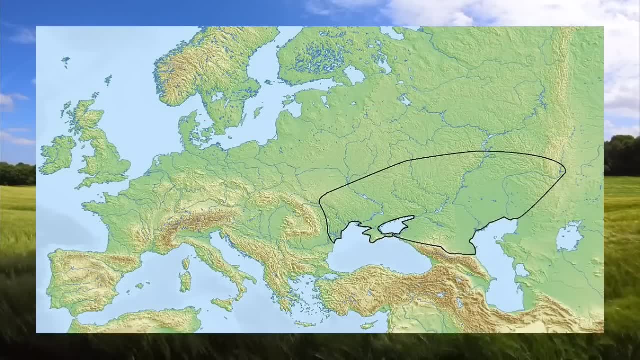 Early Bronze Age, which was around 3300 BCE to 2600 BCE, just for reference of the Copper Age and the Early Bronze Age was characterized by its nomadic, pastoralist lifestyle. The expansive grasslands of the Yamnaya culture were a ideal environment for the Yamnaya people, who relied on herding cattle. 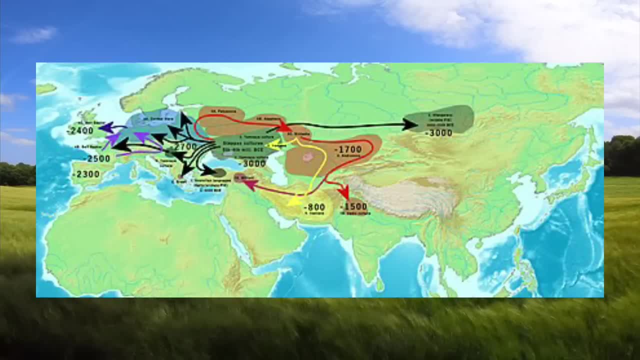 sheep and horses for subsidence. One of the most distinctive features of the Yamnaya culture was the use of kurgans, or burial mounds, which contained a variety of grave goods, such as pottery, weapons, tools and ornaments that went inside of these graves. These kurgans not only served as burial. 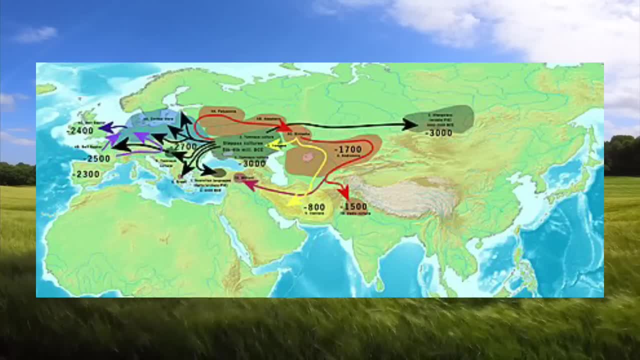 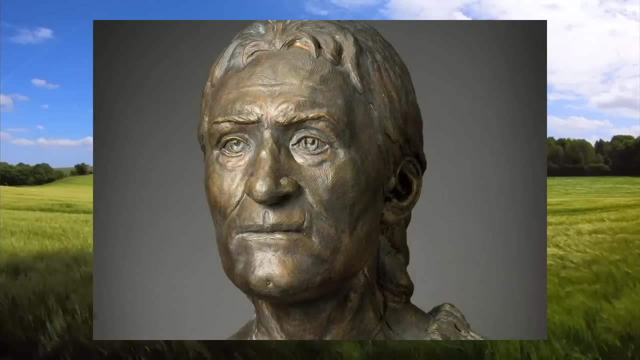 sites, but also played a role in shaping the landscape of the steppe. The Yamnaya culture is of Indo-European languages. Scholars posist that the Yamnaya people played a pivotal role in the diffusion of Indo-European linguistic and cultural elements across vast regions. This cultural 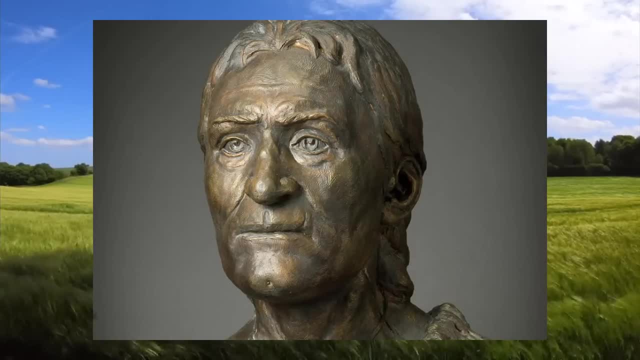 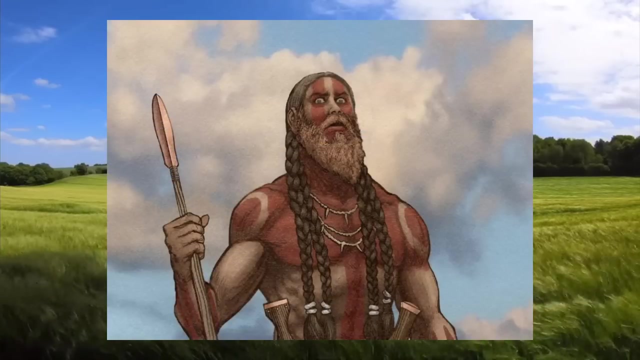 exchange is reflected in the archaeological record, where specific types of ceramics, metal artifacts and burial practices associated with the Yamnaya culture has been identified. Genetic studies, particularly analysis of ancient DNA, have provided valuable insights into the genetic legacy of the Yamnaya people. The Yamnaya culture has been identified by the Yamnaya culture. The Yamnaya culture. 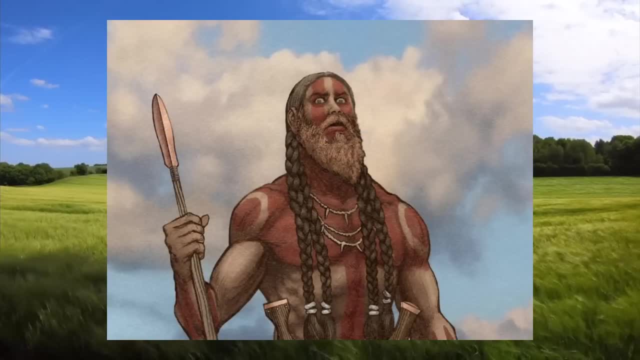 has been identified by the Yamnaya culture. The Yamnaya culture has been identified by the Yamnaya people. The Yamnaya culture has been identified by the Yamnaya people. Their influence can be traced into a genetic makeup of present-day populations, particularly in parts of Europe and South Asia. 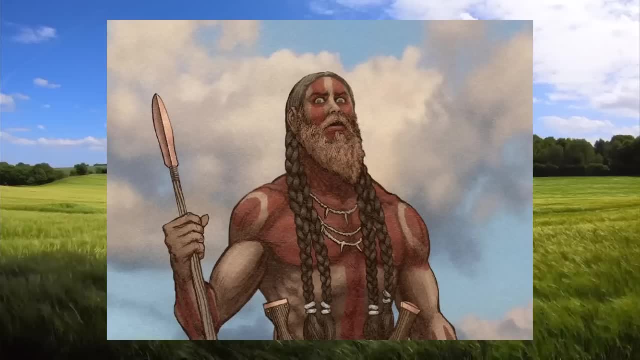 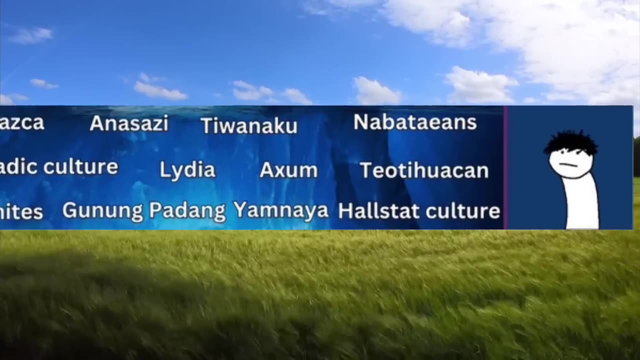 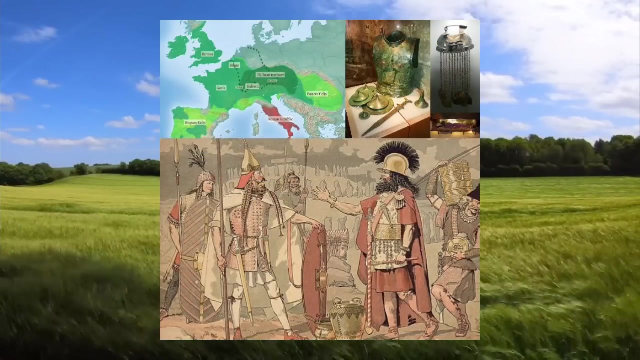 The Yamnaya culture, with its nomadic lifestyle and cultural exchanges, contribute to the intricate tapestry of prehistoric Eurasia. Hallstatt Culture- The Hallstatt culture, named after the site in Austria where its archaeological remains were first discovered, represents a significant phase in the European Iron Age Originating in the 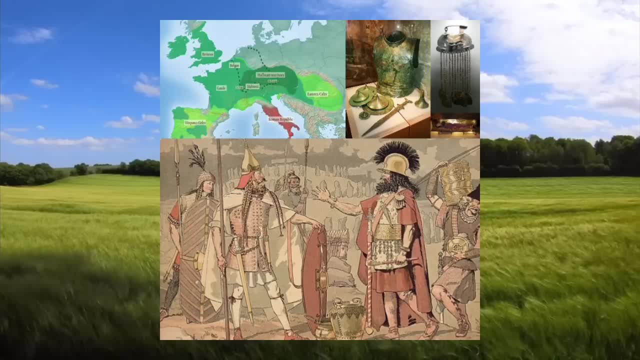 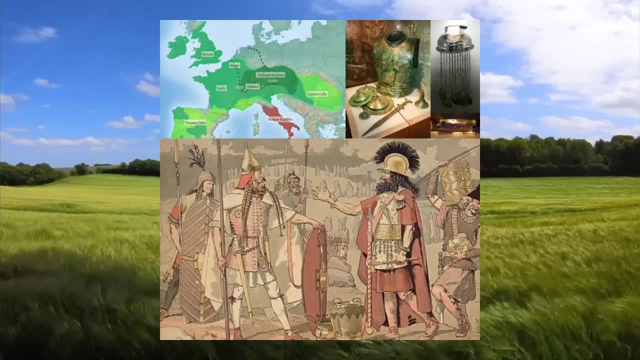 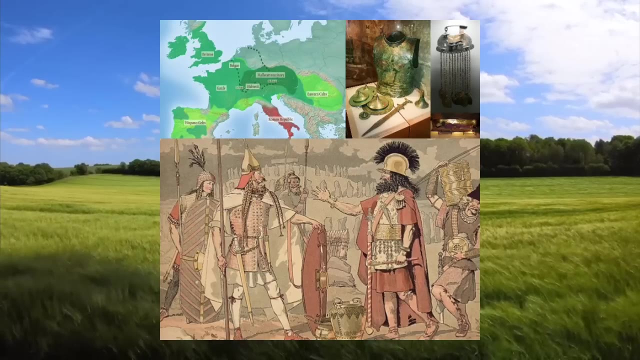 Hallstatt-Dachstein area and region, the culture's influence expanded across Central and Western Europe. The Hallstatt people were known for their diverse economic activities, including salt mining, metalworking, agriculture and trade. Salt mining in particular played a crucial role. 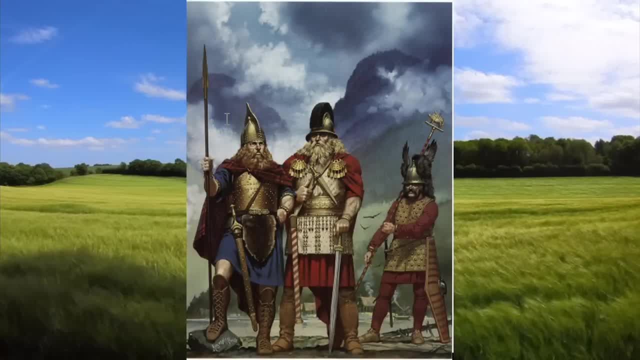 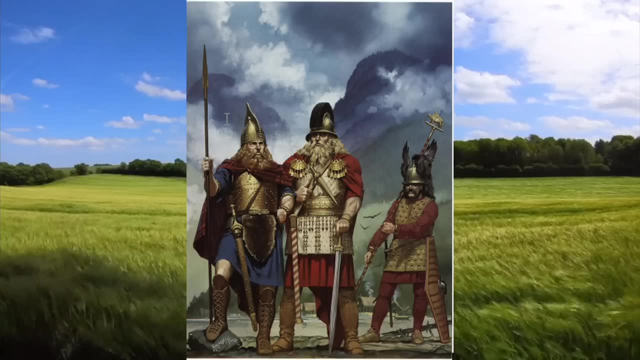 in their prosperity and the term Hallstatt is just associated with prehistoric salt mining sites. so basically, these people and the culture is just named after salt mining. The material culture of the Hallstatt people is characterized by skillfully crafted metalwork, including weapons. 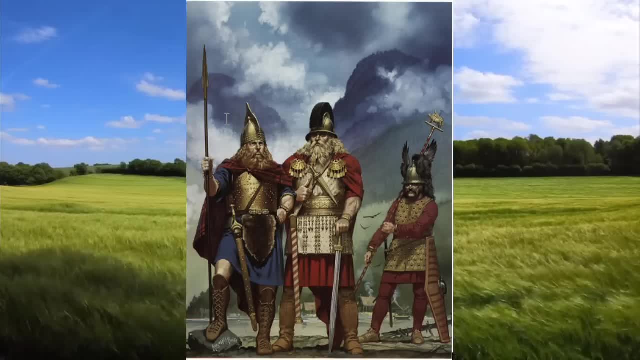 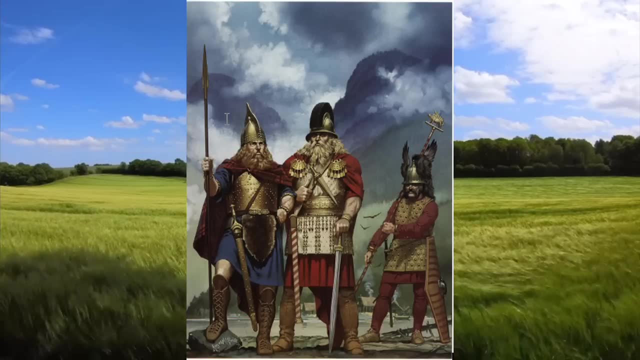 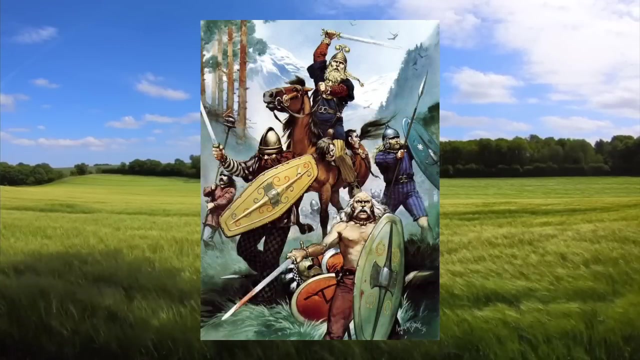 tools and ornaments. Proficiency in bronze and iron metallurgy distinguished the Hallstatt culture, and their artifacts served both functional and decorative purposes. Burial practices featured the use of tumuli, with elite individuals interned in richly furnished graves. These burials 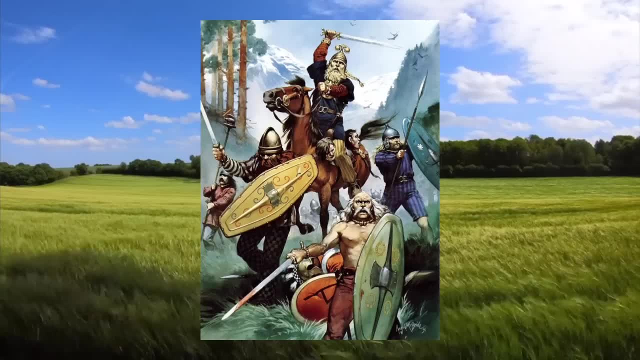 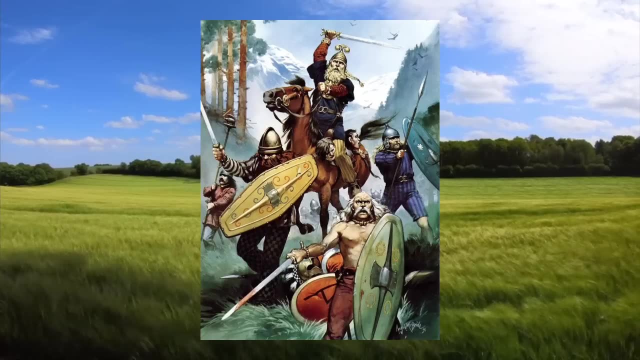 provided valuable insights into social stratification and the cultural significance attributed to specific individuals. The Hallstatt culture is characterized by skillful crafted metalwork with unique materials. within the society, Trade and cultural contacts were integral to the Hallstatt culture, evident in the distribution of artifacts and materials across the regions. 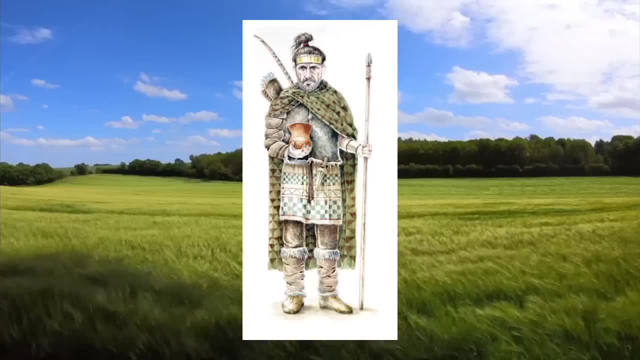 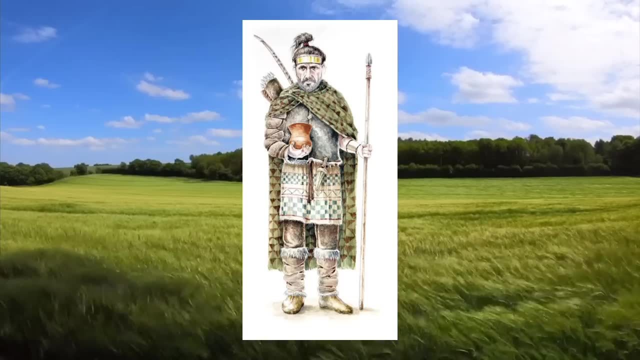 Alright, now onto tier 4, starting off with the Bell-Beaker culture. The Bell-Beaker culture, emerging in the third millennium BCE, stands as a distinctive archaeological phenomenon that left an indelible mark on the prehistoric landscape of Europe, Originated in the 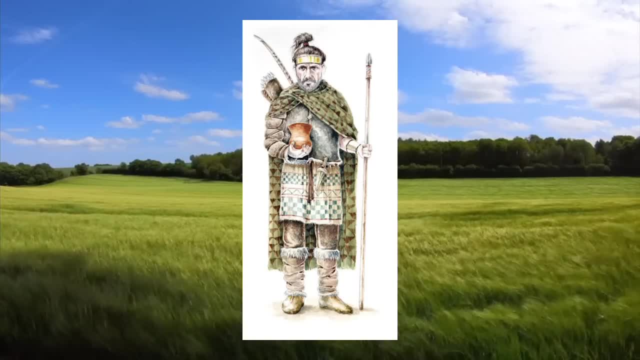 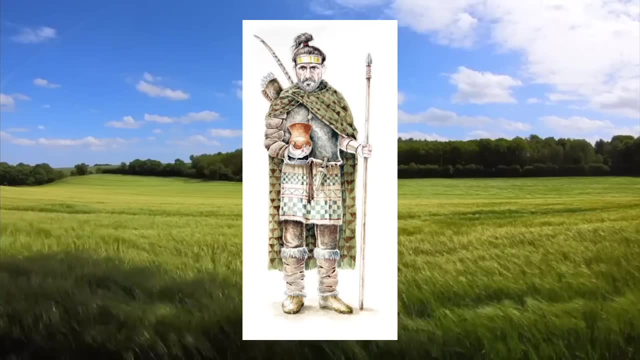 In the Iberian Peninsula around 2800 BCE. the culture's influence gradually expanded across Western and Central Europe, reaching as far as the British Isles and the Carpathian Basin. The culture derives its name from the iconic bell-shaped pottery characterized by flattered 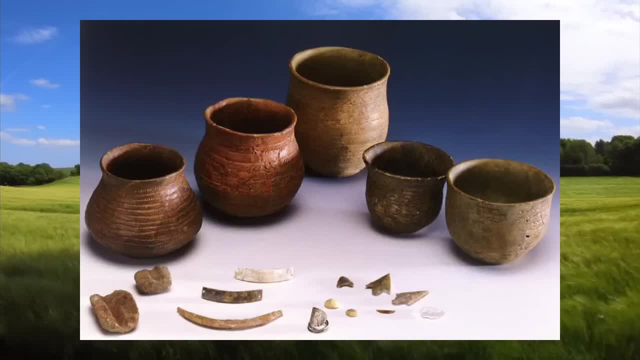 lips and often adorned with decorative patterns, particularly the distinctive beakers used for various purposes, including communal drinking Material. culture associated with the bell-beaker people extends beyond pottery, encompassing a range of artifacts that signify technological advancements. Notably, the use of copper and bronze marked a crucial transition reflecting the adoption 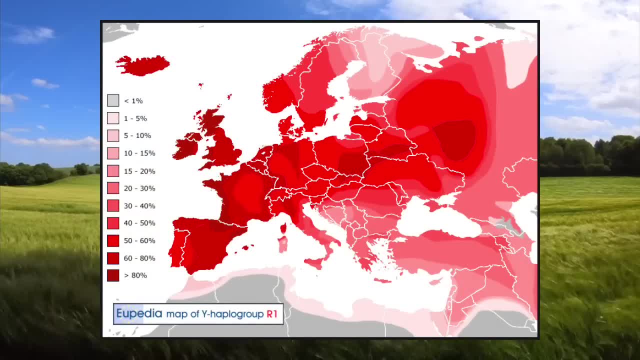 of metal tools and weaponry. Burial practices within the bell-beaker culture were diverse, with individuals interned in varying positions and accompanied by grave goods such as the characteristic beakers, Archery equipment, copper objects and, occasionally, remains of domesticated animals. 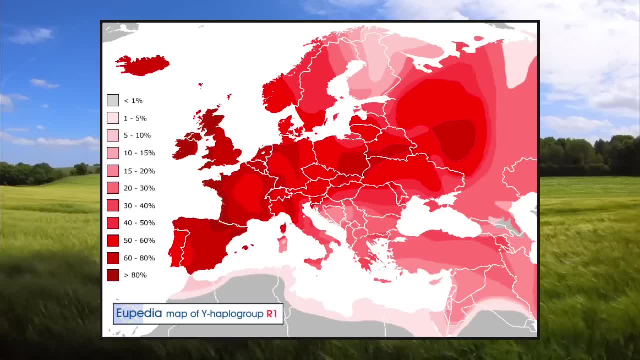 The spread of the bell-beaker culture has sparked scholarly debate, with theories ranging from migration patterns to cultural diffusion. The three identified phases, which are the early, late and final bell-beaker, chronicle the evolution and persistence of this cultural complex. 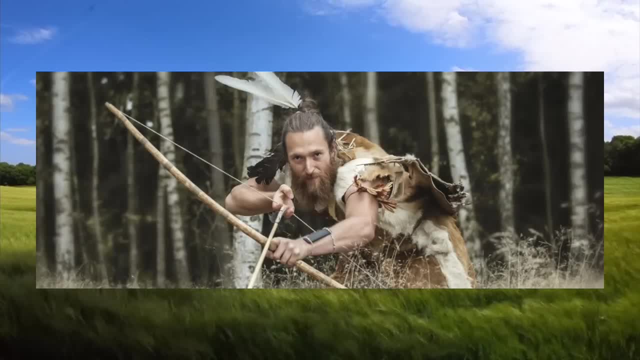 As it developed, the bell-beaker culture co-existed with the corded ware culture and played a role in the transitional period from the Noolithic to the Bronze Age. By approximately 1800 BCE, the bell-beaker culture had been used as a means of transportation. 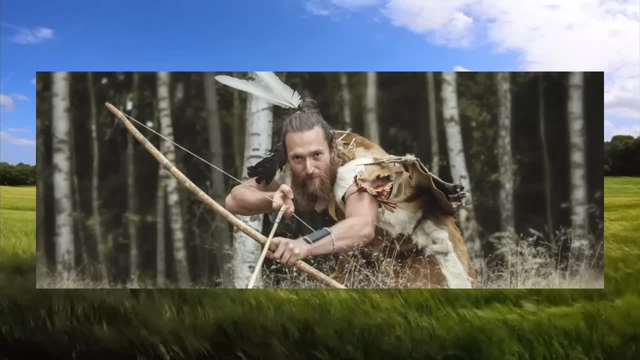 to other cultures, The bell-beaker culture began to wane and slowly disappear, leaving behind a legacy that influenced subsequent cultural developments in Europe. The reasons for its decline remain a subject of investigation, with factors such as climate shifts, socio-economic changes and interactions with neighboring cultures being considered. 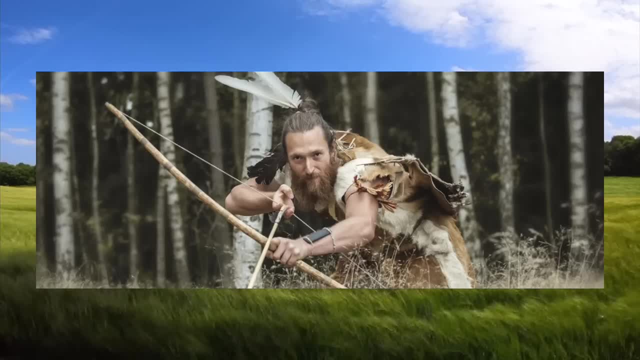 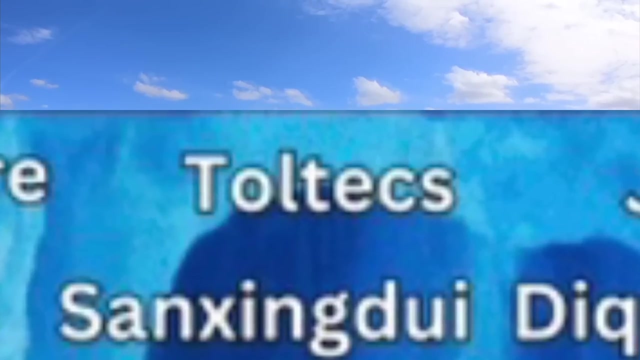 Despite its eventual decline, the bell-beaker culture remains a pivotal phase in European prehistory, making a dynamic period of technological innovation, cultural exchange and the shaping of early European societies: The Tolltecs. The Tolltecs, a prominent pre-Columbian civilization, emerged in central Mexico during the early 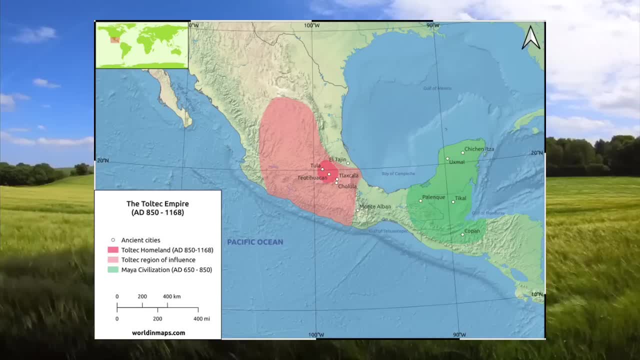 post-classic period around 900-1100 CE, associated with the legendary figure Quetzala, a feathered serpent deity. The Tolltecs considered him a cultural hero and, in some accounts, an exiled ruler. Their capital city, Tula, situated near present-day Tula de Alden, is known as the capital city. 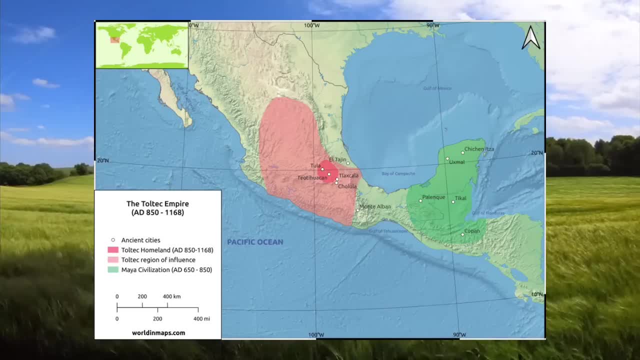 of the Tula region. There is a tradition that the Tolltecs were called the Tolltecs on their way to the capital city of the US because of their service to the state of the United States. then, in Mexico, stood as a testament to their architectural prowess, Featuring notable 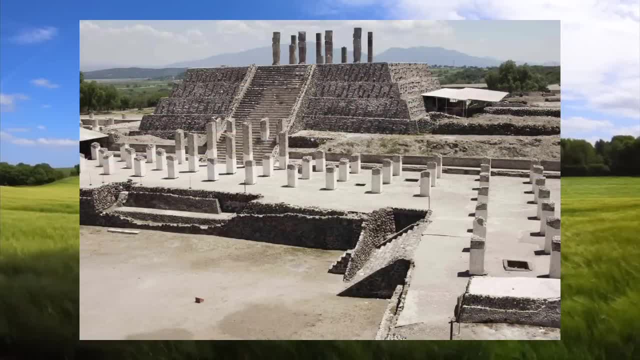 structures like the Pyramid of Quetzala renowned for military strength and expansive political influence. the Toltecs established a powerful state that controlled a significant portion of Mesoamerica. Engaged in extensive trade networks, they facilitated the exchange of goods and cultural. 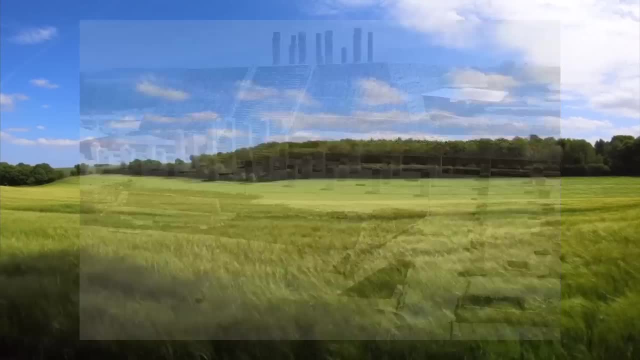 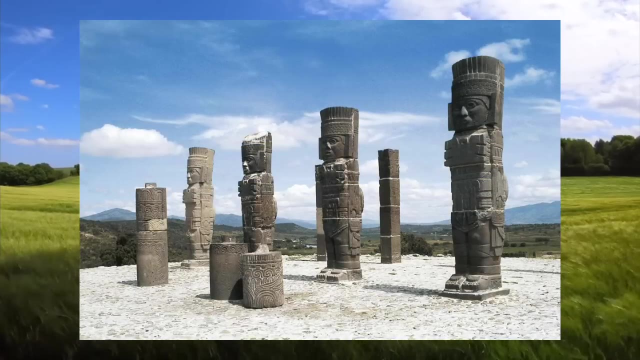 influences across the entire region. So these guys were basically just owned the entire Mesoamerica area, with iconic examples such as the Atlantean figures and the Pyramid of Quetzala. Despite their achievements, the decline of the Toltec civilization remained shrouded in mystery. Factors such as environmental changes, political instability, internal conflicts and external pressures from invading groups may have contributed to their downfall. Nevertheless, the Toltecs left an enduring legacy and the Aztecs who succeeded them in Central Mexico held the Toltecs in high esteem, Adopting and integrating elements of Toltec. 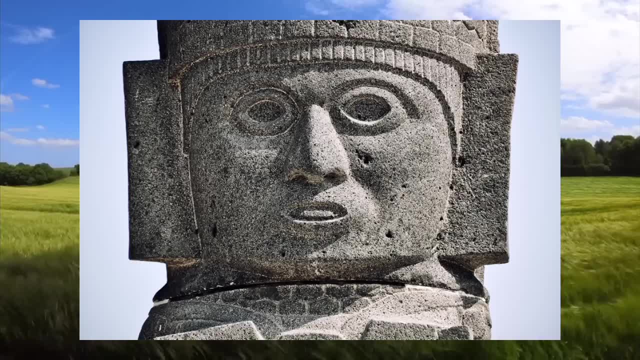 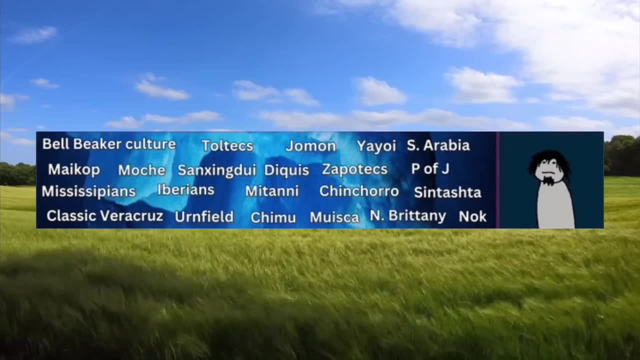 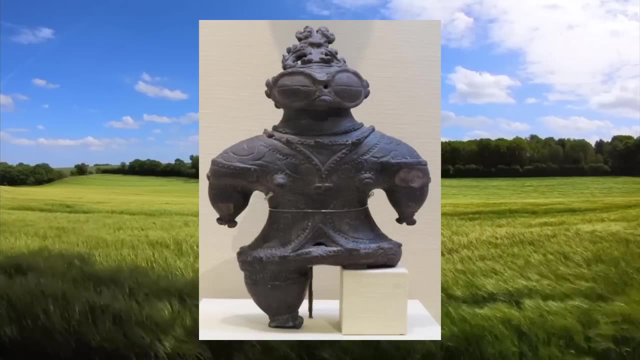 culture into their own. the Toltecs made notable contributions to Mesoamerican culture, including advancements in metallurgy, art and architecture. Jomon- The Jomon period spanning from approximately 10,500 to 1,500 BCE in Japan. 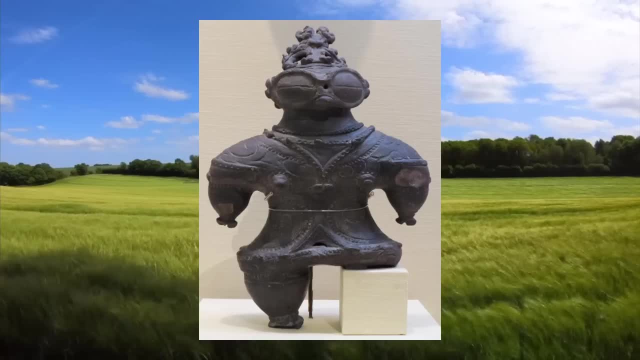 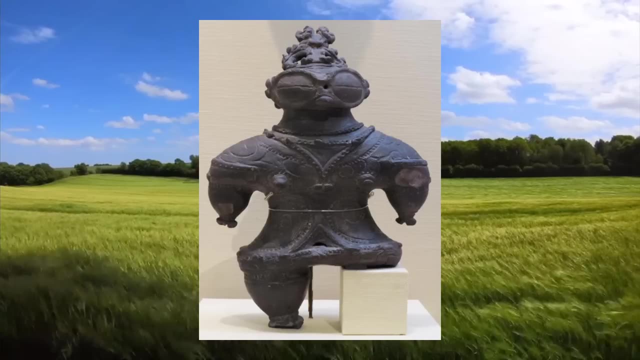 so these guys were around for like 9,000 years, so these guys basically just existed in Japan for all. of its history is a crucial chapter in the prehistoric history of the Toltec culture of the archipelago, Characterized by its distinctive cord-marked pottery and the 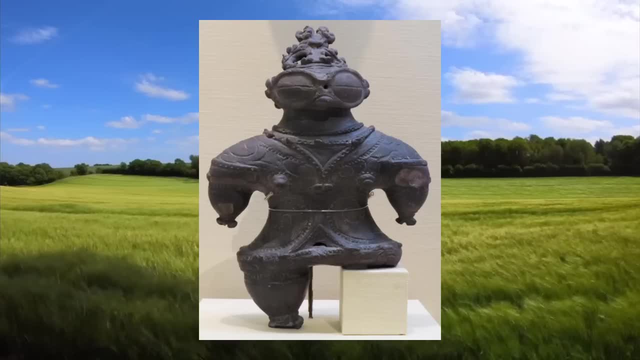 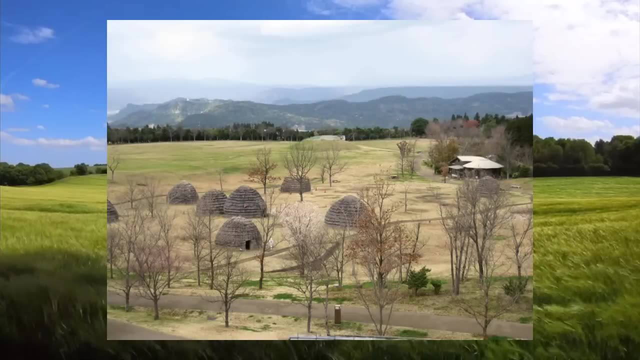 Jomon culture reflects the lifestyle of hunter-gatherers and fishermen. The period is divided into early, middle and late Jomon phases, each exhibiting unique characteristics. Central to Jomon culture is the remarkable pottery that bears cord-impressed decorations. These vessels 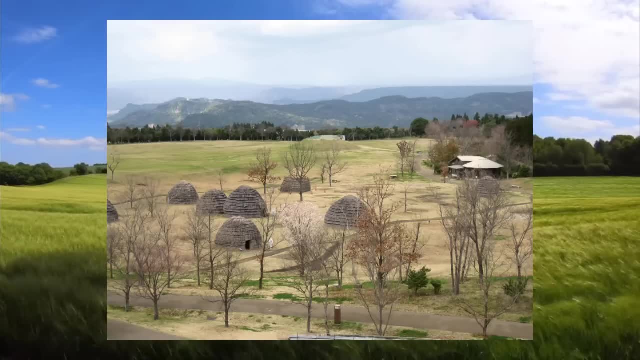 ranging in shape and size, served both practical and ceremonial purposes. The Jomon people living in pit dwellings that with that, the Jomon people were known as the Jomon people. The Jomon people were known as the Jomon people. relying on diverse range of resources, including seafood, nuts, berries and game. Cultural diversity was a notable aspect of the Jomon period, with regional variations in pottery styles and other practices. Despite their primary hunter-gatherer lifestyle, the Jomon people developed advanced. 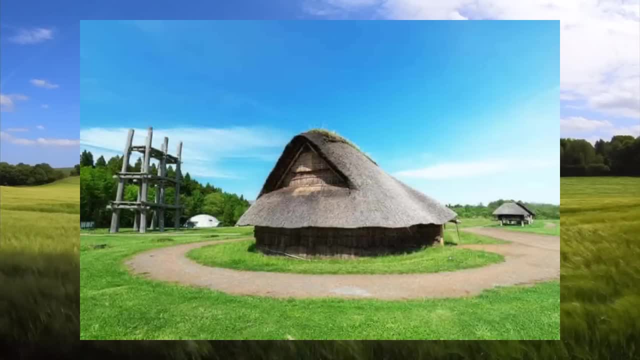 techniques in pottery production and crafted tools from stone, bone and antler. Pottery in particular played a pivotal role in their daily lives, contributing to cooking, storage and cultural expression. Burial practices during the Jomon period varied, encompassing simple pits and more elaborate. 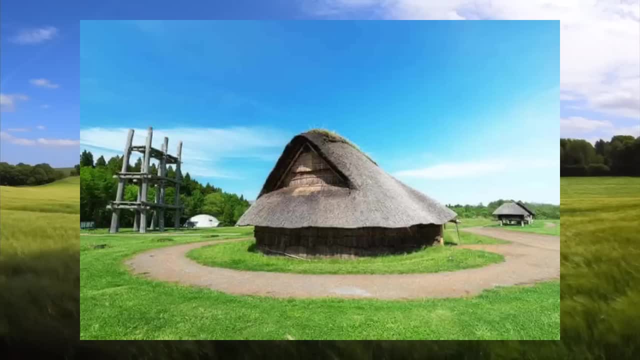 stone-lined structures. Some burials include grave goods such as pottery vessels and ornamental items made of stone or bone. Archaeological findings also point to the some existence of ceremonial sites suggesting the presence of rituals and communal gatherings. The Jomon period marked a 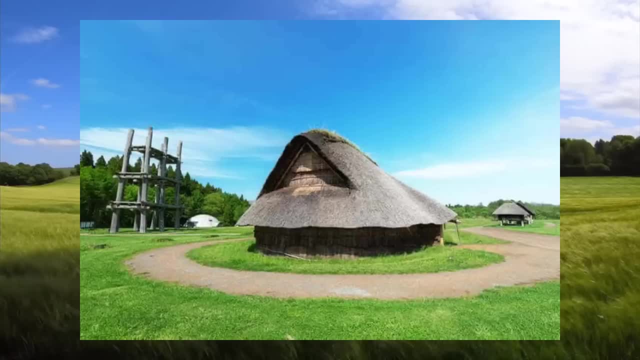 significant cultural stage in Japan's prehistory. as it transitioned into the Yaoi period, characterized by the introduction of wet rice cultivation and metalworking, The Jomon legacy persisted, and the technological advancements and unique cultural practices of the Jomon people laid the foundation for subsequent periods in Japanese history. 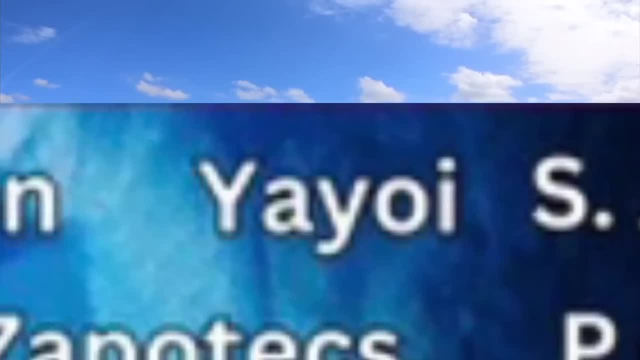 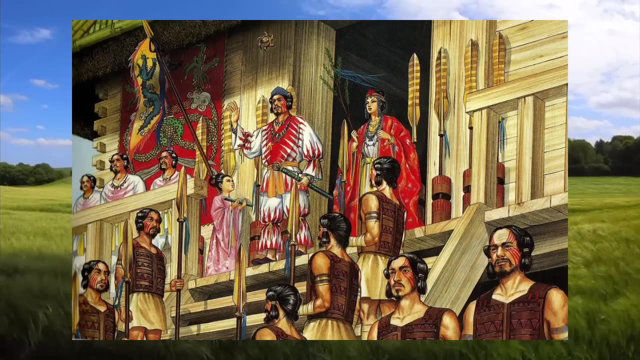 Yaoi. The Yaoi period, spanning approximately from 1000 BCE to 300 CE in Japan, signifies a transformative era following the Jomon period which we just talked about, Named after the Yaoi district in Tokyo. this period brought about significant changes in Japan's cultural landscape. 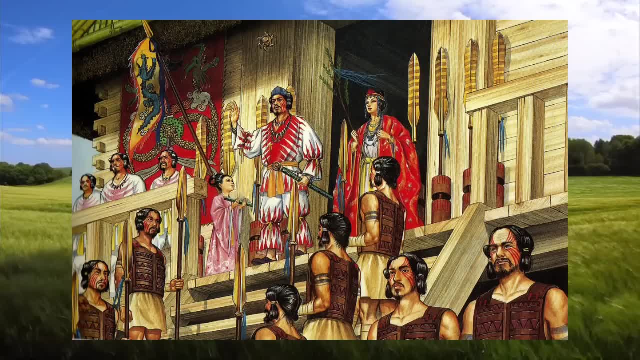 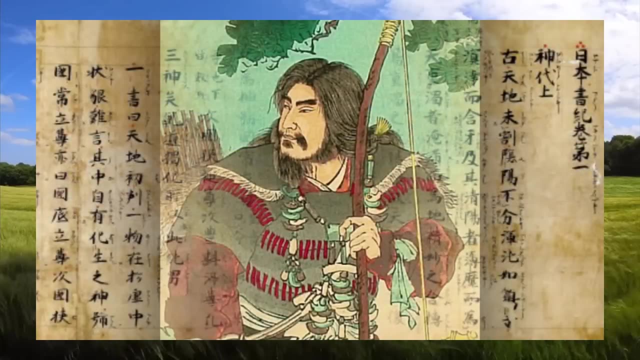 The introduction of wet rice cultivation, likely influenced by migrants from the Asian continent, marked a pivotal shift in the economy and social structure. Agriculture innovation allowed for settled communities, fostering larger villages and possibly the emergence of social hierarchies. A notable hallmark of the Yaoi period was the mastery of metalworking With the Yaoi. 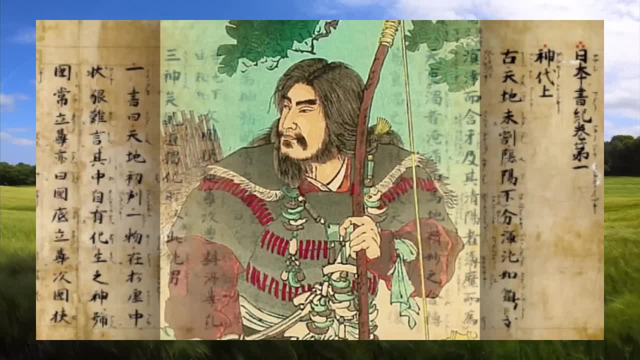 people producing bronze and iron items. this technological advancement over the preceding Jomon period played a crucial role in shaping material culture. Quartersốngקăn regrets the INC's participation in sank the Jomon period and catalyze cuisines and relics or ships that brought about Robert to the Jewish empire. Emoji of painting stands out as post-Jurgen. 1909 and Lem�장son's heroic style Introducing women and women's art and fashion. some reshaping, elevating Foi in the 19th century. A big positive of the shaved turtle. if you exit from the tuning order, from the 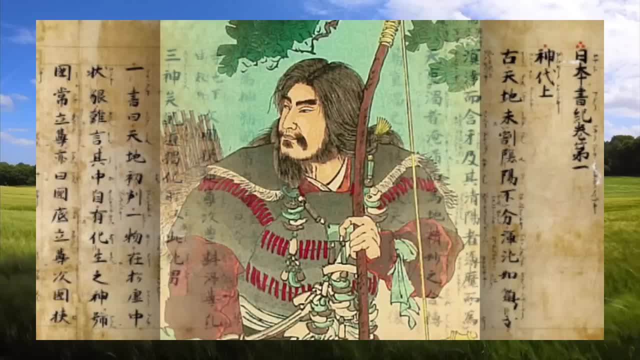 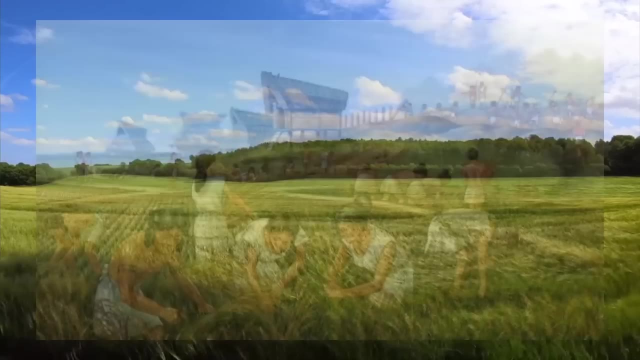 producing weapons tools and ceremonial objects. The transition from cord-marked jamon pottery to smoother decorated ceramics with geometric patter and applique designs further reflected cultural changes. As settlements grew and social structures evolved, burial practices underwent transformations as well. The Yayoi period witnessed the emergence of burial mounds, or kofun, particularly in its 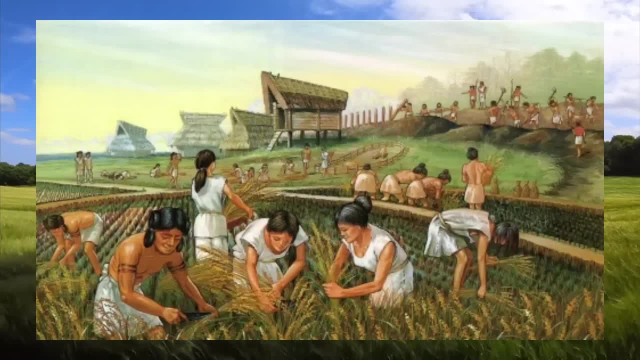 later stages. These mounds foreshadowed the kofun period that followed, characterized by the construction of elaborate burial mounds for elite individuals. Interactions with neighboring regions, notably the Korean Peninsula and China, increased during the Yayoi period. 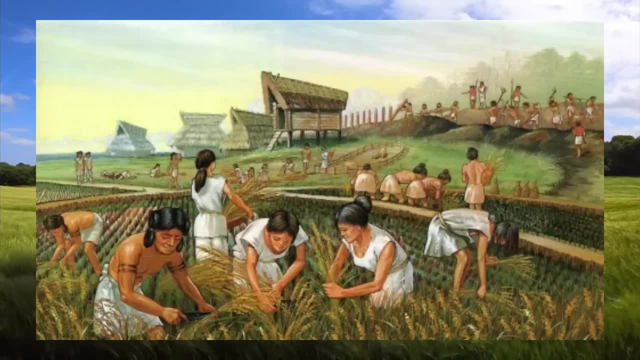 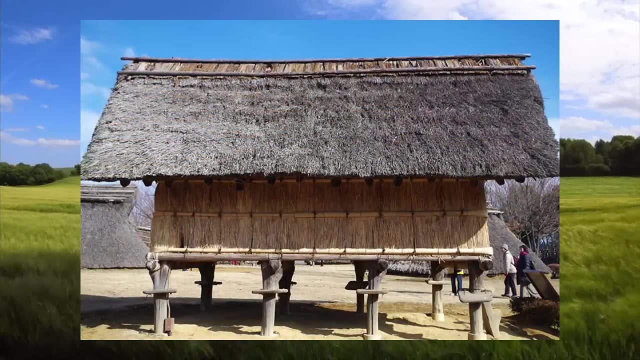 This exchange facilitated the flow of goods, technologies and cultural influences, contributing to the broader trajectory of Japanese civilization. The Yayoi period laid the groundwork for the subsequent kofun period, which marked the formation of early Japanese states. In summary, the Yayoi period represents a dynamic phase in Japanese prehistory and 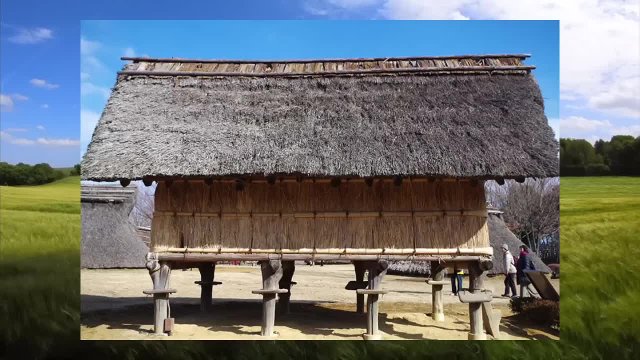 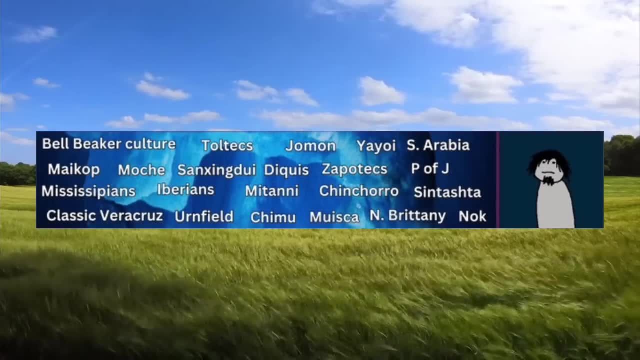 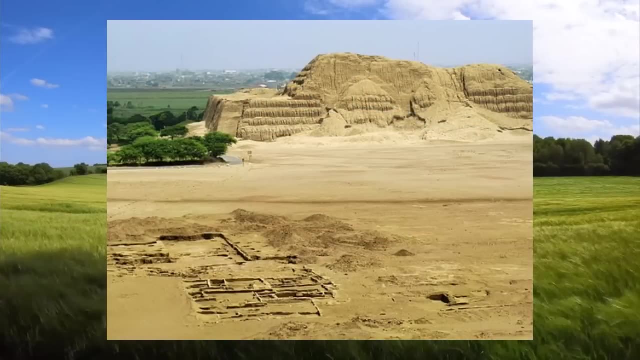 really kind of got it into not really the modern, but more modern area following the Jafon period, which we talked about earlier. Mochi: The Mochi civilization, also known as the Mochias civilization, emerged on the northern coast of Peru between 100 and 700 AD, occupying 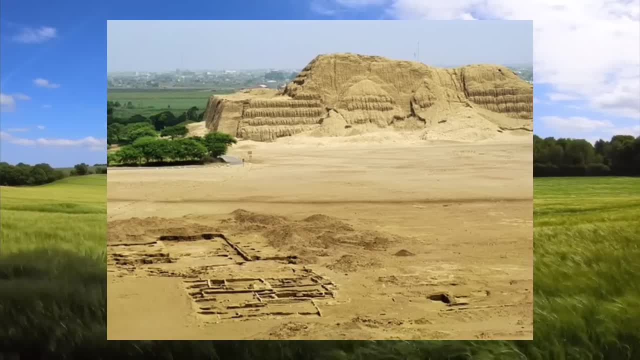 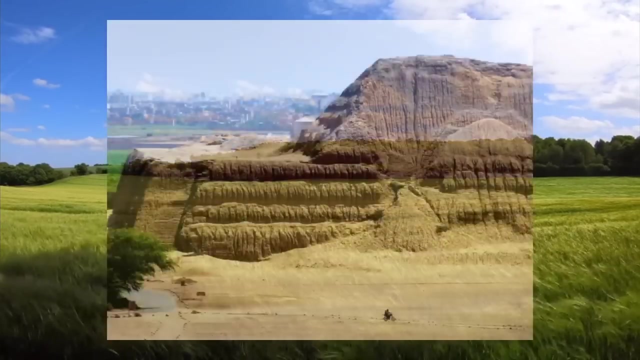 the valleys of the Chicama, Mochi and Laba Ganges In the Laba Creek rivers, the pre-Columbian society demonstrated advanced agricultural practices utilizing sophisticated irrigation systems in the arid coastal environment. Their social structure was stratified, reflecting distinct social classes and hierarchies. 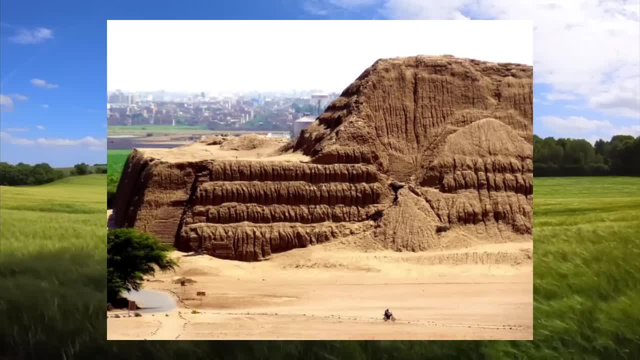 One of the most remarkable aspects of the Mochi civilization was their artistic prowess. Renowned for their pottery, the Mochi created intricate and expressive vessels depicting scenes from everyday life, religious rituals and mythology. The pottery showcased a mastery of naturalistic representations of human figurines and animals. Additionally, the Mochi excelled in metallurgy, producing elaborate gold and silver artifacts that reflected their skilled craftsmanship. Religion also played a central role in Mochi society, with a complex belief system evident in their art and architecture. Ceremonial pyramids such as the Hoa del Sol and the Huaca de la Luna served as religious. 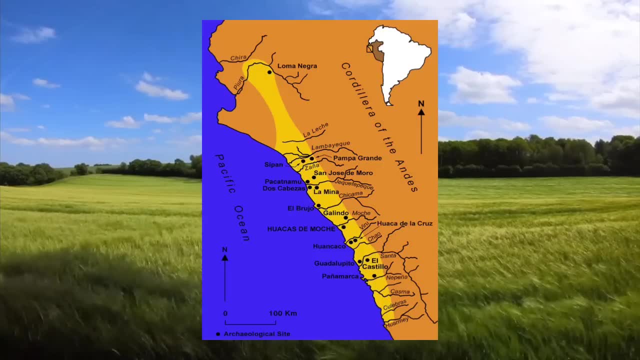 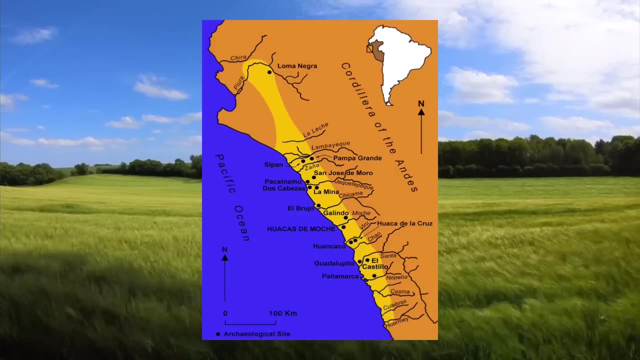 and political centers. These structures were associated with the Mochias. The Mochias were also known as the Mochias, Both rituals and ceremonies depicted in Mochi artwork. Despite their civilization's achievements, the Mochi eventually experienced a decline. 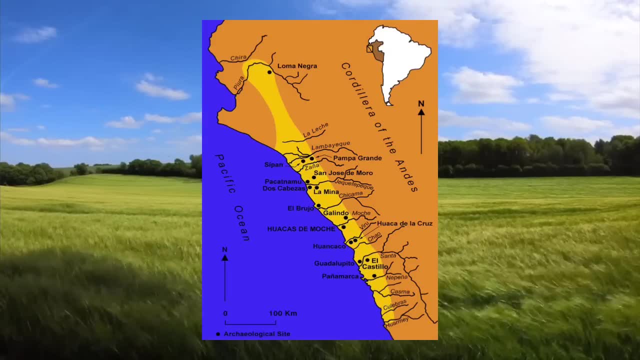 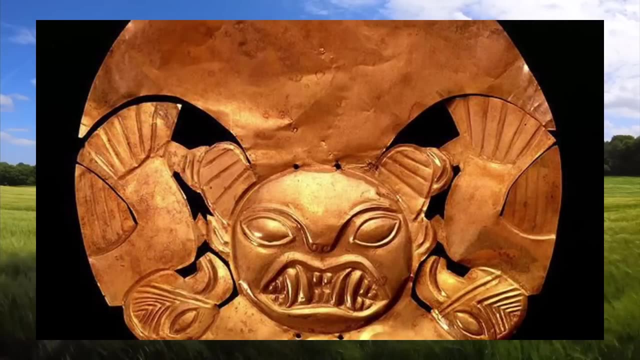 The precise reasons for their downfall remain unclear and may involve a combination of different factors, including climate change, environmental degradation, internal conflicts or external pressures. The Huacas, or pyramids left behind by the Mochi, such as the Huaca del Sol and Huaca. de la Luna stand as enduring archaeological sites that continue to contribute to our understanding of this intriguing ancient civilization. Ongoing research and excavations further illuminate the complexities of the Mochi civilization and its place in the pre-Columbian South American societies. 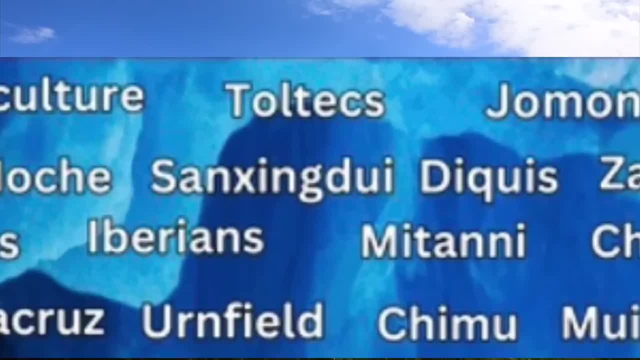 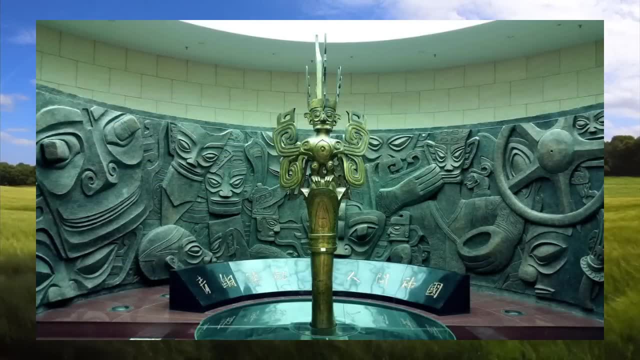 Songxingde, located near Guohang in Sichuan Province, China, entered the archaeological spotlight in 1986 following the discovery of a vast collection of Bronze Age artifacts. This was a great discovery. It was the first discovery of a bronze-age artifact. 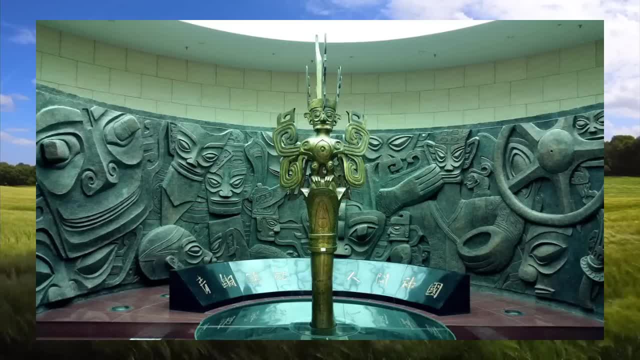 It was the first discovery of a bronze-age artifact. It was the first discovery of a bronze-age artifact. Songxingde gained prominence due to its unique insights into a Bronze Age civilization that thrived approximately 3,000 years ago during the Zhang and Zhao dynasties. 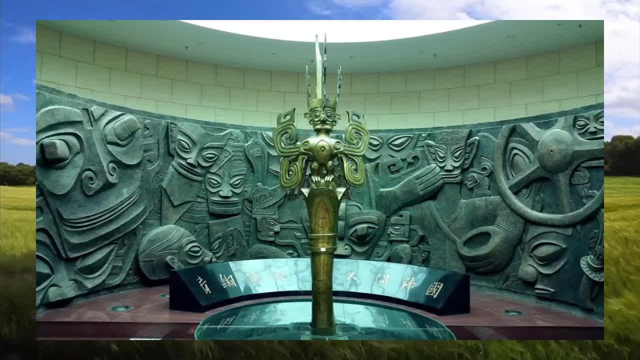 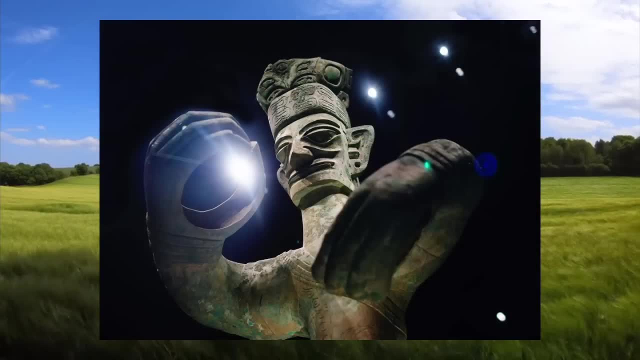 This culture, contemporaries with the ancient Chinese civilization in the Yellow River Valley, challenges previous assumptions about the homogeneity of Bronze Age cultures in China. The archaeological finds at Songxingde are characterized by their artistic and technical sophistication. Notable among these discoveries are the bronze-age carvings. 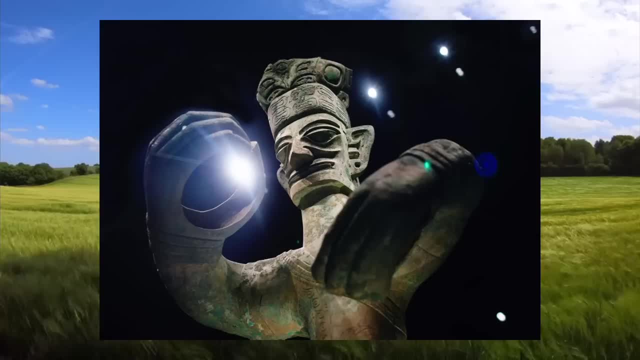 The bronze-age carvings are large bronze statues, bronze masks, jade objects, ivory and pottery. The bronze artifacts, especially the distinctive masks with exaggerated facial features, reveal a unique artistic style not previously identified in any other ancient Chinese culture. The purpose of Songxingde and the reasons behind its eventual abandonment remain subjects. 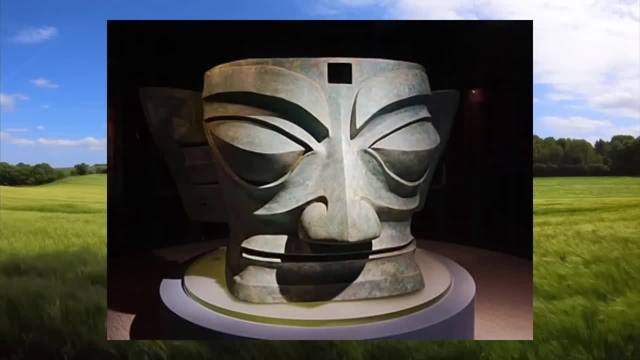 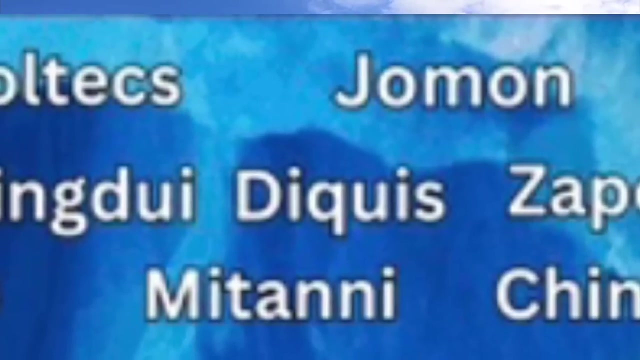 of debate. The site's significance is underscored by the discovery of a sacrificial pit containing numerous intentionally smashed and buried artifacts. The artifacts found at Songxingde have contributed significantly to our understanding of ancient Chinese civilizations. Dequiesse: The Dequiesse ancient civilization refers to a pre-Columbian culture that thrived in the 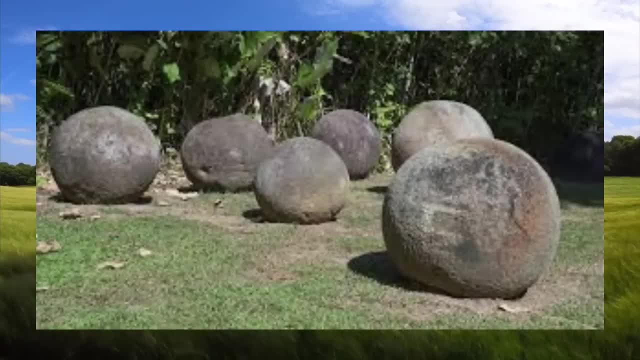 southern Pacific coastal region of Costa Rica, primarily in the Dequiesse Delta and the Osa Peninsula. The Dequiesse civilization existed from about 700 to 1538.. The Dequiesse civilization was a very popular civilization. The Dequiesse civilization was a very popular civilization. 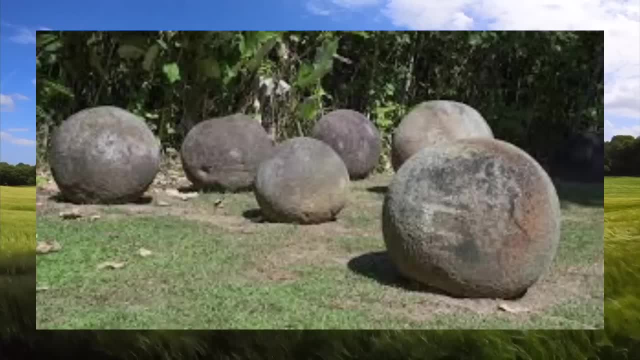 The Dequiesse civilization was a very popular civilization. It keyed the紀 Vitr něgr Towne conflict in the last century AD and is known for its distinctive artifacts, particularly the mysterious stone spheres. The Dequiesse culture left behind a remarkable archeological legacy, with a focus on the 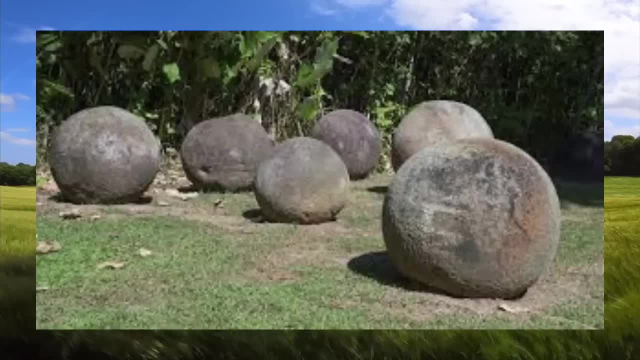 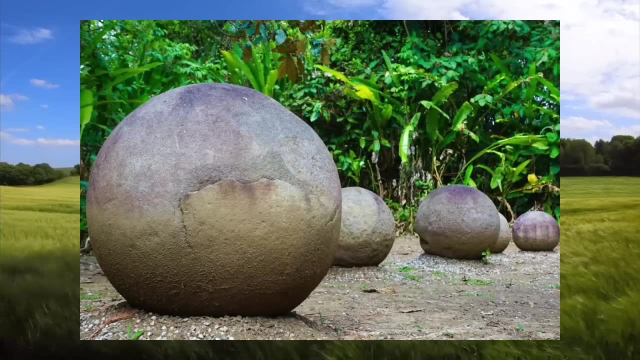 creation of stone spheres ranging from size small to monumental. These spheres, often referred to as the Dequiesse Spheres or Costa Rican Stone Spheres, were crafted with precision and are scattered all throughout the Dequiesse Delta and the surrounding. 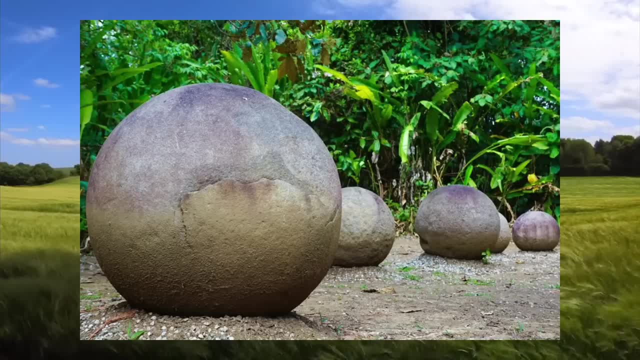 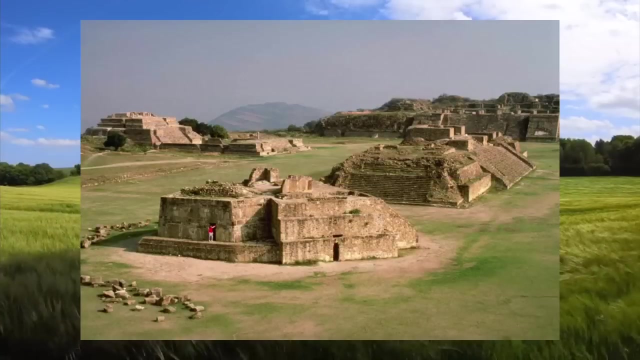 areas. The purpose of these spheres remains a subject of speculation and various different theories or cultural significance. The archaeological sites associated with the decreased ancient civilization provide valuable insights into their daily lives, their social organization and cultural practices. Zapotex- The Zapotex, an ancient indigenous civilization flourished in 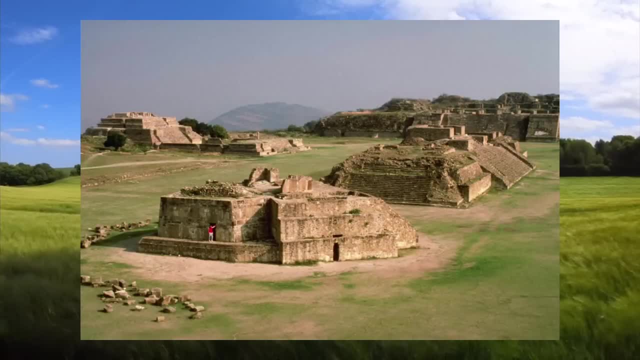 the valleys of Aaxaca, southern Mexico, and played a crucial role in the early development of complex societies in Mesoamerica. Monte Albin, established around 500 BC, served as their capital and became one of the earliest and most significant urban centers in the region. The Zapotex were adept. 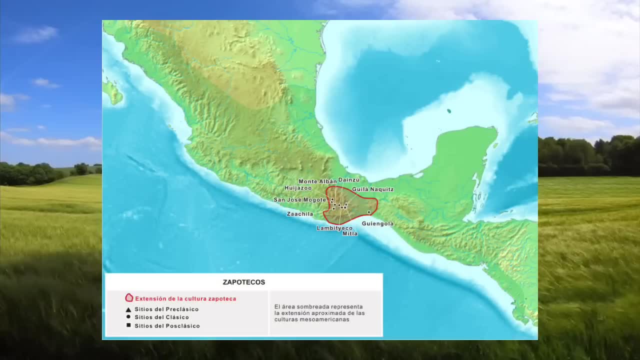 farmers cultivating maize beans and squash in the fertile Axian soil and engaged in trade with neighboring cultures. Monte Albin, characterized by its intricate stone carvings, ceremonial platforms and the ball courts, showcased advanced urban planning and engineering. The Zapotex 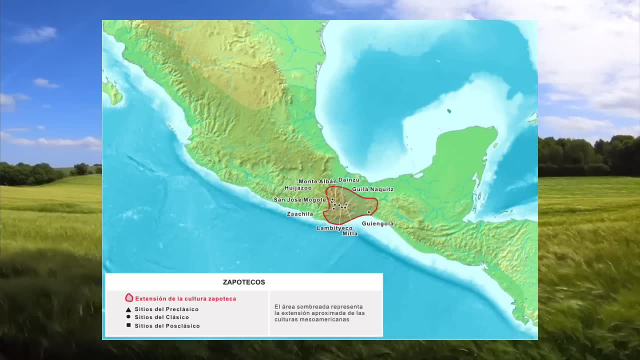 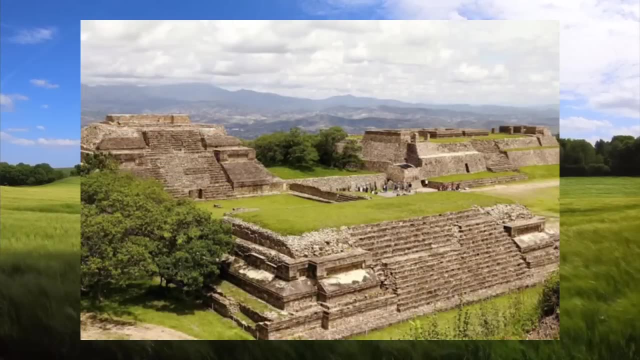 developed one of Mesoamerica's earliest writing systems, Primarily used for recording calendar information on stelae and other artifacts. their art, including pottery and jewelry, reflected a rich cultural expression. The Zapotex had a complex religious belief system incorporating deities associated with agriculture, fertility and 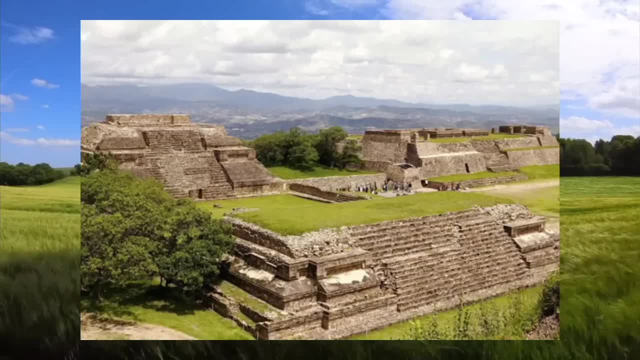 natural elements into their rituals, often conducted in ceremonial plazas and pyramids. Despite their cultural achievements, the decline of Monte Albin and their Zapotex civilization around 800 to 1000 AD remains a topic of study, with factors such as the size of the city, the size of the city's population and the 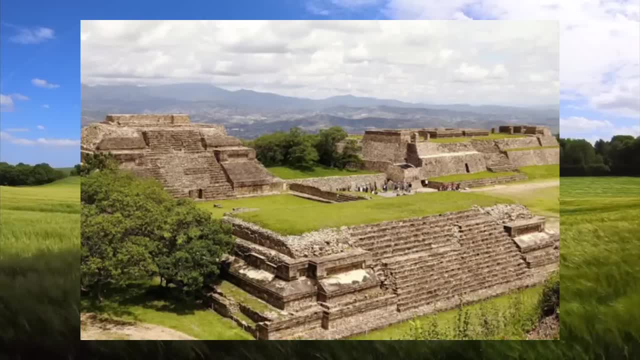 size of the city's population's population. The Zapotex were considered as potential contributors to their fall. While the ancient Zapotex civilization declined, the Zapotex people continued to be a vital culture and ethnic group in Osaka, preserving their heritage through language. 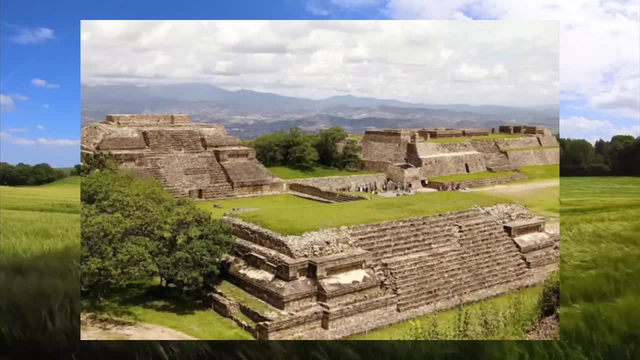 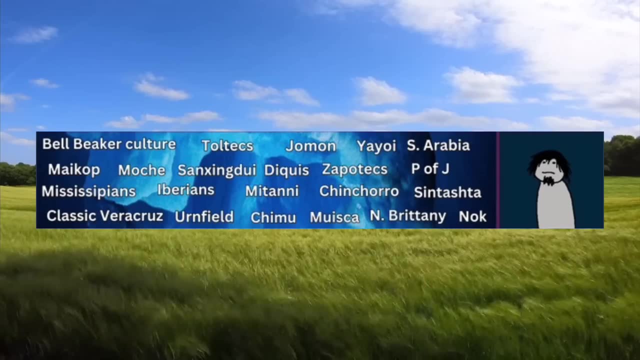 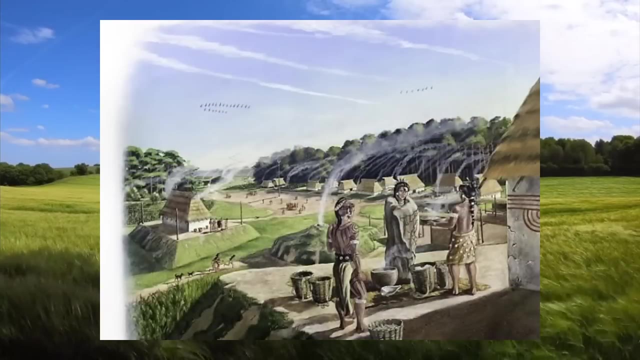 traditions and crafts. The legacy of the Zapotex contributes significantly to the broader understanding of ancient Mesoamerican civilizations. P of J Mississippians. The Mississippian culture was a native of the American civilization that thrived in Midwestern, Eastern and Southeastern United States from 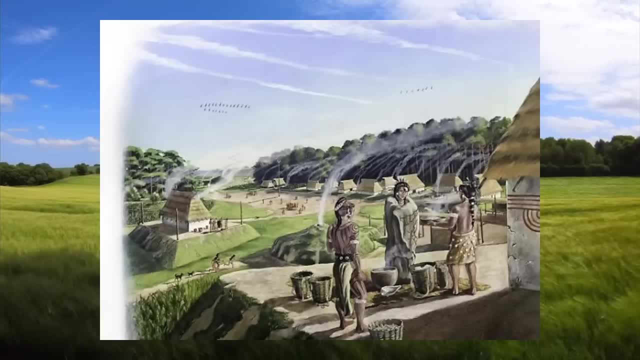 approximately 800 to 1600 AD, although the specific timeline varied across regions Noted for constructing large earthen platform mounds and other shaped mounds. this culture was composed of urban settlements and satellite villages connected by informal trading networks. The most prominent city associated with the Mississippian culture was Kohaka, situated in present-day. 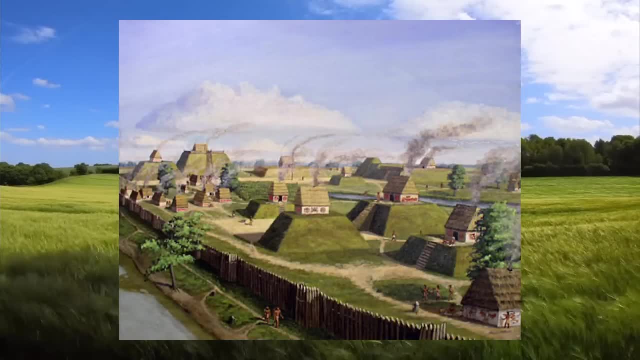 Illinois and believed to be a major religious center. The development of the Mississippian way of life originated in the Mississippi River Valley, from which the culture takes its name. Characteristics associated with Mississippian culture also appeared in the tributary Tennessee River Valley. The majority of dated Mississippian 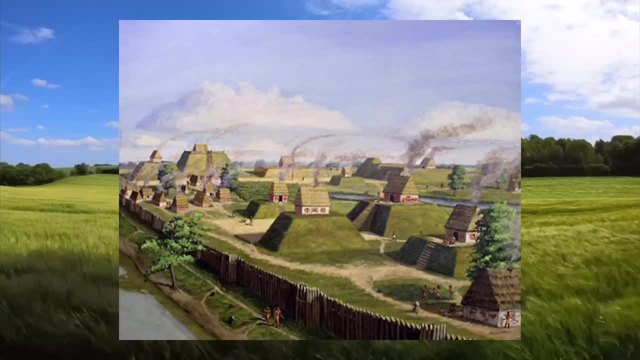 sites proceeded the year 1539 to 1540, so within a year, the time of Hernando de Soto's exploration of the area. However, exceptions include Neche's communities, which continued to practice Mississippian culture or traditions into the 18th century, The hallmark of Mississippian civilization. 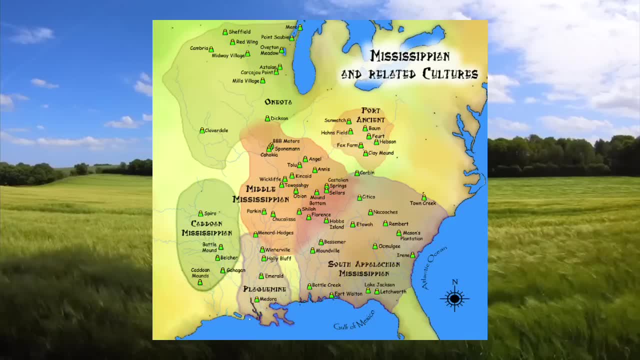 was its impressive earthen mounds, often serving ceremonial, religious or elite residential purposes. These mounds, including the iconic Monks Mound at Kohaka, reflected the complex social organization and the cultural practices of the Mississippian people. 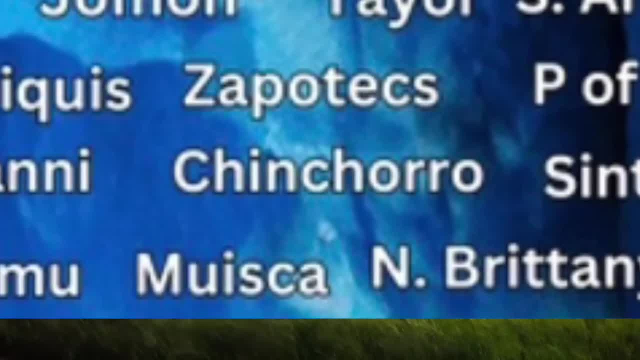 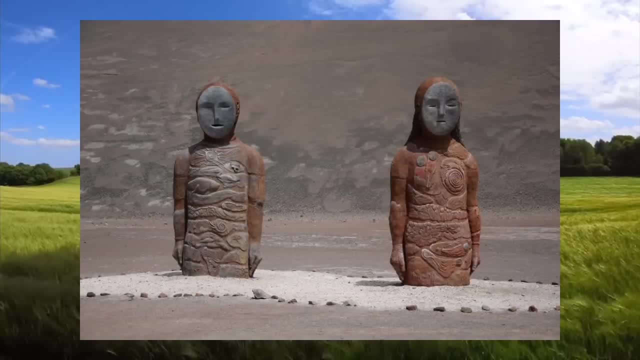 Chinchorro. The Chinchorro culture, flourishing along the coasts of present-day northern Chile and southern Peru, is dissuaded by its advanced and early mummification practices spanning a timeline from around 7,000 BCE. The Chinchorro people developed intricate methods. 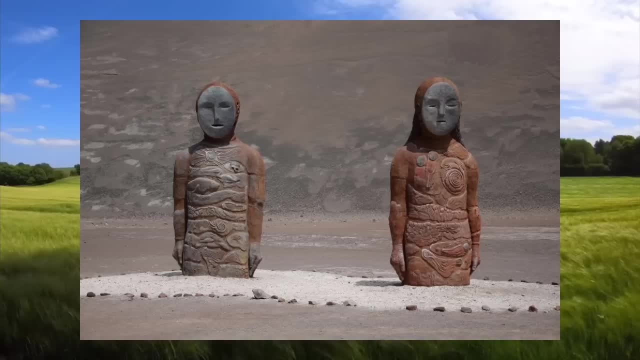 of preserving their deceased, showcasing a mastery of artificial mummification well before the renowned practices of ancient Egypt. This process involved the removal of internal organs, reinforcement of the body with sticks and wrapping in a clay and ash mixture, with further wrapping in reeds and 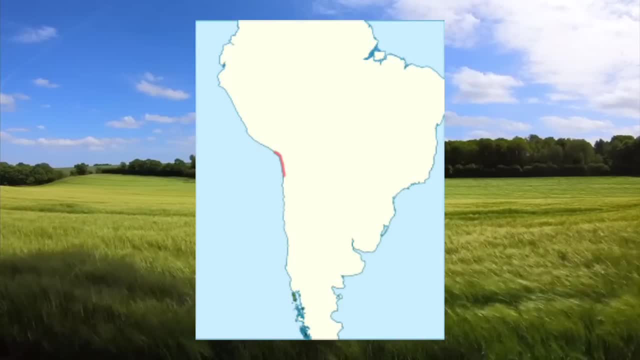 fabric. The mummification techniques of the Chinchorro people underwent two main chronological phases: The early Chinchorro, phase spanning roughly the same period of time as the early Chinchorro, The Chinchorro culture flourishing along the coasts of present-day northern Chile and southern Peru. 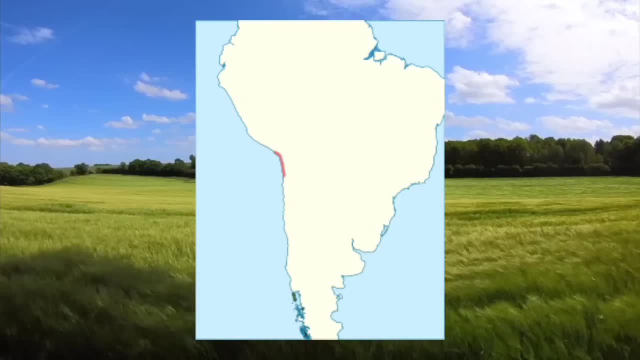 was dissuaded by the early Chinchorro culture. The Chinchorro culture flourishing along the east and southern Peru. The Chinchorro culture, wealthier at 5,200-4,000 448, It's currently felt south from the. recordings of several of these less important practices Pioneering coastal these rich ethnic tribes alike: Hdon' Ogo, Hanoi, io' vocal and records call the main tribal with many amount of руси indigenous vocabulary From which these official names can be abstractly providing. 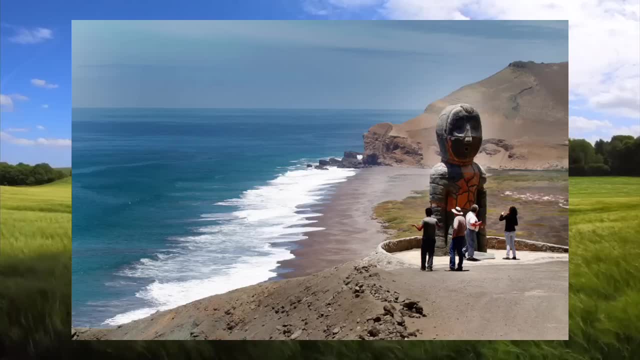 meaning as to their national origins. certain visitors all over the world will encounter environment shaped their economic and lifestyle practices. Archaeological sites have yielded a range of artifacts, including pottery baskets, fishing tools and ritual objects, providing valuable insights into their daily life and cultural richness of the Chinchorro people. 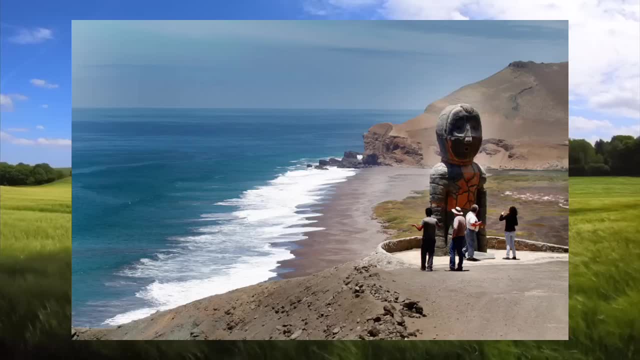 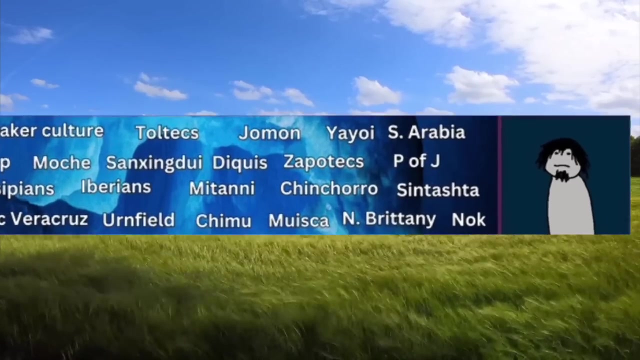 The legacy of the Chinchorro culture lies in its contribution to the understanding of early human burial practices. Their mummies, both natural and artificial, stand as a testament to the cultural complexity and adaptability of prehistoric South American societies. 5. Sintashtja. 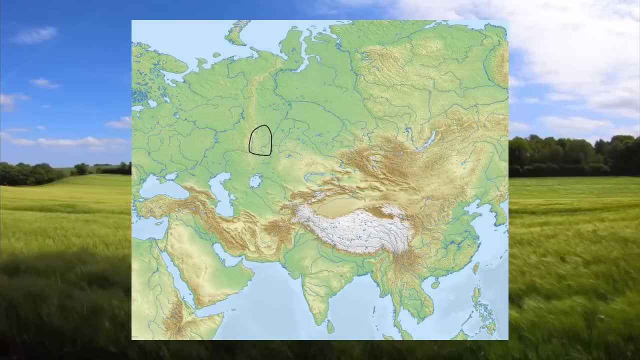 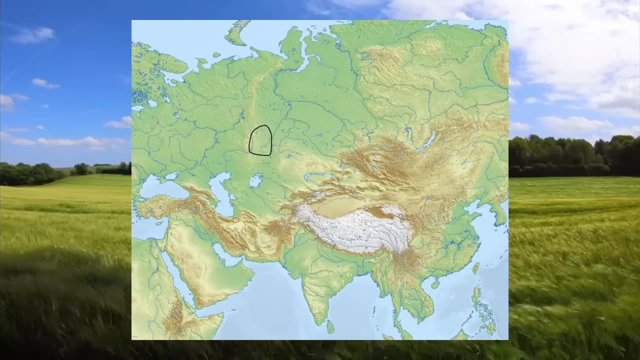 The Sintashtja culture, rooted in the southern Urals of Russia during the Bronze Age, has left a significant archaeological imprint on the Eurasian Steep. The excavations at Sintashtja have uncovered fortified settlements and burial mounds, revealing a society with an advanced 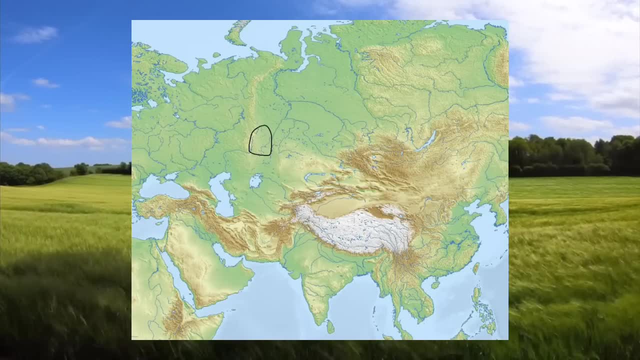 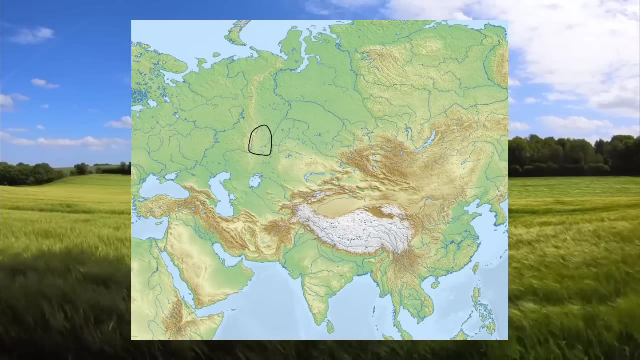 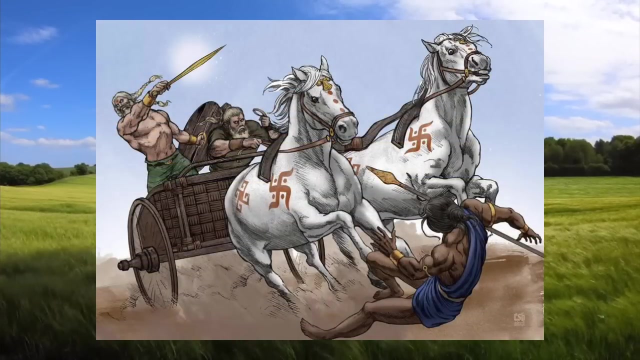 military organization and defensive capabilities. The complexity of these structures underscores the strategic and possible hierarchical nature of the Sintashtja community. At the heart of the Sintashtja culture lies its remarkable achievements in metallurgy, particularly bronze metallurgy. The people of Sintashtja were adept metalworkers. 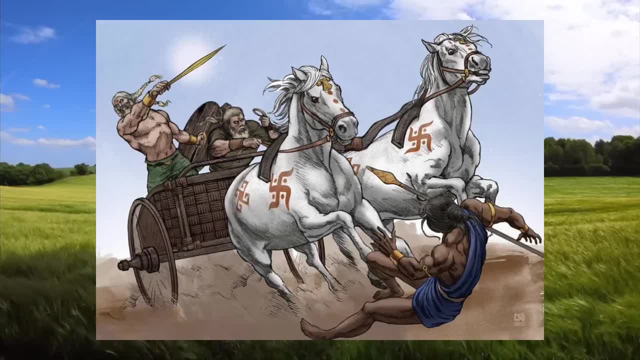 producing an array of sophisticated tools and weapons. Of note are the chariots that have spoked wheels, indicative of technological prowess and the utilization of domesticated horses. This technological advancement suggests not only an agricultural base, but also the development of mobile pastoralism, as horses played a crucial role in their culture. The 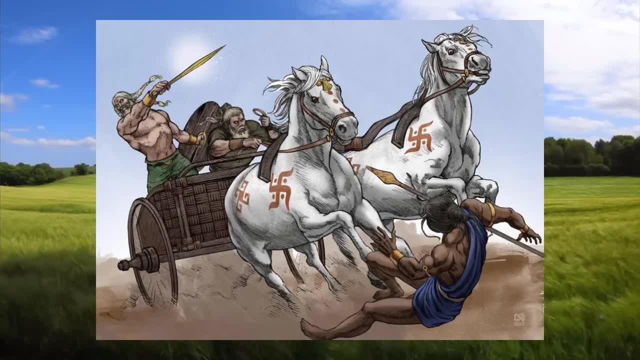 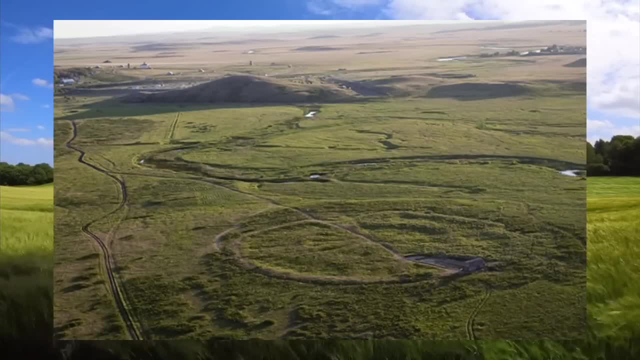 Sintashtja culture is part of the broader Andromino culture complex extended across the Eurasian Steep. It is associated with early Indo-Iranians and is seen as a precursor to later Indo-Iranian-speaking cultures. This cultural context places Sintashtja at the crossroads of 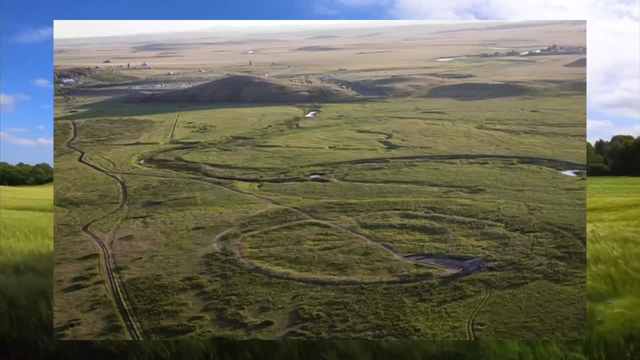 significant historical and linguistic developments, contributing to our understanding of the Indo-European migrations that shaped the demographic and linguistic landscape of Eurasia. Economically, the Sintashtja people engaged in a combination of pastoralism and agriculture, emphasizing the breeding of horses. 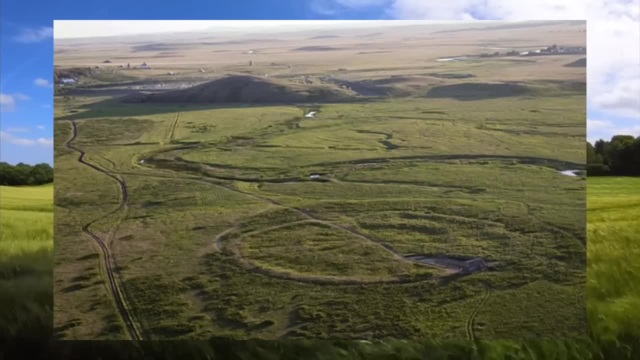 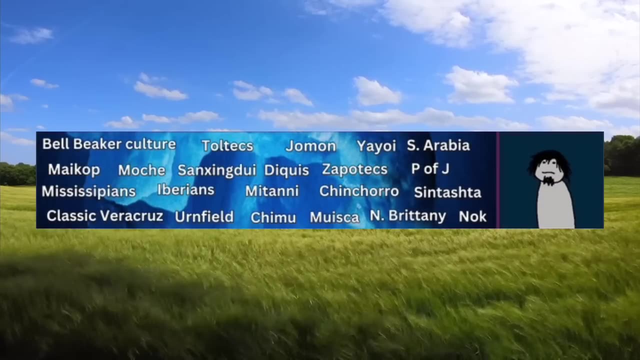 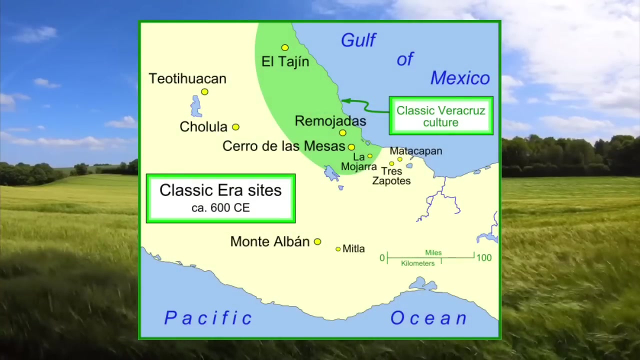 cattle and sheep, and this dual economic strategy likely played a role in sustaining their society and supporting advancements in technology and mobility. Classic Veracruz. Classic Veracruz, a cultural and artistic period that thrived on the Gulf Coast of Mexico during the Mesoamerican Classic Era, is recognized for its unique. 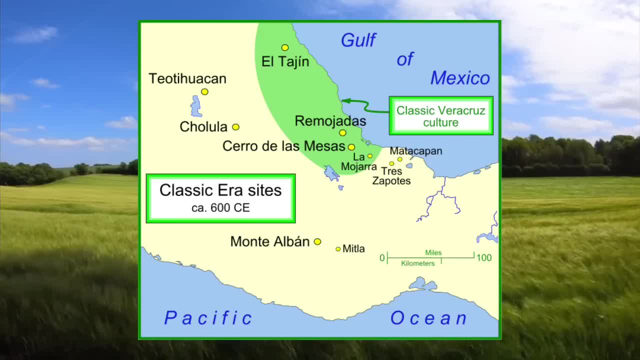 contributions to the rich tapestry of ancient Mesoamerican civilizations Situated in the coastal and lowland regions of modern-day Veracruz. this culture emerged from a fusion of influences drawing from predecessors like the Almanac and the contemporaries such as Teotihuacan and the Maya. 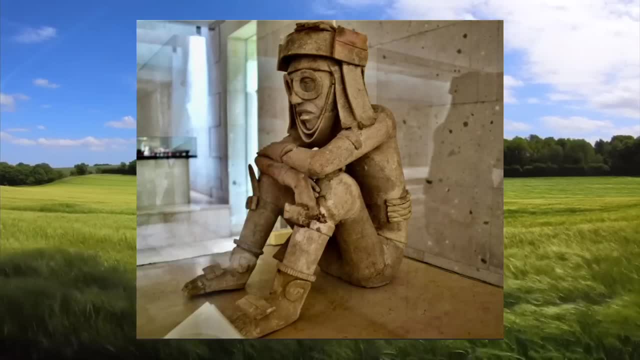 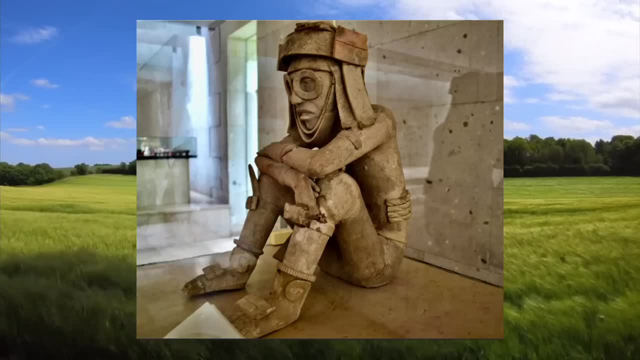 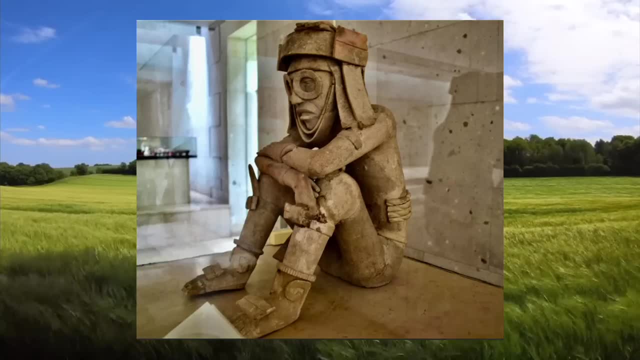 scenes related to warfare, ritual bloodletting and shamanistic practices, providing insights into the cultural and religious aspects of their society. El Tajín, a major city in the Tontanic region of Veracruz, stands as a testament to the achievements of classical Veracruz, Notable for its architectural 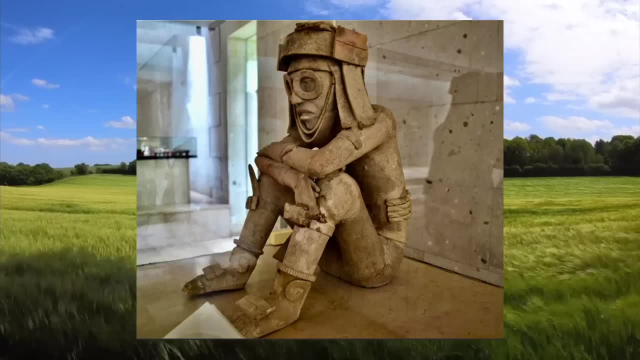 marvels such as the Pyramid of Neches and extensive ballgame courts. El Tajín reached its 10th. during the classic period, It served as a vital center for trade, religious ceremonies and artistic expression, reflecting the sophistication and vitality of classic. 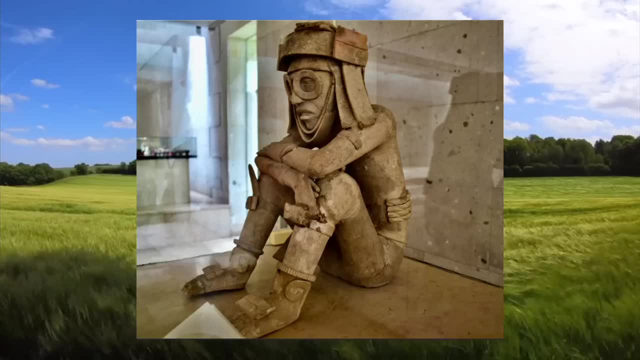 Veracruz culture. Participation in extensive trade networks was a defining feature of classic Veracruz. The region's coastal location facilitated maritime trade routes, fostering exchanges of obsidian, ceramics and luxury items with neighboring cultures. This engagement in trade contributed to the cultural dynamicism and interconnectedness 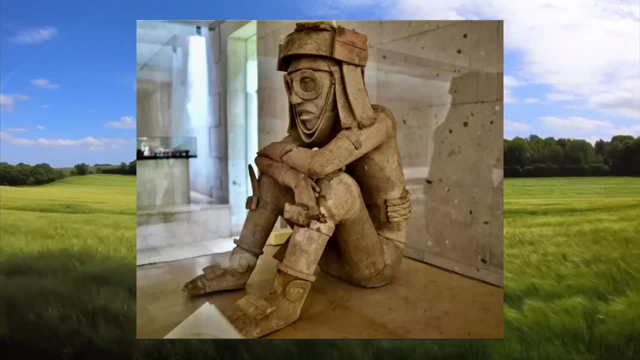 of the Mesoamerican societies during this period. Despite its cultural vibrancy, classical Veracruz experienced a decline around 1000 CE, with factors such as environmental changes, societal shifts and potential interactions with other cultures contributing to their transformation and their downfall. 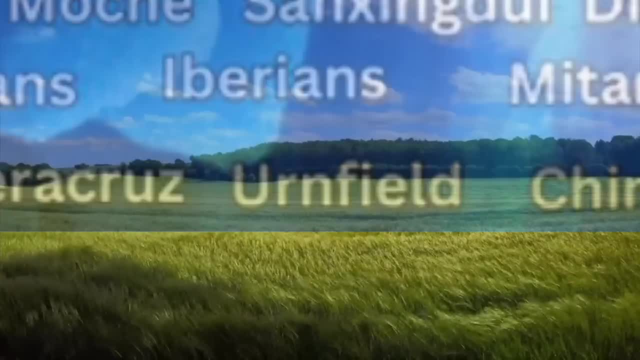 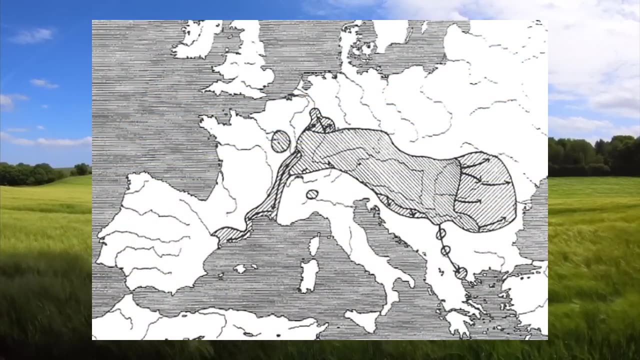 Urnfield. The Urnfield culture, spanning from around 1300 BCE to 750 BCE, stands out as a distinctive Bronze Age civilization. The Urnfield culture was established in Central Europe, Named after its characteristic burial practice of placing ceramics, remains and urns. the culture originated in regions encompassing 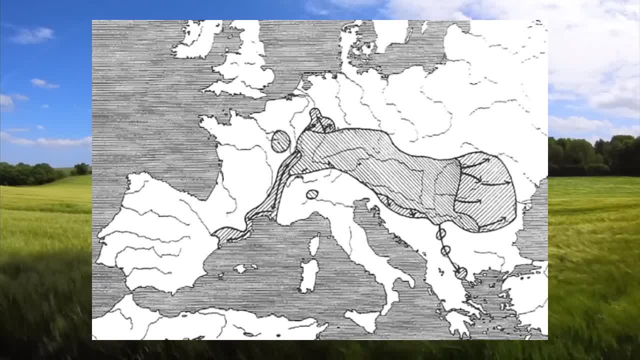 modern-day Germany, Austria, the Czech Republic and Hungary, before expanding across Central Europe. The hallmark of the Urnfield culture lies in their burial custom, creating vast cemeteries with urns arranged in fields. This culture marks a crucial transition phase, bridging 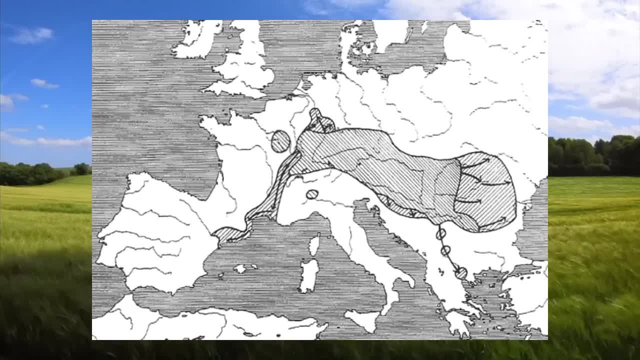 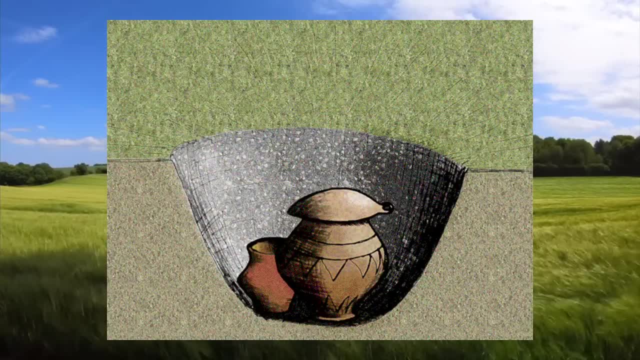 the Late Bronze Age and the Early Iron Age. As part of this transition, the Urnfield people adopted iron technology alongside their traditional use of bronze. Their economy was grounded in agriculture, livestock breeding and advanced metalworking- The production of iron tools. 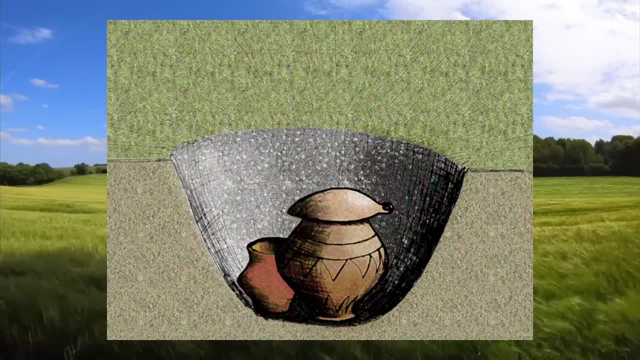 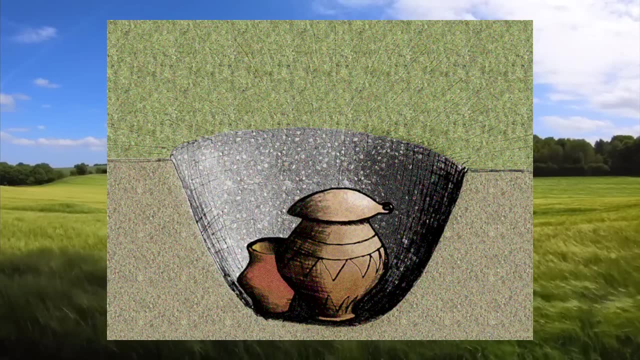 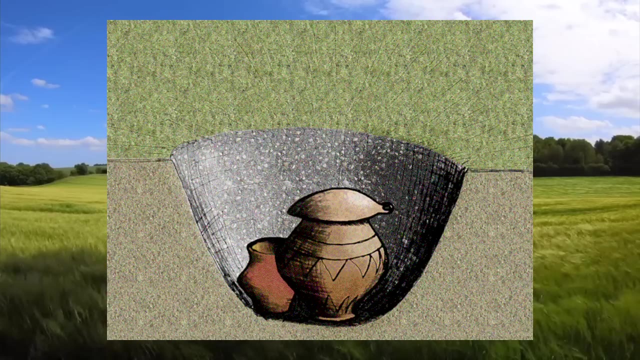 and weapons reflected a significant technological shift. during this era, The Urnfield culture was not isolated but engaged in cultural exchanges with neighboring societies. It is integrally linked to the broader framework of Central European and Alpine cultures, contributing to the rich tapestry of Late Bronze Age and the Early Iron. Age developments. Interactions during this period played a crucial role in shaping regional identities and cultural landscapes. While the precise reasons for the decline of the Urnfield culture remains elusive and highly debated, factors such as climate change, migration patterns and social transformations likely contributed to their downfall and disappearance. The decline 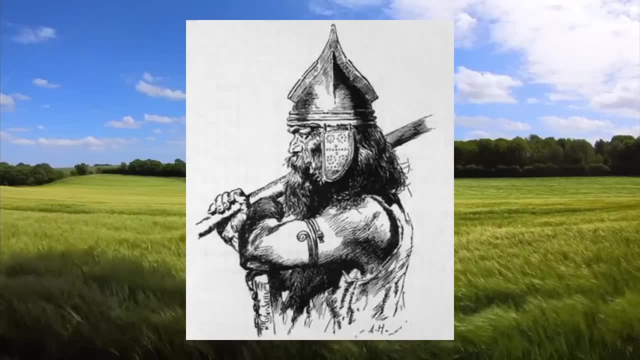 coincided with the emergence of new cultures and societies in Central Europe, signaling a dynamic period of cultural evolution. The legacy of the Urnfield culture endures through its impact on archeological records and cultural heritage. The Urnfield culture has a long history of 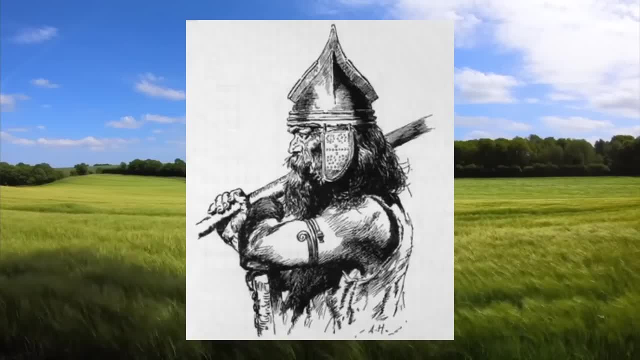 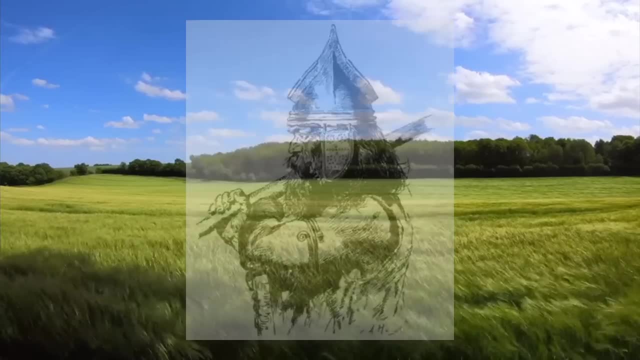 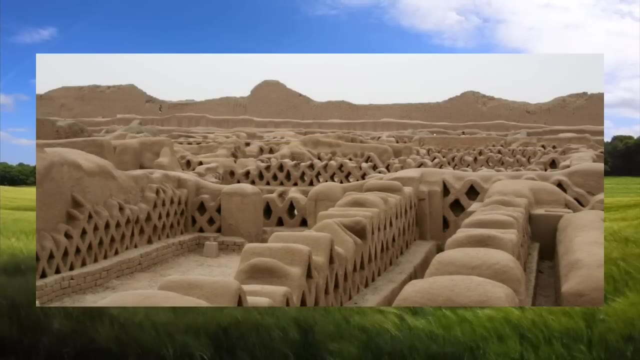 being a symbol of the historical record of Central Europe, Its unique burial practice. technological innovations and cultural interactions have left a lasting impact on the understanding of the region's ancient past: Chi Mu, The Chi Mu civilization flourishing along the northern coast of Peru. 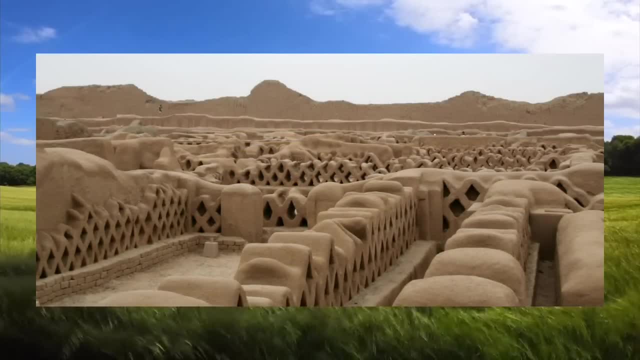 from 900 CE to 1470 CE left an indelible mark on the pre-Columbian landscape. At the heart of this ancient culture stood Chan Chan, an unparalleled adobe city and the largest in the ancient world. Chan Chan's intricate architecture featuring massive walls. 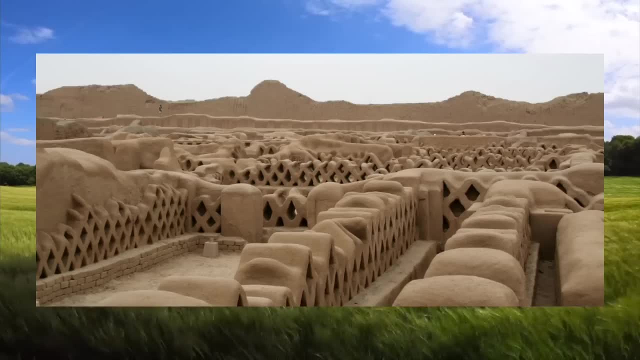 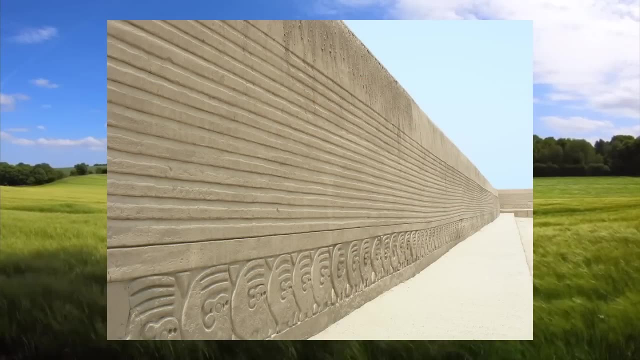 plazas and segmented compounds served as the bustling capital of the Chi Mu civilization, Organized into distinct sectors for administration, residence and ceremonies. Chan Chan exemplified the advanced urban planning of the Chi Mu people. Economically, the Chi Mu were adept farmers utilizing sophisticated irrigation systems to cultivate. 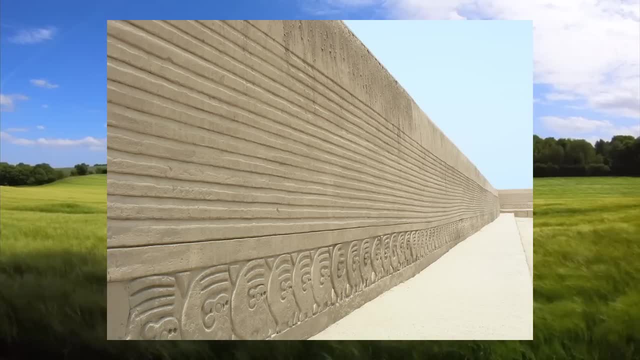 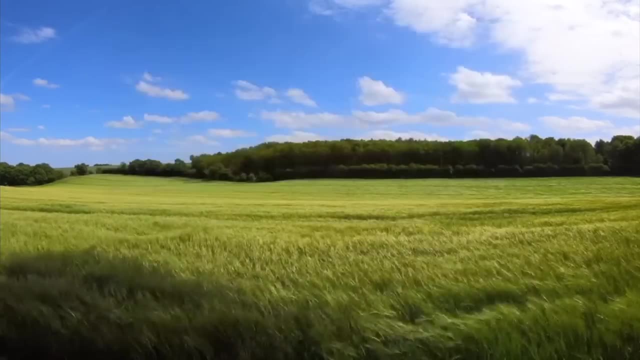 crops in the arid coastal environment. Fishing also played a crucial role in the city's way, Tapping into the rich marine resources of the coastal waters. the integration of agriculture and maritime practices supported a thriving Chi Mu economy, Renowned for their craftsmanship. 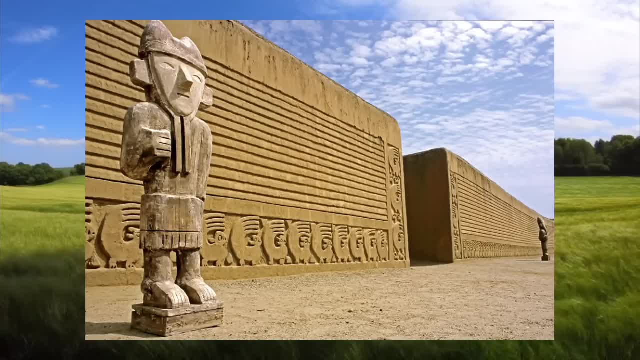 the Chi Mu excelled in metallurgy as well and textiles. Elaborate gold and silver artifacts, along with finely woven textiles incorporating cotton and various fibers, showcased the skill and artistic expression of the Chi Mu people. Their artistry extended to religious practices as well as evidenced by intrinsic 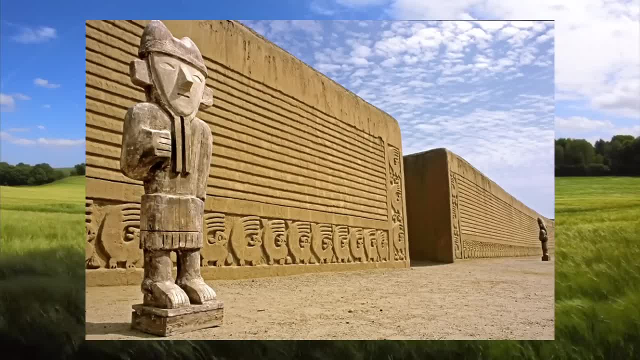 religious in both artwork and architecture. The zenith of the Chi Mu civilization coincided with the emergence of the Chamorro Kingdom around 1000 CE. Through military conquests and strategic alliances, the Chamorro Kingdom expanded its influence over a significant stretch of the. northern Peruvian coast. However, the Chi Mu civilization faced a decline in the late 15th century, marked by the encroachment of the Inca Empire In 1417 CE. the Inca ruler, Tupac Inca, led to the assimilation of the Chi Mu territory into the vast Inca Empire. The legacy of the Chi Mu civilization was pretty big and the archaeological remnants of Chon Chon and the artifacts that reflected their advanced society, The intricate urban planning, agricultural innovations and artistic achievements of the Chi Mu contributed significantly to our understanding of pre-Columbian and South American culture. 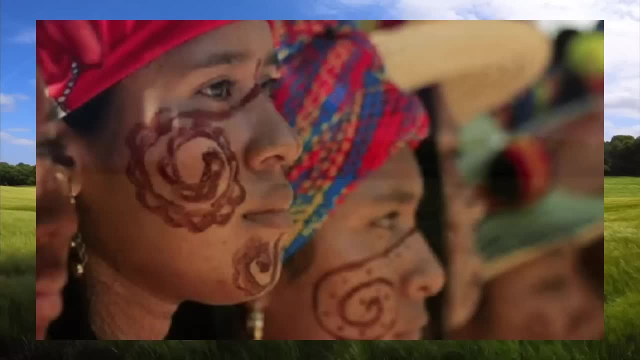 Muisca. The Muisca civilization thriving in the Colombian Andes left an enduring legacy of cultural and artistic richness. The elevated plateau served as the heartland of the Muisca, where they displayed their remarkable skills in agriculture and terracing The 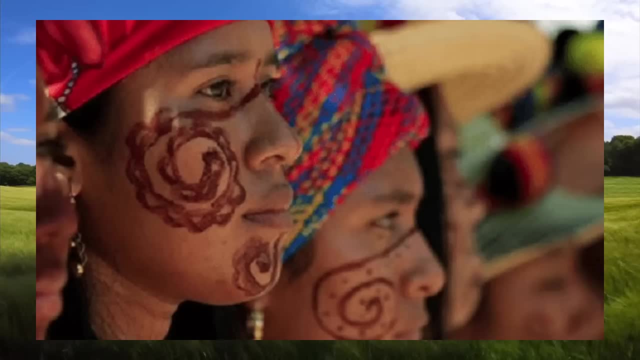 cultivation of maize potatoes and quinoa attested to their advanced agricultural practices in the challenging, monotonous terrain. One of the defining features of the Muisca civilization was their exquisite gold working. The Muisca were masterful goldsmiths, creating intricate 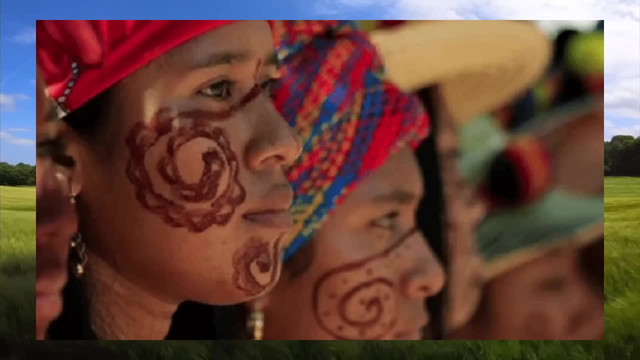 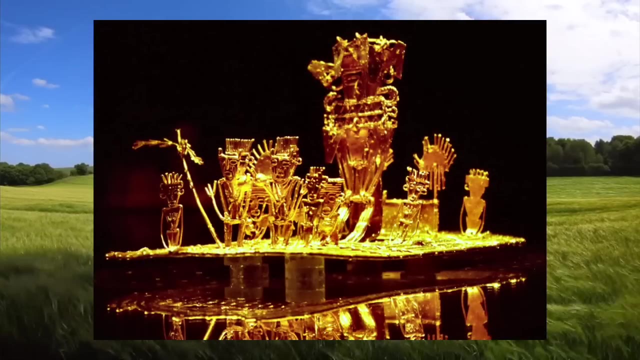 artifacts using tumbacá, a distinct greenish gold alloy. Notable among their creations were tunjos, gold votive offerings and detailed figurines. This gold working tradition contributed to the allure of Muisca culture, capturing the attention of later explorers and historians. 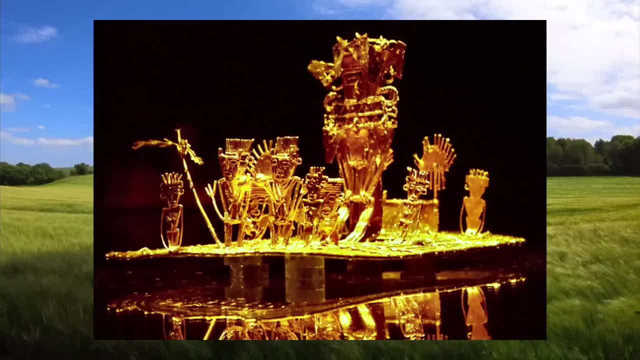 Lake Gatava holds a central place in Muisca culture linked to the legendary El Dorado ritual. According to Spanish accounts, the Zipa, covered himself in gold dust and accompanied by precious offerings, participated in a ritual on the lake. This legend became intertwined with 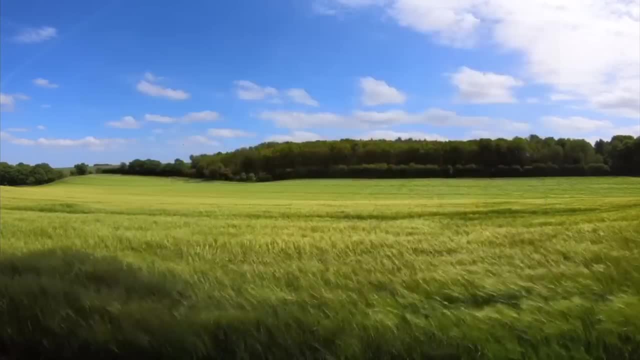 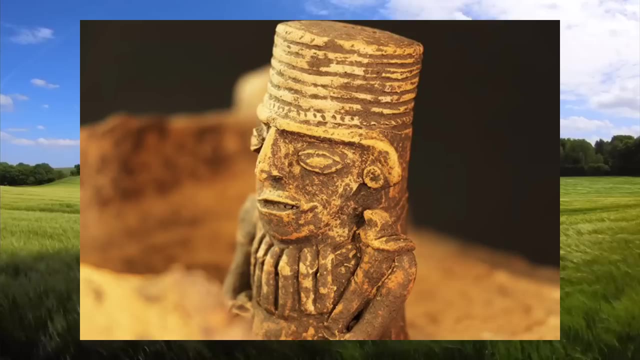 the broader myth of El Dorado, The fabled city of gold sought by European explorers. the Muisca society was organized into chiefs which led by a chief, or Zipa. Social hierarchy also played a role in the community, with distinct classes and roles assigned based on birth and achievements. The arrival of Spanish conquistadors, notably Gonzalo de Quesada, marked the downfall of the Muisca civilization in the mid-16th century, leading to colonization and significant cultural changes in the region. Despite the impact, 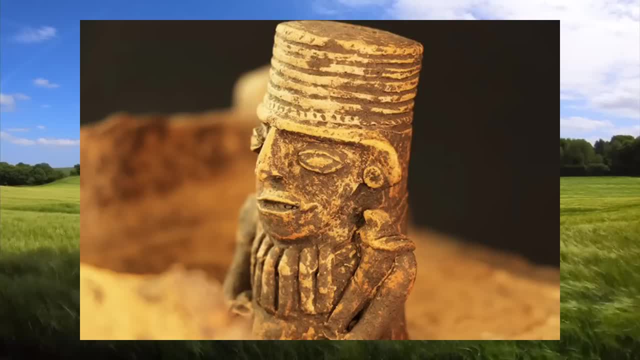 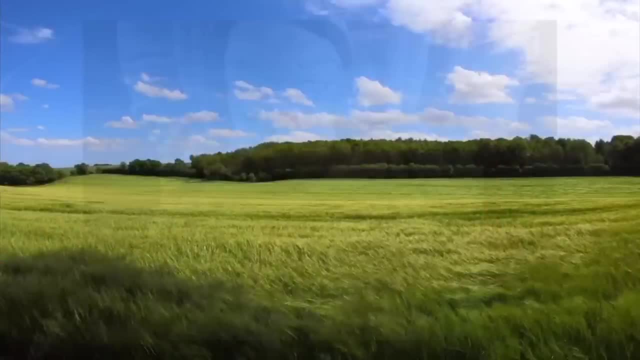 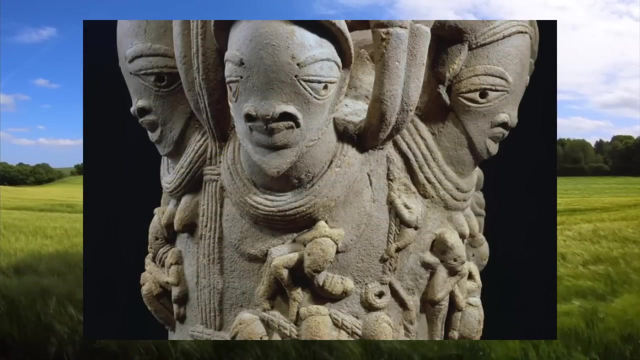 of colonization. elements of Muisca culture persisted in the cultural memory of Colombia today. Nok, The Nok culture flourishing in central Nigeria from around 1500 BCE to 200 CE stands as a testament to the early sophistication of African civilizations: The discovery of Terkada sculptures. 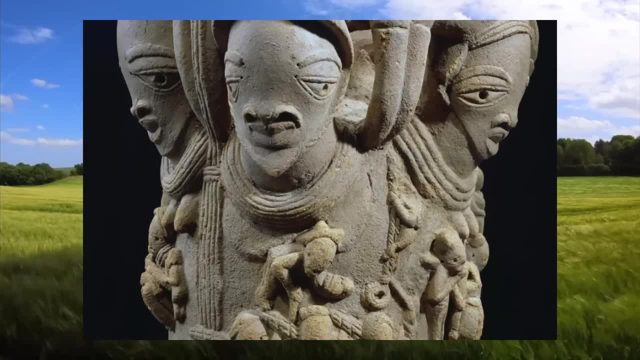 in the village of Nok in 1928 unveiled an extraordinary artistic tradition, with these sculptures, recognized as some of the earliest examples of figurative art in sub-Saharan Africa. crafted using the coiling method, Nok Terkadas portray human figures adorned with intricate hairstyles. 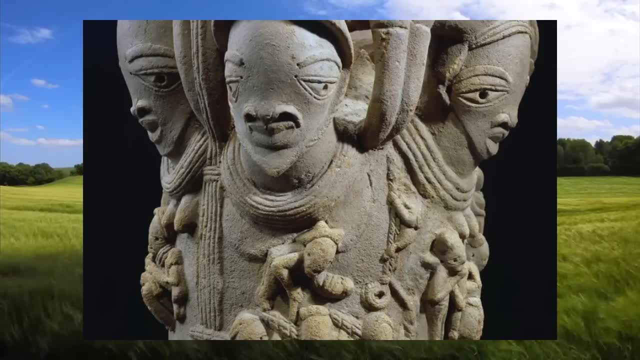 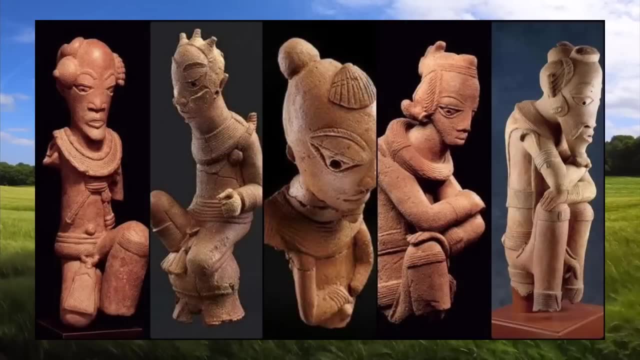 clothing and accessories, showcasing a remarkable level of artistic skill and attention to detail. Beyond their artistic prowess, the Nok people were engaged in ironworking and agriculture. They demonstrated proficiency in metallurgy, producing iron tools and artifacts, and actively participated in agriculture, cultivating crops such as malay and sorghum. 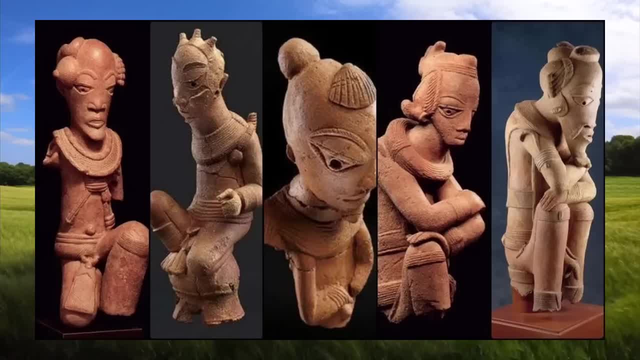 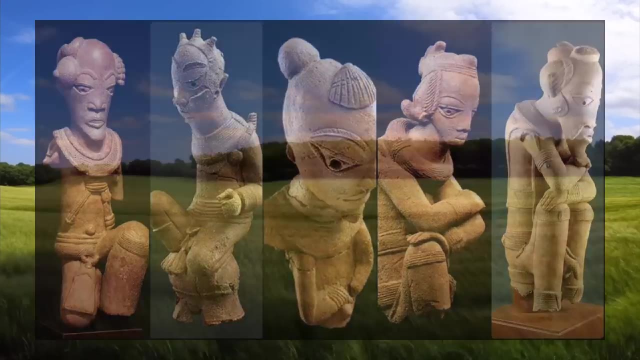 These activities suggest a complex society with a developed economic and technological foundation. The Nok Terkadas provide insights into the social complexity of the culture, hinting at a hierarchical social structure and potentially ceremonial or ritualistic practices. The figures depicted in the sculptures offer glimpses into aspects of their daily life. 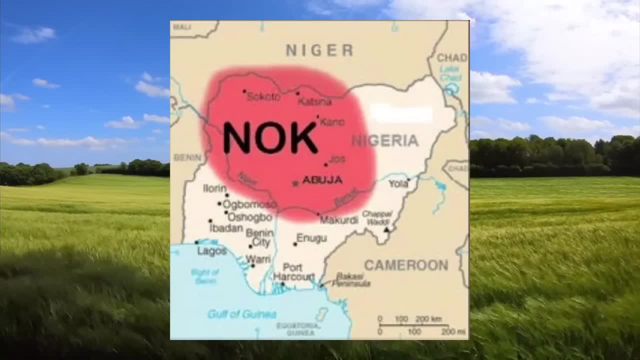 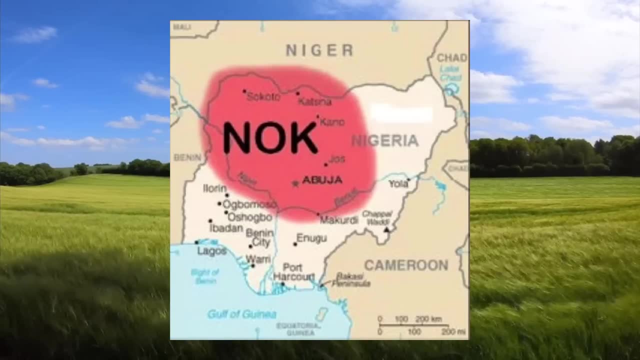 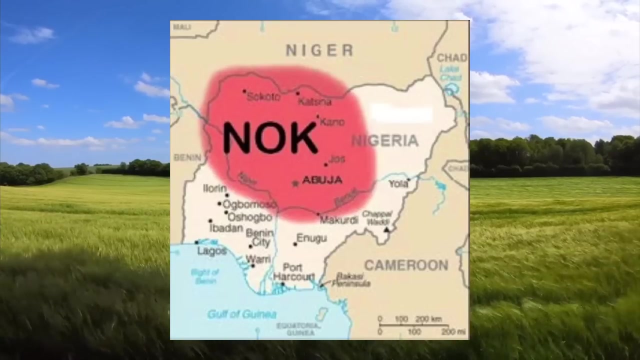 their religious beliefs and the possibility of the existence of cultural ceremonies. Despite their cultural achievements, the Nok culture experienced a mysterious decline around 200 CE, and the factors contributing to the decline remain the subject of ongoing scholarly inquiry: Environmental changes, economic shifts and internal dynamics within society. 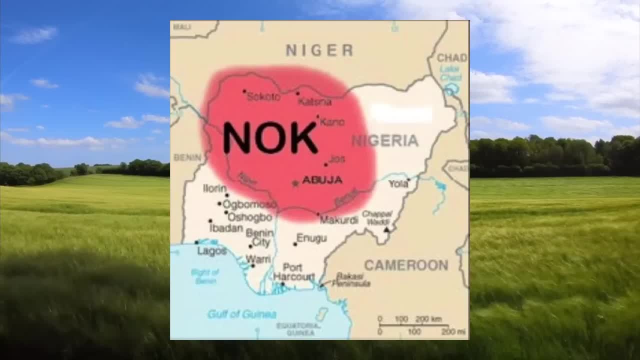 could have all played roles in the enigmatic transition. The significance of the Nok culture extends beyond just the temporal existence. The discovery of the Terkada sculptures challenged previous misconceptions about the absence of complex societies and sophisticated art in ancient West Africa. 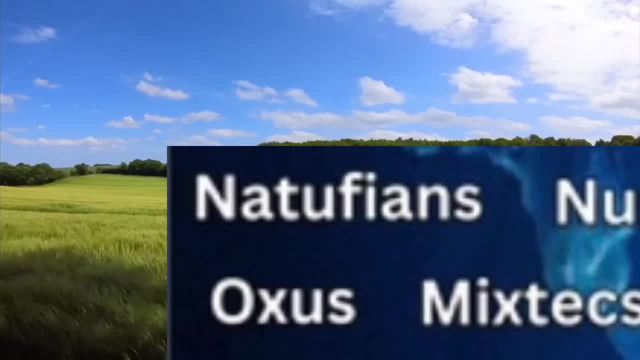 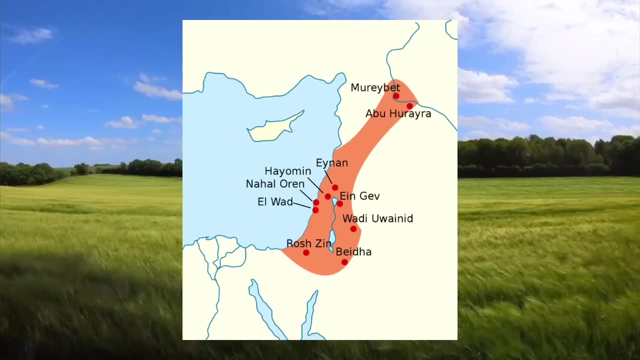 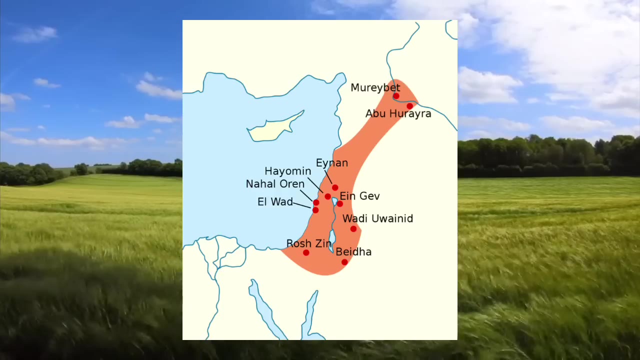 Tier 5. Natufians: The Natufian culture flourishing in the Levant region from around 12,000 to 9,500 BCE during the late Epiphy VER, holding a pivotal place in the transition from nomadic hunter-gatherer societies to more settled communities. 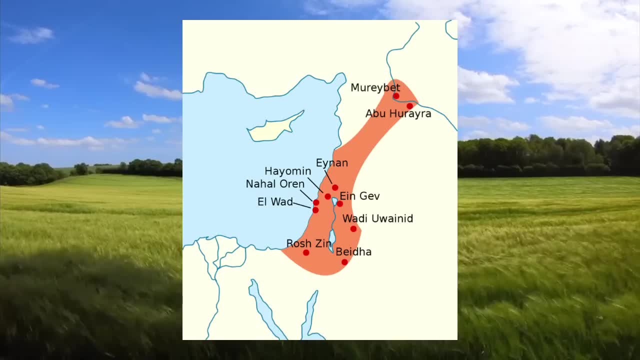 Natufian settlements, characterized by semi-permanent houses with stone foundations, showcased an early shift towards a more sedentary lifestyle. As skilled hunter-gatherers, the Natufians employed diverse substance and strategies. They hunted wild game, notably gazelles, and engaged in the work of hunting anduevas. 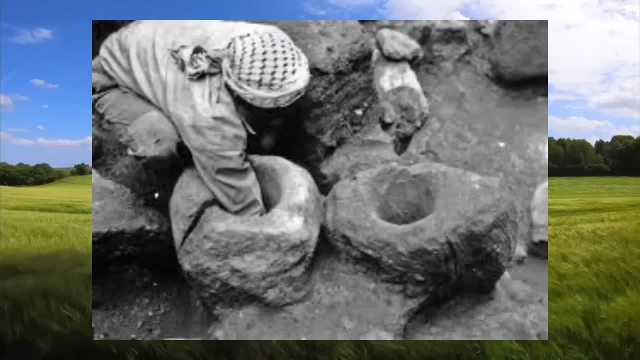 engaged in the harvesting of wild cereals. Evidence of sickles made from stones suggests early experimentation with plant cultivation, Hinting at the inceptive stages of agriculture. Natufian mortuary practices reflect the level of social organization and symbolic behavior. Elaborate burials with grave goods, including items like shells and okra, provide insights. 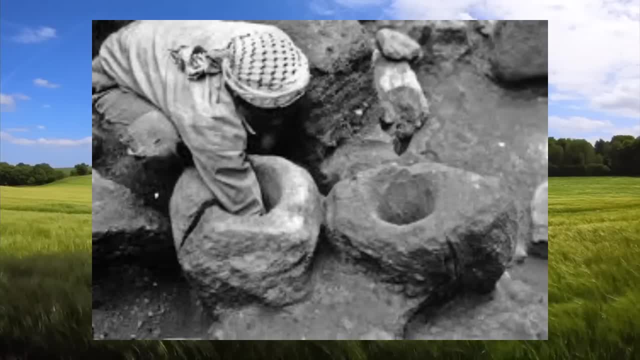 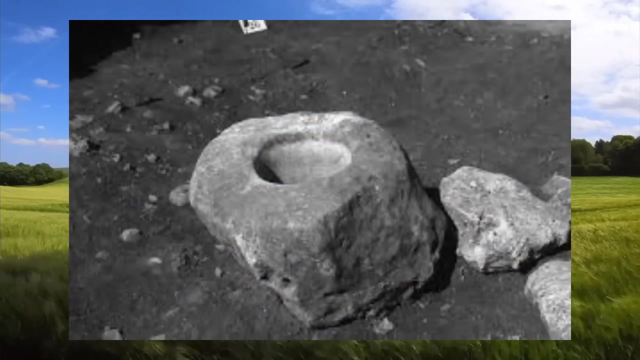 into their cultural and spiritual practices. Some burials feature the deceased in flexed positions, contributing to our understanding of their burial rituals. The Natufians crafted a variety of different tools and artifacts, including stone implements, grinding stones, bone tools and artistic items such as figurines and carvings. 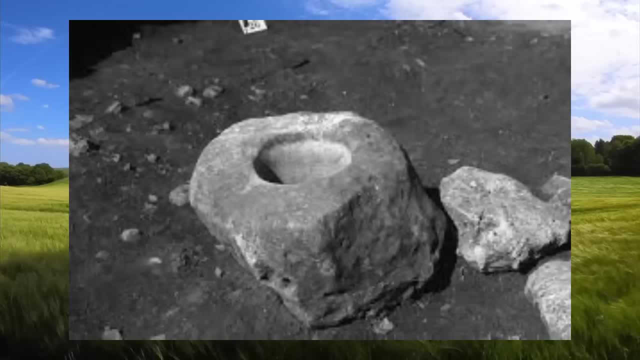 The archaeological site of Jureko, a prominent Natufian settlement, stands as a testament to their habitation and marks one of the earliest instances of continuous human settlement. Noteworthy for its transitional role, the Natufian culture foreshadowed the advent of 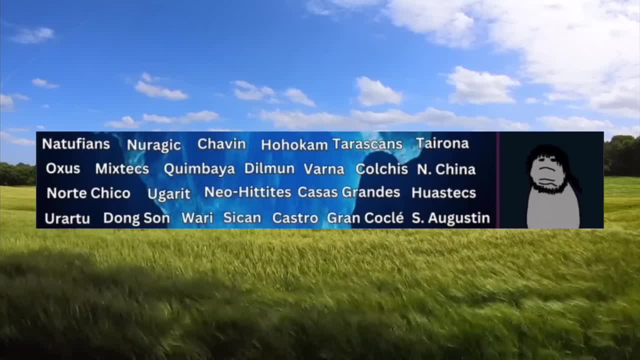 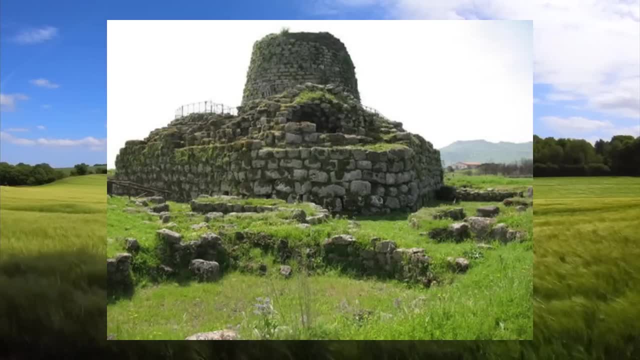 agriculture. Nuragic. The Nuragic civilization flourishing on the island of Sardinia from around 1800 BCE to 238 BCE during the Bronze Age, left a mark on its distinctive nuragy. These massive stone towers, constructed with rough honed blocks, are the hallmark of Nuragic. 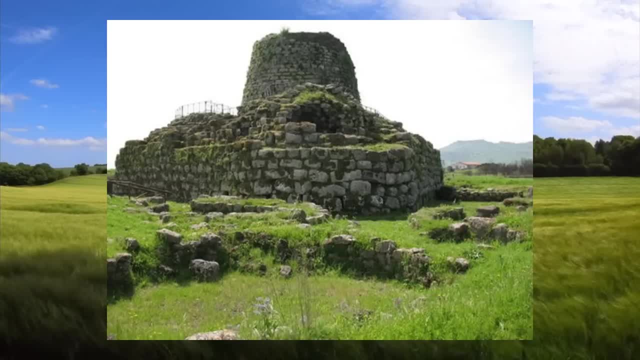 architecture Serving various different purposes, including defense, religious practices and symbols of political power. nuragy showcased advanced engineering skills and the ability to create a new world. The Nuragic civilization flourishing on the island of Sardinia from around 1800 BCE to. 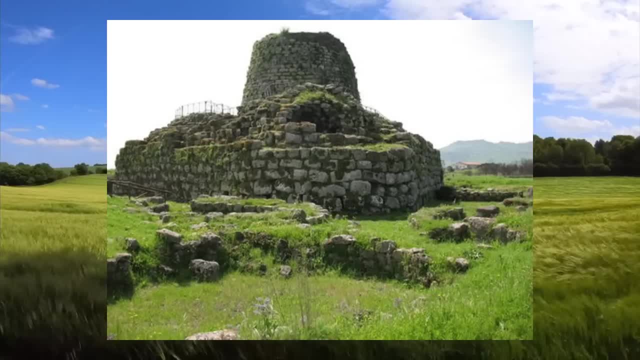 238 BCE left a mark on its distinctive nuragy Serving various different purposes, including defense, religious practices and symbols of political power. nuragy showcased advanced engineering skills and a sophisticated understanding of different construction techniques. The complexity of Nuragic architecture extends beyond just the nuragy encompassing megalith. circles, villages and sacred wells. This diversity reflects a developed society with hierarchical structures. The economic foundation rested on agriculture, pastoralism and trade. Notably the Nuragic people excelled in metalworking, producing intricate bronze artifacts, weapons. 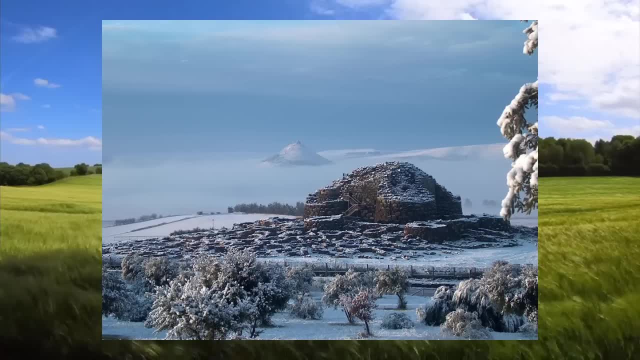 and statuettes known as bronzete. The Nuragic civilization flourishing on the island of Sardinia from around 1800 BCE to 238 BCE left a mark on its distinctive cultural and religious beliefs. Trade and cultural exchanges played a significant role in Nuragic society. 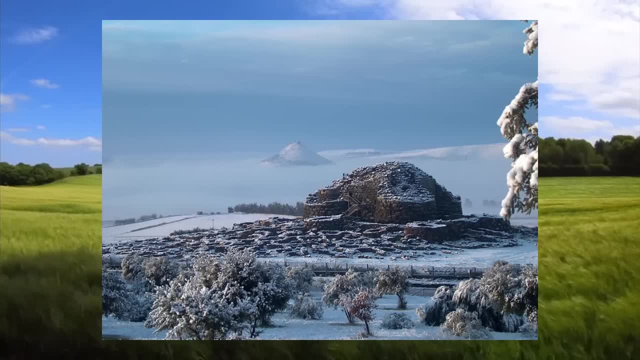 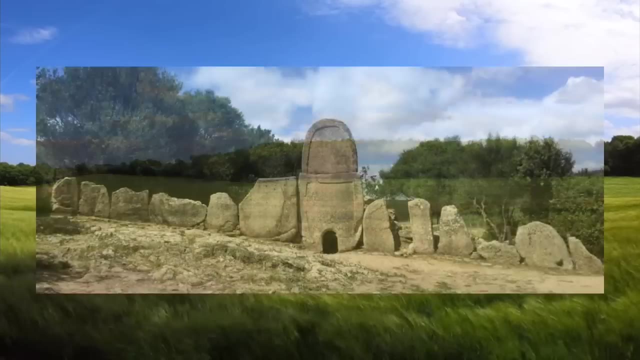 The strategic location of Sardinia facilitated maritime trade routes connecting the Nuragic people with Mediterranean cultures such as the Mycenaeans and the Phoistians. This interaction enriched the cultural landscape and influenced the development of the Nuragic civilization. The decline of the Nuragic civilization around the time of the Roman Republic's expanding 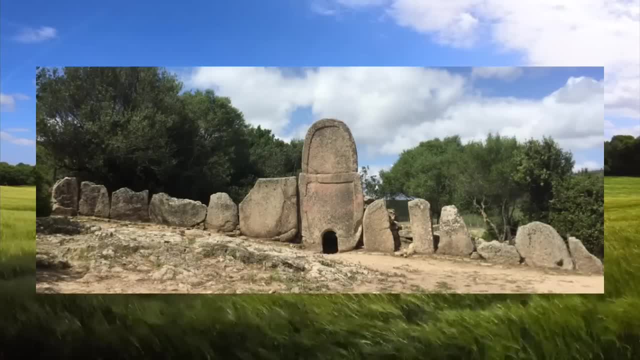 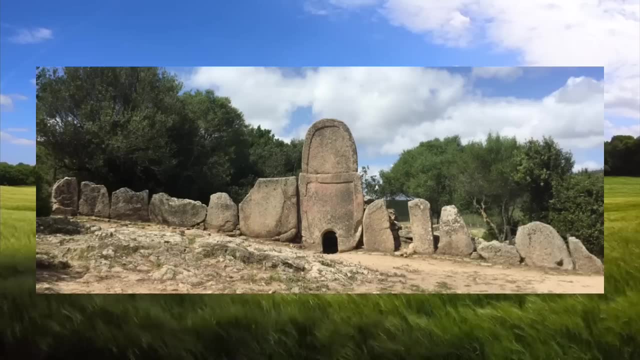 influence into the Mediterranean remained somewhat mysterious. This is not to say that the Nuragic civilization is inferior, as environmental changes, internal conflicts and external pressures like the Roman Empire may have contributed to its decline. Nevertheless, the enduring legacy of the Nuragic civilization is evident in the Nuragi and. 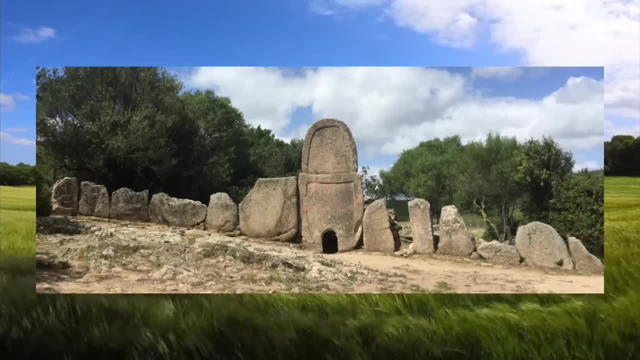 other archaeological remnants scattered across Sardinia. Today, Nuragis stand as iconic symbols of Sardinia's ancient history, capturing the fascination of scholars, archaeologists and visitors alike. The Nuragic civilization, with its unique architectural achievements and cultural complexities. 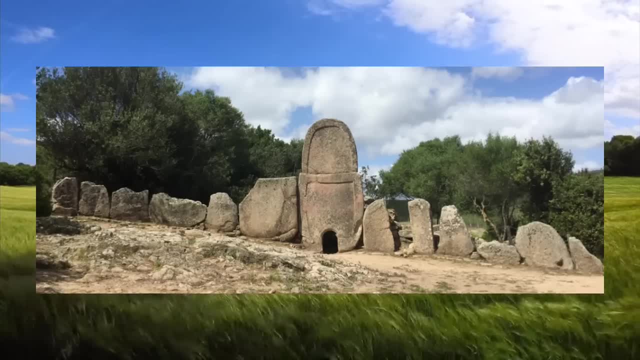 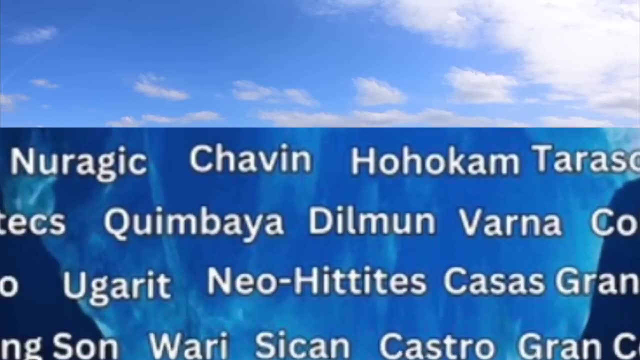 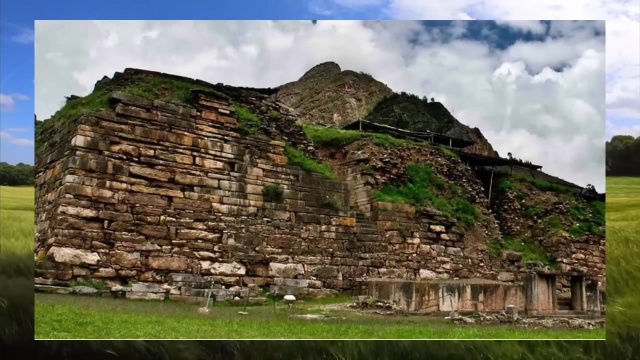 contributes significantly to the broader understanding of Mediterranean prehistory and remains an integral part of Sardinia's rich cultural heritage. Chavin, The Chavin civilization, flourishing in the Andean highlands of Peru from approximately 900 BCE to 200 BCE, left a mark on the cultural 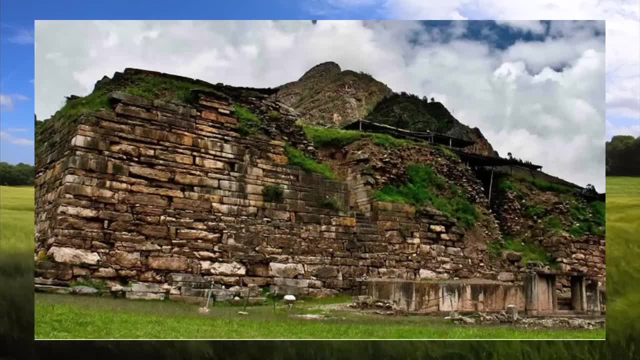 and religious landscape of the Peruvian region. At the heart of the Chavin culture stood the monumental complex of Chavin de Juntar, an elevated ceremonial center Surrounded by pyramidal structures and plazas. the iconic Lanzum, a carved stone monolith. 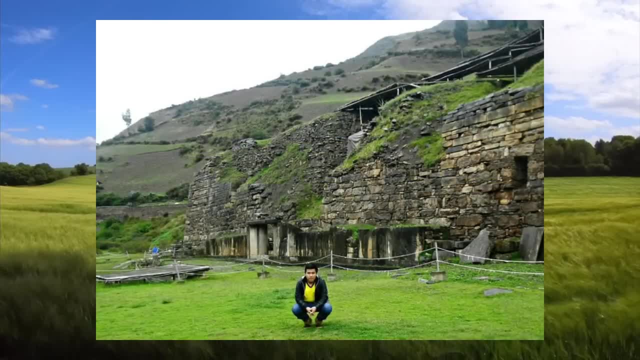 with underground galleries, served as a focal point for Chavin religious practices, representing a powerful supernatural deity. Chavin art is renowned for its symbolic and intricate iconography, expressed in various different medias, such as ceramics, textiles and different carvings. 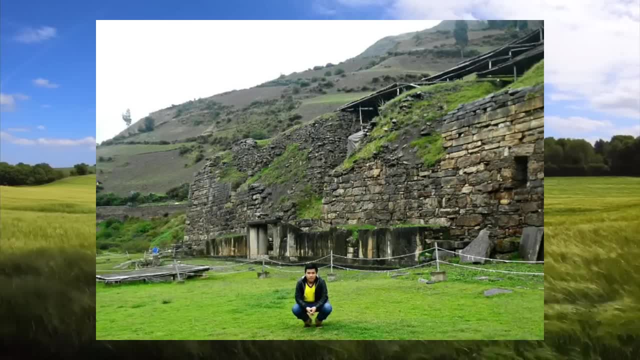 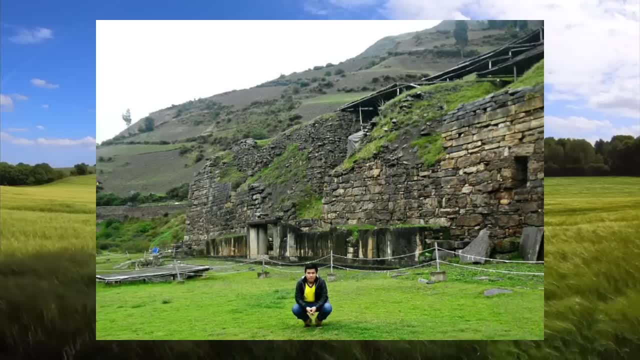 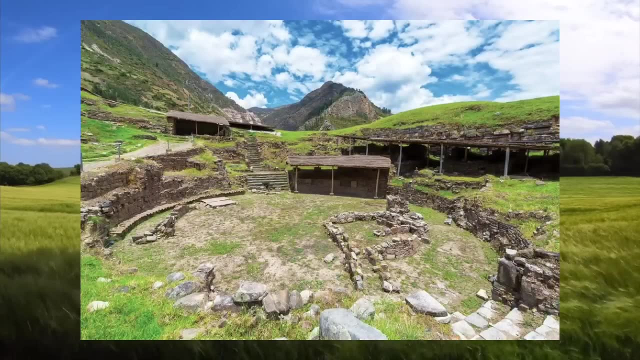 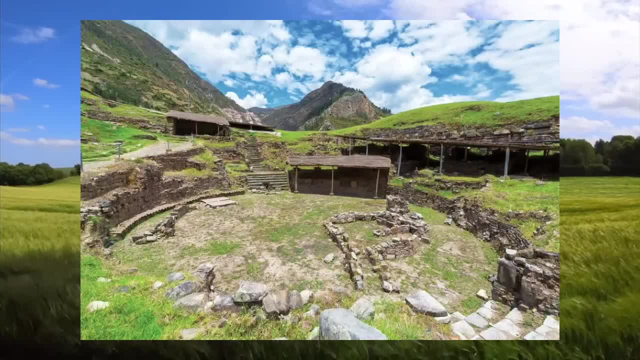 activities. the Chavin people engaged in a complex religious practice that influenced subsequent Andean cultures, leaving a lasting legacy in the region's artistic and different spiritual traditions. The Chavin economy was grounded in agriculture, cultivating staples like maize beans and potatoes. 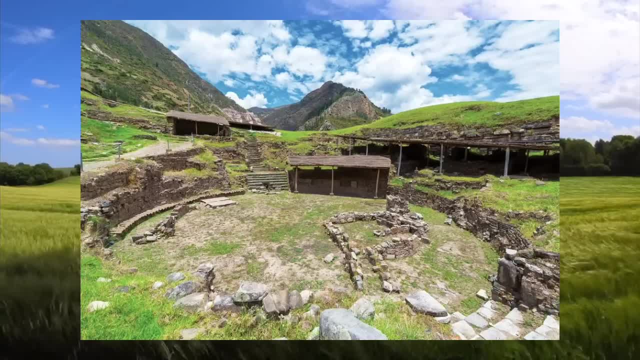 Additionally, evidence of trade indicate a primer that there, from and around the metallurgy past simply憓 up the knick-packs of these式 środküst, attacking women in the Diez. The presence of non-local materials such as marine shells highlights the Chauvin's intercontentiousness. 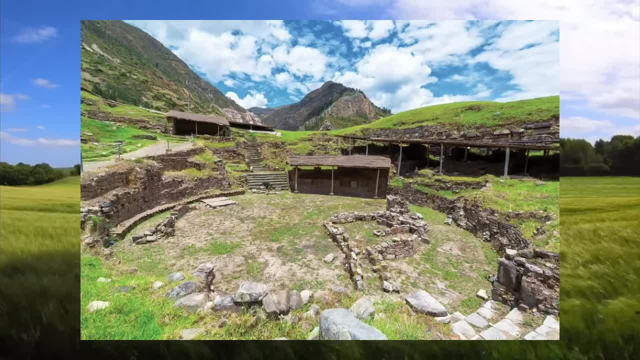 with other cultures and their willingness to trade with other cultures and civilizations in the region. While the reasons for the decline of the Chauvin civilization remain unclear and unknown, factors such as environmental changes, social transformations or the emergence of rival cultures may have. 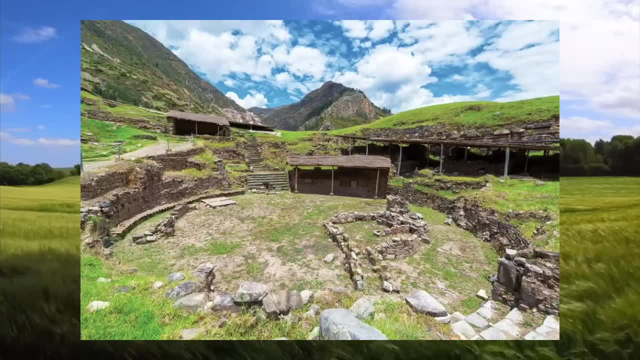 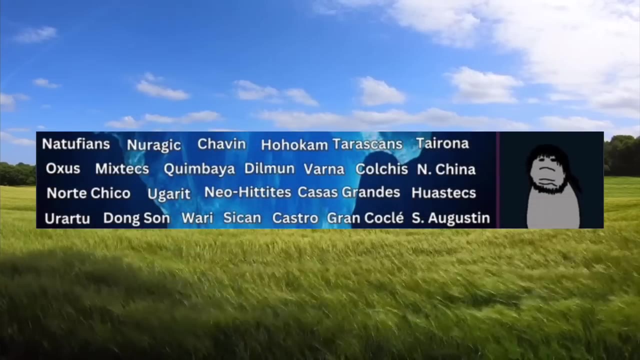 contributed to its waning influence. Nevertheless, the Chauvin culture played a pivotal role in shaping the trajectory of the Andean civilizations, influencing artistic styles and religious practices in subsequent cultures like the Paracas and the Nazca. The Hohokam, an ancient Native American culture, left a mark on the Sonoran Desert. 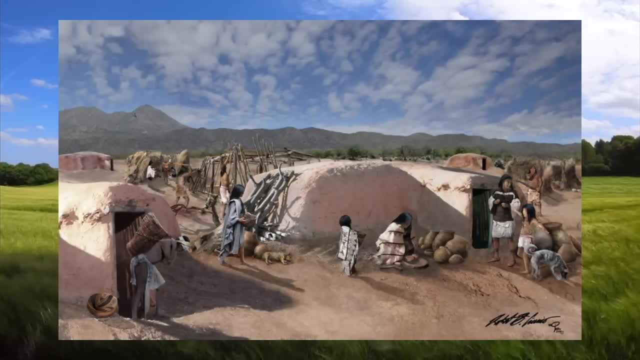 area in what is now Arizona. With their civilization flourishing from around 200 CE to 1450 CE, their unique adaptation to the arid environment was characterized by advanced irrigation systems that enabled them to cultivate their own crops. The Hohokam constructed an extensive network of canals diverting water from the Gila and 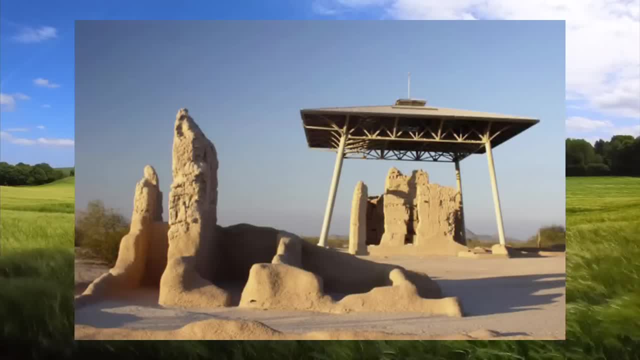 the Salt Rivers to nourish their fields and support the growth of maize beans, squash and cotton. The landscape of Hohokam settlements featured platform mounds built from caliche and soil, serving multiple different purposes, such as providing elevated spaces for restructures. 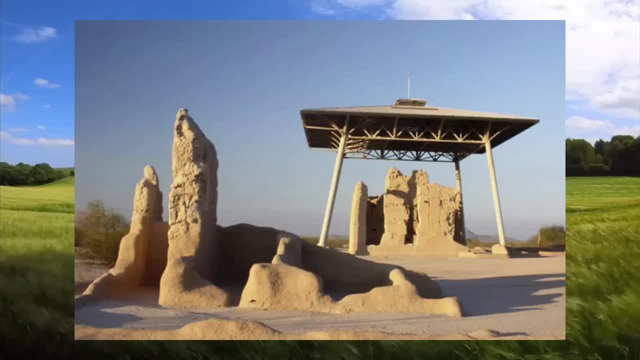 ceremonial activities and refuge from potential floods. The craftsmanship of the Hohokam is evident in their pottery. Regularly, the red on buff wear adorned with intricate geometric designs. These artifacts, along with shell jewelry and other items, showcase the artistic skills. 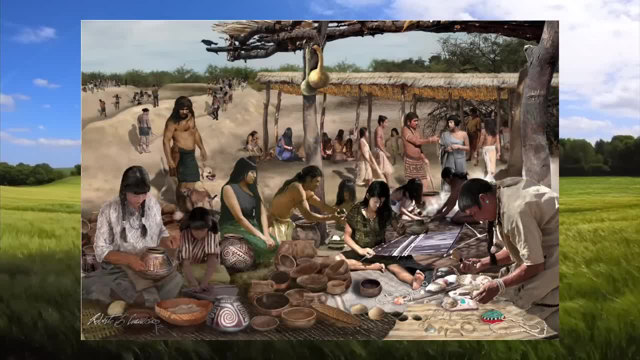 of the Hohokam people. Hohokam communities also engaged in regional trade networks, engaging goods and exchanging goods with neighboring cultures like the Mongola and the ancestral Puebloans. These facilitated the acquisition of materials such as seashells and turquoise, highlighting 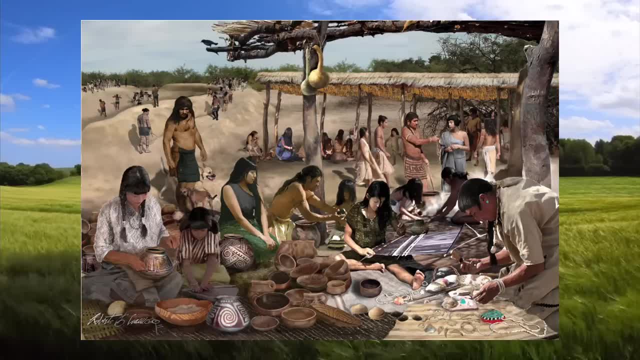 the interconnectedness of pre-Columbian societies in the American Southwest. The construction of ball courts in some Hohokam communities adds a layer of mystery to their cultural practices. and what purpose these ball courts and the rules of the associated ball game remain subjects of scholarly inquiry which people don't know what they even used. 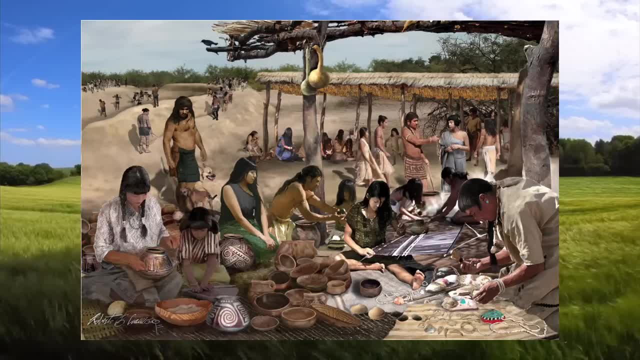 the ball courts were used for or what sports they used to play with. The decline of the Hohokam civilization around the mid-15th century is a complex phenomenon. Factors contributing to their decline include environmental changes, resource depletion and social dynamics. 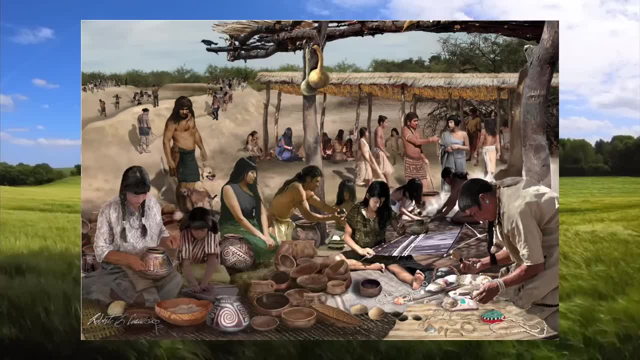 The once-thriving canal systems fell into disrepair. The Hohokam community is now a part of the Hohokam community. Its population is dispersed, leaving behind a legacy of innovation in desert adaptation and a rich archaeological record that continues to provide valuable insights into the complexities. 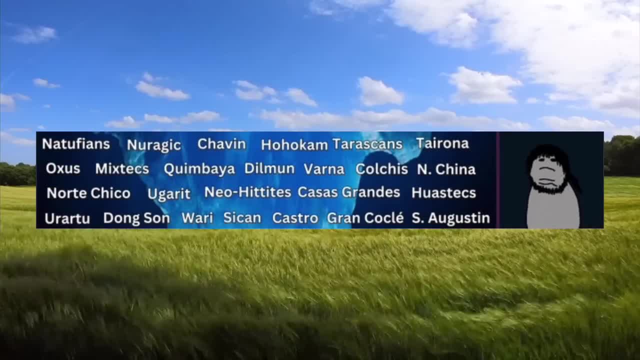 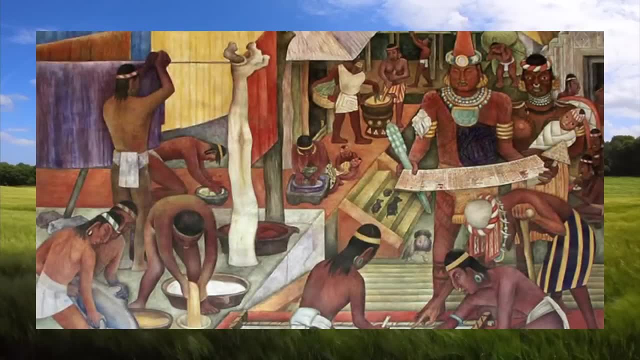 of prehistoric southwestern cultures Tarrasquins. The Tarrasquins, also known as the Purapecha, were a remarkable indigenous civilization that flourished in western Mexico during the late post-Classic Period spanning the 14th to early 16th centuries. 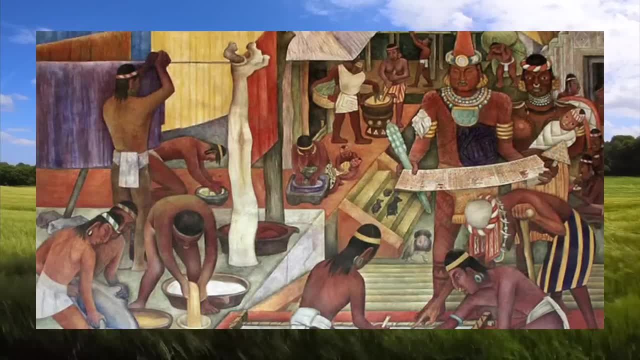 Their capital city, Tizioquito, was in fact, Tijucan, a document that dates back to the fall of the El Tijucan Conquest of the Spanish Revolution. Tuscan, situated on the shores of Lake Pasecuaro, served as the political, economic and religious 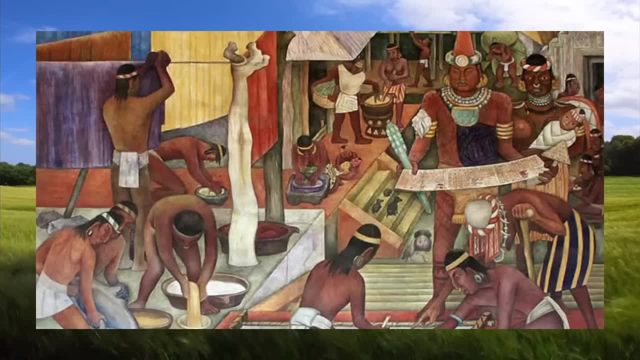 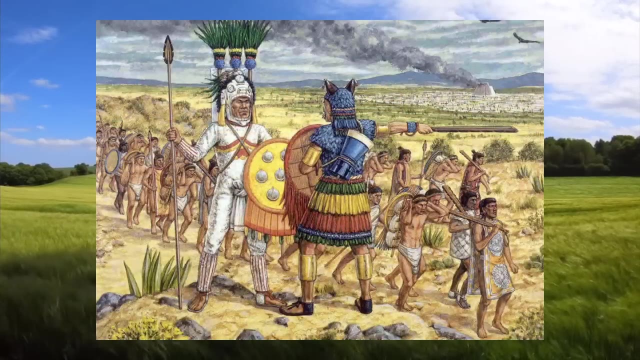 hub for the Tarascon realm. Despite their territorial ambitions of the Aztec Empire, the Tarascans displayed notable resistance and maintained their independence. Agriculture played a pivotal role in the Tarascan economy, with innovative techniques such as raised fields and terraced farming employed to maximize productivity in the hilly terrain. The Tarascans 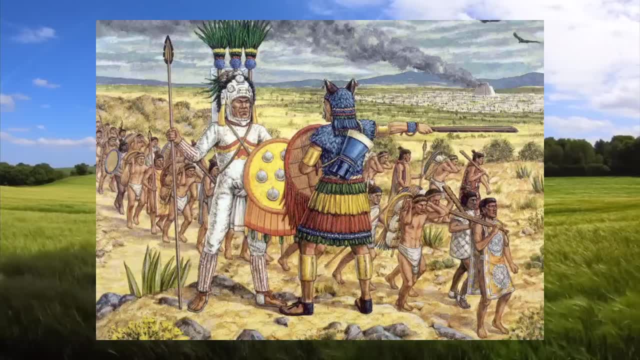 were skilled artisans renowned for their distinctive Maokun-style pottery and intricate metallurgy, producing copper and bronze objects ranging from tools to ornamental items. The Tarascan political structure featured a centralized authority led by the Khazadzi, the ruling king. 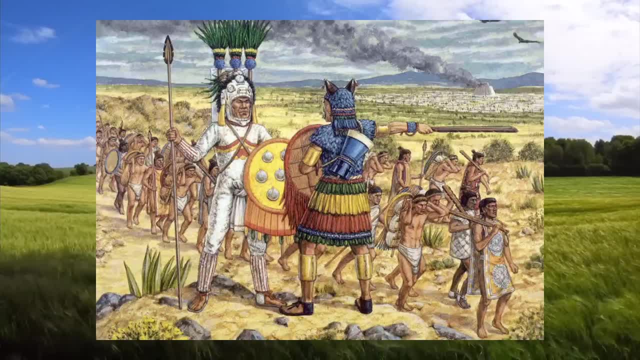 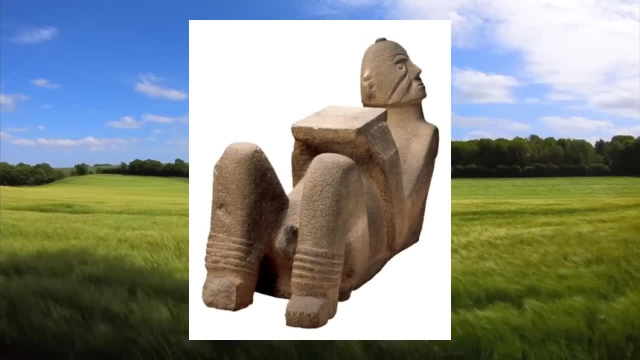 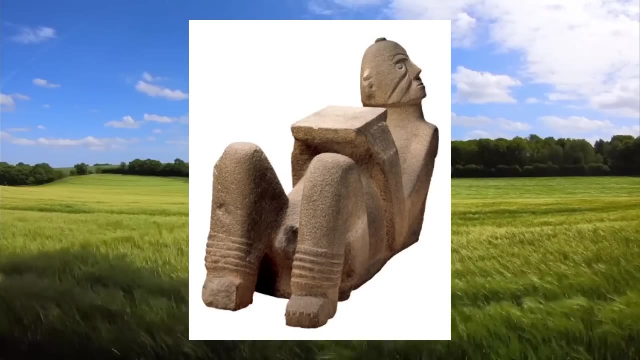 Their religious beliefs were polytheistic, involving different ceremonies, rituals and the variation of various different deities. Temples and ceremonial centers were integral to their urban architecture, reflecting the spiritual significance embedded in their society. Lake Pasecuaro held cultural and religious importance for the Tarascans with islands. like Jantizo, serving as venues for the ceremonial activities, including the observance of the Day of the Dead. However, the arrival of Spanish conquistadors, notably Hernán Cortés, marked a turning point in Tarascan history. Despite their initial resistance, the Tarascans succumbed to. 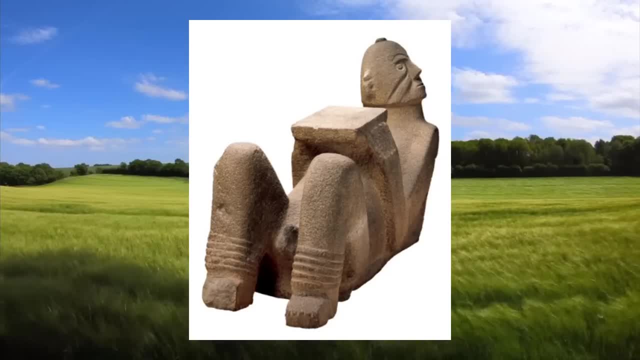 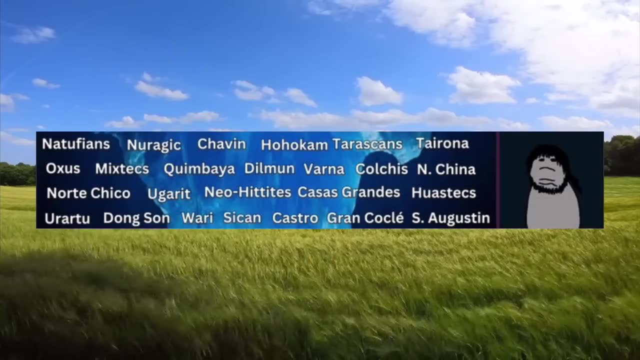 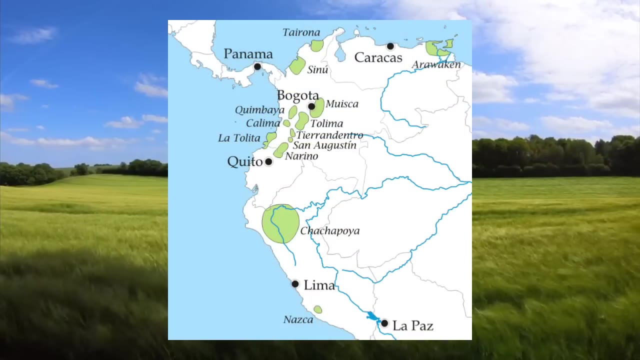 the devastating impact of European diseases and military conflicts, leading to the decline of civilization and the end of the Tarascans Tyrona. The Tyrona civilization flourishing in the northern coastal region of present-day Colombia from around 200 CE to 1600 CE represents a significant chapter in pre-Columbian history. 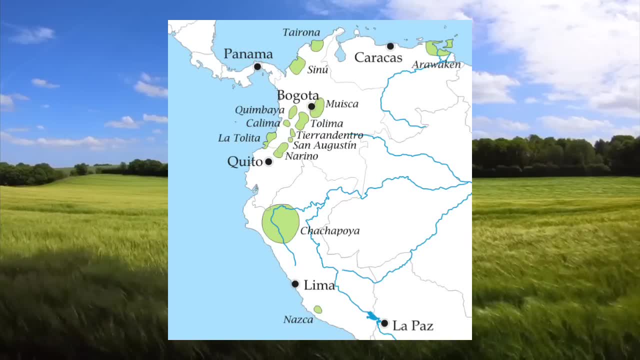 Thriving in diverse environments, from the Caribbean coast to the monotonous Sierra Nevada de Santa Marta, the Tyrona people showcased advanced agricultural practices. Terraced farming on steep slopes allowed them to cultivate stable crops like maize beans, squash and cassava. Tyrona was also known as the land of the Tarasque people. Tyrona was a 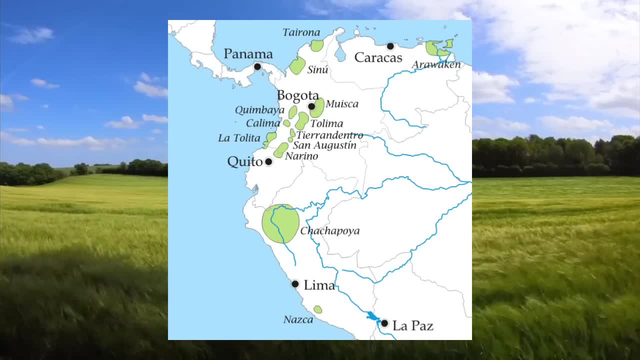 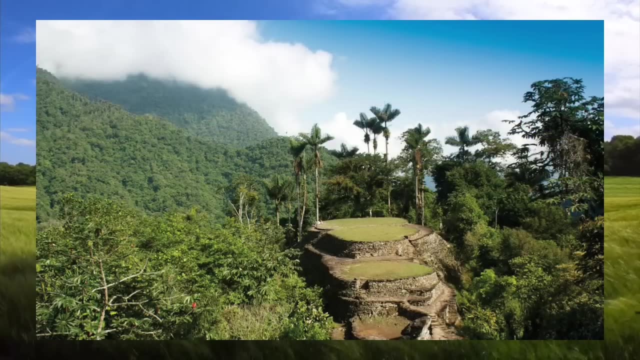 land of the Tarasque people. Tyrona settlements varied in size and location, with communities situated along rivers in the lowlands and others in the elevated highlands. Their architectural prowess is exemplified by the Ciudad Paredada, a monumental architectural site known for its 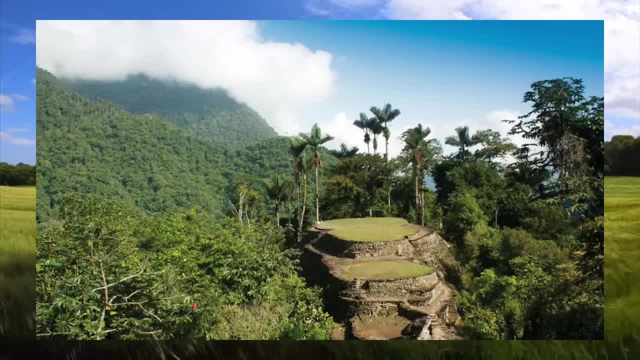 stone structures, terraces and retaining walls. This city, also called Tayuna, stands as one of the most largest pre-Columbian urban centers in all of South America. Gold played a significant role in Tyrona culture as well, and their exquisite gold work attests to their skill in. 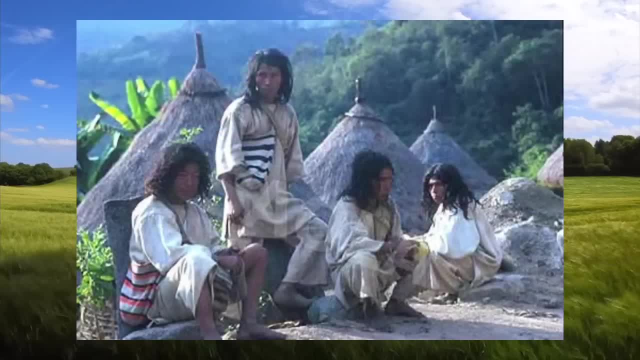 goldsmithing. The intricate gold artifacts produced by the Tyrona people not only demonstrated their craftsmanship, but also held cultural and symbolic importance within their society. The social organization of the Tyrona featured a complex structure with distinct, different roles for leaders, priests and common people. Chiefdoms likely governed different regions. 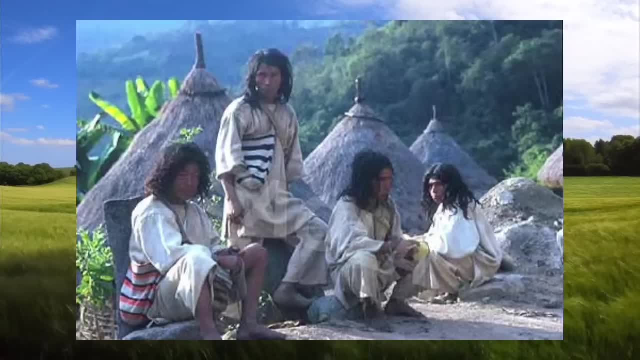 contributing to a well-organized society. However, the reasons behind the decline of the Tyrona civilization also remain a subject of scholarly inquiry, Encompassing environmental factors, the state of the Tyrona population and the economic明白 nature of this civilized. 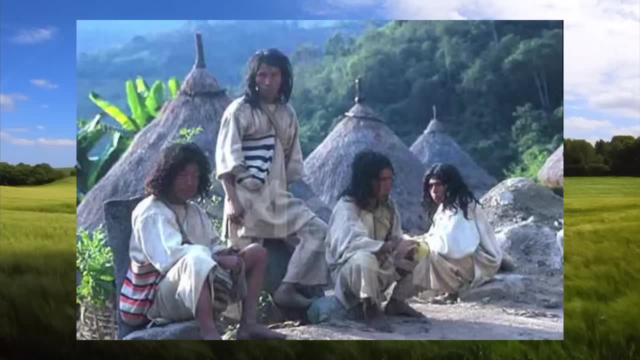 civilization influenced the development of the European civilization from the time of the Chaldeans, The dynamics and potential impacts of European contact in the late 15th century. And, if you haven't noticed already, European contact is really the decline of all of these different civilizations in all of South America. It just went to show how bad. 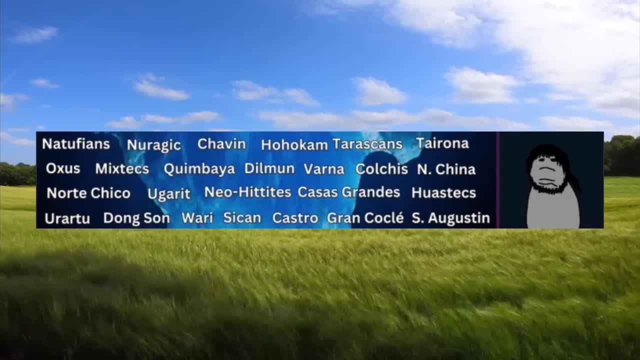 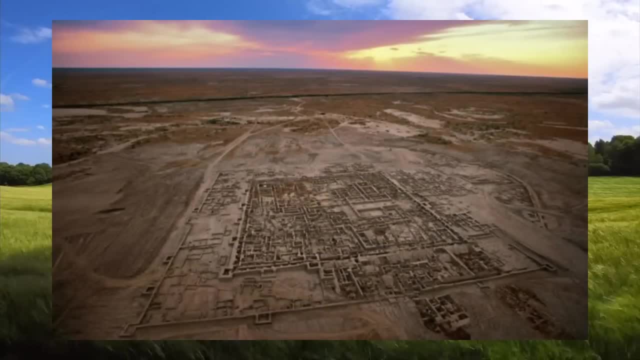 the Europeans just influenced all of South American societies because they were doing fine, until the Europeans showed up and just spread disease all over them. OXUS, The Oxy civilization flourished in from around 1700 BCE in Central Asia along the bates of the Oxus River, represented a distinctive Bronze Age. 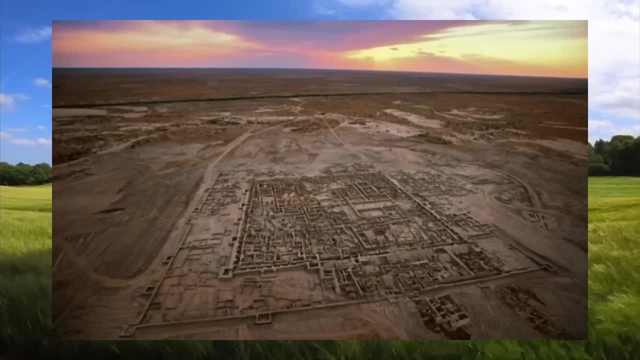 society, with notable urban centers such as Ganara Tepe, Tolagok and Namagaza Tepe. These settlements, characterized by advanced architectural planning, included monumental structures and residential areas that showcased the sophistication of the Oxus civilization. Agriculture played a pivotal 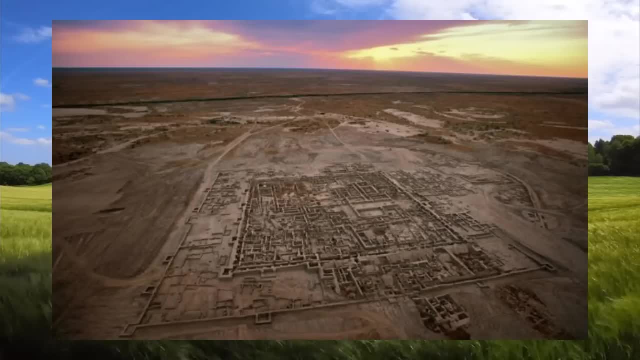 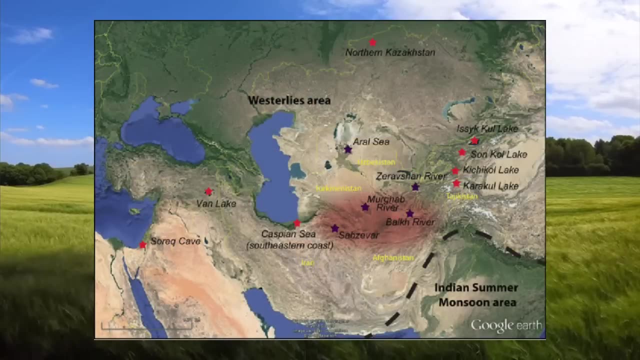 role in the Oxus way of life, with the cultivation of crops like wheat, barley and fruits. The people demonstrated ingenuity in adapting to the arid Central Asian environment by developing different advanced irrigation systems to enhance agricultural productivity. This ability to harness and manage 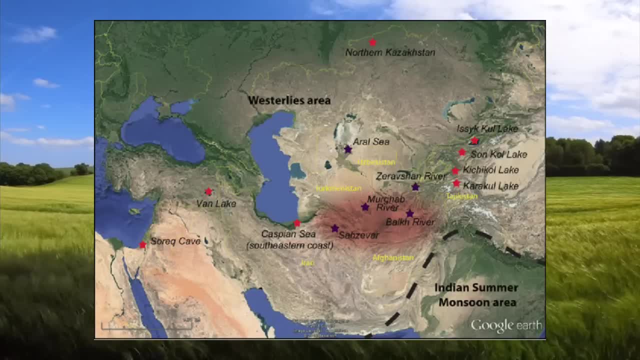 water resources reflected the civilization's resourcefulness. The Oxus civilization actively participated in different trade networks that reached neighboring regions, establishing connections with the Mesopotamian and the Indus Valley. Architectural findings, including distinctive pottery, metal objects and intricate seals, attest to cultural exchanges and trade interactions. 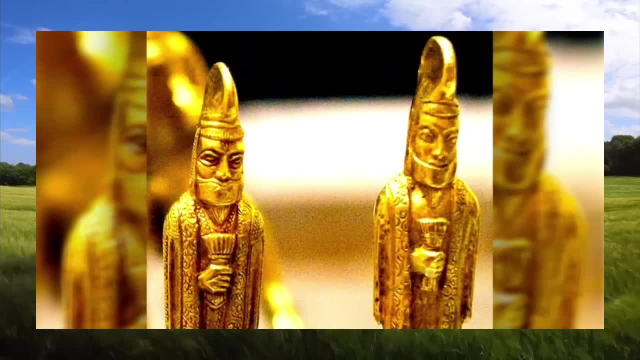 Contributing to the richness of the Oxus material culture. Despite the archaeological evidence of a well-organized society, the language spoken by the Oxus people remains undeciphered and unknown, and there is no indication of a writing system associated with their entire civilization. 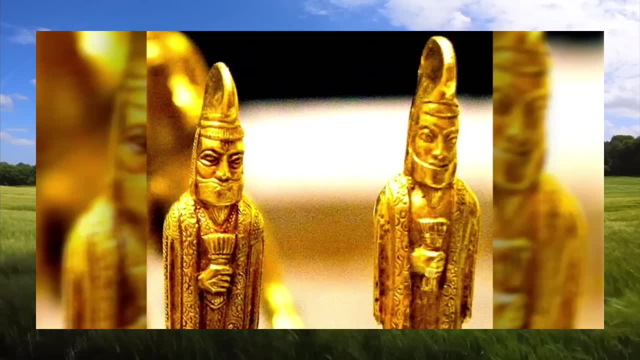 Consequently, much of our understanding of the Oxus society is derived from the excavation of their settlements and the artifacts they left behind, And other than that, in the decline of the Oxus civilization around 1700 BCE, remains shrouded in mystery and various different 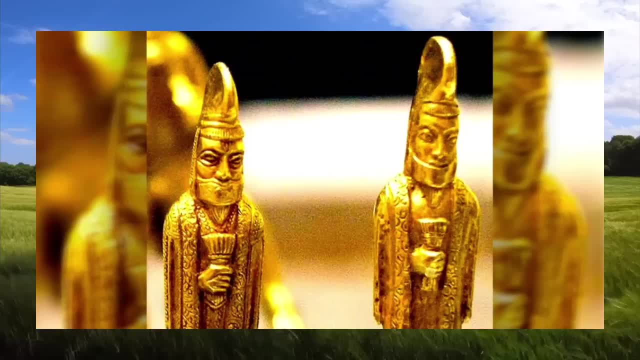 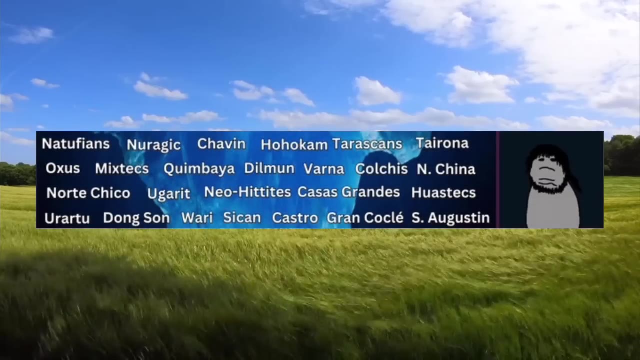 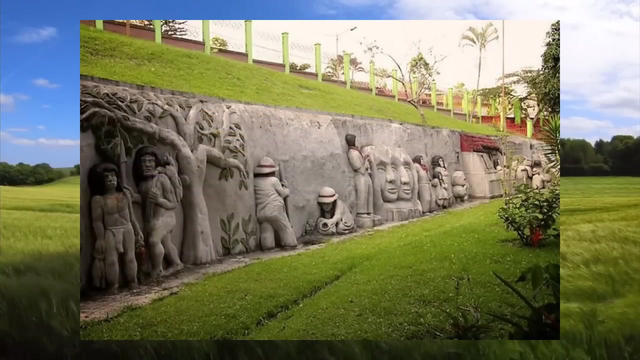 cultural結識和暁ty and the Konanistana Artifactology that have existed in the past In the history and earliest records of the Oxus, the Oxus, each of the worst-known of the age in the history of the Oxus. 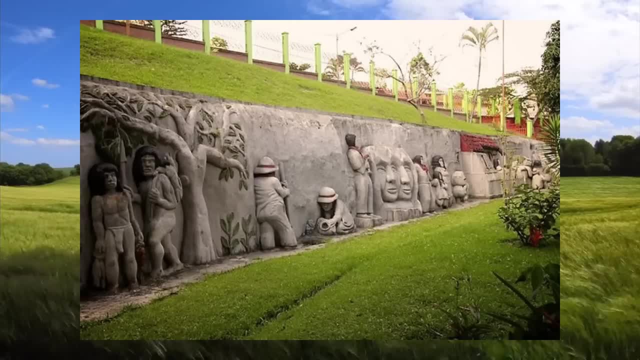 The Xerox250 was the first observation of the Oxus. The Oxus, in addition to the royal name of the Xerox, became the intended name of the Xerox, which is a later name for thex. RUSSIA, remarkable chapter in the pre-Columbian history. Situated in the Andean region, particularly the 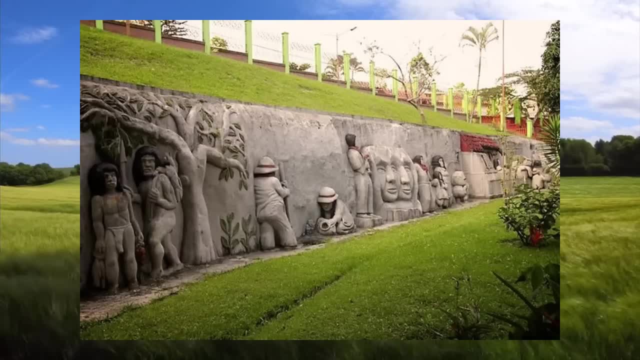 Cuaca River Valley. the Quimbaya people navigated diverse landscapes, including mountains and valleys. Their economy relied on agriculture, cultivating staples like maize beans, squash and yams in their fertile soils, employing terraced agriculture to adapt to the monotonous. 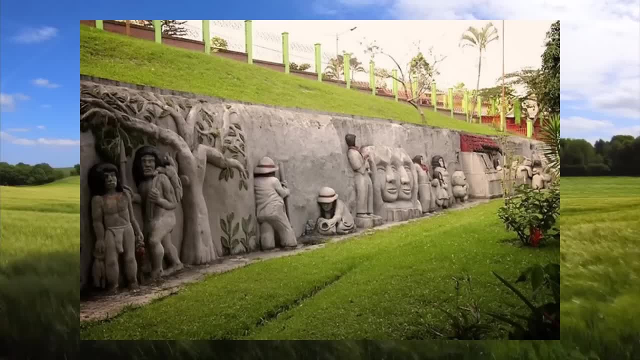 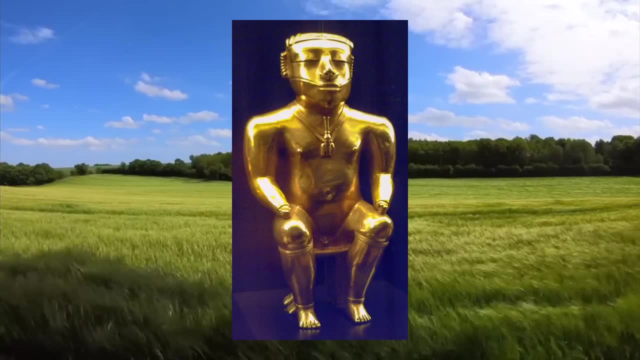 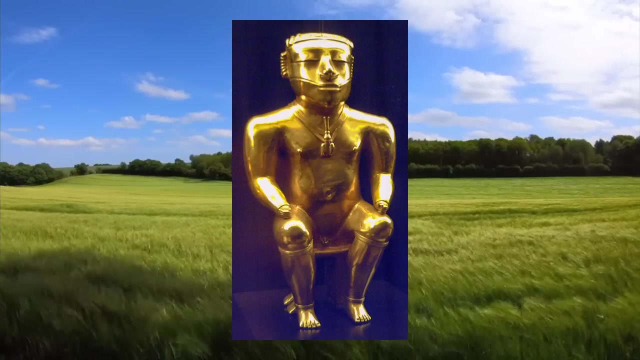 terrain. The Quimbaya are most renowned for their extraordinary skill in metallurgy, especially goldsmithing. Their intricate gold figurines and different artifacts, notably the iconic Quimbaya airplanes with winged features, attest to their remarkable precision and artistic sensibility. These golden creations have become iconic symbols of the 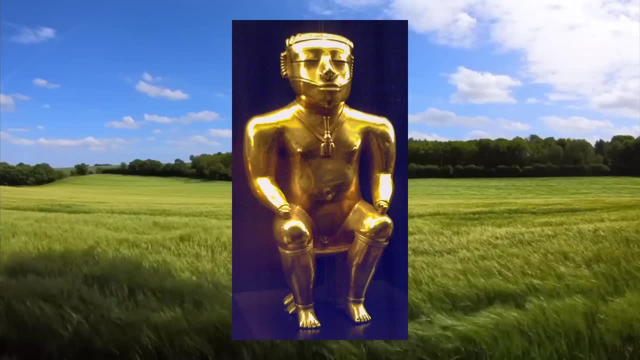 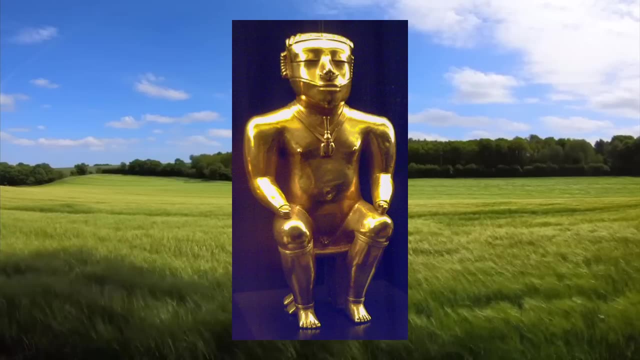 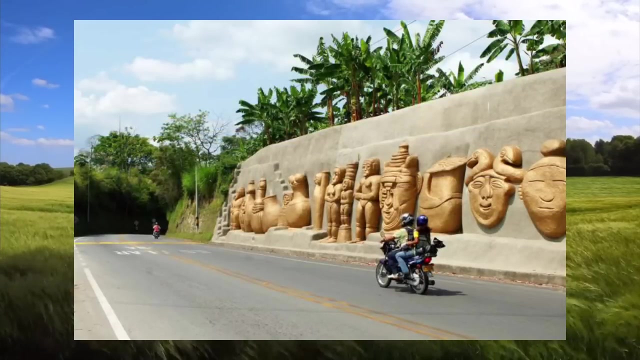 Quimbaya culture and showcase their mastery of metal craftsmanship. In addition to their gold work, the Quimbaya produce distinct pottery adorned with geometric patterns and stylized depictions of animals and human figurines. Their material culture, including ceramics and gold artifacts, reflects a keen artistic sensibility and an engagement with symbolism. The Quimbaya 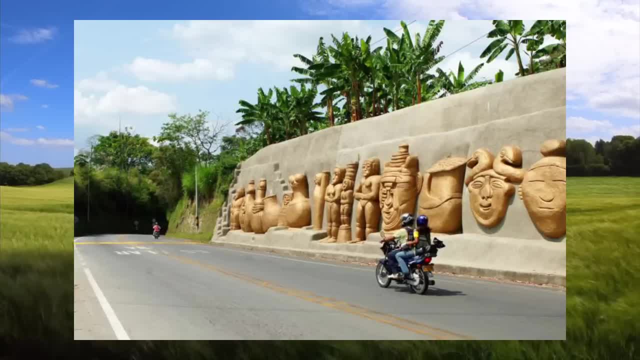 civilization is one of the most famous civilizations in the world. The Quimbaya civilization actively participated in trade networks, fostering exchange with neighboring cultures and contributing to the cultural diversity of the Andean region, While their social structure and religious practices are not extensively documented or known at all. 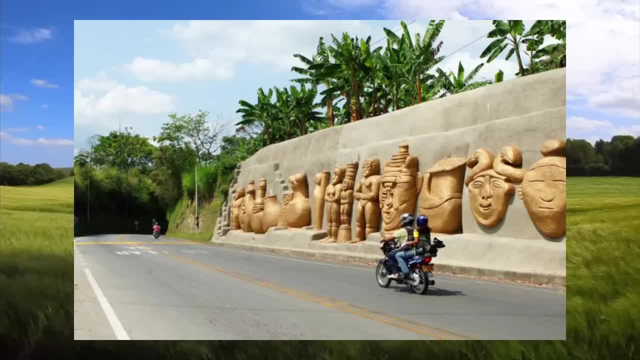 architectural and archaeological evidence suggests the presence of hierarchical elements and spiritual rituals. The arrival of Spanish clandestinators in the early 16th century brought significant changes to the Quimbaya civilization In the impacts of European diseases. once again, cultural shifts. 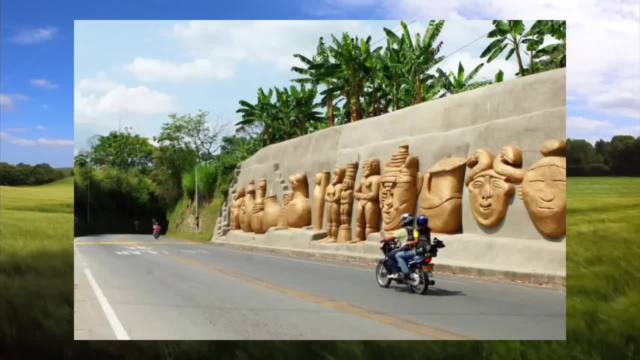 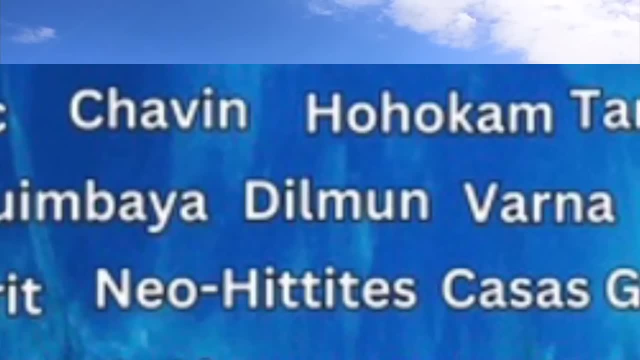 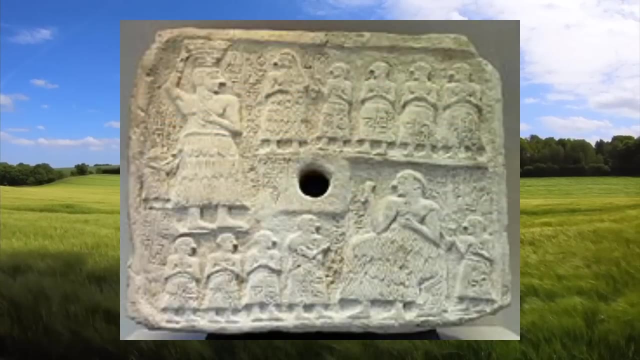 and the extraction of precious metals played a role in the decline of the indigenous cultures in the region. Dilmun. Dilmun, an ancient and enigmatic civilization, occupied a strategic location in the Eastern Arabian Peninsula, With its exact boundaries often debated among scholars, it is not really known. 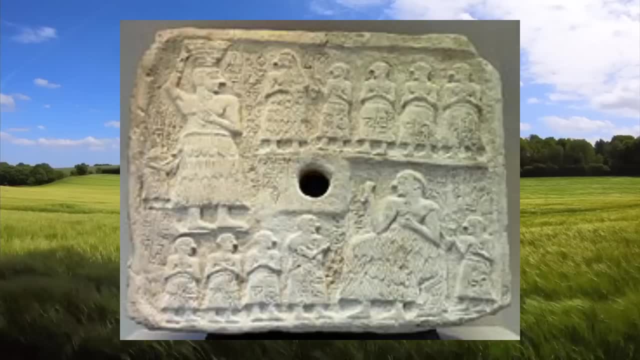 where they exactly were, but they have a rough estimate. Recognized as a crucial trade hub, Dilmun facilitated maritime routes connecting Mesopotamia to Indus Valley, Magan and the Andes. The end of the era, the Andes were the most popular and popular destination for the phuant people and the 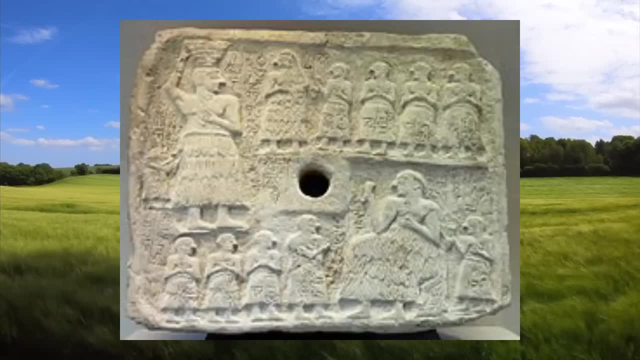 Gunn and other regions in the ancient Near East. Its prominence is immortalized in the Epic of Gilgamesh, where Dalam is portrayed as a parasitical land associated with the quest for eternal life. Agricultural, particularly the cultivation of date palms, was a key aspect of 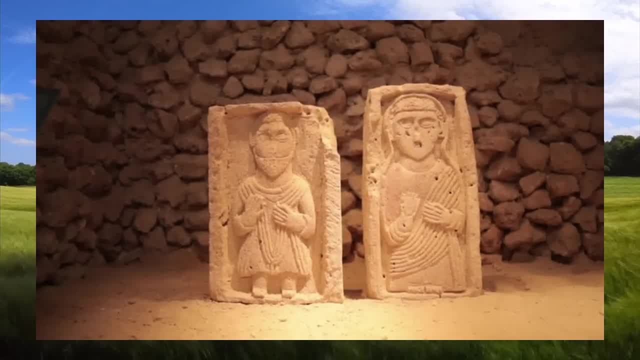 Dalam's economy, emphasizing the fertility of its land. The people of Dalam were known for their expertise in irrigation techniques, a crucial skill for sustaining agricultural productivity in such an arid and dry environment. Dalam's decline remains shrouded in mystery, with factors. 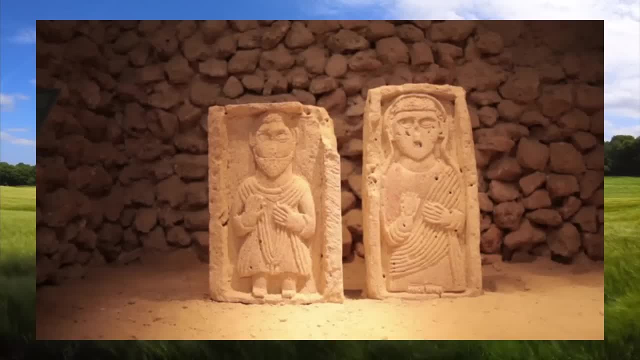 such as environmental changes, shifts in trade routes or geopolitical transformations, potentially contributing to its disappearance from all historical records. Despite this uncertainty, archaeological excavations, particularly on the island of Bahrain, have unearthed artifacts like cylinder seals, pottery and burial mounds, which help give us findings and glimpses into their 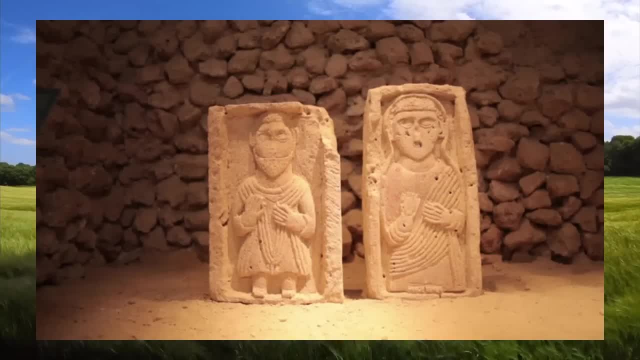 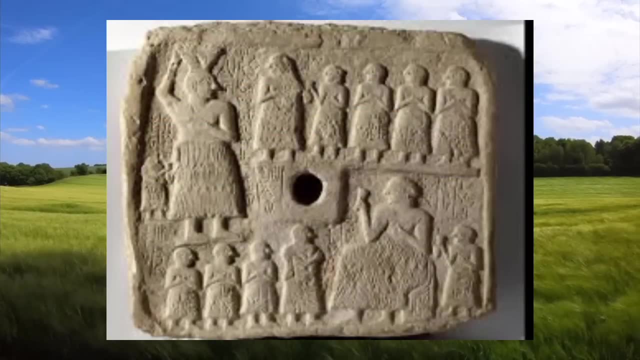 daily life, their trade activities and the religious symbolism of the land. The mention of Dilmun in ancient texts and its association with the mythical realm of immortality underscores crucial and historical significance. While the precise details of Dilmun's history may remain elusive, its impact on the trade networks and cultural exchanges, 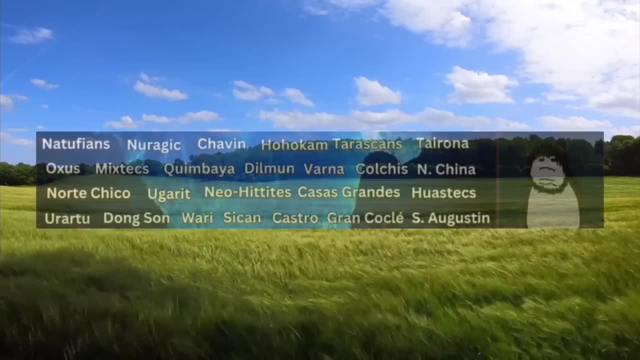 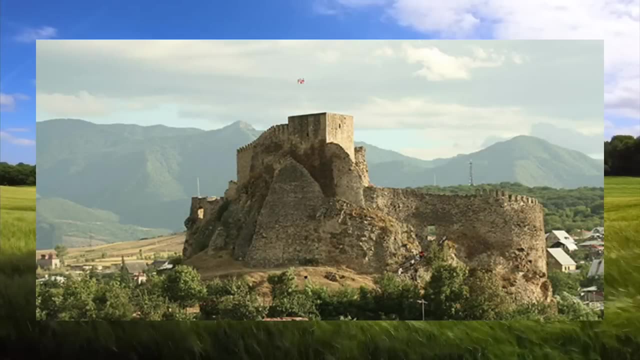 and religious exchanges is pretty important. Colchis. Colchis, situated along the eastern coast of the Black Sea in what is now western Georgia, holds a unique place in both Greek mythology and ancient Greek mythology. It is a place of great importance to the people of Dalam. 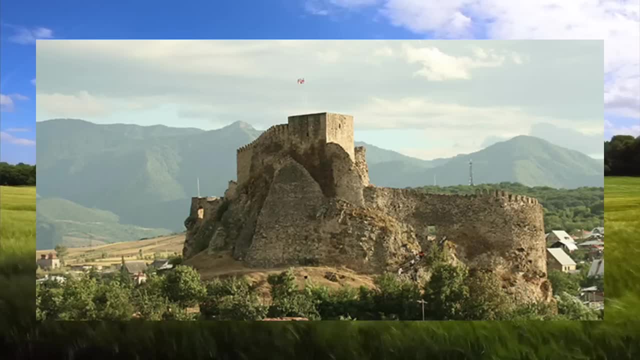 It is a place of great importance to the people of Dalam. It is a place of great importance to the ancient history, Best known for the destination of Jason and the Argonauts in their quest for the golden fleece. Colchis became the mythical realm ruled by King Aedias, where the legendary fleece 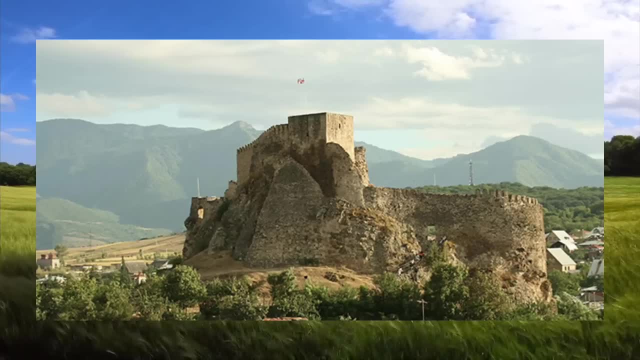 was guarded. The tale of the Argonauts, which involves Medea, the daughter of Aedias, adds a layer of mystique to the region. Despite and beyond its mythological fame, Colchis was a region for significant economic and cultural importance, blessed with fertile soil and gold deposits in 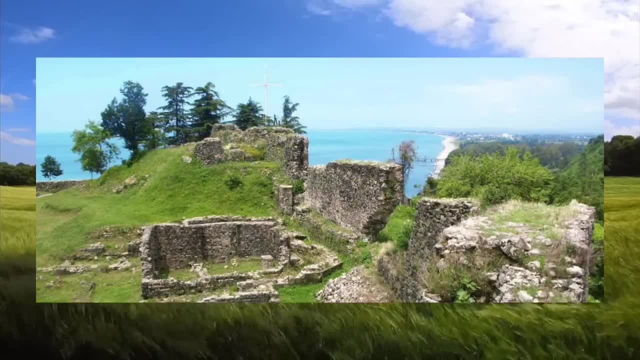 its river, so they were really able to be a big part of agriculture and agriculture. Colchis was a very important area in the world because it had so much valuable resources. Its strategic location along the Black Sea also made it a center of interest for Greek and Persian influences. 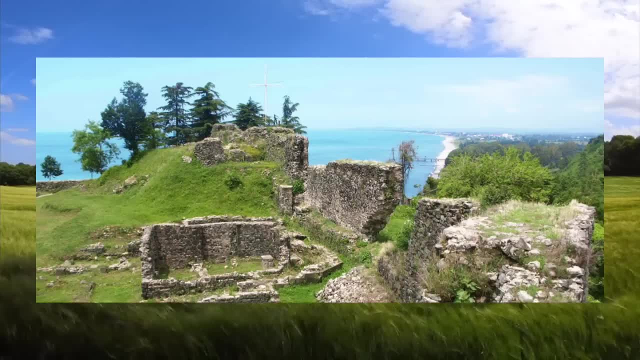 often caught in the power struggles between these ancient civilizations. Colchis' historical trajectory involved periods of incorporation to major empires including the Persian Empire, the Hellenistic Seludid Empire and later the Roman and Byzantine spheres of influence. 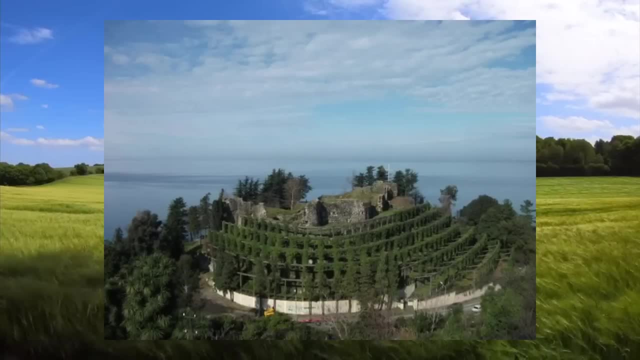 Archaeological excavations have uncovered evidence of urban centers, fortifications and burial sites, shedding light on the material culture and the historical developments of the region During the Roman period. Colchis became part of the Roman Empire and was integrated into the province of. 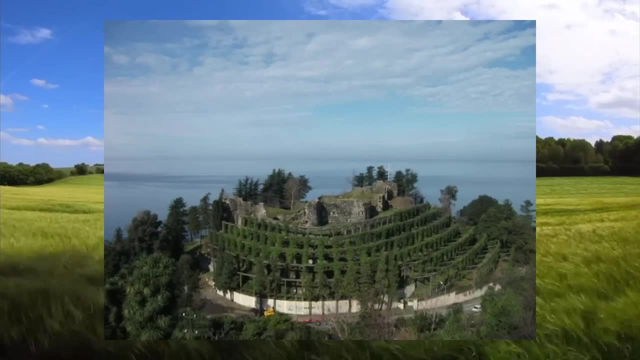 Lazicum. recognized for its strategic importance as a gateway to the Caucasus, The region underwent further cultural and political transformations later. The spread of Christianity in Colchis contributed to its evolving identity within the religious and the cultural landscape of the Roman Empire. Colchis, with its mythical allure and the historical significance, remains a 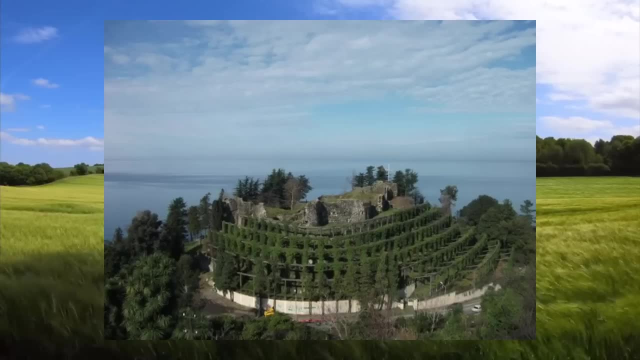 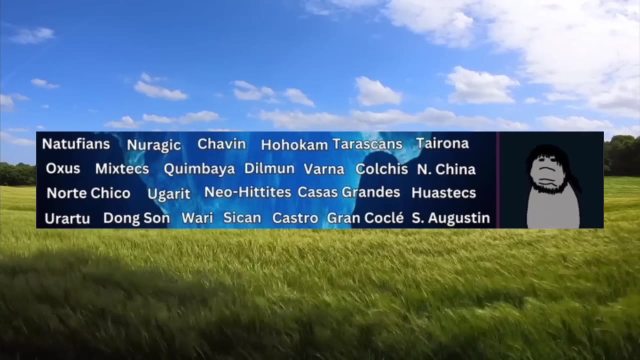 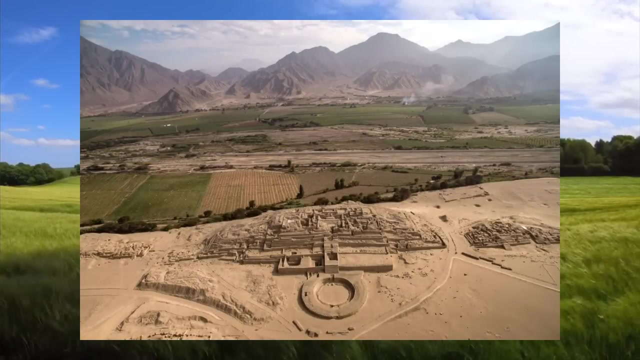 captivating chapter in the ancient world. Its legacy is woven into the fabric of both myth and history, and the very famous Roman Empire Norte Chico, also known as the Coral Supe civilization, stands as a remarkable testament to the early complexities of societies in the Americas, Flourishing along the central and north. 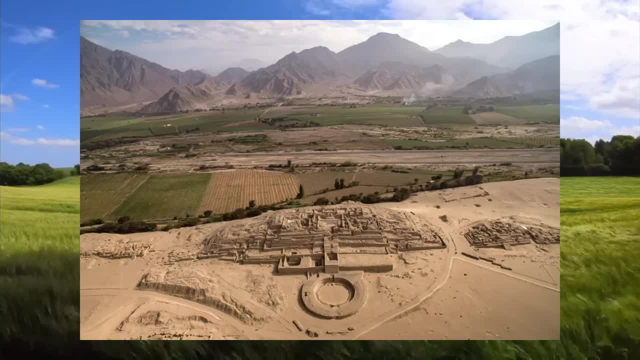 central coast of present-day Peru. Norte Chico emerged around the late 19th century. The city's history dates back to 3,500 BCE, making it one of the oldest known civilizations in the Western Hemisphere. The civilization reached its end around 3,000 BC, leaving behind a legacy of 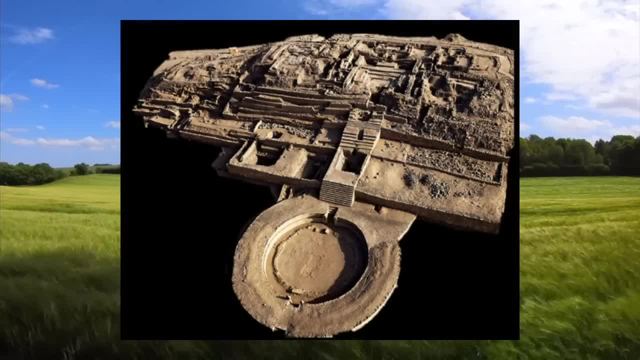 impressive urban centers, with Coral being recognized as one of the oldest cities in the Americas. At the heart of Norte Chico's urban landscape were monumental architectural features, including large platform mounds and a central pyramid. The layout of these urban centers reflects sophisticated planning and construction techniques, suggesting a well-organized and 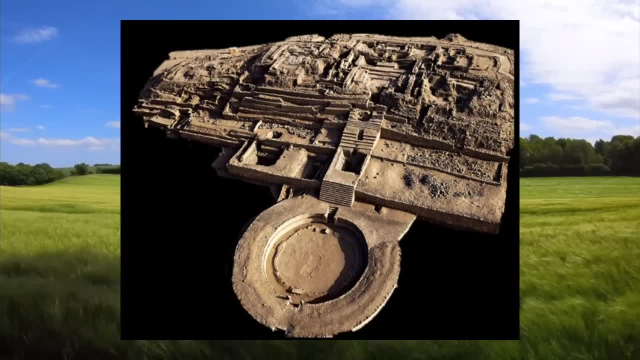 civilized society, Notably Coral, lacked defensive fortifications, challenging traditional assumptions with the necessity of such structures for ancient civilizations. So the lack of the walls and stuff like that kind of showed these were the only civilization in the entire area because they didn't have to defend anyone. Agriculture also played a pivotal role in the Norte Chico's 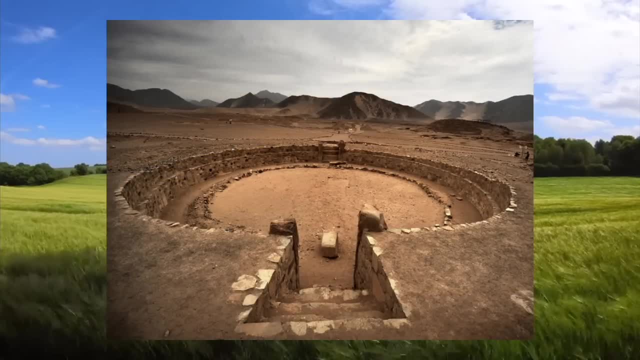 economy with the cultivation of crops like cotton, beans, squash and tubers in the fertile river valleys. The civilization also capitalized on the rich marine resources along the Pacific coast, engaging in fishing and maritime activities. Evidence of trade networks indicates interactions with neighboring regions and other Andean cultures. Despite its earlier. 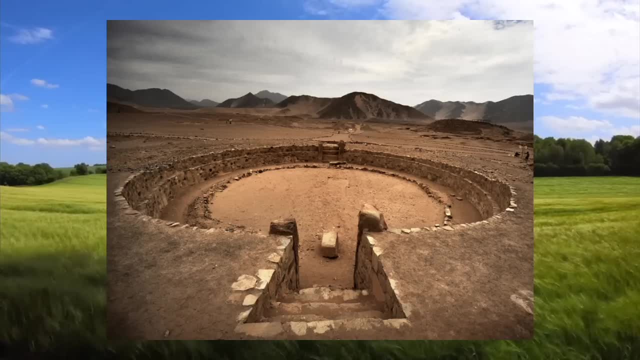 achievements. Norte Chico experienced a decline around 1800 BCE and the exact reasons remain subject of inquiry and debate. Proposed factors include environmental changes, alterations in the river courses or shifts in social dynamics. The study of Norte Chico challenges previous 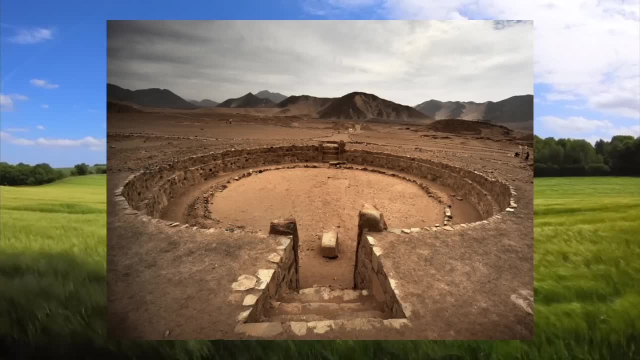 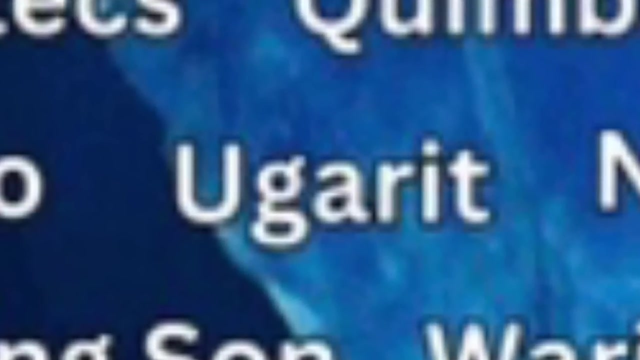 assumptions that advanced civilizations in the Americas only emerged later in Mesoamerica and the Andes, highlighting the complexity and how ancient this civilization was in human history. in the Western Hemisphere, Ugarit Ugarit- positioned on the northern coast of the Mediterranean Sea in what is now Syria. was a prominent city-state during the Bronze Age. Its historical significance lies in its role as a major port and a trading hub, facilitating maritime routes connecting the Aegean, Cyprus, Anatolia and the Levant. The city thrived economically through extensive trade, dealing in commodities like timber. 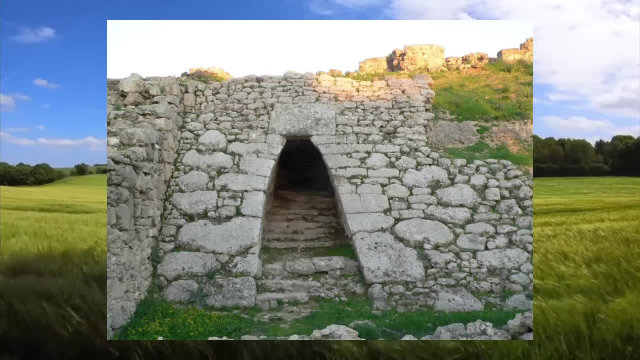 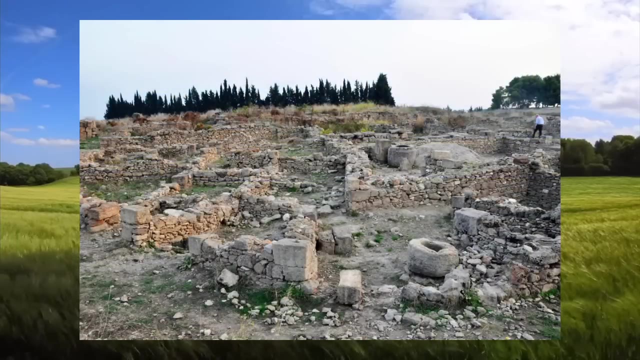 metals, textiles and olive oil. Its strategic location contributed to Ugarit's prosperity in the cultural interactions, making it a crucial intermediary in the trade networks of the ancient civilizations. One of the most remarkable archaeological finds at Ugarit was a collection of cuneiform tablets discovered in the royal palace. These tablets written 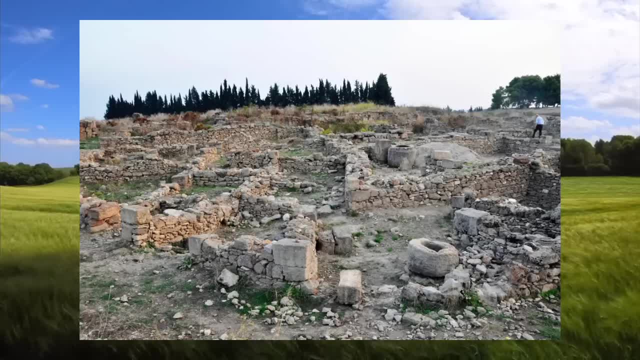 in the Ugarit script contain administrative records, economic texts and literature. The Ugarit texts included the Baal Cycle describing the adventures of the storm Gav and the Baal, providing invaluable insights into the political, economic and religious life of the city. 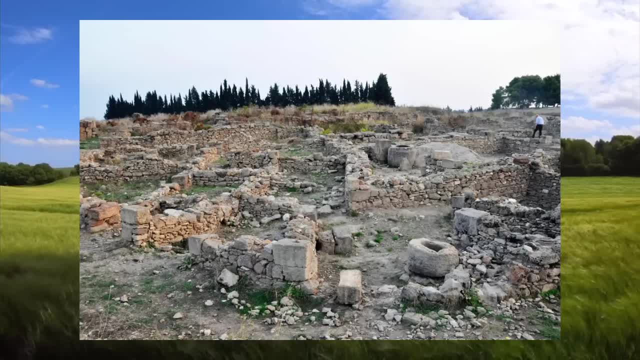 Around 1200 BCE, Ugarit faced a catastrophic event, possibly an invasion or a natural disaster leading to its abandonment. The city was eventually forgotten until its rediscovery in 1928 by French archaeologist Claude Chauffer. Subsequent excavations revealed well-preserved ruins. 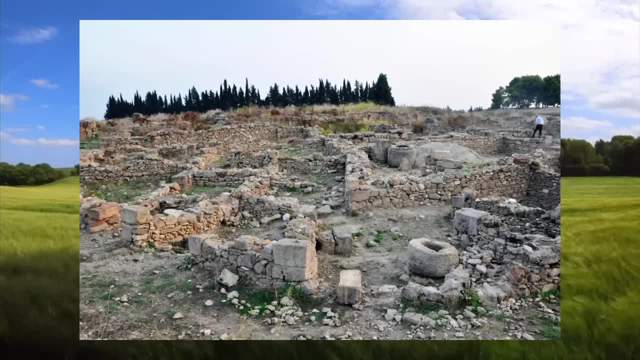 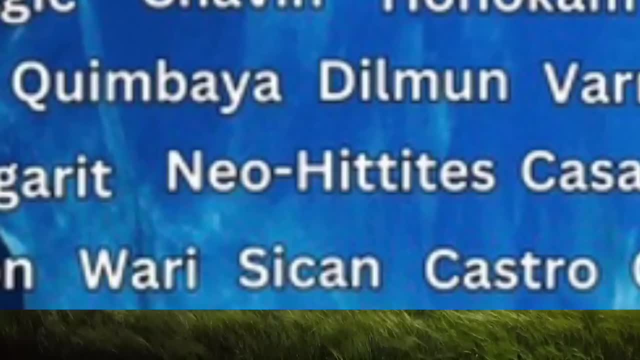 shedding light on Ugarit's architecture. Ugarit is one of the most important archaeological sites in the world. It is one of the most important archaeological sites of the European context. Neo- The Neo-Hittite state emerged in Anatolia following collapse of the Hittite. 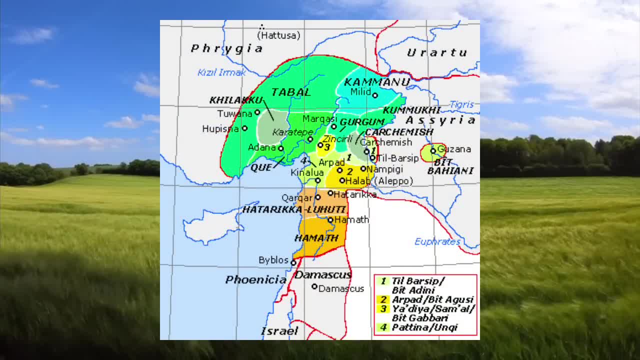 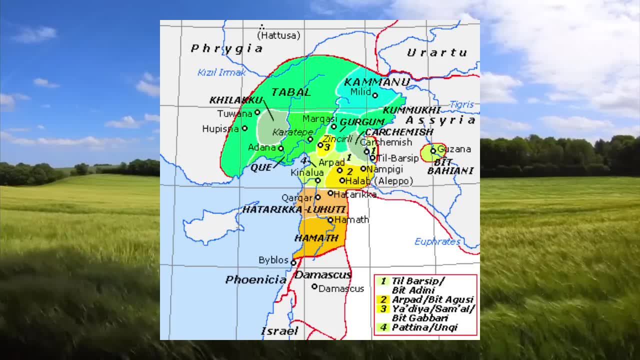 Empire around 12th century BCE. This collapse created a vacuum leading to the formation of smaller political entities, collectively known as the Neo-Hittite states. These states, characterised by a fusion of Hittite traditions and influences from neighboring cultures, became properly recognized. 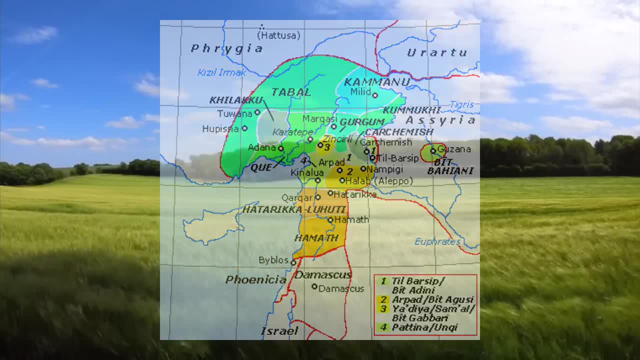 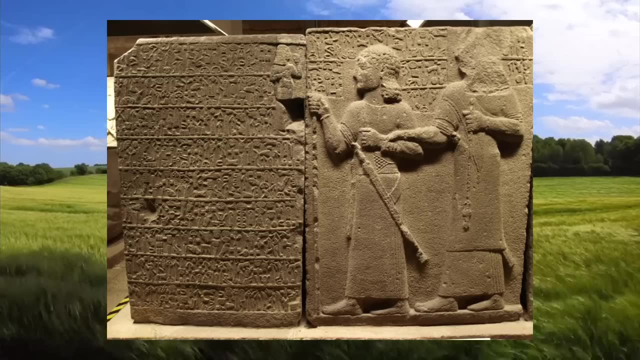 became prominent during the Late Bronze Age and the Early Iron Age, lasting from the 12th to the 7th centuries BCE. The political landscape of the Neo-Hittite states was diverse, consisting of city-states or small kingdoms, each governed by local rulers or kings. 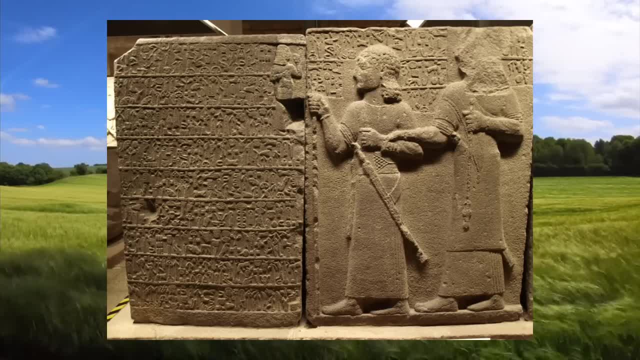 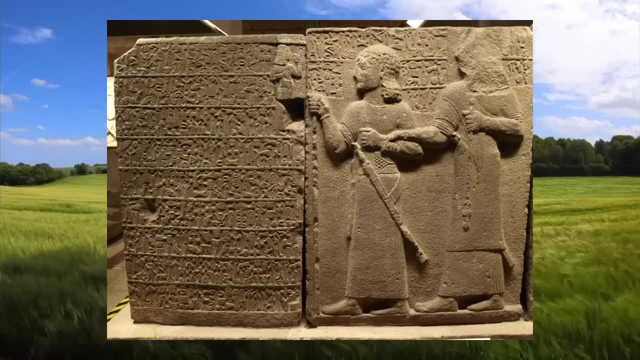 Notable among these states were the Carchemish, Matalite, Maled, Gergrim and the Carchemish. Despite the collapse of the Hittite Empire, the Neo-Hittite states demonstrated cultural continuity by the use of the Luwian hieroglyphs for inscriptions and incorporated artistic 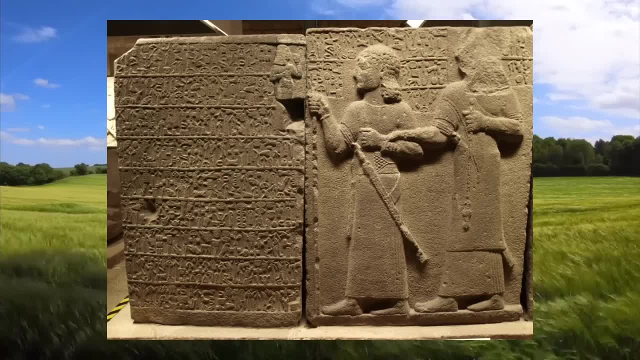 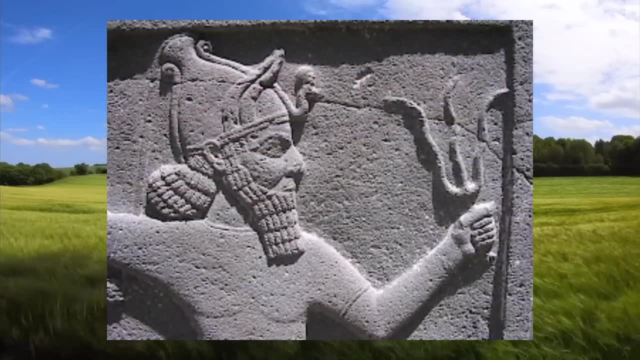 styles reminiscent of their Hittite predecessors, Influenced by surrounding cultures such as the Assyrians, Parthenians, Eurasians and the Armenians. the Neo-Hittite states participated in a dynamic geopolitical landscape marked by military conflicts, shifting alliances and power struggles. 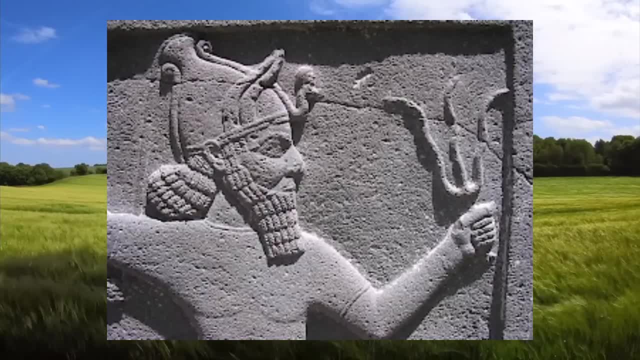 They engaged in both internal disputes and external conflicts with neighboring powers. The Neo-Hittite states gradually faced challenges, including invasion and the invasion of the Middle East. There was also invasion by the Assyrians, internal strife and pressure from expanding regional powers like the Parthenians and the Eurotians. By the 7th century BCE, many of these states had either disappeared or been absorbed into larger political entities and just disappeared as a whole. Casas Grandes stands as a testament to the ancient cultures that once flourished in northern Mexico during the Medieval Period, which was around 1200 to 1450 AD. 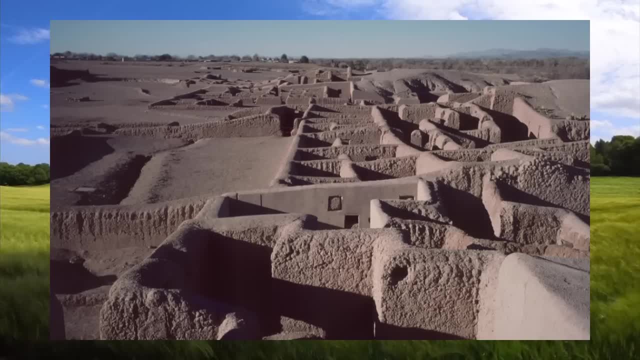 Situated in the Casas Grandes. Casas Grandes is one of the most important places in the world. Located in the Casas Grandes Valley in Chihuahua, the archaeological site features distinctive multi-storied structures earning it the name Big Houses. 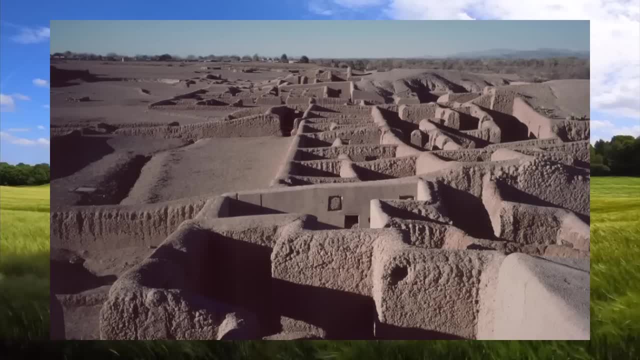 These adobe structures, arranged in a planned layout, reflect advanced urban planning and architectural skills. The Casas Grandes culture was characterized by its prominence as a major trading and cultural center. Engaged in extensive long-distance trade networks, the site showcased a rich material culture. 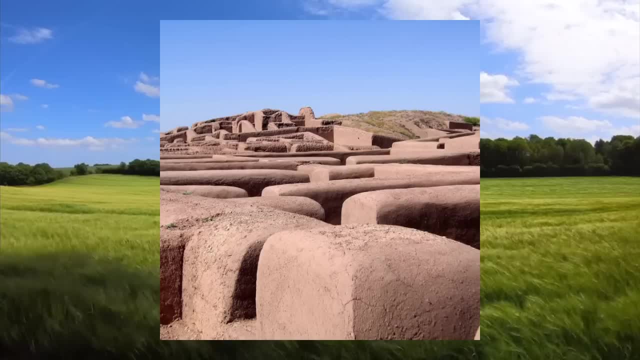 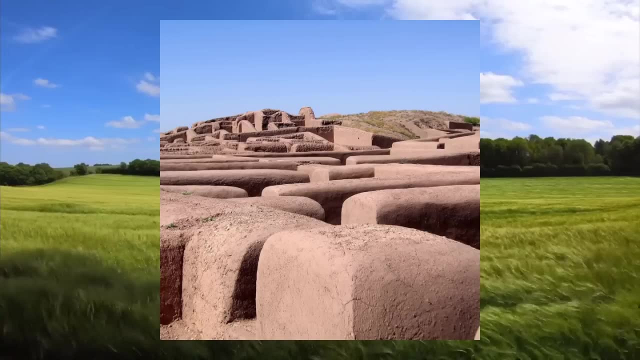 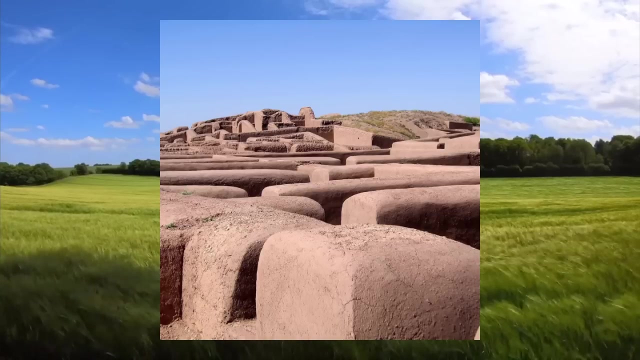 with artifacts such as macaw feathers from Mesoamerica and turquoise from the American Southwest. Modern activity highlights the cultural exchanges and economic interactions that redefined the region during its peak occupation in the 14th and 15th centuries. The ceramics of the Casas Grandes are renowned for their quality and artistic expression. Pottery featured intrinsic geometric designs and polychrome decoration, indicating a highly developed artistic tradition within the community. Agriculture played a crucial role in sustaining the sedentary lifestyle of the inhabitants, with the fertile Casas Grandes Valley providing suitable conditions for the community to live. 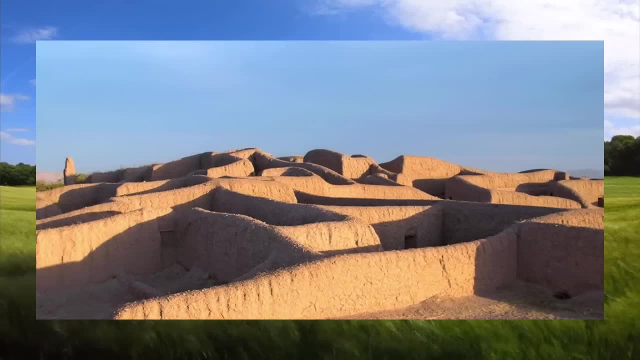 in The Casas Grandes Valley is known for cultivating crops like maize beans and squash. Despite its significance, the decline of the Casas Grandes around the mid-15th century remains a mystery. Scholars propose various different factors, including environmental changes, resource. depletion or social and political distributions as possible contributors to the site's abandonment. Casas Grandes gained archaeological attention in the late 19th and early 20th centuries, with notable excavations conducted by researchers like Charles de Pesso. The Casas Grandes Valley is one of the most important archaeological sites in the world. 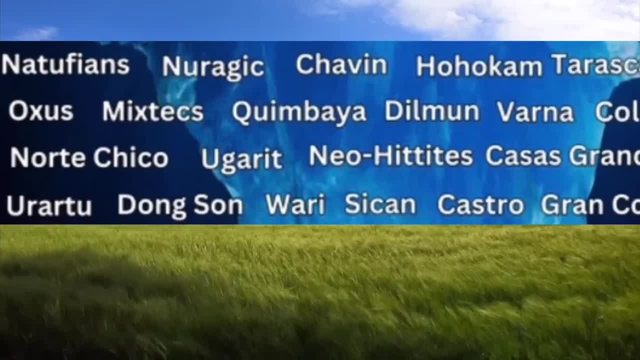 It is one of the most important archaeological sites in the world. It is one of the most important archaeological sites in the world. It is one of the most important archaeological sites in the world. 8. Dong Son: The Dong Son culture flourishing in northern Vietnam's Red River Delta during the Bronze. 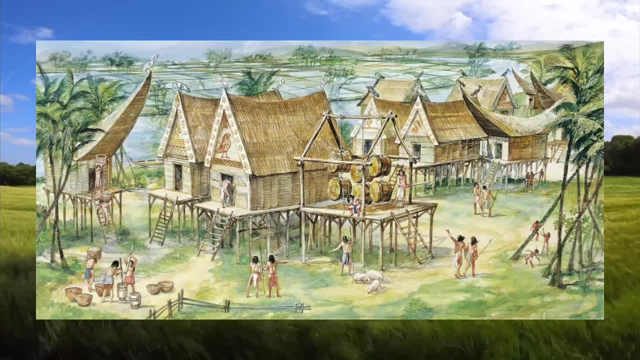 Age is renowned for its sophisticated metallurgy, notably the creation of intricate bronze drums. These drums, considered masterpieces of ancient Vietnamese art, reveal the Dong Son people's advanced metalworking skills. Cast using elaborate techniques, the drums were adorned with detailed depictions of daily 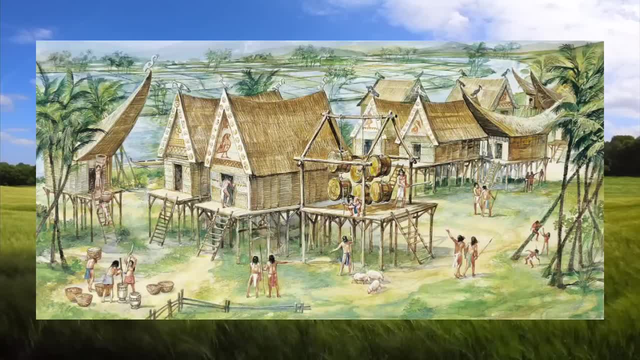 life, mythical creatures and symbols of authority. The craftsmanship involved in their production, from creating reinforced beams to the creation of high-pressure metalwork. The left hand side of the bronze system is based on theitas, the upper right hand side of the bronze stem. 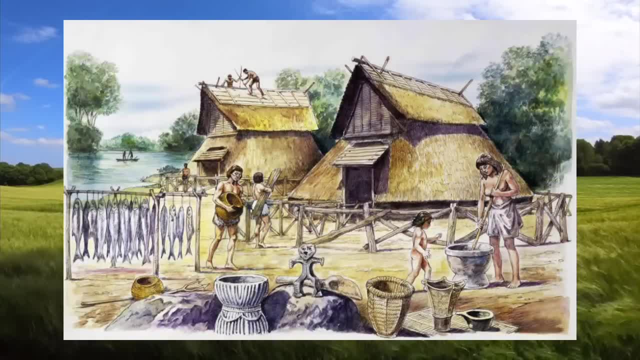 The upper right hand side of the bronze stem is the upper left hand side in clay molds to final finishing touches reflects the culture and the technological advancements and achievements of the Dong Sun civilization. Beyond metallurgy, the Dong Sun culture exhibited a multifaceted society engaged in agriculture, ceramics and distinct burial. 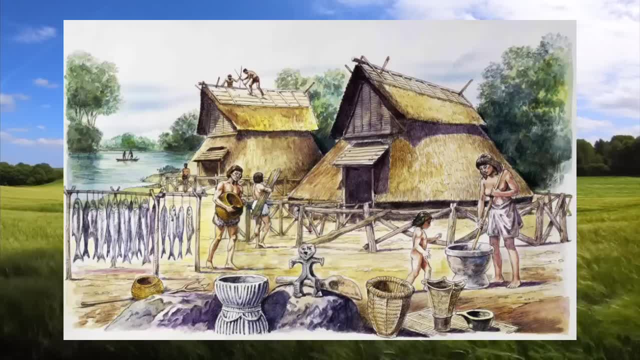 customs. Rice cultivation played a crucial role in the agrarian economy, and settled communities thrived in the fertile plains of the Red River Delta. Evidence suggests that Dong Sun had trade connections with neighboring regions, enriching their cultural landscape with influence from China and India. The decline of the Dong Sun culture remains somewhat unknown. with proposed 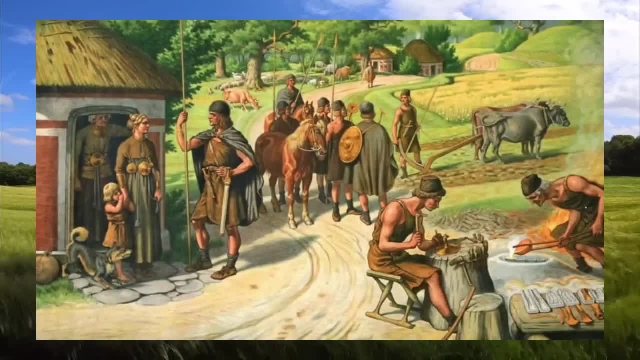 factors once again being environmental changes, shifts in trade patterns or interactions with other neighboring cultures. Despite its eventual decline in the early century CE, the Dong Sun culture has left an enduring legacy. The bronze drums, in particular, not only stand as archaeological. 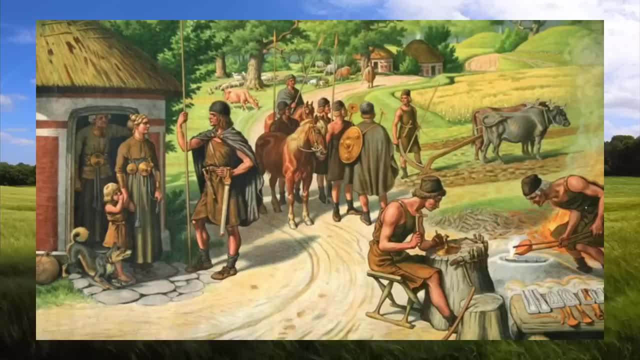 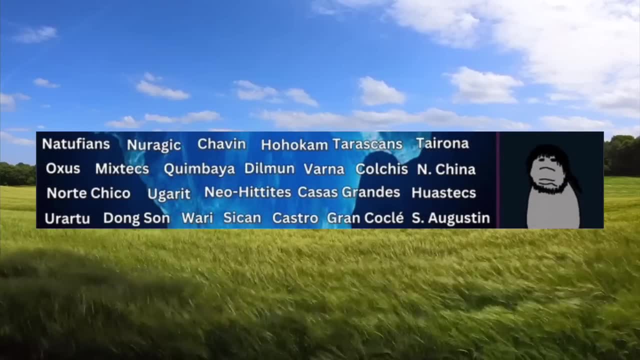 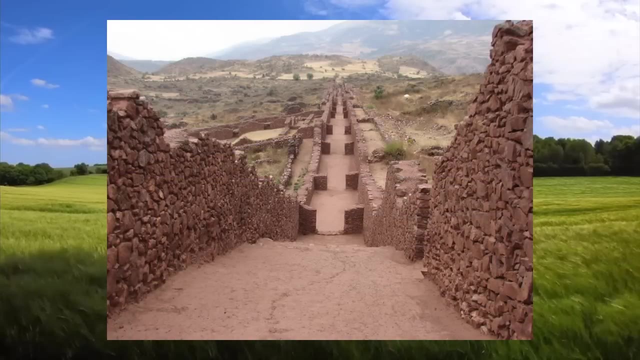 treasures, but also serve as potent symbols of Vietnamese culture, identity permeating folklore, literature and contemporary art. 2. The Wari civilization flourishing in the central highlands of present-day Peru from 600 to 1000 CE stands as a testament to the sophistication of pre-Columbian Andean cultures. 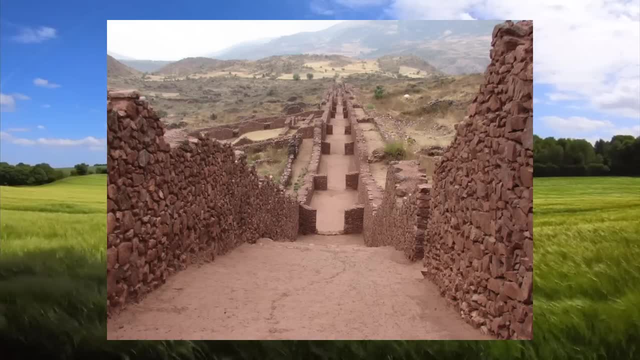 Censored around the city of Huari in the Ayachua Valley, the Wari Empire displayed remarkable architectural achievements, featuring well-planned urban areas with multi-story buildings, plazas and extensive infrastructure. 3. 4. The Wari were served as the hub for political, economic and religious activities, showcasing 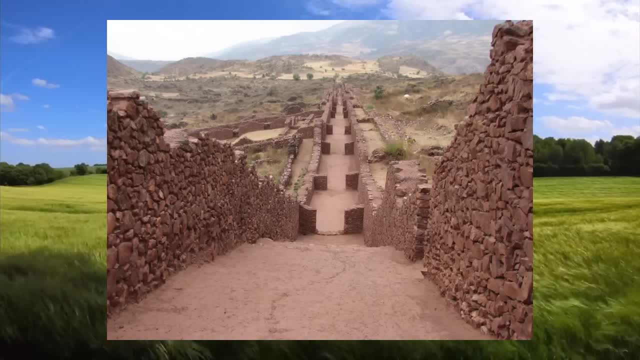 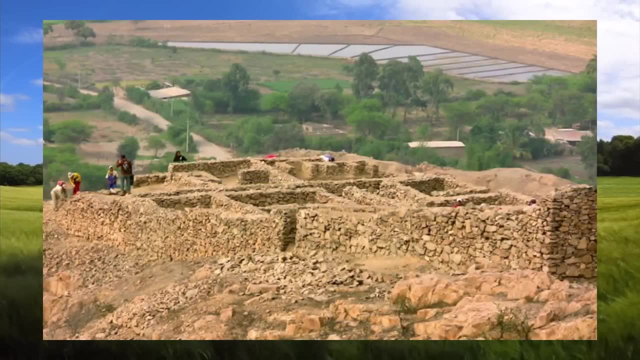 the organizational prowess of the Wari people. Agriculturally, the Wari implemented innovative techniques such as terraced fields, allowing them to cultivate crops in the challenging, monotonous terrain. Their ability to sustain a large population contributed to the success and the longevity of the civilization. 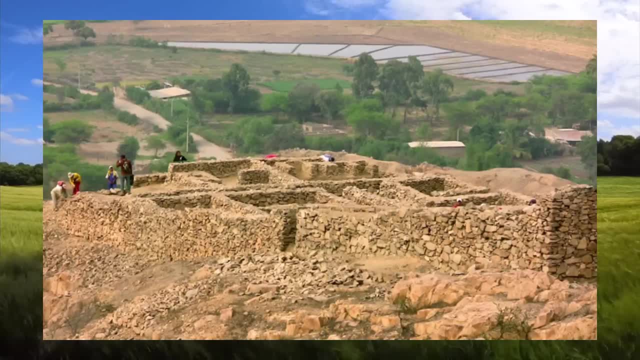 The Wari are particularly renowned for their distinct artistic style, evident in their textile designs, pottery and intricate metalwork. 5., 6., 6., 7., 8., 9., 10., 11., 12.. 13., 14., 15., 16., 17., 17., 18., 19., 19., 20., 21., 22., 23., 24., 25., 26., 27.. 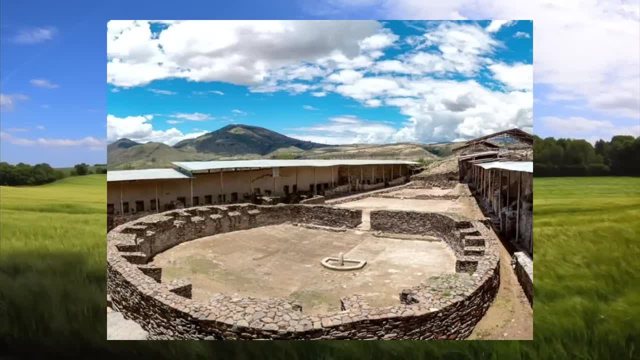 28., 29., 29., 30., 31., 32., 24., 31., 2., 0., 2., 4., 1., 5., 0., 6. 6.. 1., 4., 7., 8., 8., 3., 5., 6., 7., 6., 7., 8., 9., 9., 10., 10., 16.. 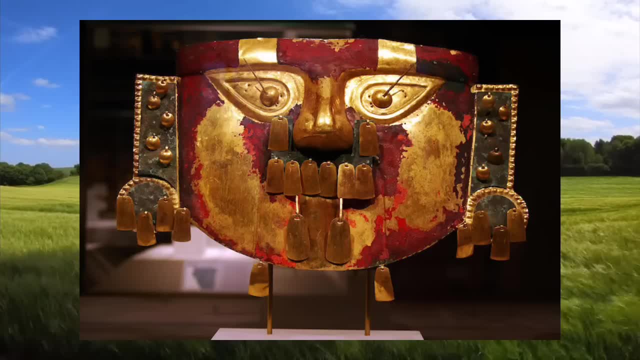 the Shikun people showcase remarkable skills in metallurgy, particularly in the crafting of gold and silver artifacts. Their mastery of sophisticated techniques such as alloying and guiding is evident in the intrinsic masks, jewelry and ceremonial vessels that have become hallmarks of 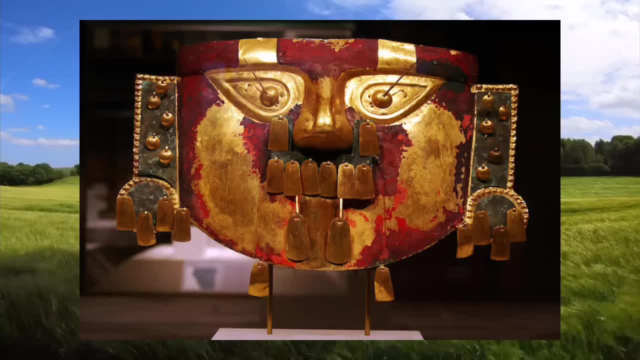 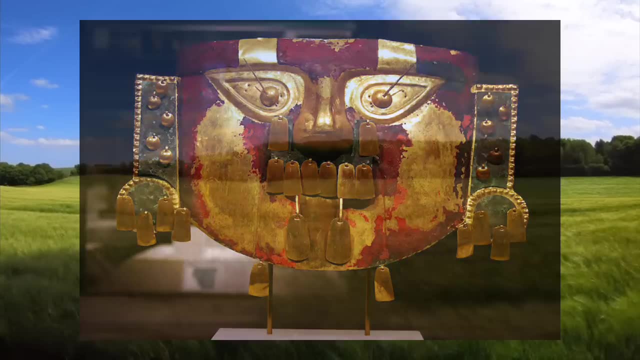 Saiken metalwork. Elaborate burial practices characterize the Saiken culture, revealing social stratification and the importance of certain individuals within their society. Tombs discovered at Saiken archaeological sites contain individuals adorned with rich grave goods, providing insights into the cultural and religious significance. 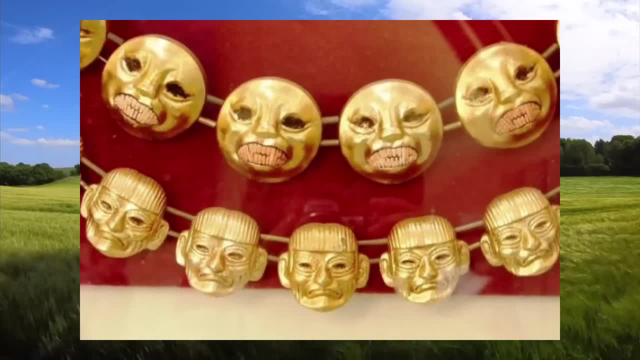 attached to death and the afterlife. Saiken ceremonial centers, notably Baton Grande, played central roles in religious and administrative activities, serving as hubs for ceremonies and rituals. In addition to their metalworking prowess, the Saiken people produced distinctive ceramics featuring symbolic and mythological motifs. The art of the Saiken. 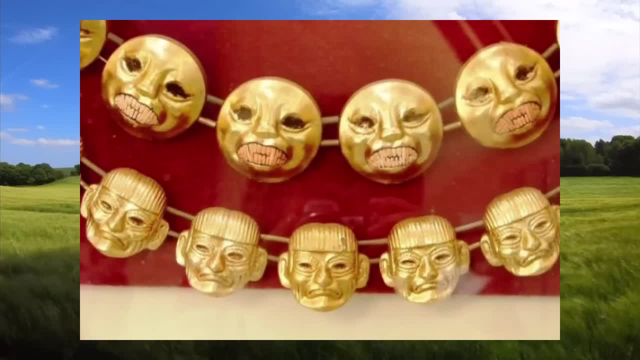 civilization reflects their religious beliefs and cultural practices, offering glimpses into the narratives that shaped their worldview. The Saiken economy was grounded in agriculture, with efficient irrigation systems supporting the cultivation of crops, particularly maize, in the desert environment. Despite the notable achievements of the Saiken culture, the factors contributing to its decline remain enigmatic and 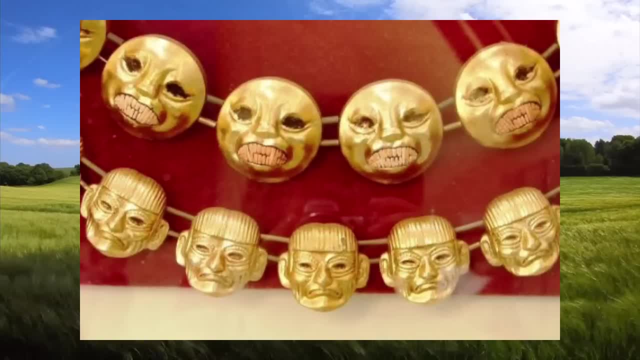 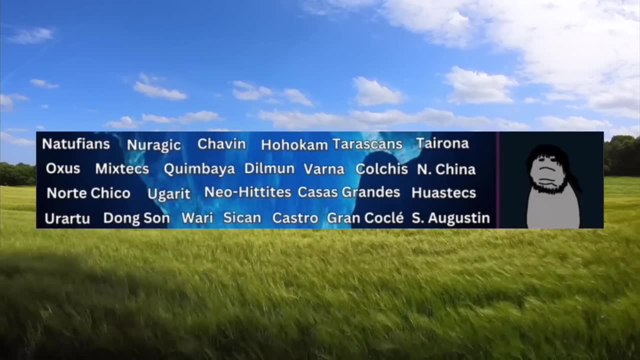 unknown, Environmental changes, social dynamics and potential external influences may have all played roles in the waning and disappearance of the civilization Castro. The term Castro culture refers to a pre-Roman island of the Saiken region. The Saiken region is a region of the Saiken region, which is a 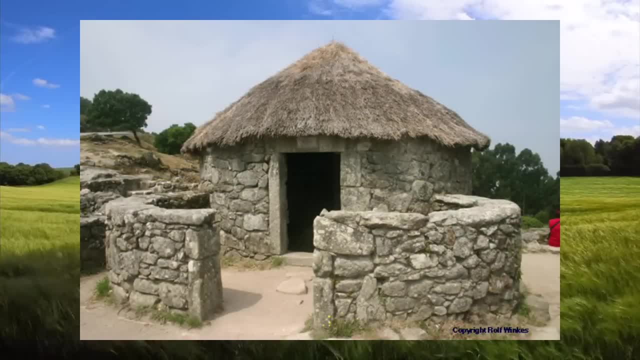 region of the Saiken region, which is a region of the Saiken region. which is a region of the Saiken region. Iron Age Celtic culture in the northwestern Iberian Peninsula, including Calcea, Astrulis and northern Portugal, Named after its characteristic hill forts or castros. 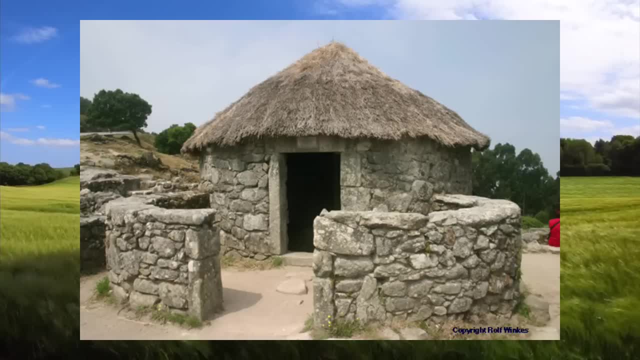 these fortified settlements were strategically positioned on elevated terrain, often surrounded by defensive walls and ditches. Circular or oval-shaped huts made of wood and thatch were common within these hill forts, arranged in concentric patterns. Agriculture played a crucial role in the society, with the cultivation of crops like wheat and barley, along with the 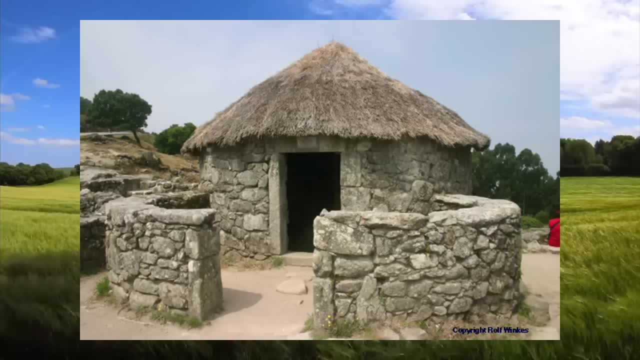 raising of livestock. The Saiken culture was a place of great interest for the Saiken people. the castro people were skilled metalworkers producing bronze iron tools, weapons and ornaments. Artistic expression was evident in pottery, sculptures and metalwork featuring. 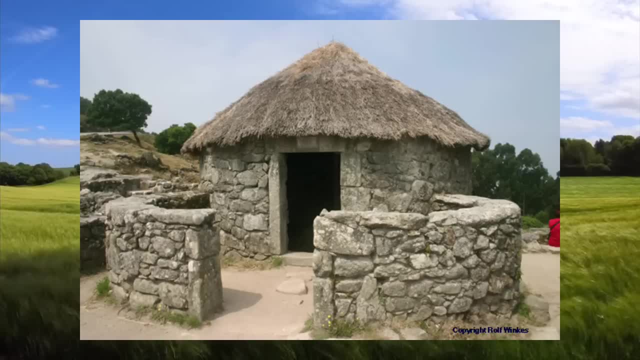 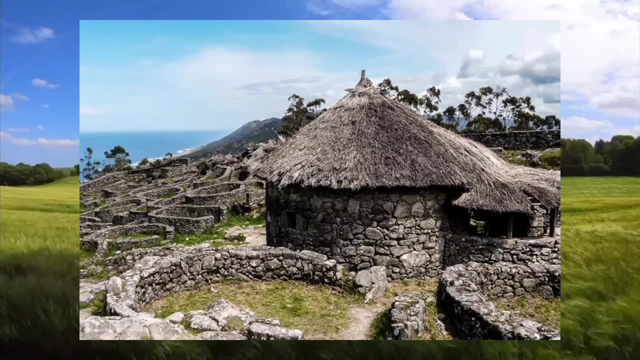 intricate designs with geometric patterns and animal motifs. Social organization likely involved a hierarchy, with a ruling elite residing in the central part of the hill forts, while the surrounding areas housed the common population. The castro culture had interactions with neighboring Celtic, Iberian, Bohesian and Greek cultures thriving from the 9th century BCE until the Roman. 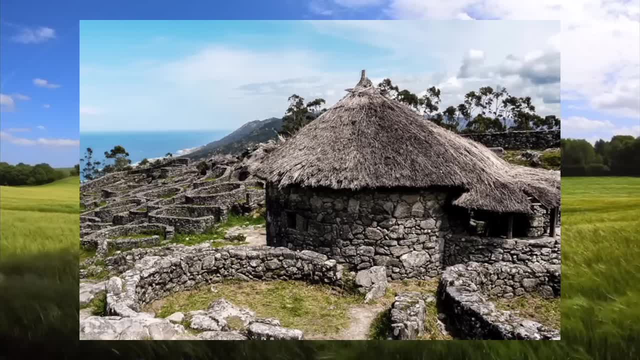 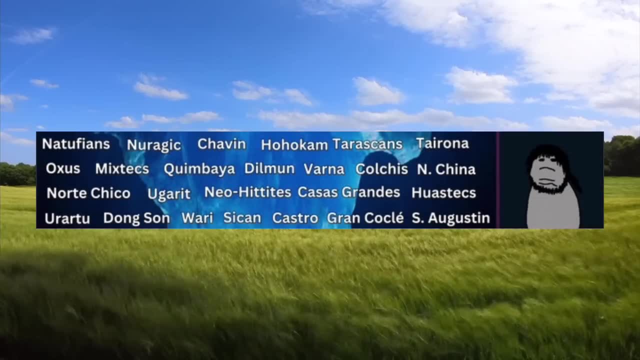 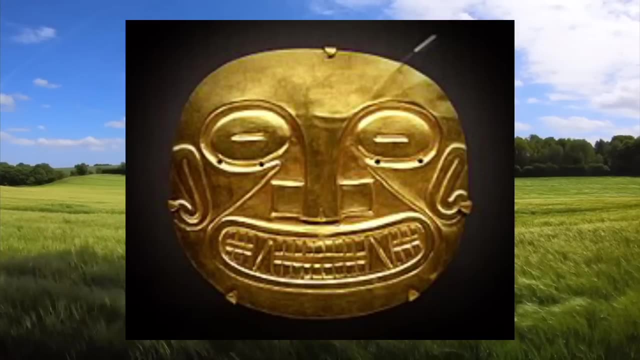 conquest in the 1st century AD. The castro culture was a place of great interest for the Saiken people, which is why it is considered a source of cultural heritage. Gran Cosle Represents a significant archaeological culture area in pre-Columbian Central America particularly. 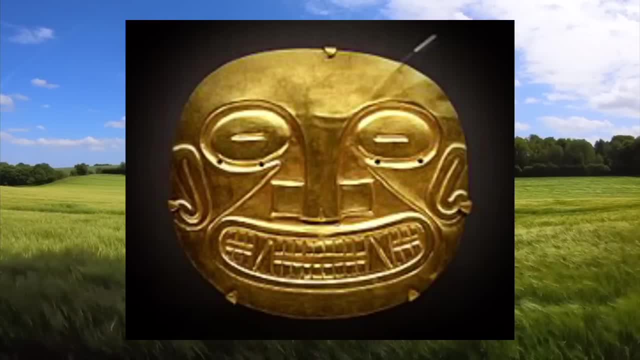 in the modern-day Panamanian providence of Cocle. This area encompasses multiple identifiable native cultures, loosely designed by pottery styles, with distinct periods such as the La Mula period, the Tenoizo period and the Cubita period. The La Mula period is a period 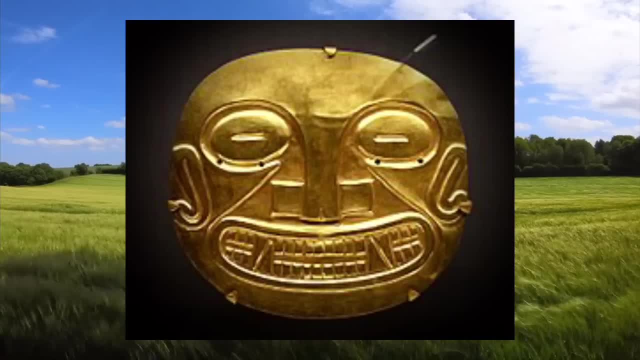 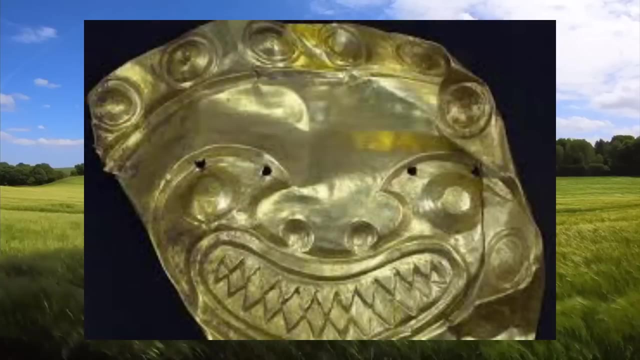 that includes the La Mula period, the Tenoizo period and the Cubita period. The La Mula period is a period that includes the La Mula period, the Tenoizo period and the Cubita period. The. The artifacts uncovered in this region, dating all the way back to the poorly studied La Mula period to later periods, include impressive examples of work: gold and other metals, carved bone, shell and whale ivory, textiles, jewelry with semi-precious stones and pottery. 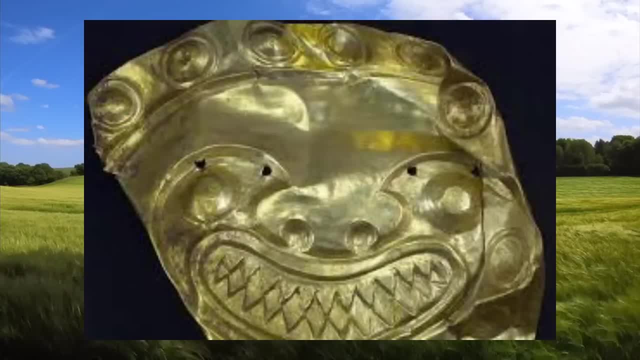 The gold work from Concle was traded widely in the region, reaching as far as Concle in Yucatan. The archaeological site of Cito Conte, though unfortunately damaged in the 1920s by unprofessional excavation, has still been yielded valuable findings. 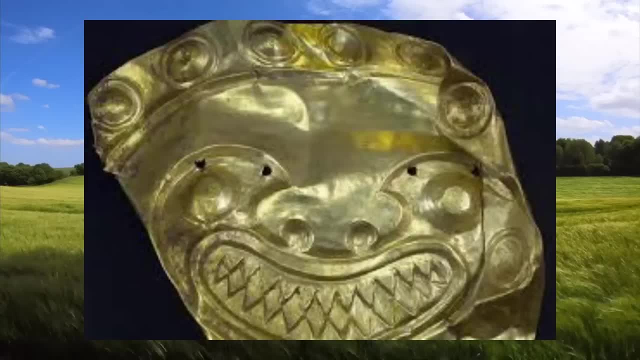 Subsequent, more careful excavations by archaeologists such as Samuel K Lothrop and J Alden Mason in the 1930s and 40s at Cito Conte in Elcano have provided important insights into the Concle culture, even though some of it was destroyed before. 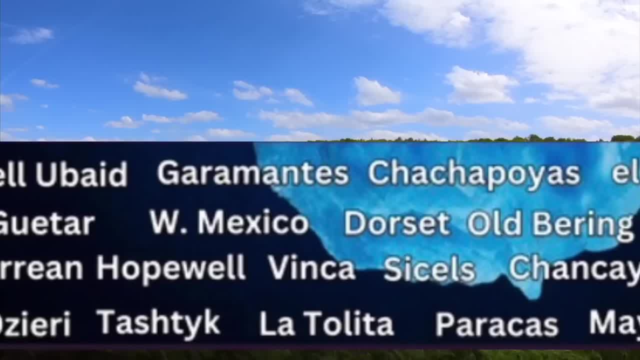 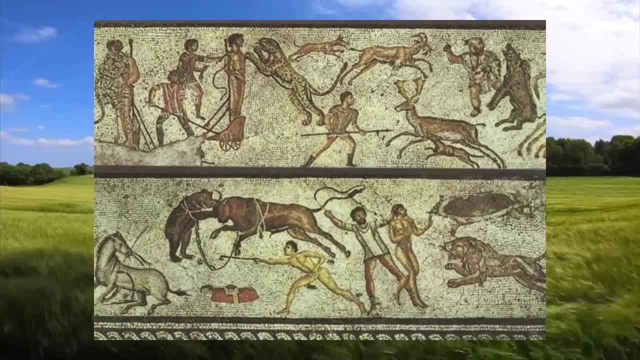 All right. now on to Tier 6, starting off with the Garamantes. An ancient Berber people occupied the region of Fasan in southwestern Libya, crafting a remarkable civilization in the heart of the city During the first millennium BCE to the 6th century CE. their strategic location along trans-Saharan trade routes facilitated connections between the Mediterranean and sub-Saharan Africa. 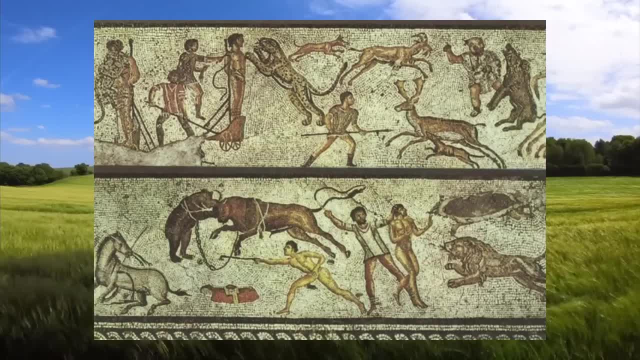 One of the Garamantes' notable achievements was their mastery of underground irrigation systems. They ingeniously constructed gnats, or fregara, tunnels designed to extract water from underground aquifers, enabling agriculture, cultivation and the arid desert environment. 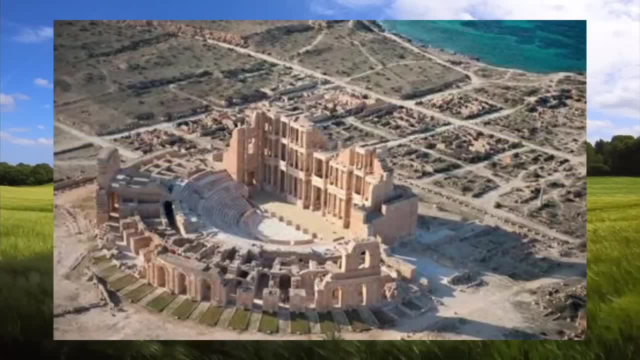 This technological prowess played a pivotal role in their ability to sustain civilization. The Garamantes established connections with neighboring cultures and engaged in commerce with the Roman Empire. Their urban centers, including the capital city of Garma, served as hubs for political, economic and social activities. 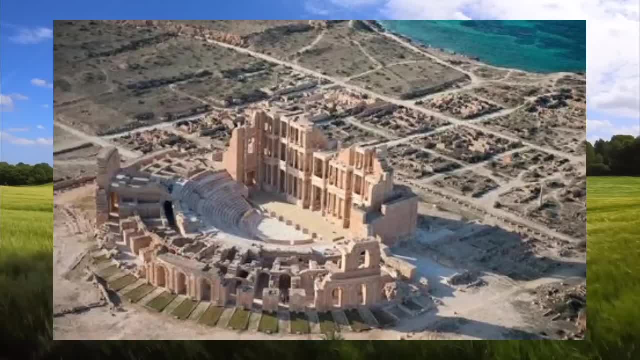 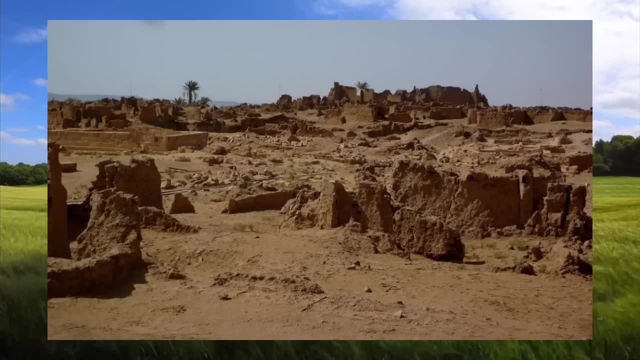 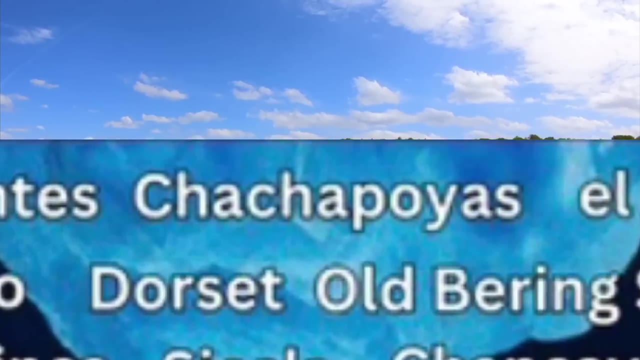 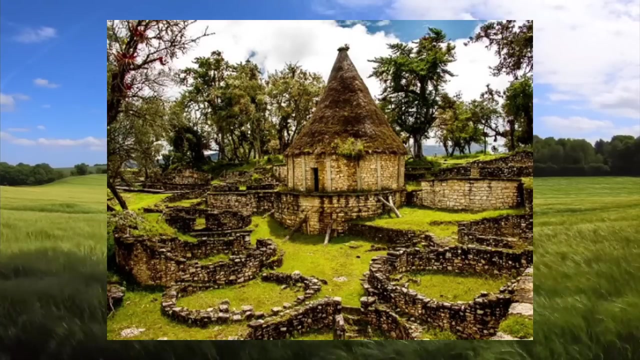 Despite their accomplishments, the decline of the Garamantes remains uncertain. Factors such as shifting trade routes, environmental changes and potential conflict with neighboring groups may have all contributed to the civilization's eventual decline. Chacapoyas- Chacapoyas, an ancient Andean culture that thrived in the cloud forests of northern Peru, left an indelible mark on their unique civilization from the 9th century to the mid-16th century. 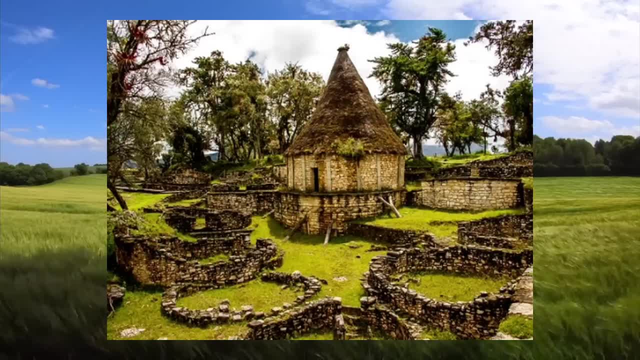 Renowned for their impressive architecture. the Chacapoyas built structures like the Fortress of Quilap, situated on a mountain ridge and surrounded by high walls with circular buildings. This architectural prowess is also evident in other sites, such as the Sacropagy of the Caran and the Fortress of Rivage. Distinctive burial practices set the Garamantes' position as the center of the Garamantes' civilization. Chacapoyas, an ancient Andean culture that thrived in the cloud forests of northern Peru, left an indelible mark on their unique civilization from the 9th century to the mid-16th century. 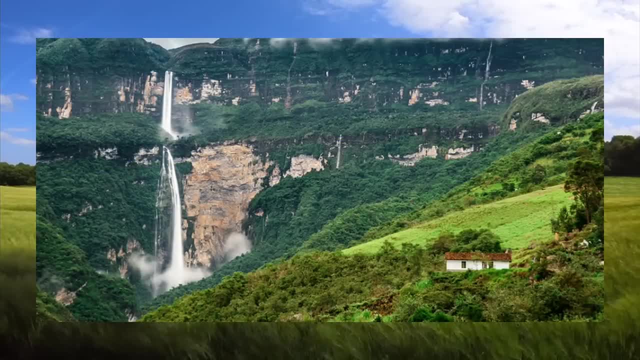 This architectural prowess is also evident in other sites, such as the Sacropagy of the Caran and the Fortress of Rivage. Chacapoyas, an ancient Andean culture that thrived in the cloud forests of northern Peru, left an indelible mark on their unique civilization from the Garamantes' civilization. 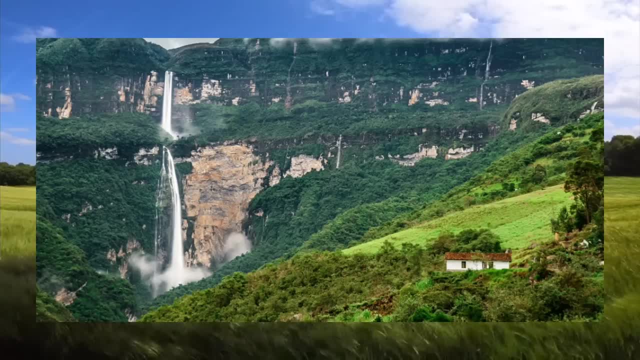 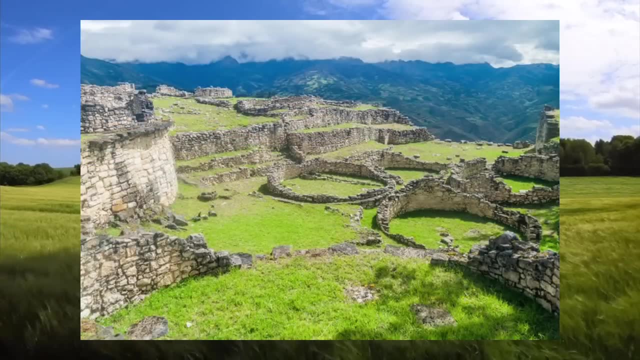 Chacapoyas, an ancient Andean culture that thrived in the cloud forests of northern Peru, left an indelible mark on their unique civilization from the Garamantes' civilization. The arrival of the Spanish in the 16th century also marked a new chapter, as the Chacapoya region faced the challenges of colonization, including demographic decline due to introduced diseases and social upheaval. and today the archaeological legacy of the Chacapoyas captivates historians and archaeologists. 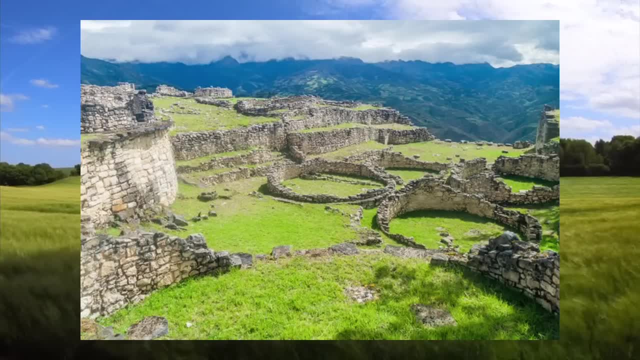 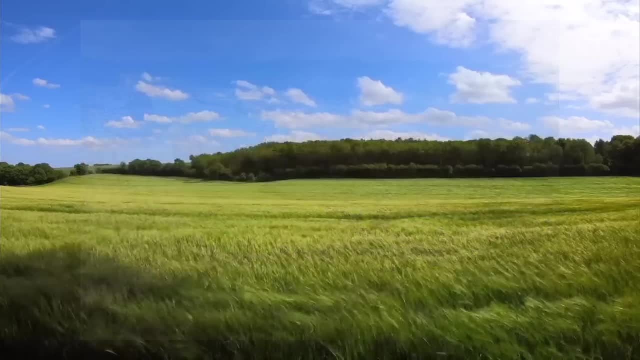 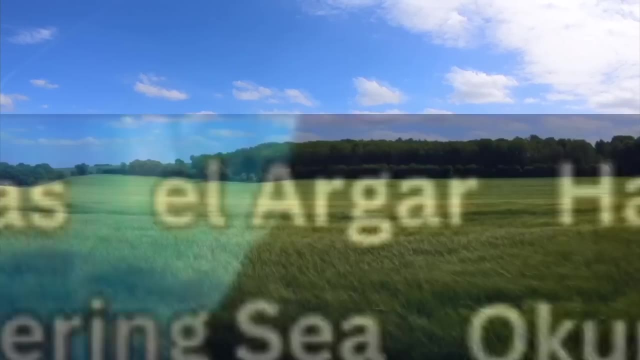 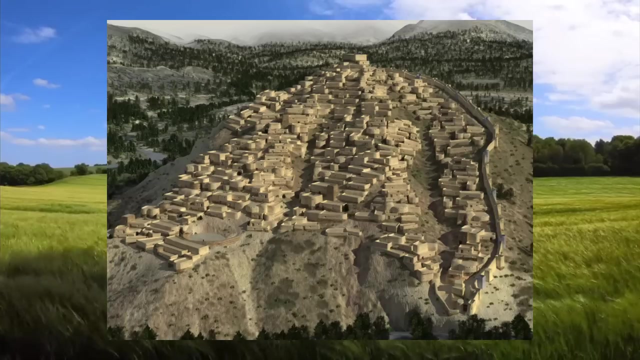 The region of Chacapoyas in northern Peru is home to well-preserved sites that offer insights into the culture and architectural achievements of this fascinating Andean civilization, El Argar. The El Argar civilization, thriving in the southeastern Iberian Peninsula during the second millennium BCE, from approximately 2200 to 1550 BCE, is named after the archaeological site of El Argar in Almeria, Spain, characterized by distinct material culture and social organization. 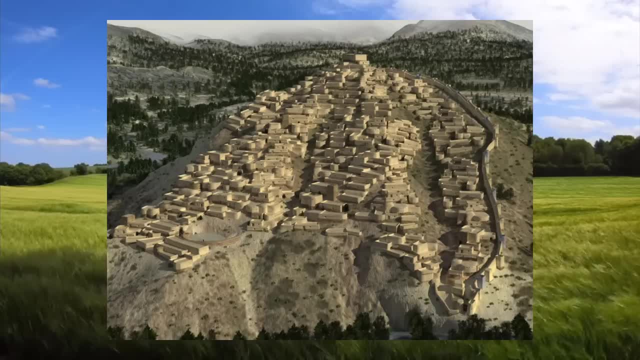 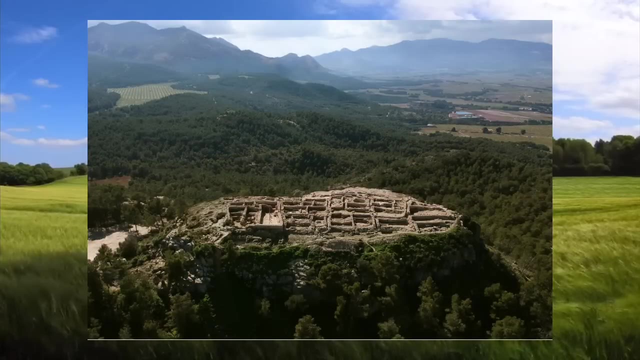 El Argar settlements were strategically fortified, often perched on elevated terrain and surrounded by defensive walls suggesting a need for protection from other cultures or civilizations. Social hierarchy was evident in El Argar society, reflected by undifferentiated burial practices in varying sizes of dwellings. 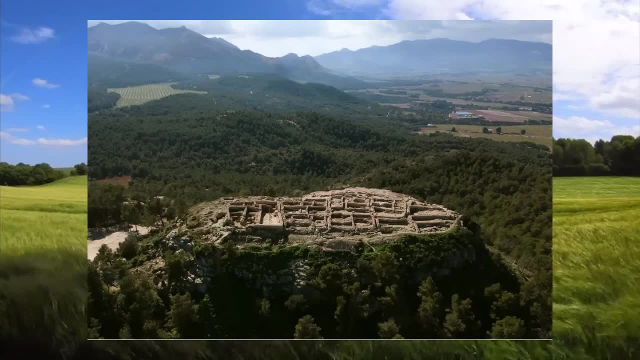 Certain burial contained valuable grave goods highlighting indications of social stratification. The ceramic tradition of El Argar was marked by unique shapes and painted geometric patterns, showcasing the culture's artistic achievements. Metalworking played a crucial role in El Argar as well, with the civilization demonstrating proficiency in crafting bronze items, including weapons, tools and ornaments. 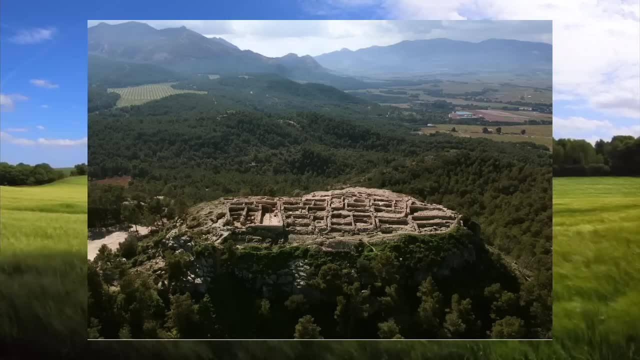 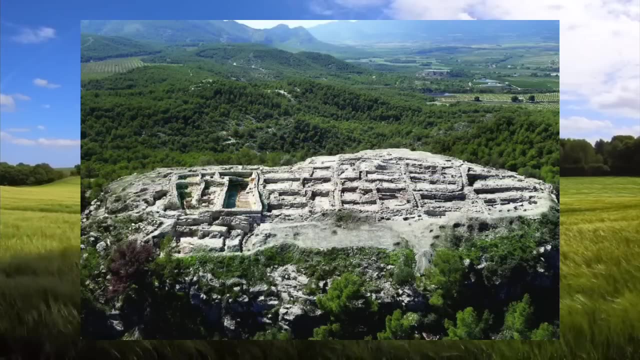 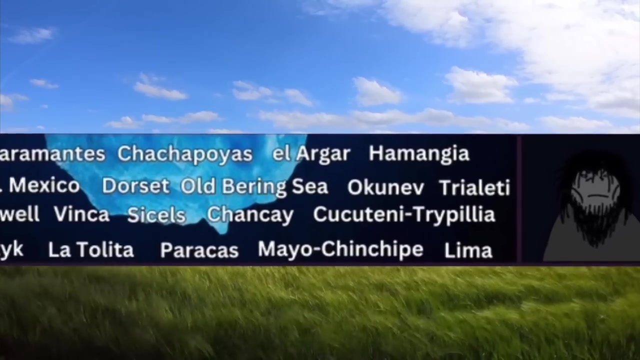 Metal objects found in burials underscore the significance of these items. in their society Engaged in agriculture, the El Argar people also cultivated crops such as cereals and lugames, and practiced animal husbandry, including the raising of cattle- Homongia. 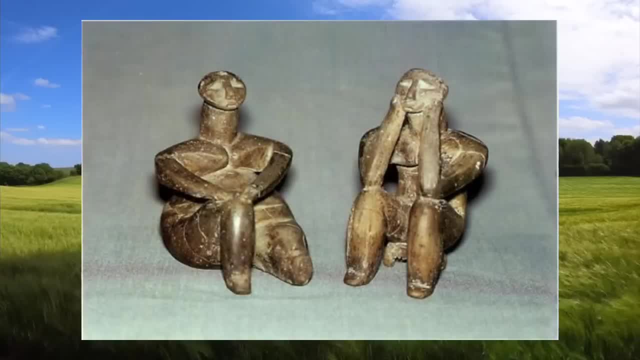 The Homongia culture flourishing in the 6th millennium BCE in the territories of present day Romania and Bulgaria derives its name from the archaeological site of Homongia situated on the Black Sea coast of the Sea of Tartus, The Khabarov. 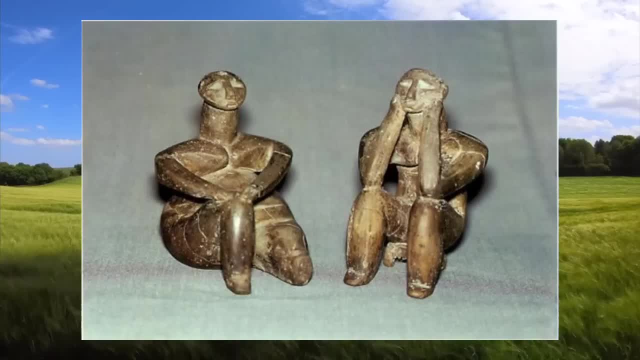 Khabarov. Khabarov, on the Black Sea coast of Romania. Characterized by its distinctive pottery, the Neolithic culture offers valuable insights into the technological prowess and lifestyle of its ancient inhabitants. Hamanjia pottery stands out for its intricacy and fine craftsmanship, featuring geometric 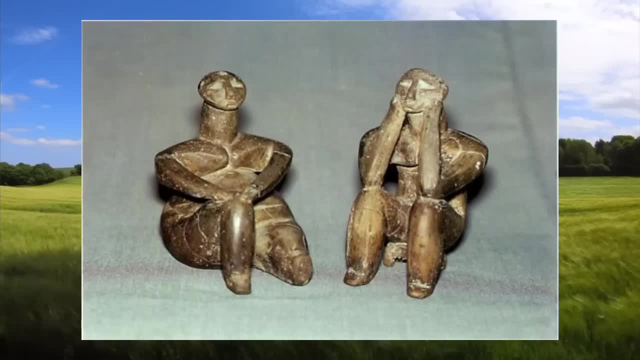 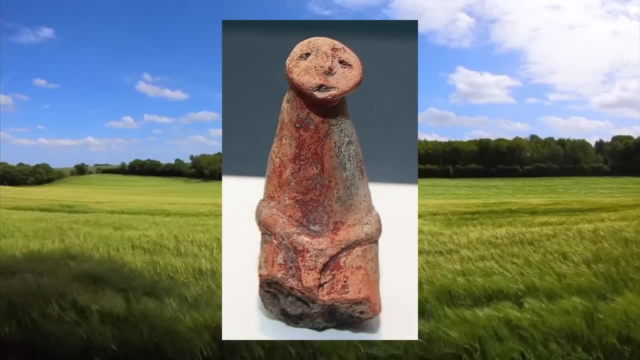 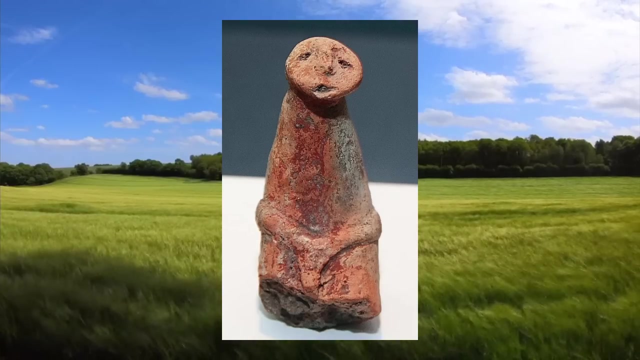 patterns, zoomorphic motifs and anthropomorphic representations. This artistic skill suggests advanced capabilities in ceramics. The Hamanjia people lived in small villages and settlements, strategically positioned near rivers and coastal areas to ensure access to water resources and to facilitate transportation. The economy of the Hamanjia culture was centered around agriculture, animal husbandry and 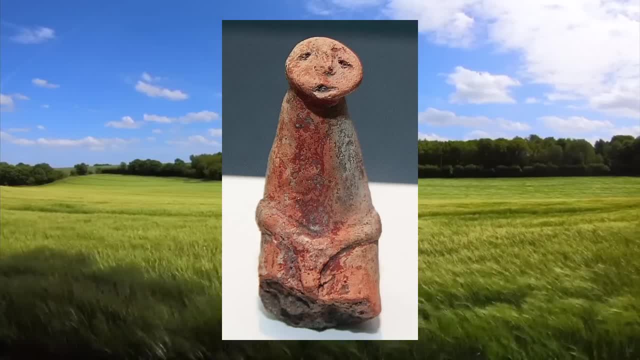 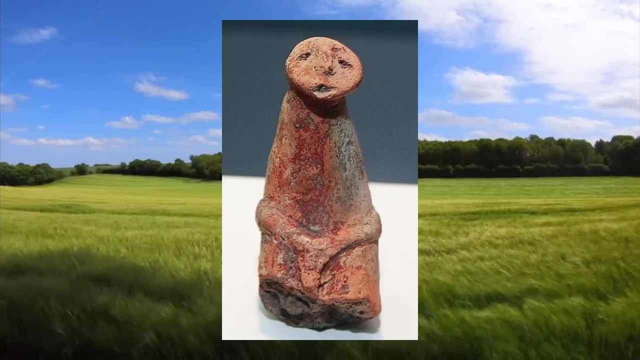 fishing. They cultivated crops like wheat and barley, while domesticating animals such as cattle and sheep. in addition to pottery, Hamanjia artisans crafted various tools from stone, bone and antler. Personal ornaments, including jewelry, made from shells to bones, have also been discovered. 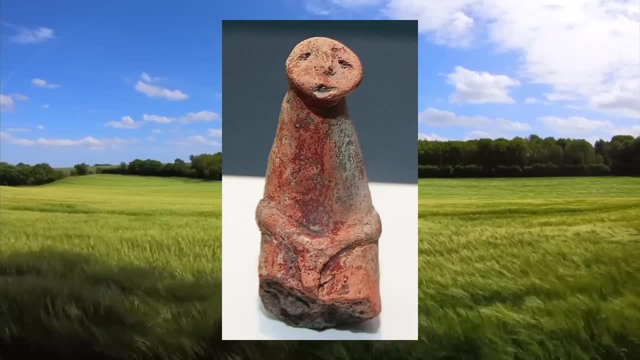 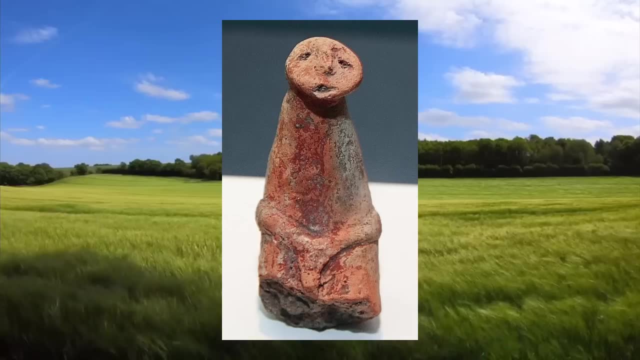 at Hamanjia sites. Trade and interaction were integral to the Hamanjia culture. The Hamanjia culture was evidenced by the exchange of raw materials and finished goods with neighboring societies. The Hamanjia people participated in a broader cultural network system with the Danube region. 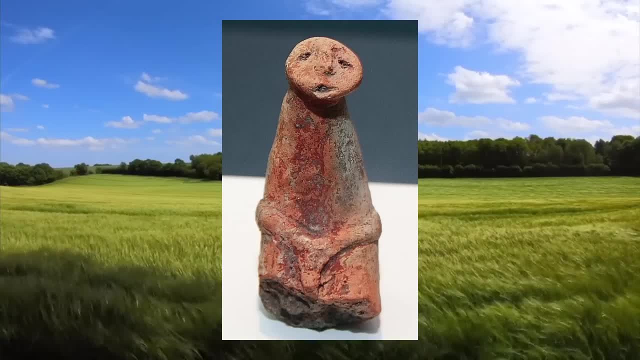 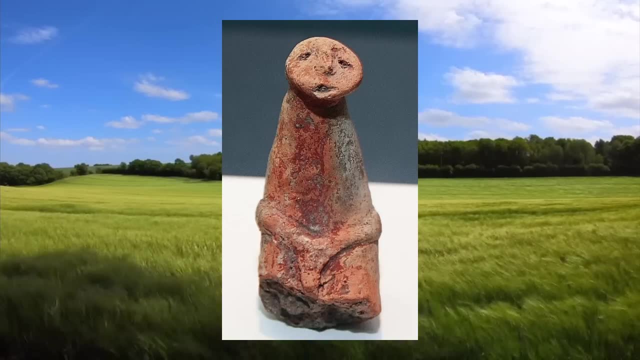 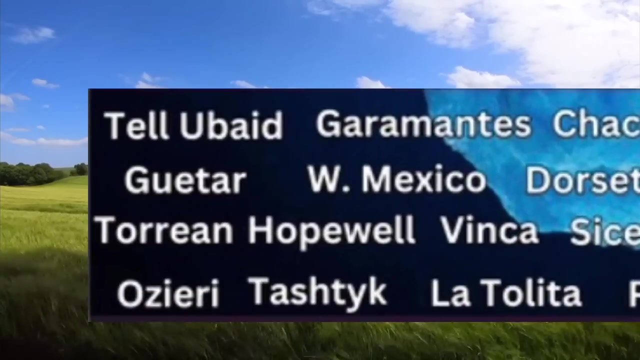 The broader context of Southeastern European prehistory and the Hamanjia culture occupies a significant place, contributing to our understanding of early agricultural societies and their advancements in crafts, particularly in the development of pottery. Guattar, Guattar, Guattar. 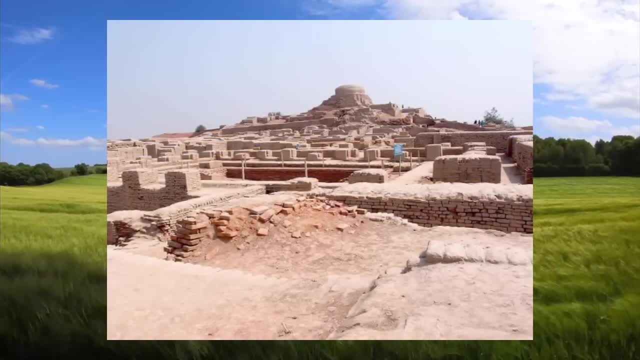 Guattrã Guattrã, Guattrã, Guattrã, Guattrã Guattrã. In the early 1860s, an indigenous people, pre-Columbian era, inhabited the central region of Costa Rica, contributing to the rich tapestry of cultures in Central America, thriving in 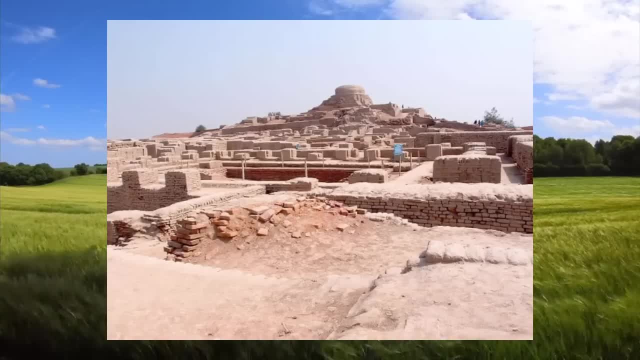 what is now known as Costa Rica. The Guattar people were integral to the intermediate-area cultural complex. Their society was characterized by a strong connection to agriculture, with the focus on cultivating staple crops like maize beans and squash. Within their communities, the Guattar developed a complex social structure reflecting various 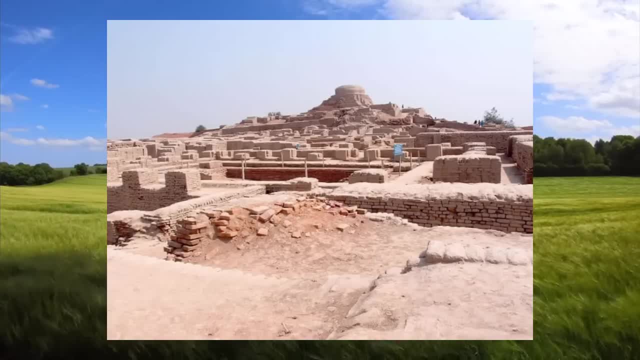 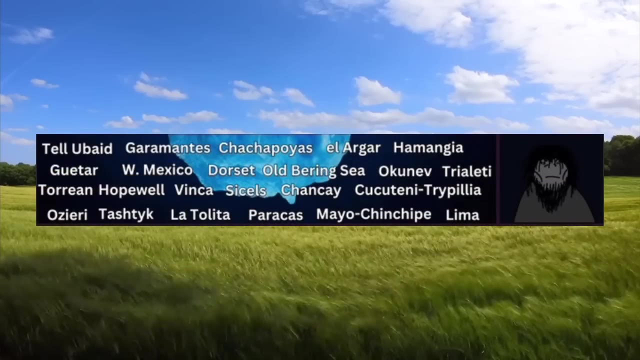 roles and responsibilities. Guattar Guattar Guattrã organization often included individuals fulfilling specific roles within their community, contributing to the overall well-being and functionality of their society. The legacy of the Qatar people is a significant part of the cultural history of Costa Rica. 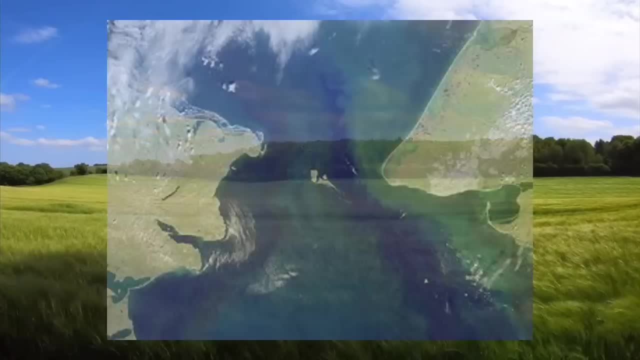 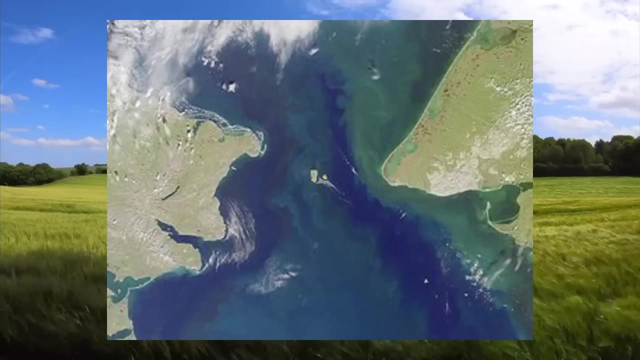 Old Bering Sea. The Old Bering Sea culture, spanning from around 200 BCE to 500 CE, was an archaeological phenomenon centered in the coastal regions of western Alaska and eastern Siberia. Known for its distinctive artifacts, particularly intricate ivory carvings, this culture showcased 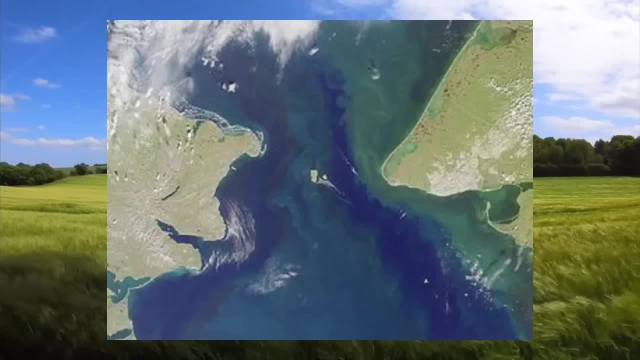 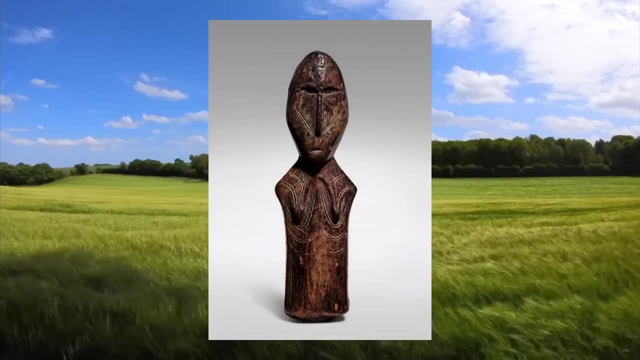 the artistic and technological prowess of its inhabitants. Artistic expression was a hallmark of the Old Bering Sea culture, as evidenced by the skillfully crafted ivory carvings depicting animals, humans and mythological figurines. These carvings served various different purposes, from personal adornment to ritual objects. 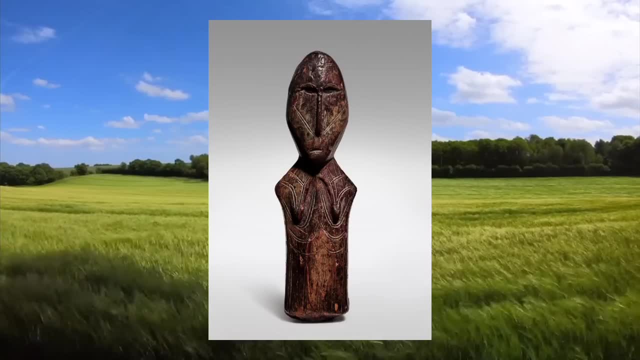 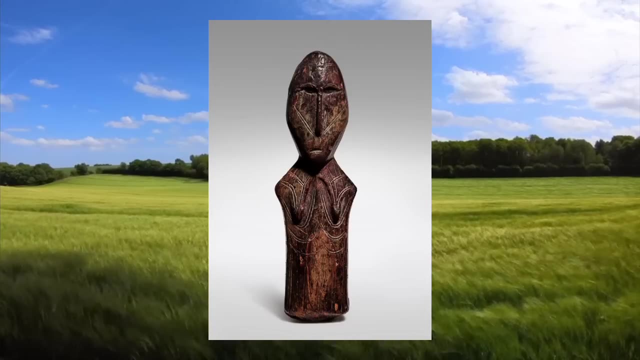 highlighting the cultural significance of art in their society. Substantive strategies were deeply rooted in the culture. The culture was rooted in the coastal environment, with hunting and fishing forming the backbone of their livelihoods. Marine resources, including seals and other mammals, played a vital role in sustaining 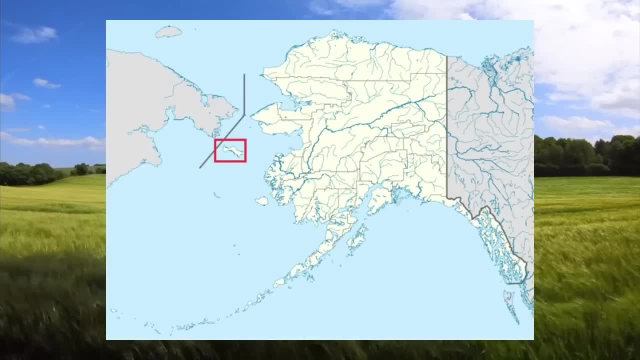 the communities of the Old Bering Sea. Participation in extensive trade networks was another key aspect of the Old Bering Sea culture. The exchange of materials such as ivory, marine shells and other goods contributed to the cultural interactions and the sharing of resources across different arctic regions. 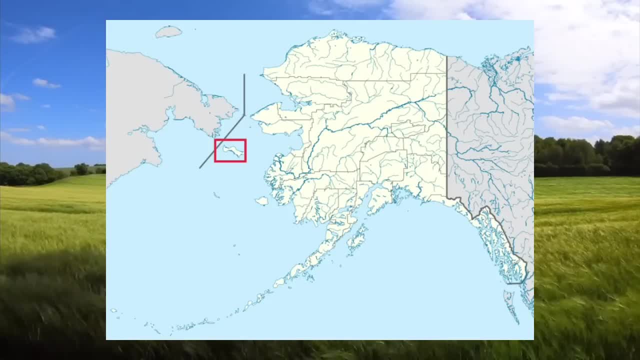 Burial practices of the Old Bering Sea people reflect special and specific cultural traditions, With individuals interred alongside valuable grave goods like ivory, carvings and tools. these artifacts provide archaeologists with valuable insights into the cultural and social dimensions of the society, shedding light on their cultural beliefs and practices. 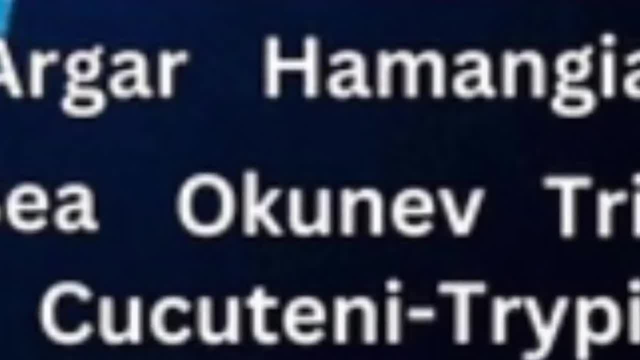 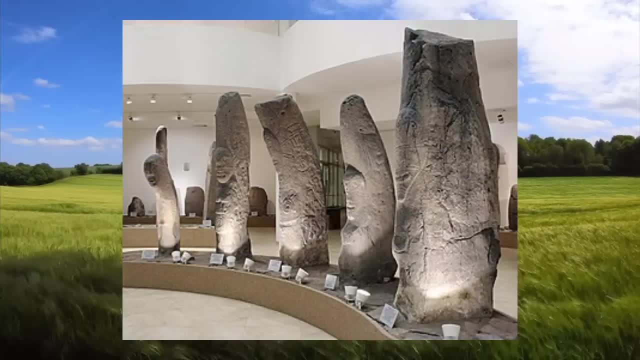 Akhunev. The Akhunev culture, flourishing in southern Siberia during the Bronze Age from the second millennium BCE to the early first millennium BCE, is distinctive for its unique burial practices and artifacts. Typically, Akhunev burials involved the construction of kurgans or burial mounds with the deceased 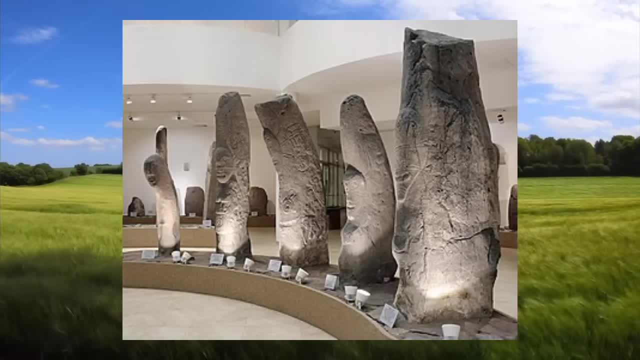 placed in wooden or birch bark. coffins, Grave goods such as pottery, tools and ornaments were often included, reflecting the cultural significance attached to these items In terms of their economy and lifestyle. the Akhunev people engaged in a mixed-substance. strategy combining elements of pastoralism, hunting and gathering. They herded domesticated animals like cattle, sheep and goats, while also relying on hunting and gathering for subsistence. They diversed approach to livelihood. They contributed to their adaptability in the southern Siberian environment. 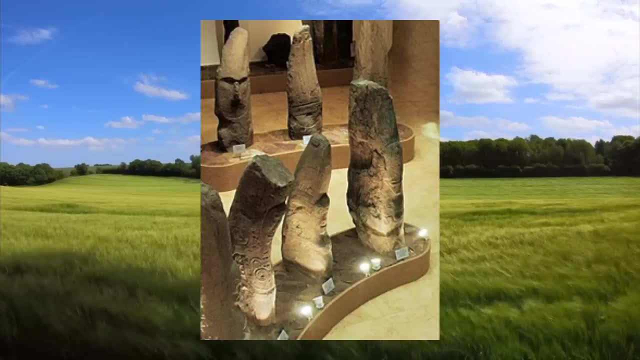 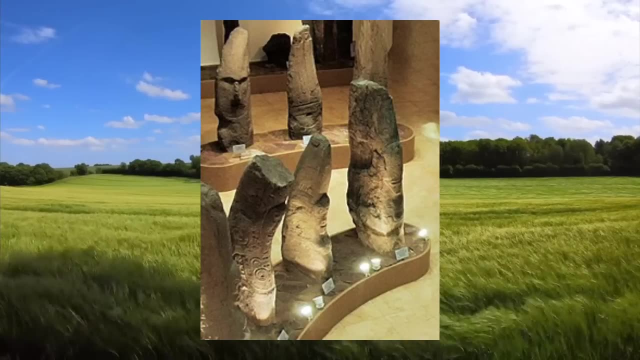 Archaeological findings from Akhunev sites encompass a variety of artifacts showcasing the technological and artistic skills of their culture. Pottery, stone and bone tools, as well as metal objects, provide valuable insights into the material culture of the Akhunev people and their interactions with the surrounding. 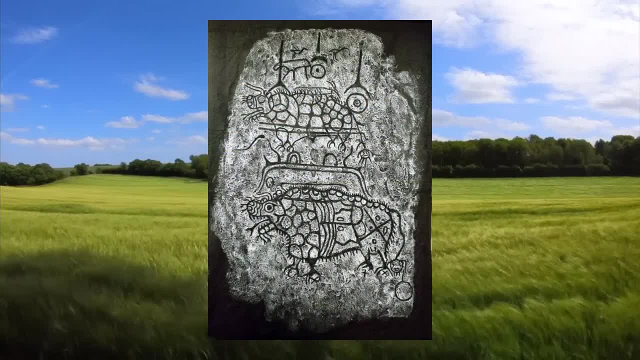 environment. Chronologically, the Akhunev culture is part of the broader Andorov cultural complex, which encompasses various Bronze Age cultures in the Eurasian steppe region. The Akhunev culture predates the Akhunev culture of the Eurasian steppe region. 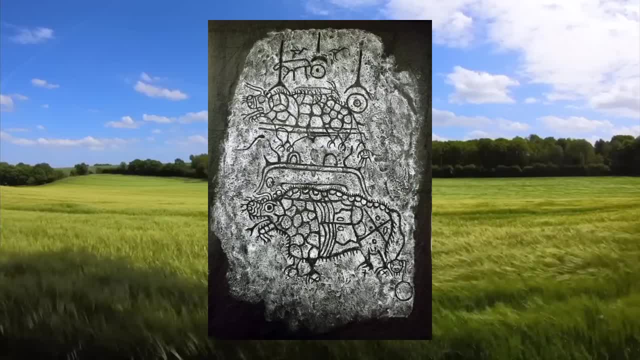 The Akhunev culture predates the Akhunev culture of the Eurasian steppe region. The Akhunev culture is part of a series of cultural movements comprising many of the most well-known cultures, such as the Scythians and the Sarmatians, contributing to our understanding. 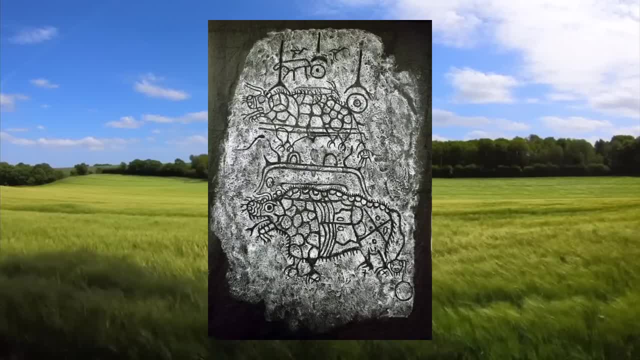 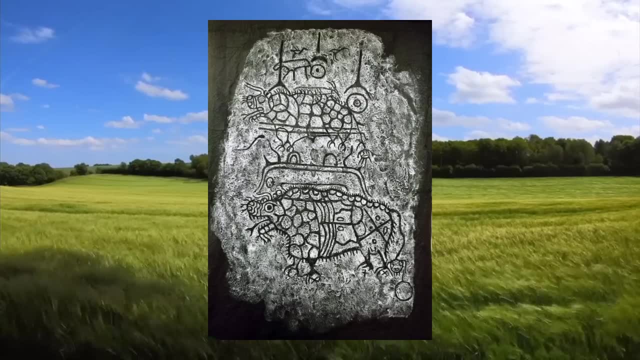 of the cultural evolution and the vast geographical expanse, Archaeological sites associated with the Akhunev culture have been unearthed in the Monastigov Basin of southern Siberia. These sites, ranging from burial grounds to settlements, serve as windows into the daily 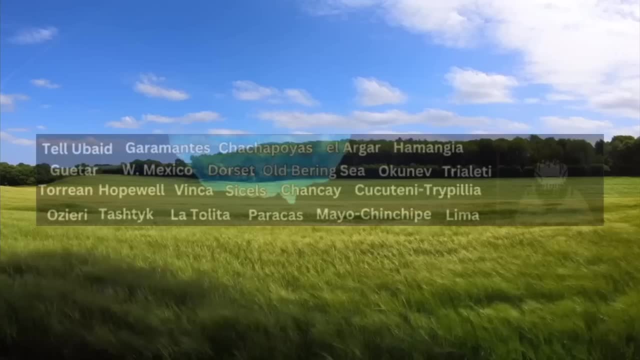 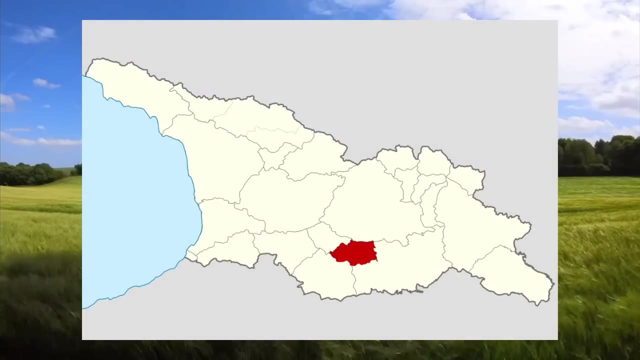 lives and practices of the Akhunev people. 3. Trialedi- Trialedi. the Trialedi culture, spanning from the 3rd to 2nd millennium BCE in the Central and Eastern South Caucasus left an indelible mark on the region's prehistory. 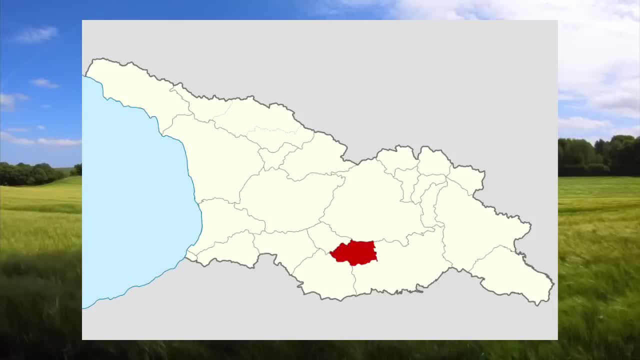 Named after the Trileti region in Georgia. this Bronze Age culture is characterized by its fortified settlements strategically perched on elevated sites. Defensive walls and towers at these locations suggest a degree of social organization and perhaps a need for protection. The material culture of the Trileti people is distinct, featuring pottery with specific 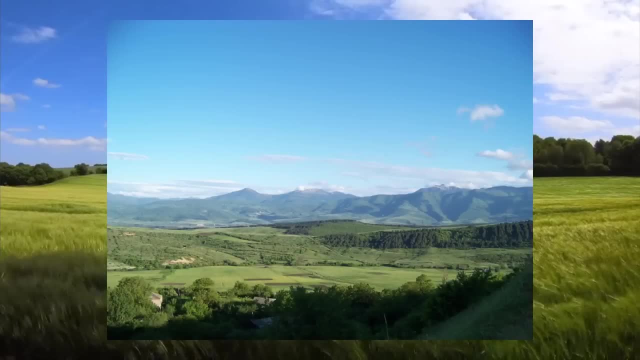 shapes and different decorations, along with an array of metal artifacts, including tools, weapons and personal ornaments. This technological and artistic prowess showcases the sophistication of the Trileti culture. A significant aspect of Trileti life was the metalworking, particularly in the bronze department. 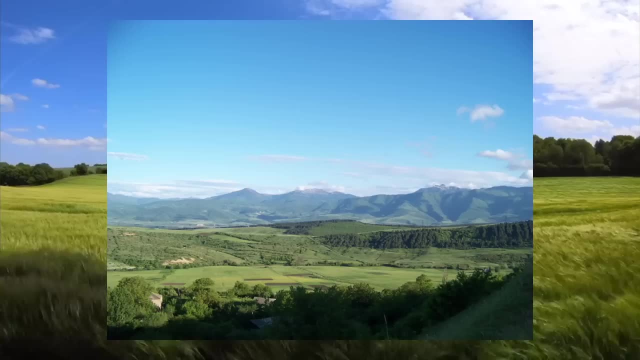 The presence of well-crafted bronze objects indicates the importance of metallurgy possibly playing a role in trade networks and exchanges with neighboring cultures such as the Kura-Arax culture. Participation in trade networks is indeed a likely aspect of Trileti culture fostering. 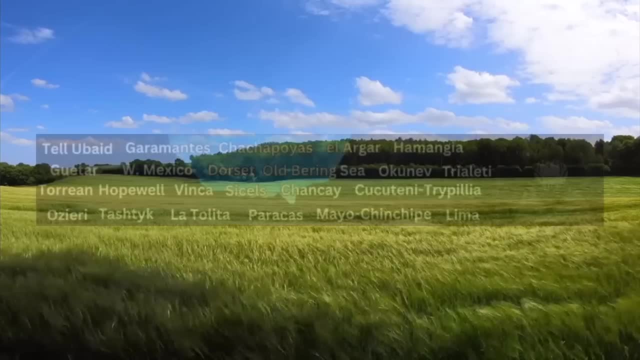 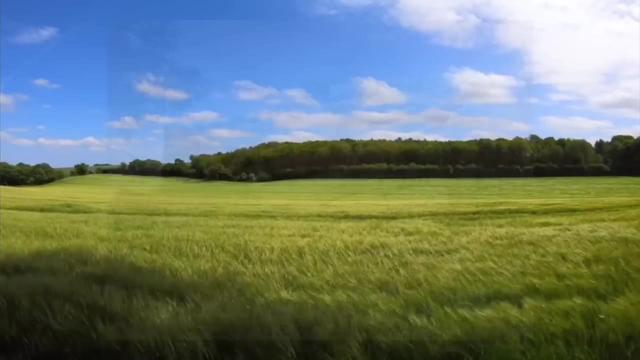 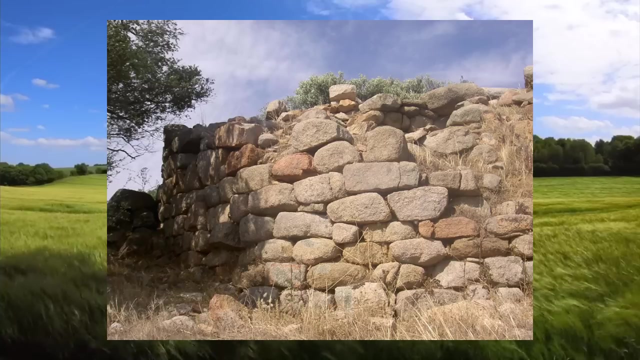 interactions and cultural influences. The Trileti culture is known for its prominence during the Middle Woodland period in eastern North America, which was around 100 BCE to 500 CE, just for reference, was characterized by distinctive ceremonial and artistic practices. One of the most notable features of the Hopewell tradition was extensive trade networks that 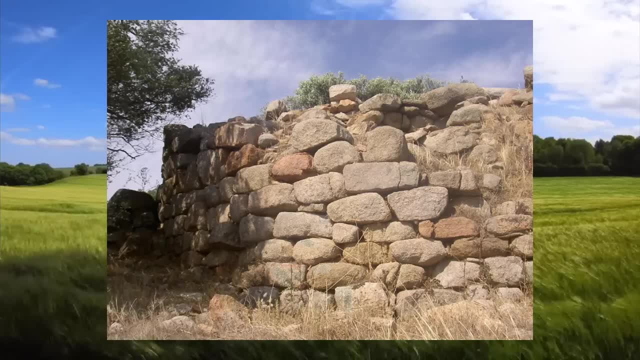 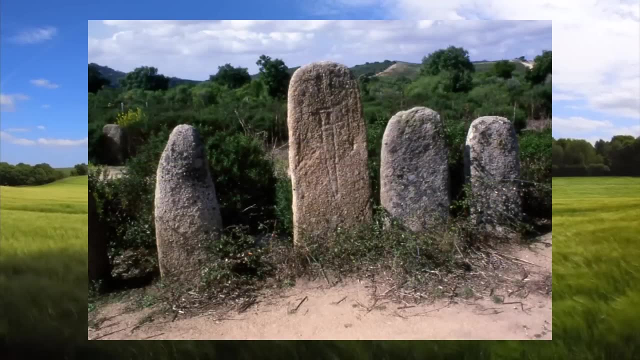 connected various different regions. Materials such as exotic minerals, shells and other different goods were exchanged over pretty long distances, indicating complex social interactions. The artistic achievements of the Hopewell people were evident in the elaborate burial mounds they constructed. These mounds often contained intricate burial offerings, including finely crafted artifacts. 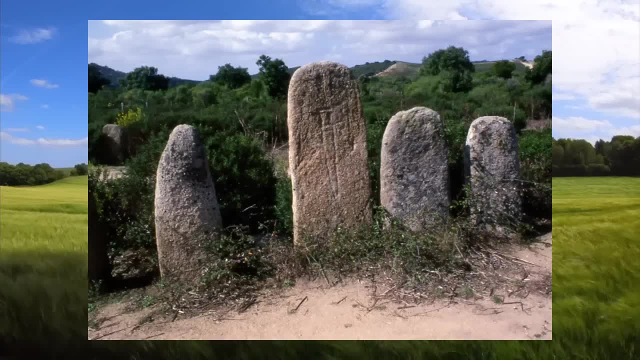 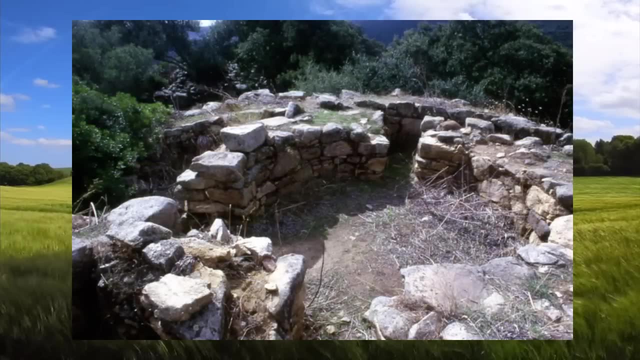 and objects made from exotic materials. The Hopewell also exchanged in the construction of geometric earthworks such as the famous octagon and circle at Newark Earthworks in Ohio. The decline of the Hopewell culture is not fully understood, but factors such as environmental 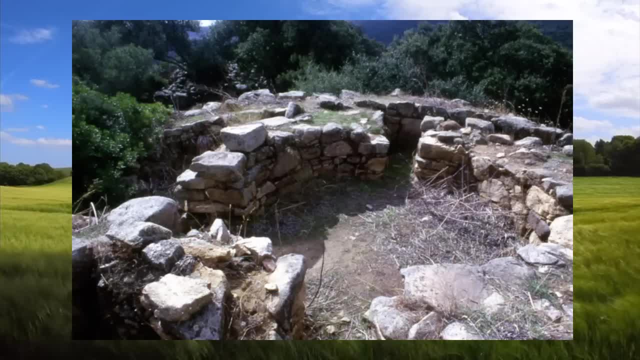 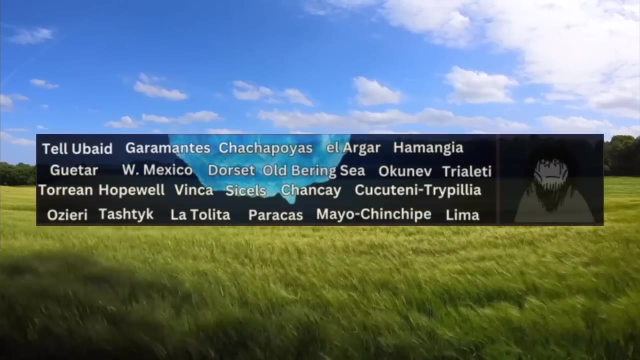 changes, shifts in social discipline and the use of materials such as metals, materials, materials and materials are all important. The legacy of the Hopewell tradition is significant in understanding the diversity and complexity of North American cultures in North America, particularly during the Middle Woodland period. 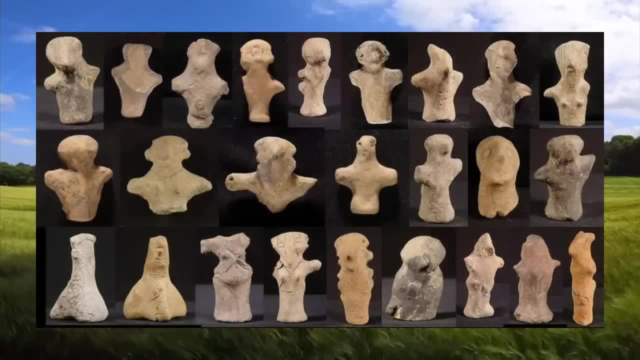 Vinca. The Vinca culture spanned from approximately 5,700 to 4,500 BCE in the central and western Balkans. It represents a pivotal Neolithic civilization in Southeast Europe, Noted for its well-organized settlements, some evolving into complex urban centers. 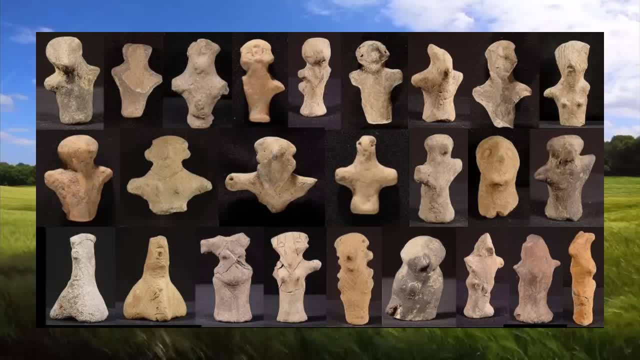 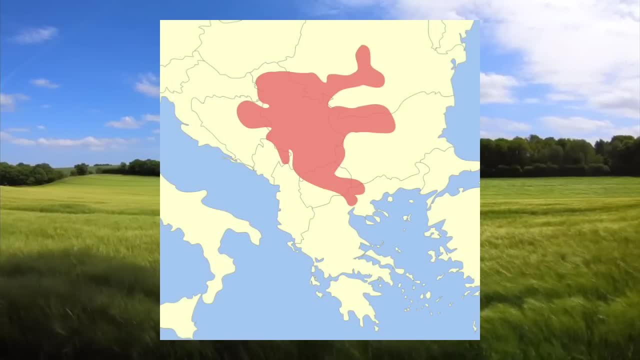 and Vinca communities exhibited advanced architecture with rectangular houses and public structures. A hallmark of the Vinca culture is its distinctive pottery adorned with intricate patterns, including geometric designs and depictions of different animals and humans in the activities they did. This reflects a highly developed ceramic industry. 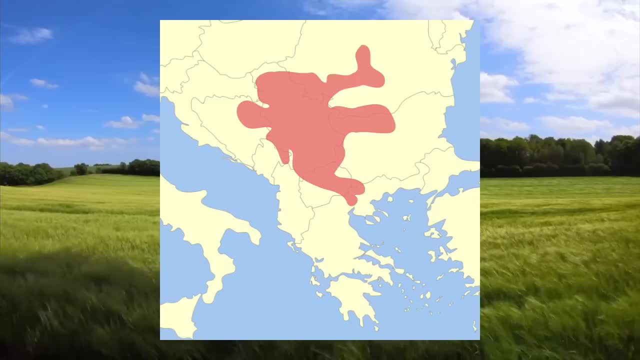 The economy of the Vinca people centered on agriculture, The Vinca culture, and animal husbandry, cultivating crops like wheat, barley, peas and lentils, and domesticating cattle and pigs and sheep. Artifacts from the Vinca culture comprise diverse materials, including stone bone. 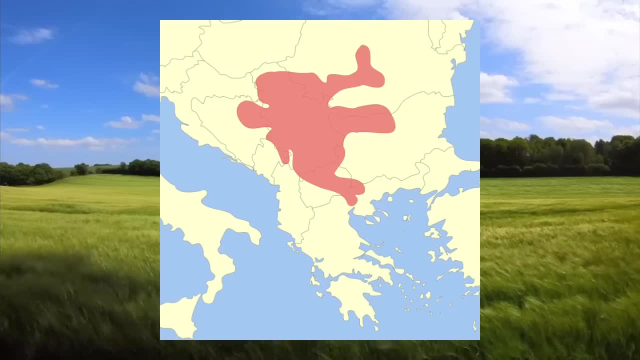 and clay. These items serve various different purposes, ranging from tools and implements to figurines and ritual objects. Notably, the Vinca script, a system of symbols found on certain artifacts, remains enigmatic and no one really knows how they are fully deciphered. 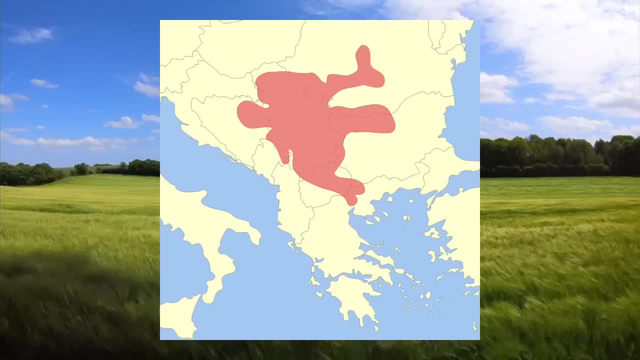 And I don't think they'll ever be fully deciphered. The Vinca people are known for their ingenuity. The Vinca people engaged in trade and neighboring cultures, exchanging goods and raw materials. Evidence also suggests cultural interactions with contemporary civilizations in Europe. 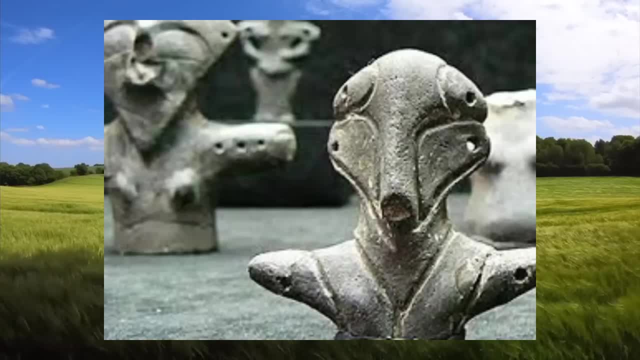 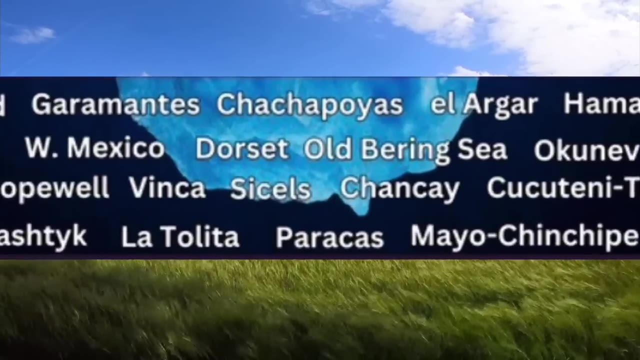 and the Near East. Despite its significance, the decline of the Vinca culture remains unclear and unknown, and people think it disappeared because of shifts in substance, strategies or interactions with other cultures possibly contributing to its eventual disappearance. Sissels- The Sissels, an ancient Italic people, left a 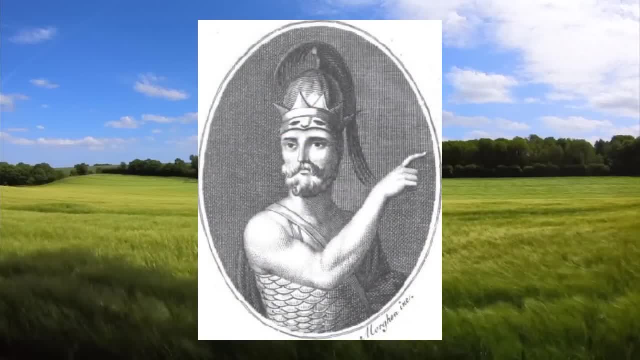 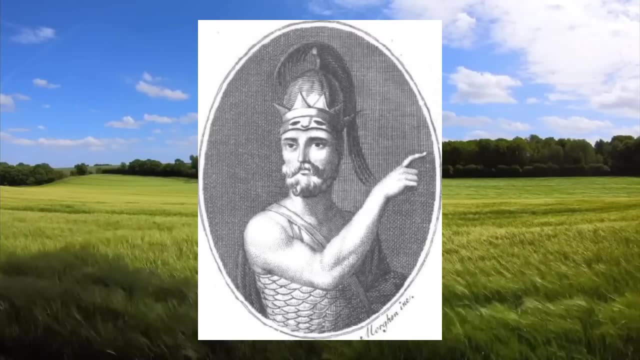 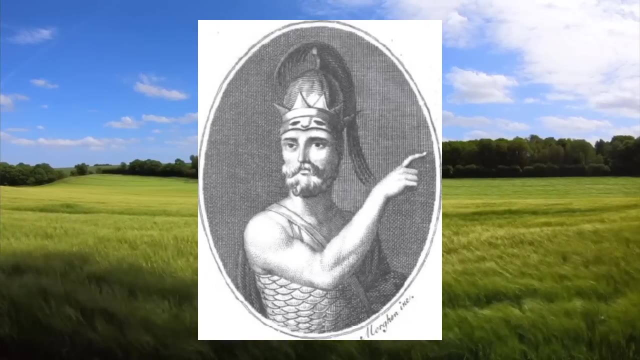 significant imprint on the history of Sicily. Thought to have migrated from the Italian mainland, possibly regions like Calabria or Apulia, the Sissels settled in eastern and central Sicily alongside the Sissian and Elamites. Their hilltop villages, fortified for defense, became characteristic of their settlements. 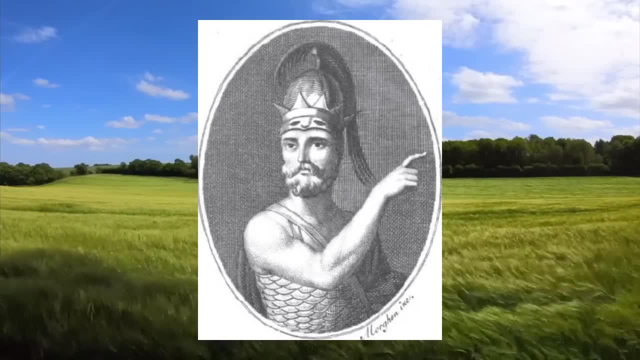 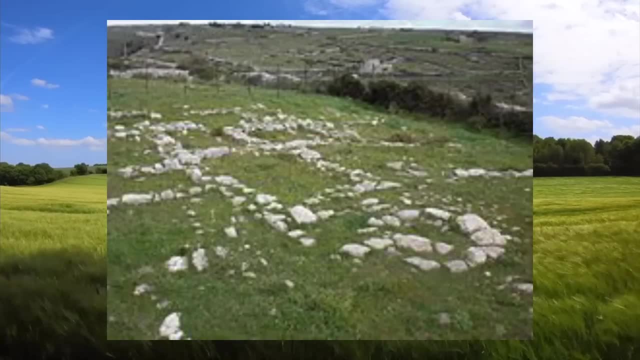 reflecting an agricultural and pastoral way of life. Distant in culture, the Sissels were not isolated from the influences of neighboring people, particularly the Greeks. The 8th and 7th century BCE saw interactions and conflicts between the Sissels and Greek colonists contributing. 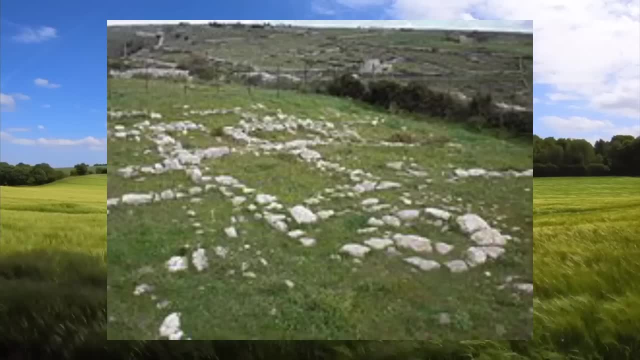 to the blending of cultures. Over time, the Sissels adopted elements of Greek culture and language, leading to a gradual assimilation. The historical references to Sissels can be found in different writings, such as those by the Thessalites, shedding light on their presence and the interactions in ancient Sicily. 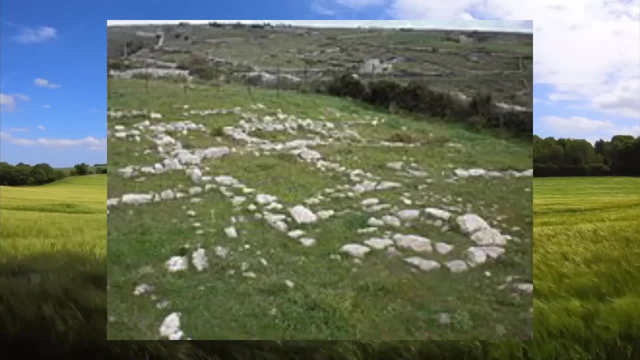 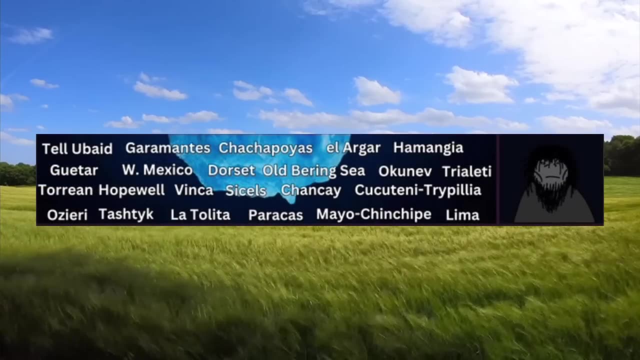 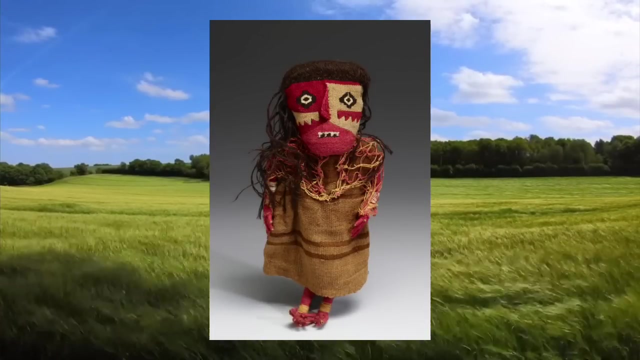 as part of the larger tapestry of all of Sicilian history, The Sissels played a role in the island's evolution into a diverse cultural melting pot. 9. Chanque: The Chanque culture, flourishing on the central coast of Peru from 1000 to 1470 CE, left a. 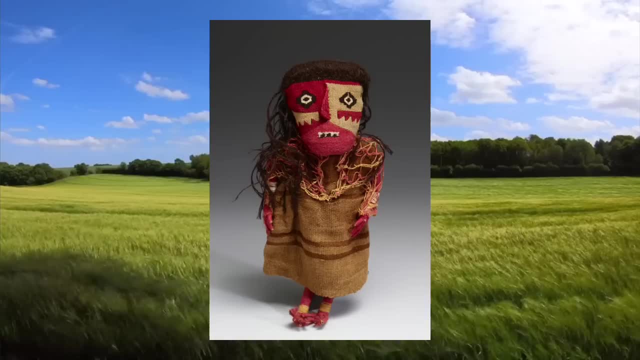 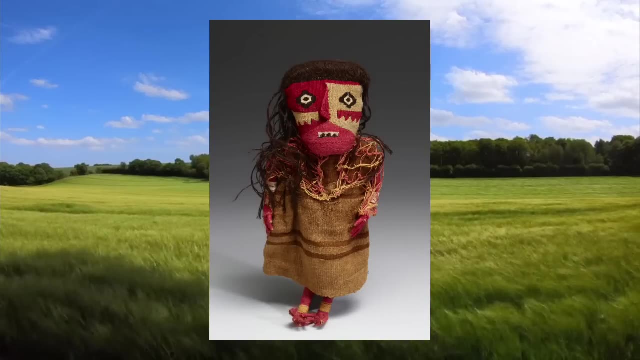 mark with its distinctive art textiles and burial practices. Renowned for their exceptional weaving skills, the Chanque people produced intricate textiles featuring elaborate designs like geometric patterns, animals and human figurines. Their textiles, considered among the finest in ancient Peru, attested to the sophistication 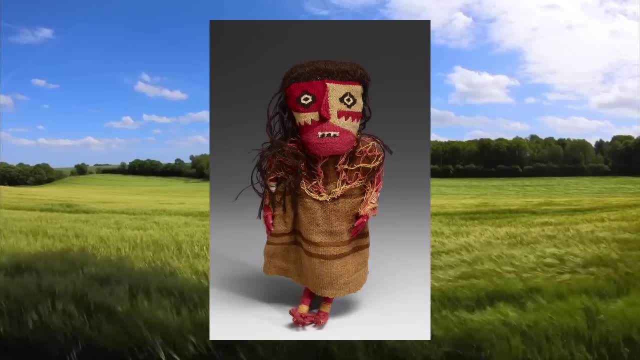 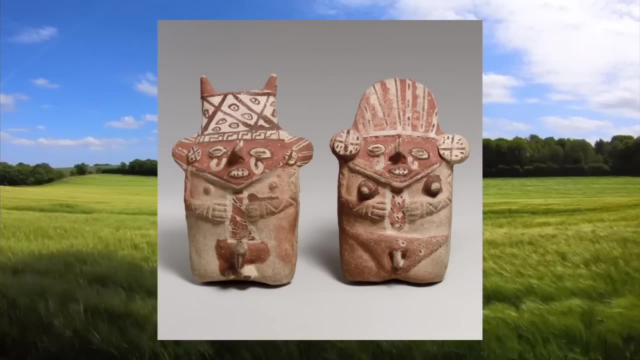 of Chanque craftsmanship In the realm of ceramics. the Chanque culture exhibited a unique style characterized by a polychrome decoration with painted or incested designs. These ceramics adorned with motifs or stylized animals, humans and mythological beings. 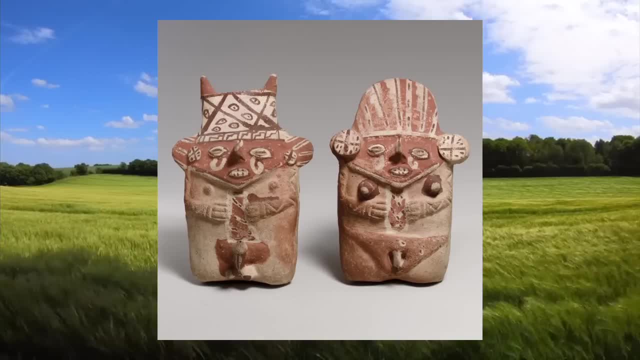 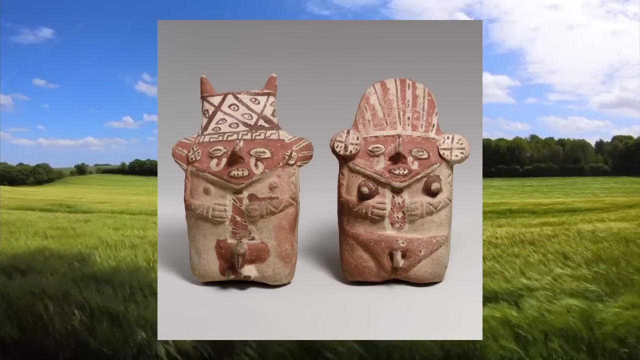 served both utilitarian and ritualistic purposes. One of the most distinctive aspects of the Chanque culture was its burial practices. The deceased were placed in flexed positions and enveloped in finely woven tiles forming burial bundles or fardos. These bundles contained an array of offerings, including pottery, textiles and personal. 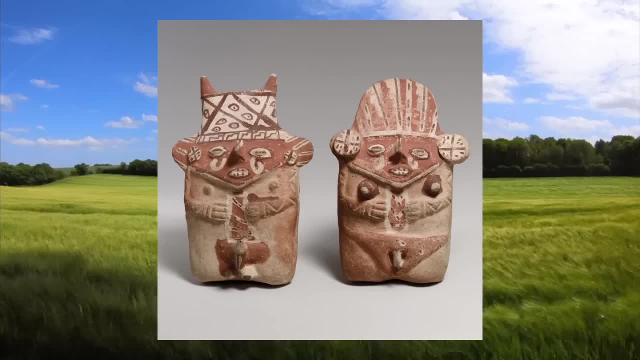 items Emphasizing the cultural significance of ritual and symbolism in Chanque society. evidence suggests a complex social structure within the Chanque culture, featuring social hierarchies and elite classes. Burial sites where elaborate goods and grave goods point to distinctions within the community. 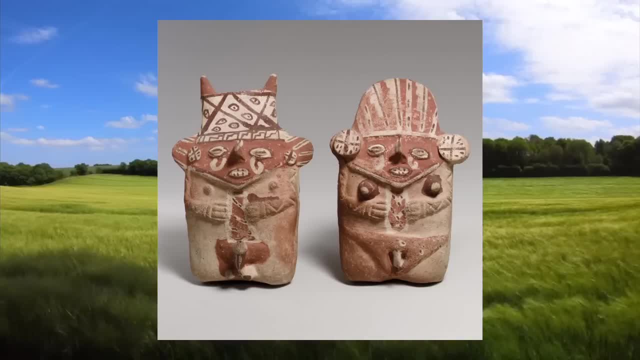 Geographically situated on the coast, the Chanque people engaged in trade and interactions with neighboring cultures, facilitating the exchange of goods and ideas. The decline of the Chanque culture coincided with the assimilation into the expanding Inca Empire. Factors contributing to the decline include the destruction of the Inca culture, the 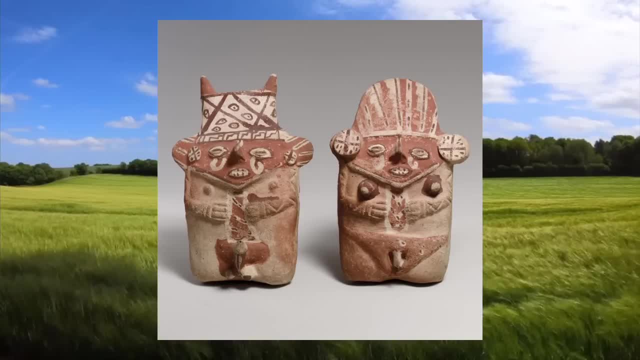 spread of the Inca civilization, the rise of the Inca nation and the rise of the Inca culture itself. The rise of the Inca culture may have included environmental changes, shifting social dynamics and the expansion of the Inca Empire. 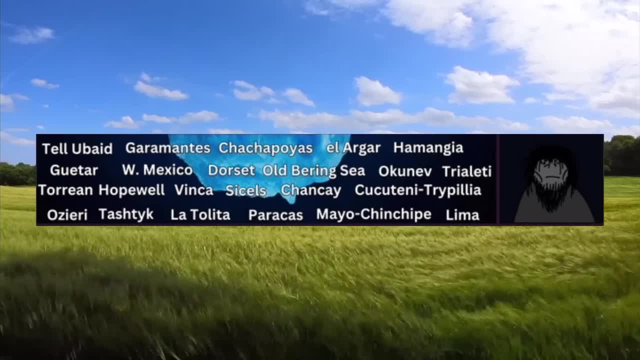 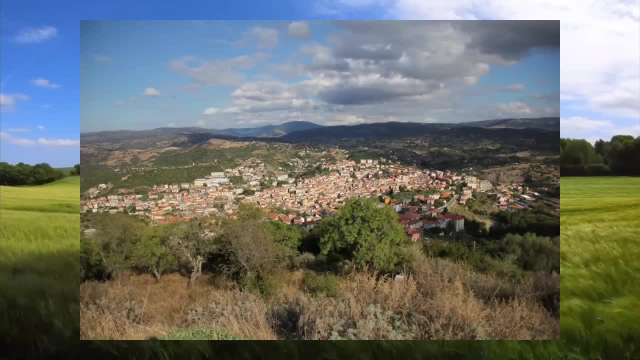 2. OZIRIE. The Ozeri culture flourishing on the island of Sardinia during the late Neolithic period from around 3500-2700 BCE is a significant chapter in the prehistory of the region, Named after the town of Ozeri, where key archaeological discoveries were made. this culture left a 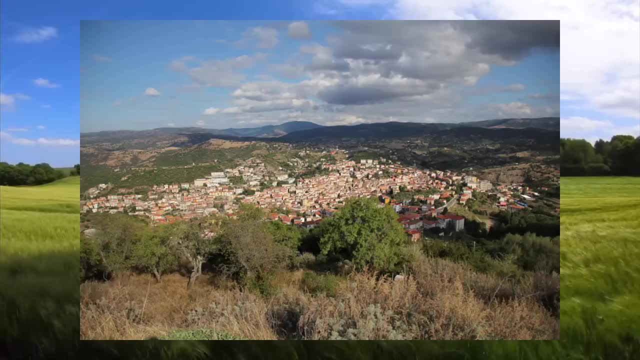 distinctive mark on Sardinia in the first half of the 18th century. 7. ancient landscape. Osiri settlements were characterized by stone structures, including circular huts, strategically positioned on hills or near water sources. The people of Osiri are particularly renowned for their elegant and intrinsically decorated. 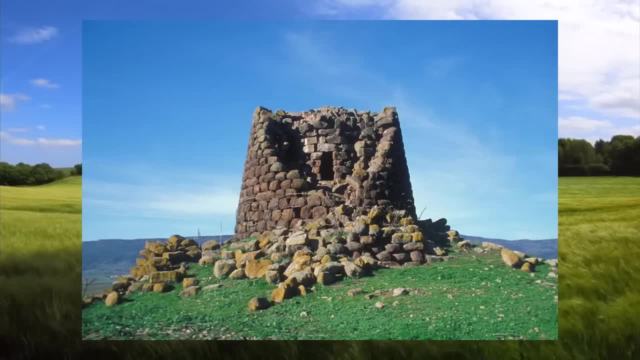 pottery. The ceramics feature a variety of different motifs, including geometric patterns, zoomorphic figurines and human representations, often adorned with red and black pigments, showcasing the artistic prowess of the culture. Art and symbolism played a vital role in the society, evident in artifacts like statuettes and sculptures depicting humans and animals. 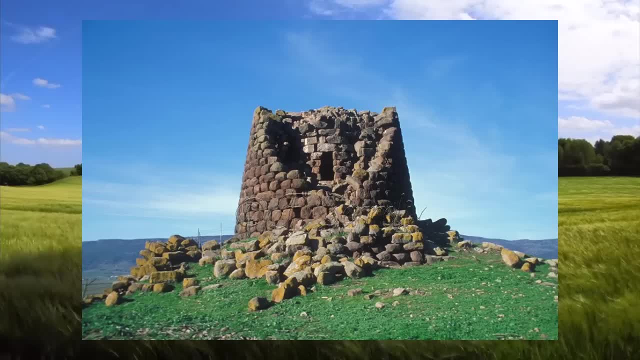 These items are believed to have held symbolic or religious significance, providing a glimpse into the spiritual dimensions of the people. Burial practices of the culture included both inhumanitions and cremations, with grave goods interned alongside the deceased. These goods, ranging from pottery to tools and personal ornaments, offer valuable insight into the 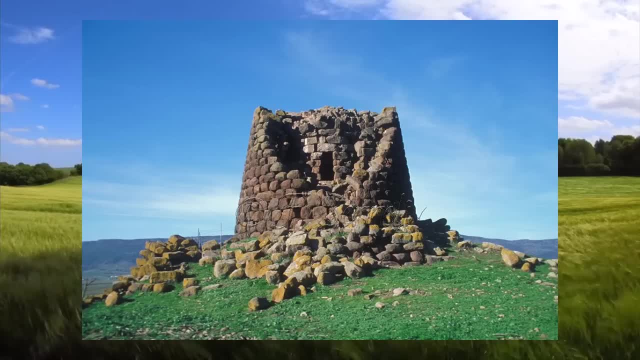 material culture in the daily life of the Osiri people. The economy of the Osiri culture was based on the combination of the culture of the people of Osiri and the culture of the people of Osiri. The Osiri culture was based on the combination of agriculture. 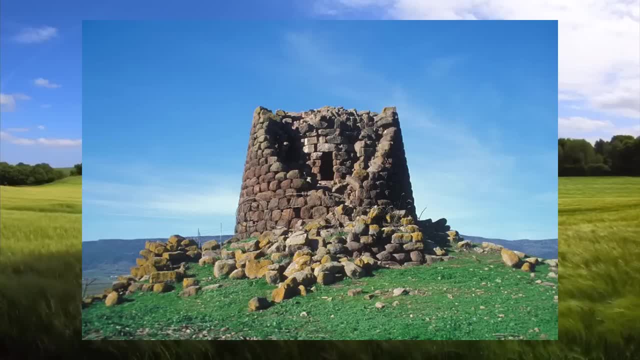 animal husbandry and fishing. They cultivated crops such as wheat and barley and domesticated animals like cattle and sheep, reflecting the diversified and sustainable strategy of the economy. Overall, the Osiri culture represents an important phase in Sardinia's prehistory. 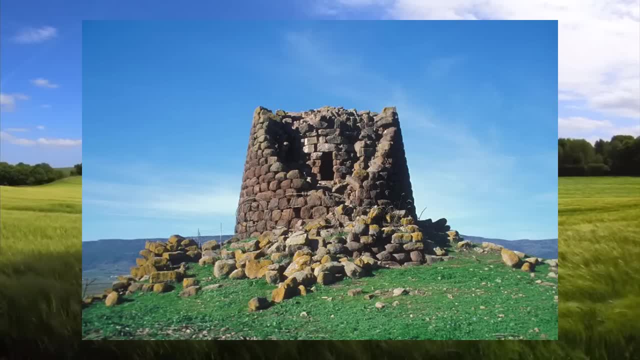 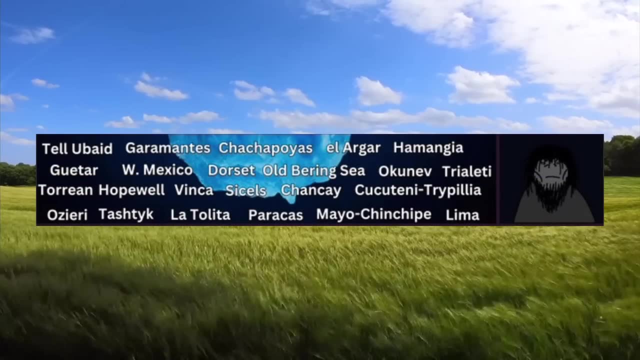 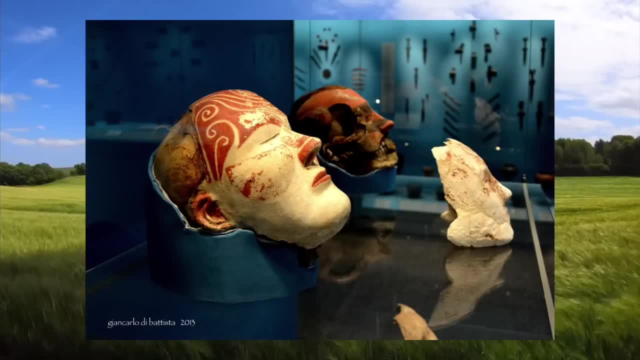 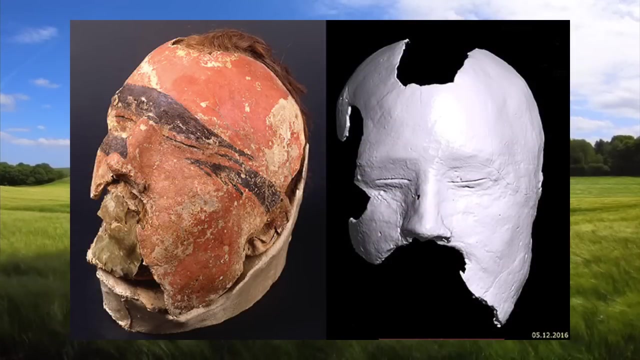 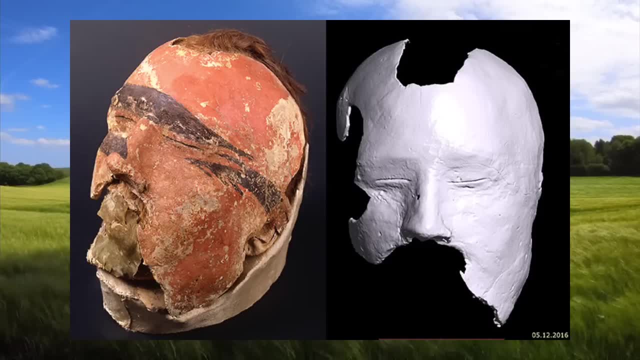 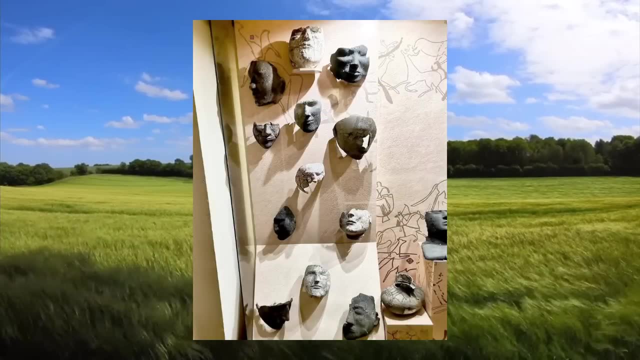 Tashdik, Tashdik, Tashdik: adaptability of detachment people to their environment. Situated in the basin, a crossroads for various cultures, detachment culture was likely influenced by and engaged in trade and cultural exchanges with neighboring societies. The region served as a nexus connecting different 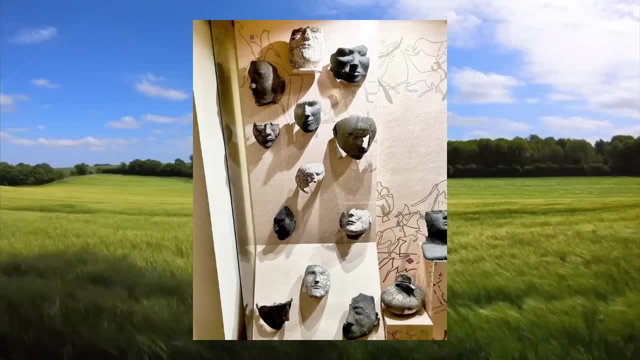 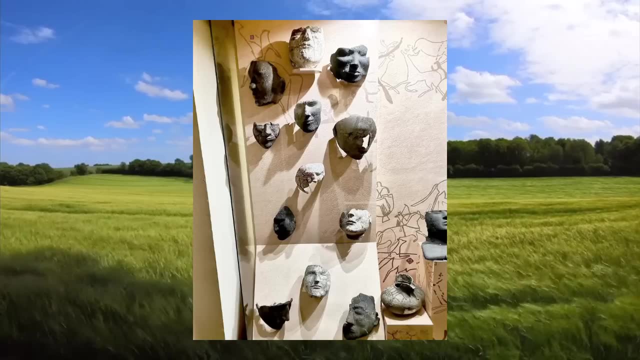 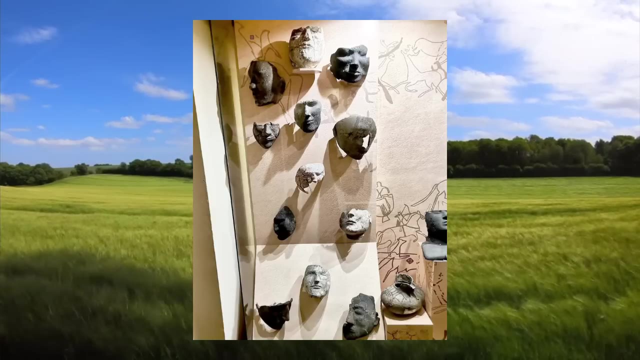 communities, fostering interactions and the exchange of goods and ideas. The decline of detachment culture remains a subject of inquiry and debate, with various different factors potentially contributing to its disappearance and decline, which were environmental changes, migrations of animals that just changed it up, and interactions with other cultures. 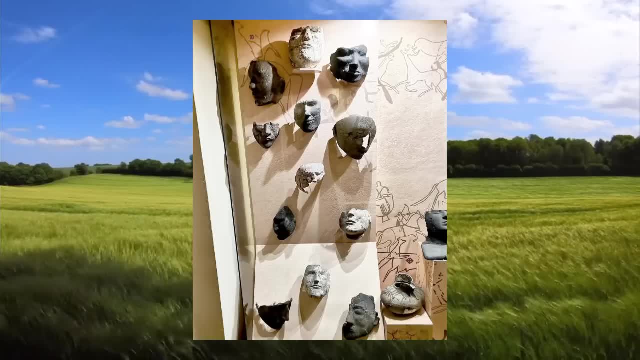 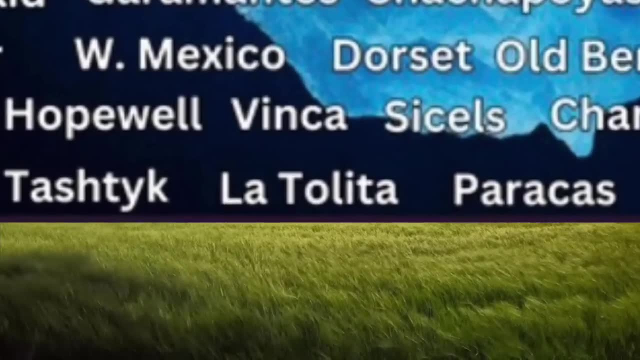 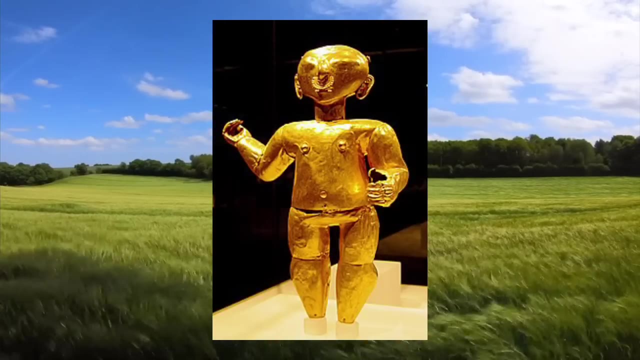 are among the possible explanations of this eventual decline of the distinctive Iron Age culture, La Tolita. The La Tolita culture, flourishing along the Pacific coast of present-day Ecuador from approximately 600 BCE to 200 CE, is the single's first remarkable artistic achievements. 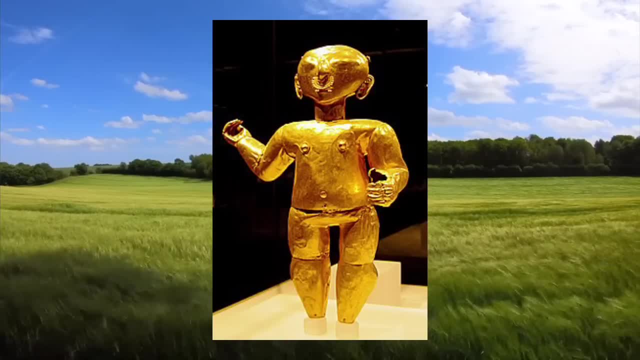 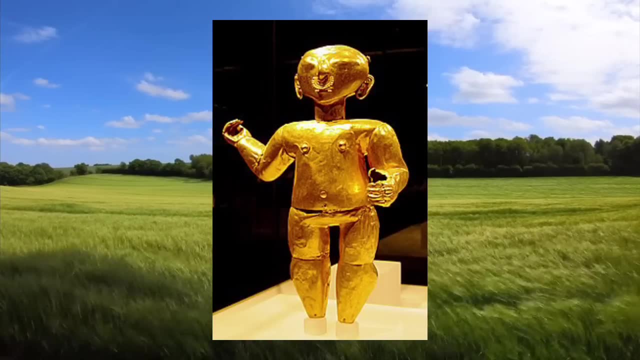 particularly in pottery and gold work, Skilled ceramics within the La Tolita culture, crafted by the La Tolita culture and the La Tolita culture of the La Tolita culture of the Pottery, adorned with intrinsic designs featuring stylized representations of human and animal. 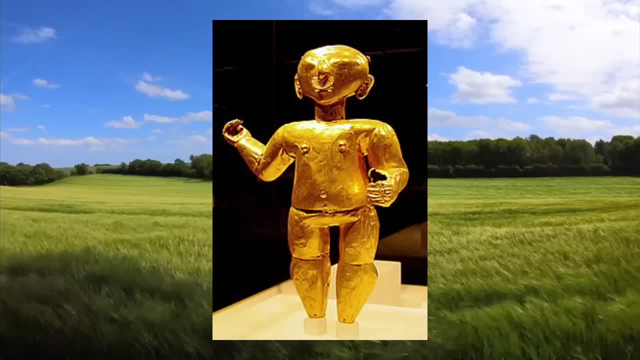 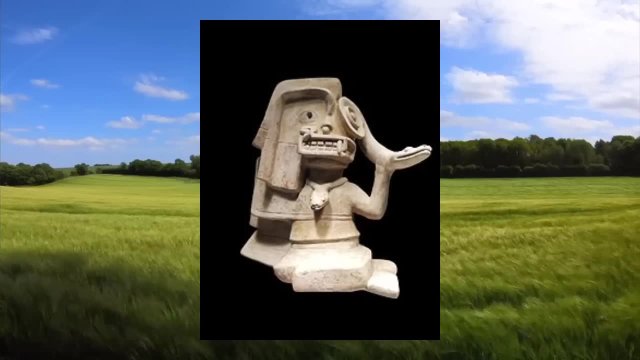 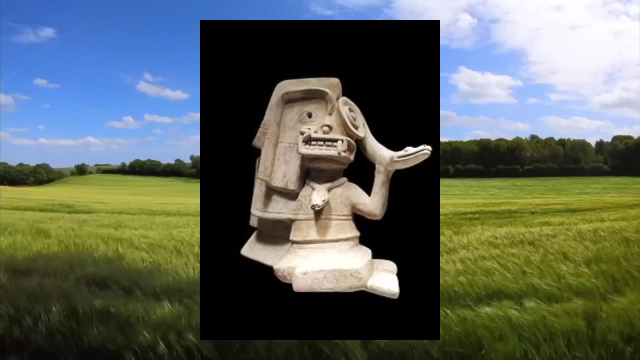 figures, The meticulous incisions and painted decorations of the pottery reflect a high level of artistic sophistication. One of the most hallmarked features of the La Tolita culture is its mastery of gold work. Artisans created exquisite gold artifacts, including jewelry, figurines and ceremonial objects. These items showcased not only the exceptional 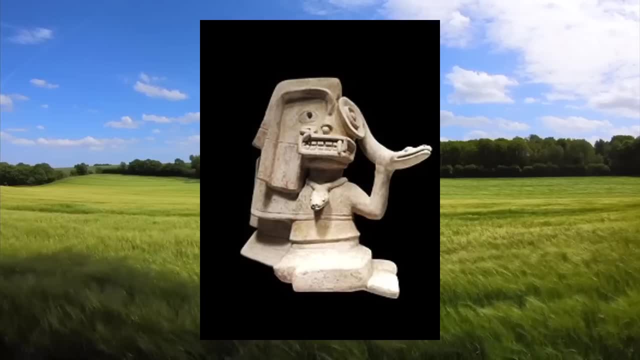 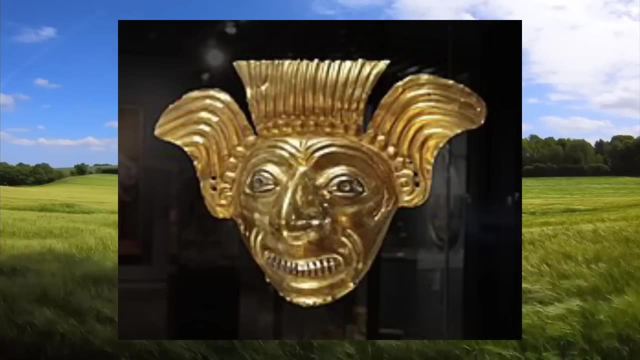 craftsmanship of the society, but also intricate iconography, often depicting animals and mythological beings. The presence of such gold items suggested social complexity, potentially tied to elite or ritualistic activities within La Tolita society. La Tolita engaged in extensive trade networks interacting with neighboring cultures along the Pacific coast. 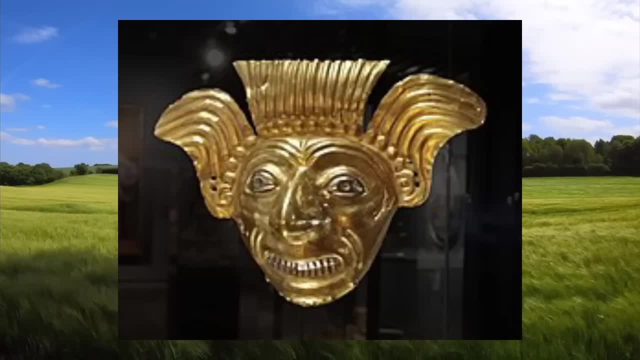 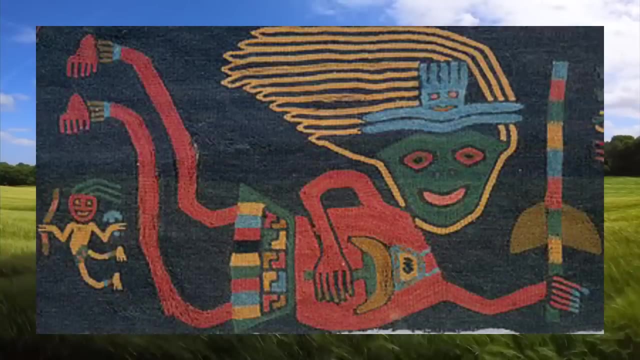 and likely participating in broader trade routes. The exchange of goods, including ceramics and gold items, facilitated cultural diffusion and contributed to the richness of artistic traditions in the region. Paracas- The Paracas culture, thriving on the arid southern coast of Peru from approximately 800 BCE to 100 BCE. 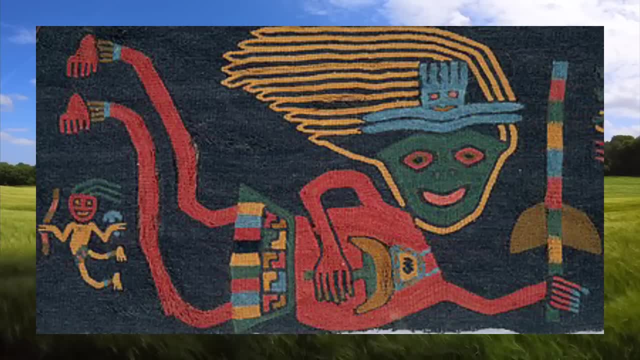 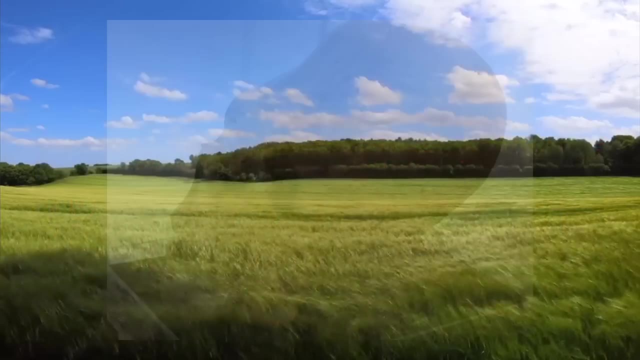 stands out for its exceptional artistry and cultural practices. Foremost among its achievements are the renowned Paracas tiles, Considered among the finest in the ancient Andean world. master weavers employed intricate techniques such as embroidery and tapestry to create textiles featuring vibrant colors and elaborate designs, often depicting animals and mythological 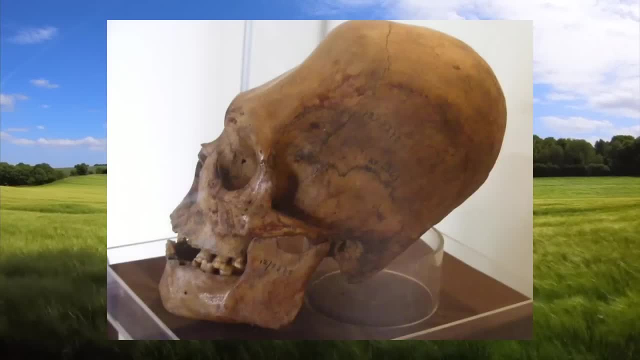 figurines. Elaborate burial practices are a hallmark of the Paracas culture. The Paracas culture is a culture of the deceased. wrapped in multiple layers of finely woven textiles, These burial bundles serve both practical and symbolic purposes, offering protection to the deceased and acting as 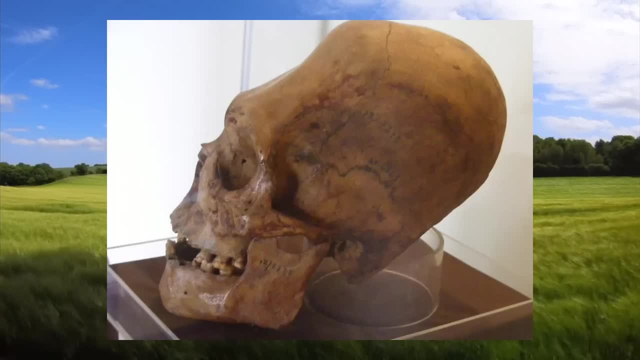 significant markers of identity or social status to the dead. Paracas ceramics, characterized by stylized depictions of animals and humans, displayed a high level of craftsmanship. The use of polychrome techniques employed multiple covers and enhanced the visual appeal of the pottery. The Paracas region is also known for the geoglyphs- large-scale ground dwellings. 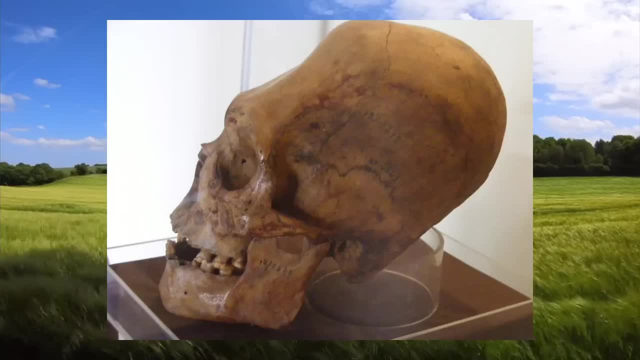 and the use of crafts such as carvings. In the early 18th century, the Paracas culture was considered to have ritual or ceremonial significance. Cranial deformation was another distinctive practice among the people, shaping the skulls of infants to achieve elongated forms. 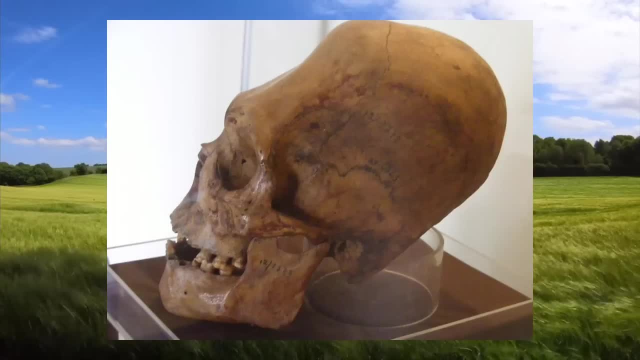 This practice, along with the intricate textiles, played a role in signaling social identity and status within the community. The Paracas culture, situated along the coast, had a strong connection to maritime activities, fishing and marine resources and the Paracas culture, as it was the only other Native language to be used to describe the Paracas culture. All of this 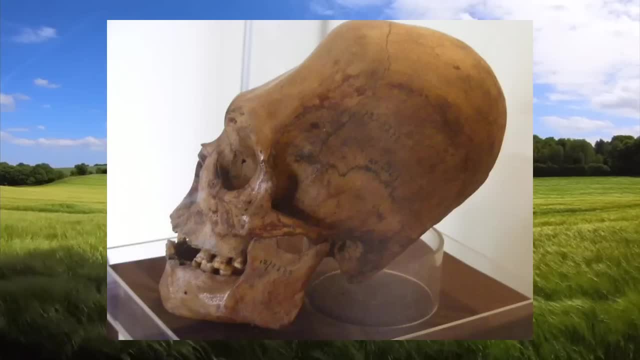 resources were integral to their community and daily lives. Over time, the Paracas culture gave away to the Nazca culture in the same region, making a transition to the cultural and artistic transitions of the area. The enduring legacy of the Paracas culture lies not only in its unique 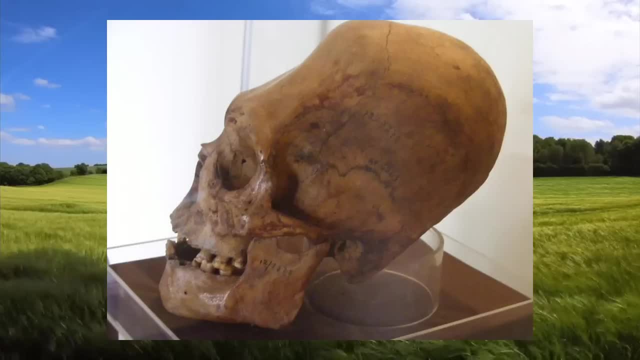 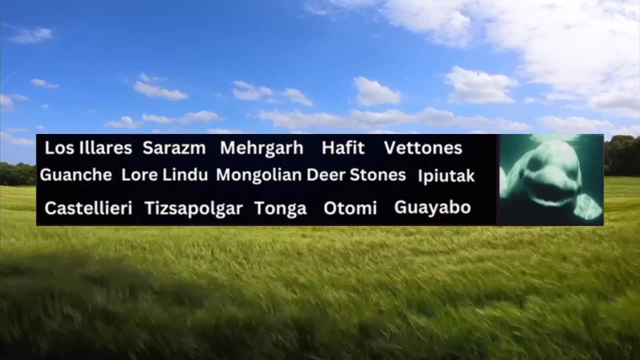 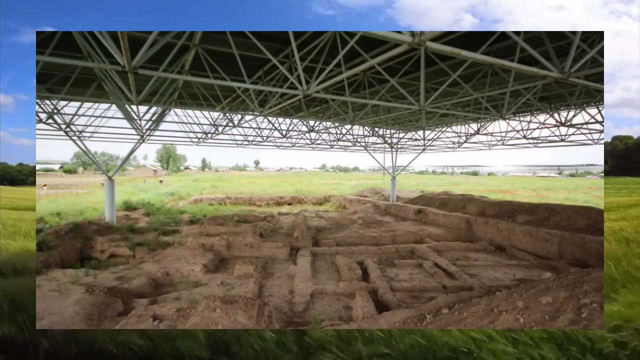 artistic expression, but also in the archaeological insights gained from the Paracas necropolis and surrounding sites. Alright, now onto tier 7, starting off with Sarazim. Sarazim, situated near Panadrek in Kazakhstan, stands as one of Central Asia's oldest known settlements. Dating. 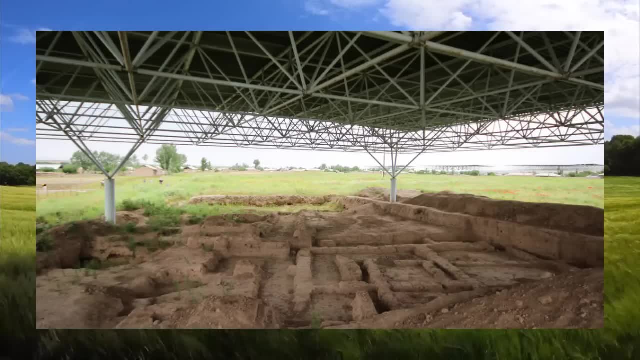 all the way back to 4th millennium BCE. this archaeological site, occupying an area of approximately 100 hectares, is celebrated for its status as a proto-urban or early urban center, showcasing advanced organization and complexity for its time. The settlement was inhabited from: 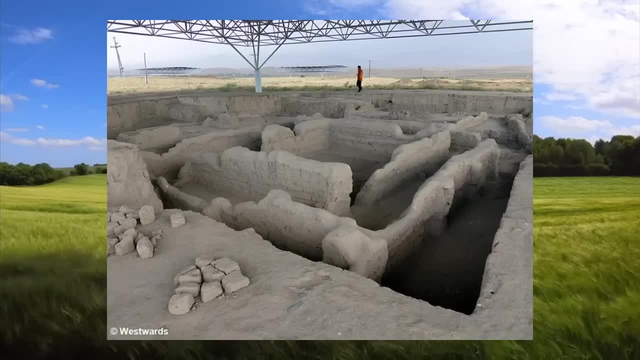 around 3500 BCE to 2000 BCE. The urban plan of Sarazim reveals a well-organized layout with distinct quarters encompassing residential areas and a large number of buildings, The residential areas, public spaces and specialized structures. This early urban center provides a 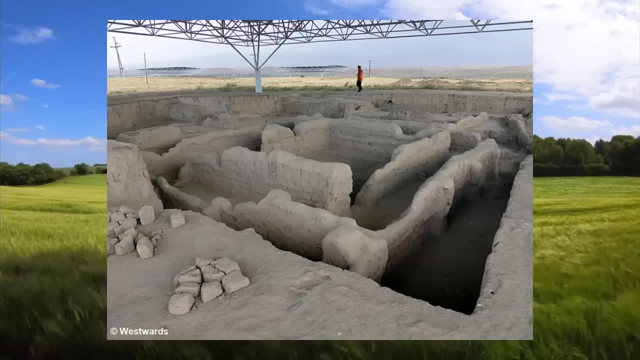 glimpse into the sophistication of societal structures during this period. Excavations at Sarazim have unearthed a rich array of artifacts, including pottery adorned with distinctive red and black designs, as well as tools and ornaments. Sarazim's significance extends beyond just its local context, indicating early cultural exchanges in Central Asia. The site 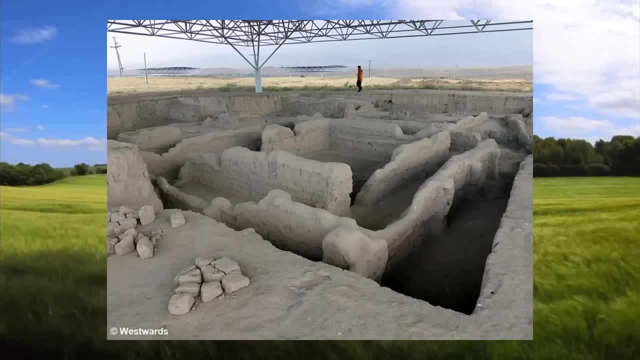 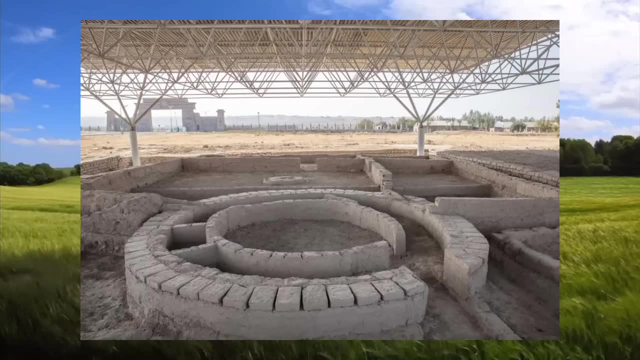 reflects evidence of interactions with neighboring regions, suggesting a network of trade and cultural contacts. Sarazim is one of the most important cultural sites in the region, and the site is a historical landmark that contributes to the diversity of the settlement. Agricultural practices were fundamental to the community's sustenance, with inhabitants cultivating crops. 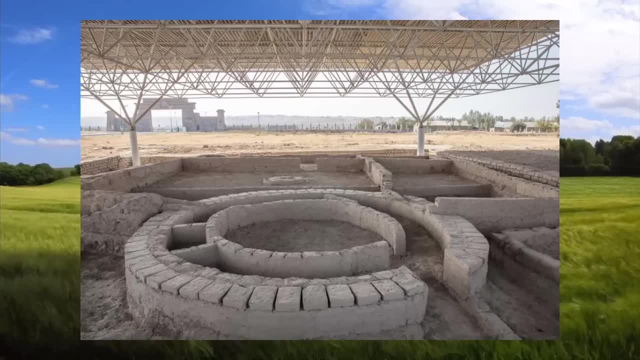 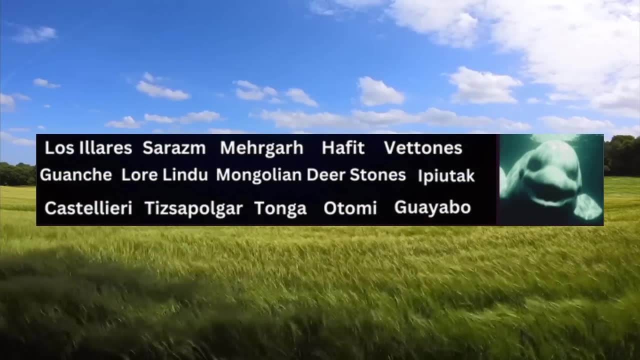 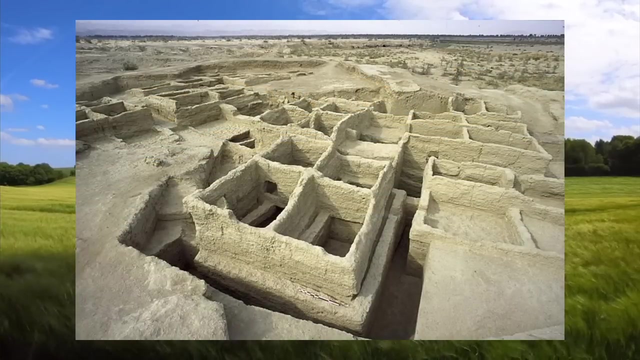 such as barley wheat and various fruits. The proximity of Sarazim to the Zamfri River likely played a pivotal role in supporting successful agricultural activities. Megarth Megarth, situated in the Biolo-Christian province of Pakistan, stands as a pivotal archaeological site that provides crucial insights into the very early 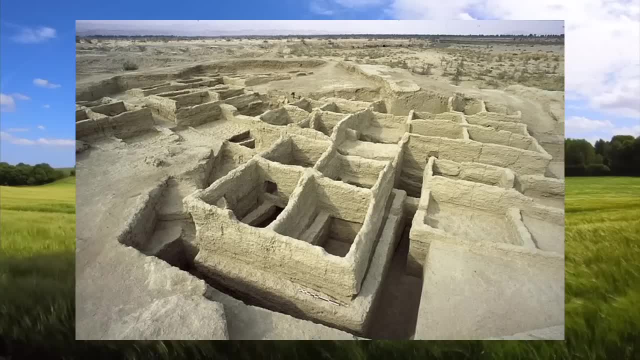 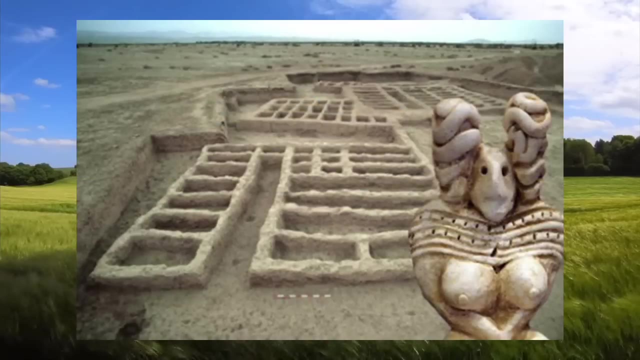 human settlement and agricultural practices in South Asia. occupied from around 7000 BCE to 2000 BCE, Megarth represents a significant transitional period from a nomadic, hunter-gatherer lifestyle to settled agricultural communities. At Megarth, the inhabitants embraced a Neolithic lifestyle. 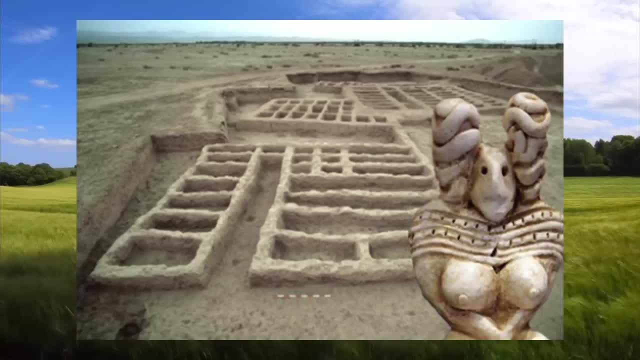 marked by the domestication of plants and animals. The cultivation of crops such as wheat and barley, alongside the herding of sheep and goats, demonstrated a groundbreaking shift in human socioeconomic practices. The settlement features mud brick structures indicative of settled life, and the distinctive pottery discovered at the site showcases advanced craftsmanship. 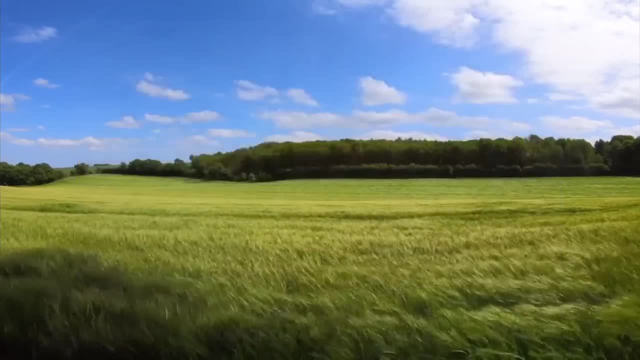 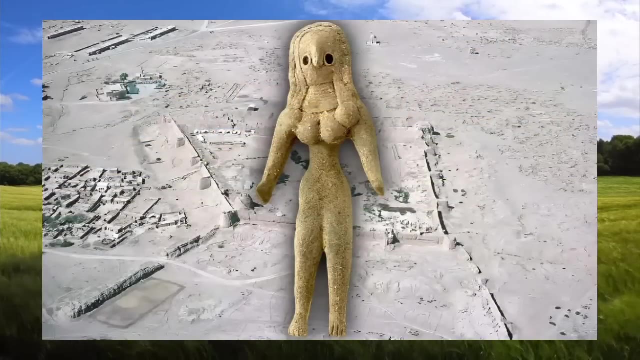 and unique designs. Excavators at Megarth have unearthed a well of artifacts, including tools, ornaments, figurines and pottery. The site's burial practices, characterized by elaborate interments with personal items and adornments, provide valuable glimpses into the social and potentially religious aspects of the site. 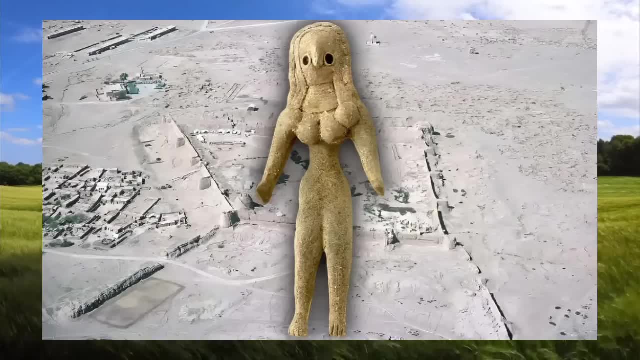 potentially religious aspects of the community. Magarth also played a role as a hub for trade in cultural exchanges with neighboring regions in the very early stages of human civilization. Its strategic location contributed to the interactions and connections with surrounding communities. The cultural developments at Magarth laid the groundwork. 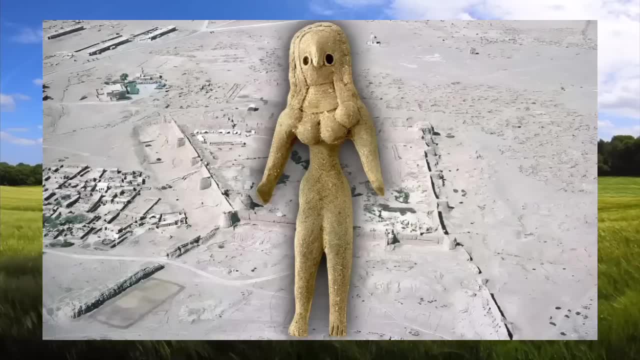 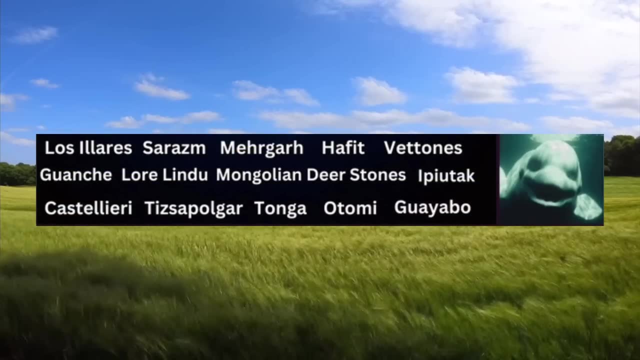 for the later emergence of the Indus Valley civilization, representing a critical phase into the transition from the Neolithic to the Chao Catholic period. Hafit- the Hafit culture named after the prominent Jebel Hafit Mountain in the United Arab Emirates. 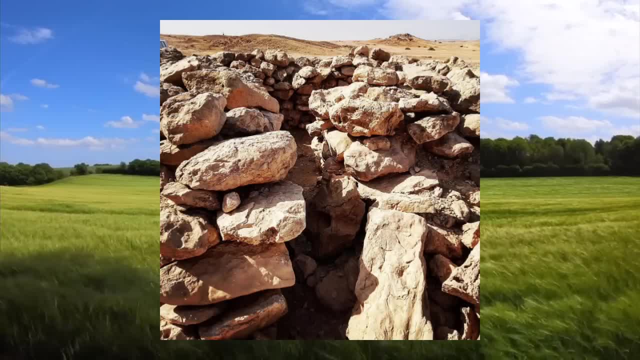 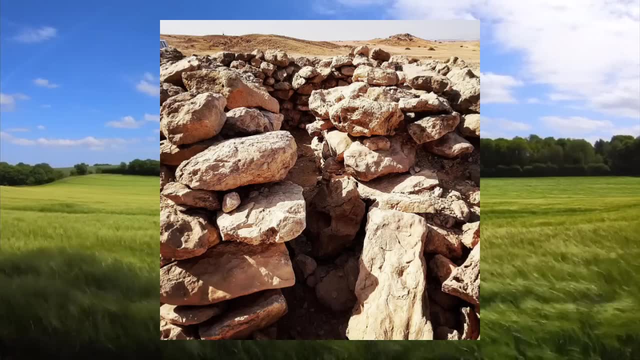 flourished in the Eastern Arabian Peninsula during the Bronze Age, roughly spanning from 3,200 to 2,600 BCE. One of the distinctive features of the Hafit culture is its unique burial practices, as evidenced by the construction of beehive tombs. 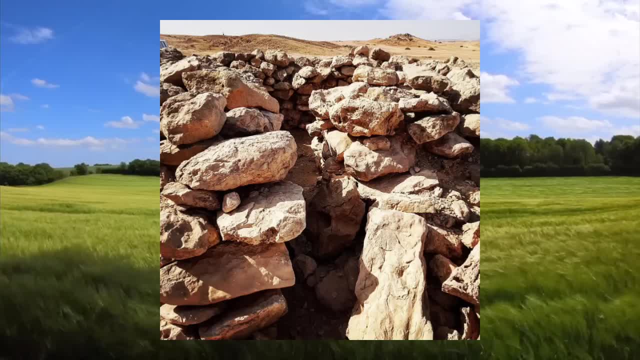 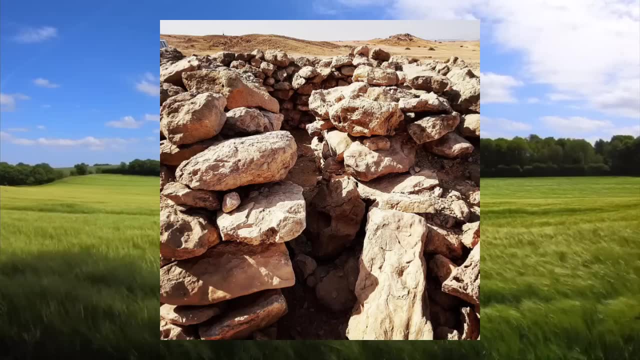 These collective burial sites, shaped like beehives and made of stone, were utilized for interning multiple individuals, along with accompanying artifacts like pottery and personal items. Geographically centered around Jebel Hafit in the Al Ain region, the Hafit culture showcased. 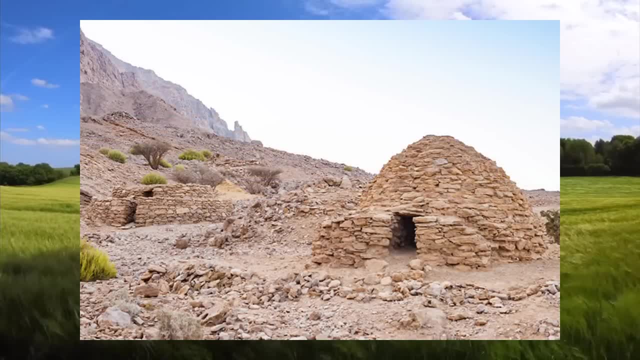 adaptability to the very arid environment of the Arabian Peninsula. Their mixed economy included agriculture, herding and domesticated animals, which all played a crucial role in sustaining their communities. Artifacts from the Hafit period, particularly pottery, stand out for their intricate designs and varied forms. 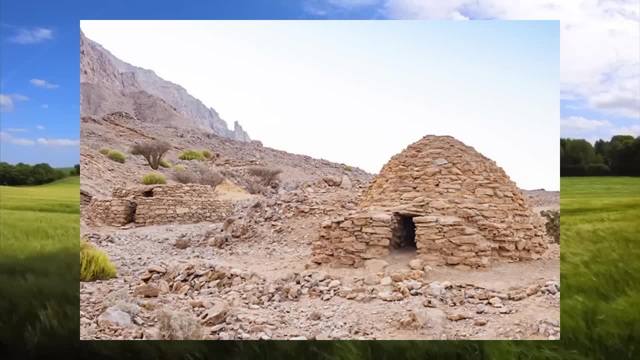 reflecting the cultural and artistic expressions of this ancient society. Defensive structures, including stone, stone walls and watchtowers, suggest a level of social organization in the recognition of security concerns. The Hafit culture is part of the broader cultural sequence in the Arabian Peninsula during the Bronze Age. 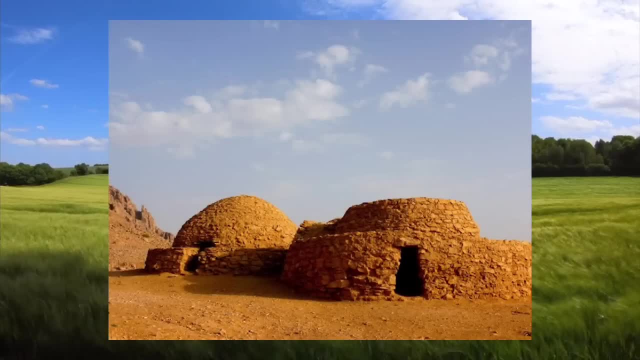 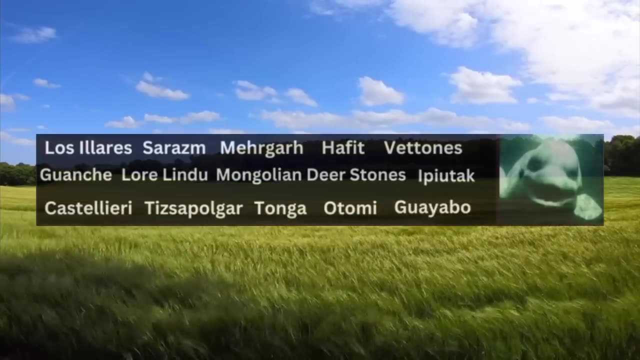 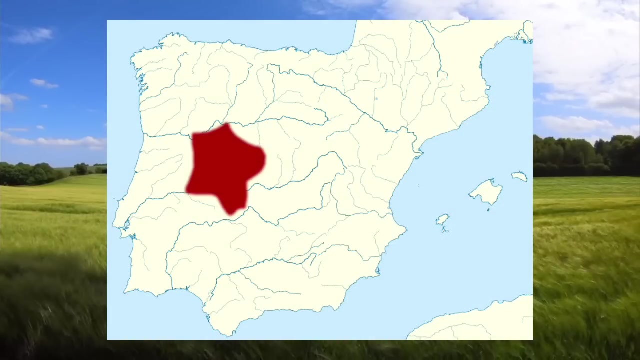 preceding the Umm al-Nar culture. Its archeological remains provide valuable insights into the burial rituals, daily life and the interactions of ancient communities in this arid region. Vitones. Vitones, an ancient Celtic-speaking people, inhabited the western part of the Iberian Peninsula. 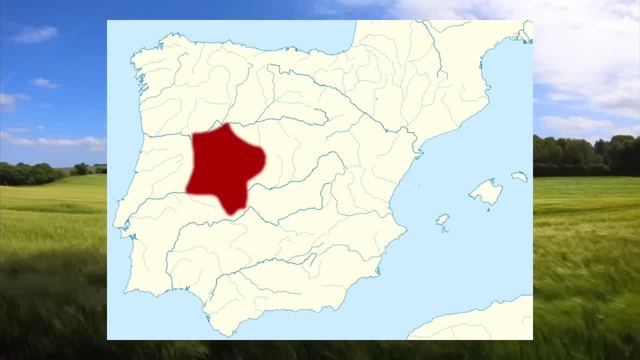 occupying regions that now include the Iberian Peninsula, formed central and western Spain and northeastern Portugal. living in a terrain that influenced their way of life, The Vitones were primarily agricultural and pastoral, engaging in farming and herding. Their settlements often fortified hilltops. 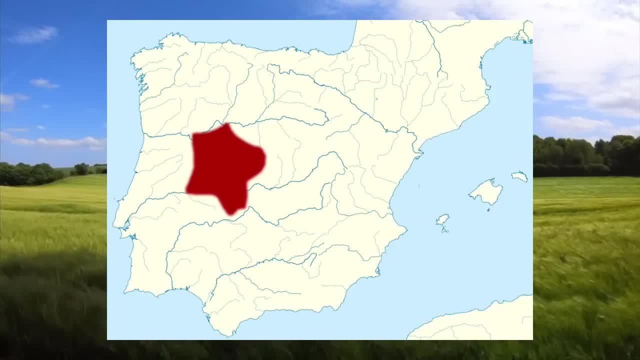 with defensive walls reflected a need for protection, highlighting the challenges of external threats. in their historical context, linguistically connected to the broader Celtic cultural sphere, The Vitones spoke a Celtic language, placing them within the larger framework of Celtic-speaking people in ancient Europe. 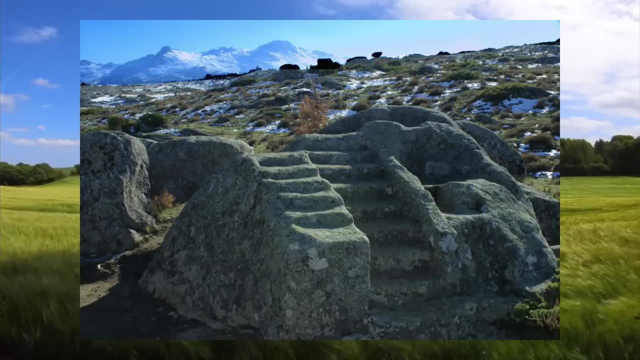 Their archeological record provides valuable insights into their material culture, revealing artifacts and structures that contribute to our understanding of their daily life and interactions with neighboring groups. As the Roman Republic expanded its influence into the Iberian Peninsula, the Vitones, like many indigenous peoples, came into contact. with Roman forces and over time the Vitones and other tribes in the region became assimilated into the Roman Empire and just got taken over by the Roman Empire, as we've seen a lot already, marking a significant transformation in their sociopolitical landscape. 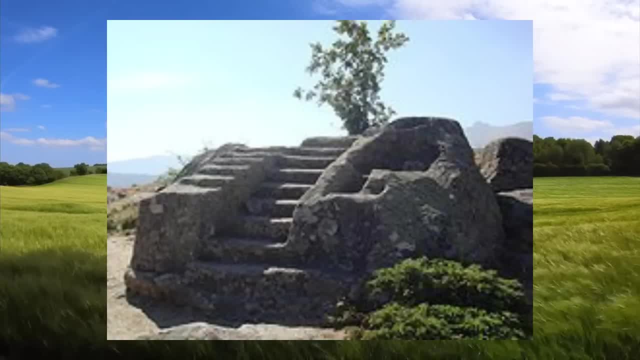 While historical records about the Vitones are limited, the combination of archeological evidence, linguistic connections and a broader context of Roman conquest enhances our comprehension of the Vitones and their place in the complex mosaic of pre-Roman Iberia, Guanche. The Guanches indigenous to the Canary Islands were the original inhabitants of this archipelago, situated off the northwest coast of Africa. Believed to have originated from North Africa, specifically associated with the Berber people, the Guanches likely settled on the Canary Islands around the first millennium BCE. inhabiting islands like Taranafe, Gran Canaria, La Palma and La Gomera, The Guanches developed a distinct way of life. The Guanches were skilled farmers and herders, cultivating crops such as barley and practicing animal husbandry with goats. 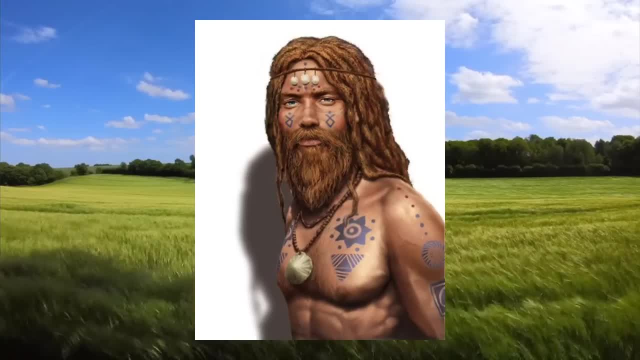 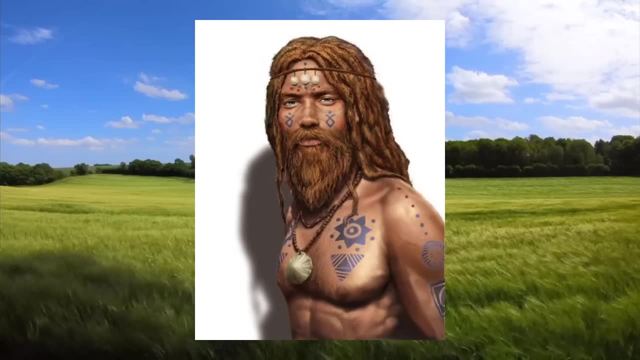 Their societal structure consisted of small chiefdoms or kingdoms, which were each led by kings. Descriptions from early European explorers portrayed the Guanches as tall, with light skin, fair or reddish hair and engaging in practices like body painting. 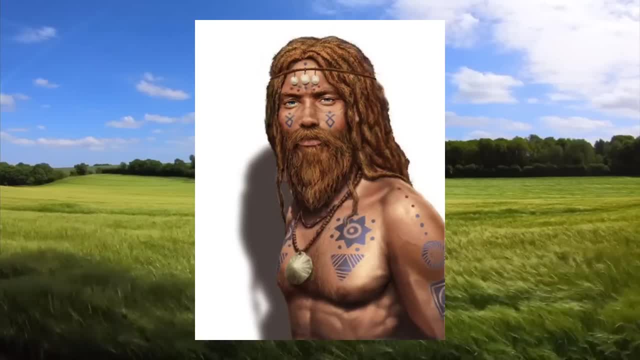 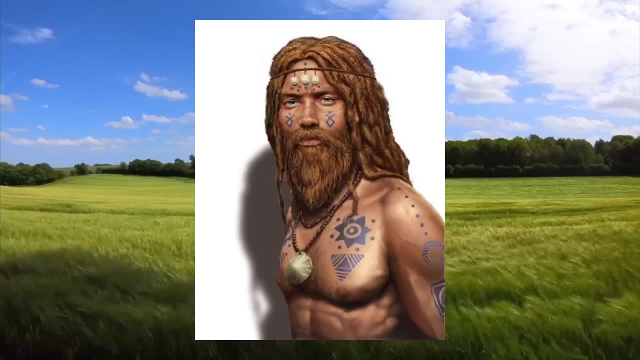 and scarification. In terms of spirituality, the Guanches adhered to a polytheistic belief system, worshiping deities associated with nature and fertility. Lummification was also a common place and practice, and the bodies of the deceased were often placed in burial caves. The Guanches language, known as Guanche, believed to have belonged to the Berber language family, but unfortunately became extinct after European colonization. The arrival of European explorers, particularly the Spanish, marked a transformative period of the Guanches, which basically just ended them. because of the warfare, Disease and forced labor which just ended the Guanche population. Despite this decline, the legacy of the Guanches endures in archeological sites, artifacts and cultural remnants, offering a glimpse into the rich and distinctive cultural heritage of the original inhabitants. 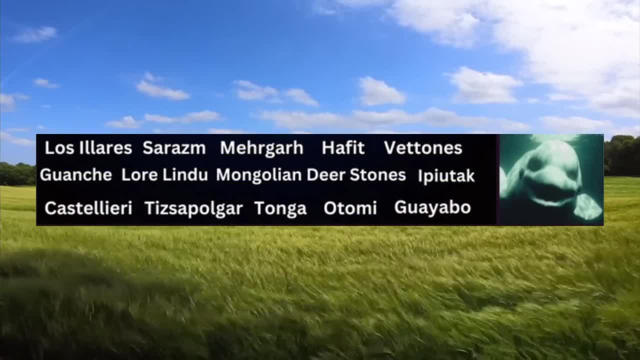 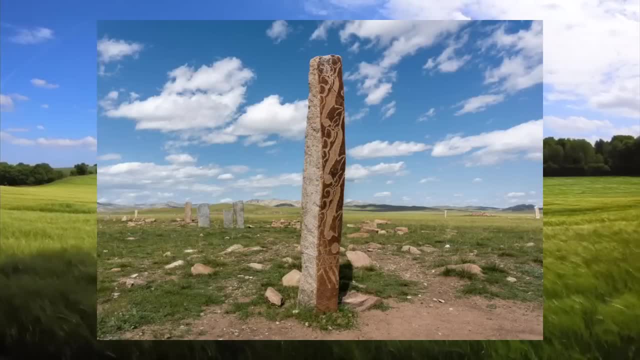 of the Canary Islands. Mongolian Deer Stones. Mongolian Deer Stones, dating all the way back to the Bronze Age and the Iron Age, are remarkable megalith monuments scattered all across Mongolia, particularly in the central and northern regions, Characterized by their large upright stones. 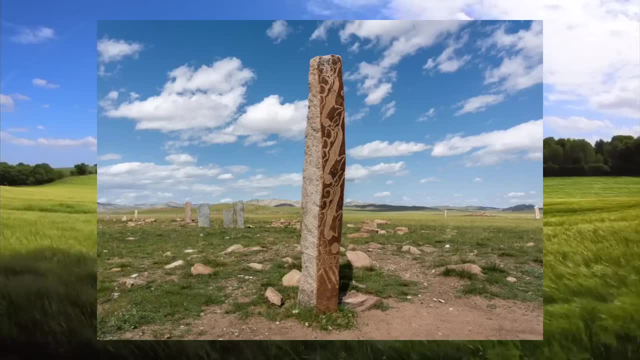 adorned with intricate carvings. the most prominent motifs include stylized depictions of deer, often with elaborate antlers, alongside other symbolic and abstract designs. The purpose and meaning of these stones have been subject of inquiry and debate, with prevailing theories suggesting roles. 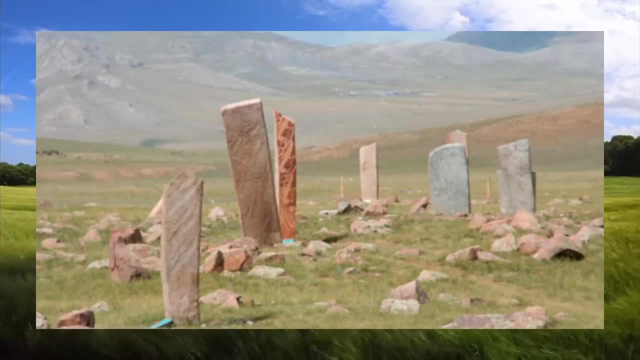 in marking burial sites serving as ceremonial or religious markers or commemorating significant events or individuals. Distributed primarily in areas like the Alcorn Valley and the Kholskobov Providence, Deer Stones form part of larger ceremonial landscapes, often associated with stone circles, rectangular structures. 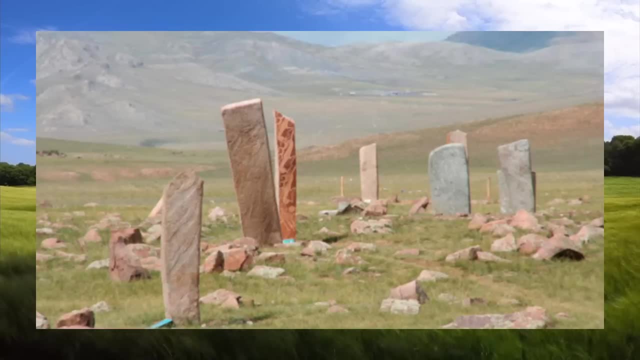 and burial mounds. These configurations hint at the complex and multifaceted roles these monuments played in ancient nomadic cultures. While the exact function remains elusive and unknown, the Deer Stones are invaluable cultural artifacts reflecting the artistic prowess and spiritual significance of the nomadic communities that once thrived in Mongolia. 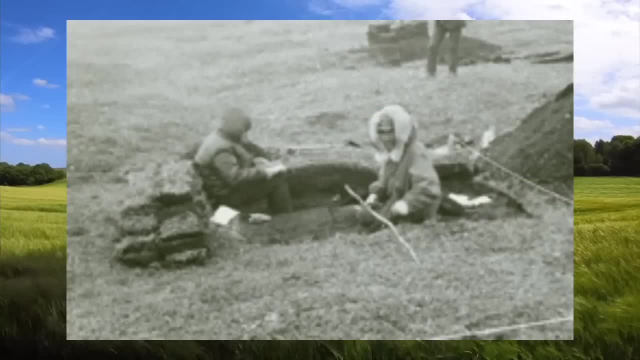 Ipu Attack. The Ipu Attack culture flourished in the Point Hope area of Alaska during the late prehistoric period, which was around 200 BCE to 500 CE, and it stands as a testament to the resilience of ancient Arctic communities in adapting. 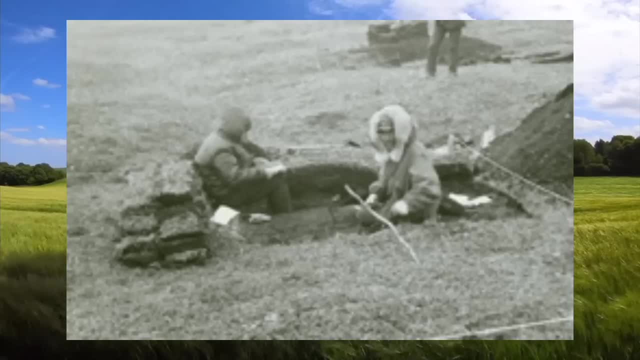 to their challenging environment and their freezing environment. Central to the survival was the subsidence strategy based on hunting and gathering, where marine mammals, fish, birds and local plants all played essential roles. Distinctive architectural features of the Ipu Attack culture include semi-subterranean 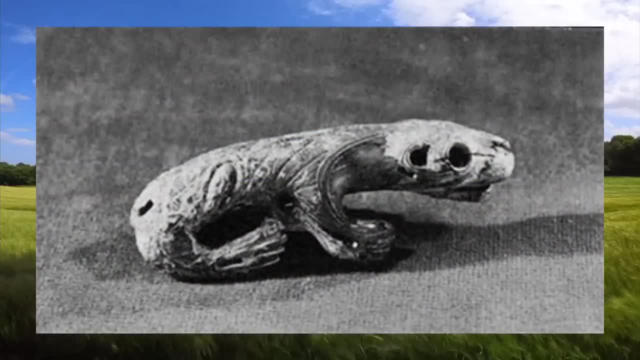 semi-subterranean houses with tunnel entrances, offering insulation against the harsh Arctic conditions. These structures were communal, often shared by extended families, reflecting a close-knit social organization. Artistic expressions of the Ipu Attack people are notable for their ivory carvings and figurines. 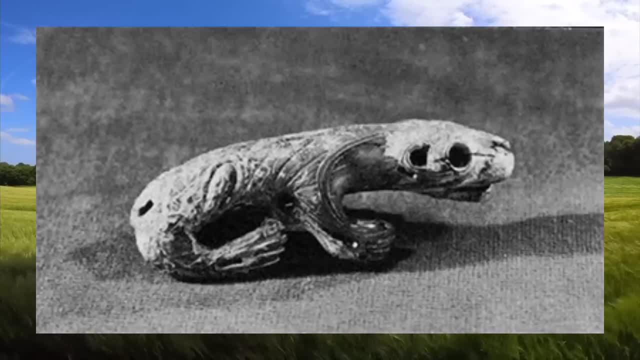 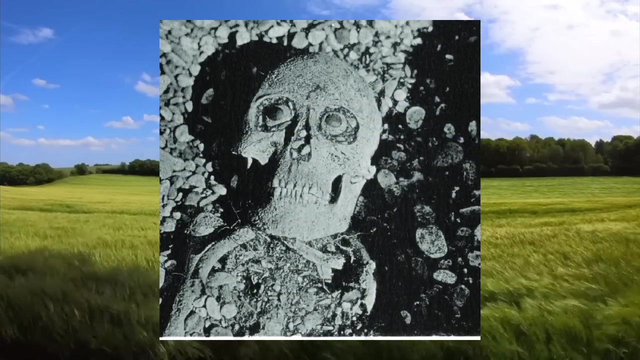 These artistic artifacts depict human and animal forms, providing insights into the cultural and spiritual dimensions of the community. Additionally, their tool assemblages showcase adaptability to the Arctic landscape, demonstrating their resourcefulness and utilizing available materials. Burial practices among the Ipu Attack involve the use: 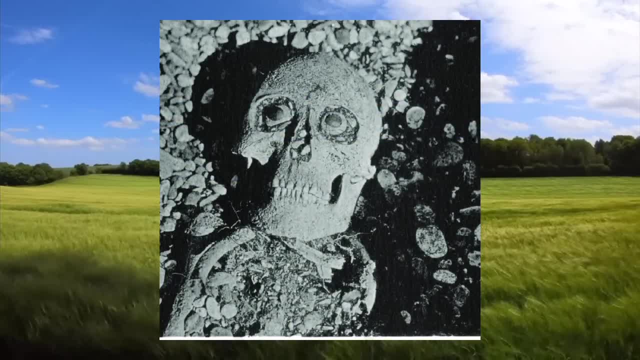 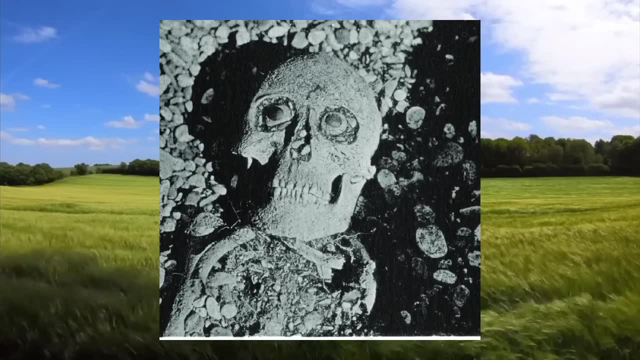 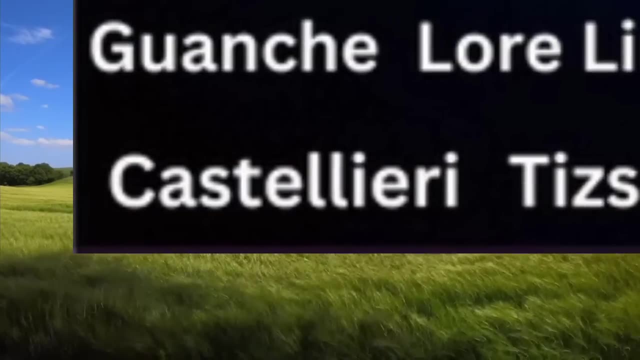 of underground chambers or pits with grave goods such as tools, ornaments and occasional animal offerings accompanying the deceased. These practices provide a glimpse into the spiritual beliefs and social structure of the Ipu Attack people Castellari, referring to the specific type. 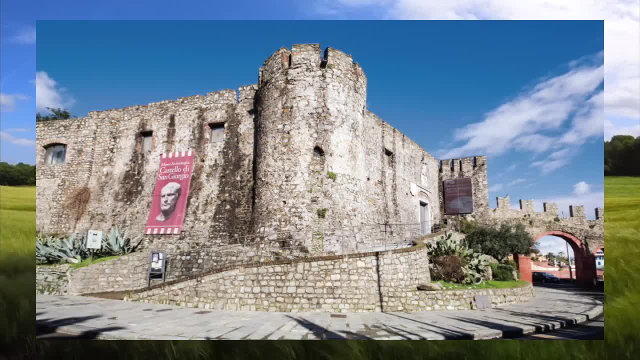 of archaeological site are ancient hill forts found in various regions of Europe, notably in the Eastern Alps, the Northern Adriatic and the Southern Atlantic. Castellari, referring to the specific type of archaeological site, are ancient hill forts found in various regions of Europe, notably in the Eastern Alps, the Northern Adriatic and the Southern Atlantic. 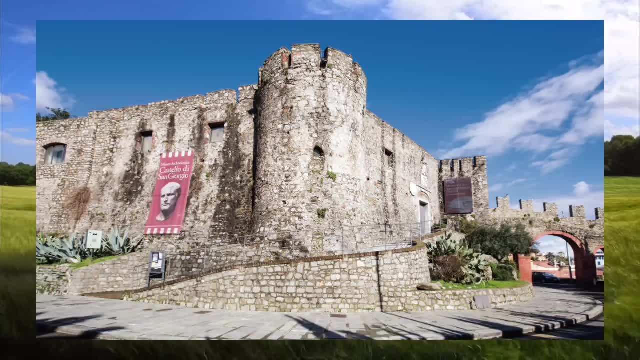 and the Western Balkans. The term, derived from the Italian word for castle, describes fortified settlements characterized by dry stone construction. These hill forts are strategically positioned on hill tops, leveraging any natural defence advantages, and are enclosed by walls that vary in thickness & height. 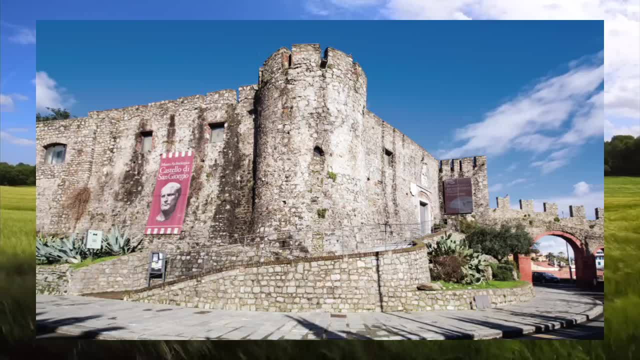 Dating the way back to the Bronze Age and the Iron Age. Castellari sites serve as tangible remnants of prehistoric settlement patterns and fortification strategies. The purpose of these hillforts remains the subject of scholarly debate And people don't really know. 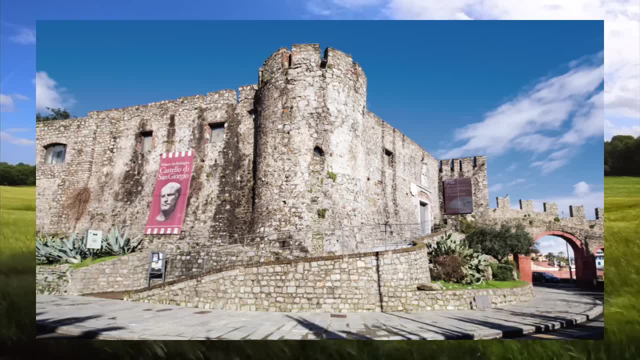 were for, but they think goes for defense against external threats and other theories. however, some researchers also propose ceremonial or symbolic functions with these hilltop forts, suggesting that these sites played a role in social and political activities. archaeological excavations at castelletti sites have unearthed a variety of artifacts, including pottery, tools and other items. 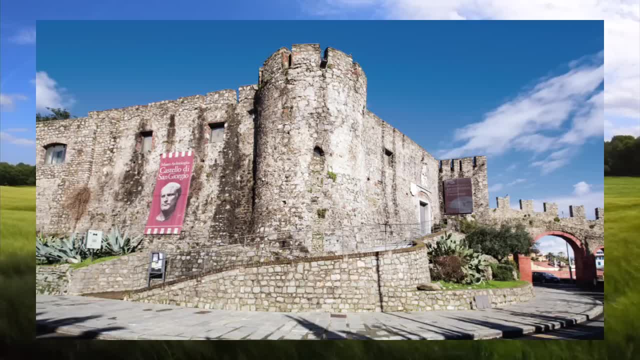 providing insights into their daily lives of the ancient communities that inhabited these hill forts. the construction techniques and cultural context of castellari contribute to our understanding of the diverse socio-cultural dynamics of prehistoric european communities during in different periods and history. while the term castellari is commonly used in italian and 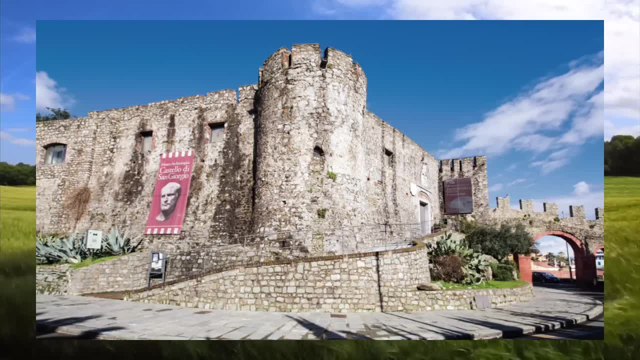 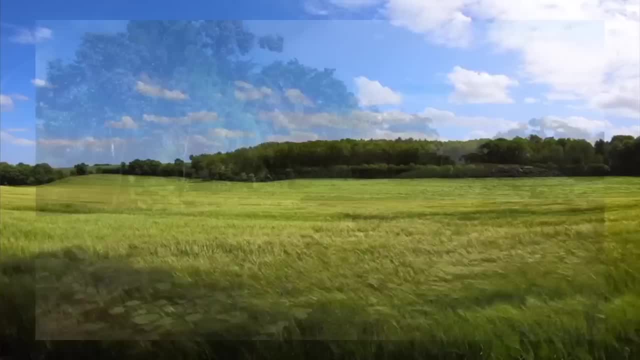 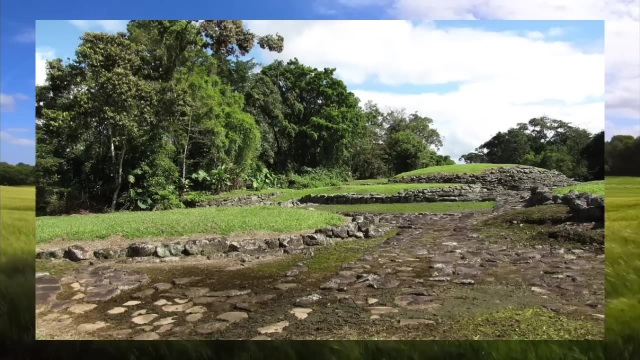 slovenian literature. similarly fortified hill sediments with different names exist in neighboring regions. guayabo, an archaeological site nestled in the turlebo valley of costa rica, stands as a testament to the ancient civilizations that once thrived in the region, occupied from approximately 1000 bce to 1400 ce. this pre-columbian site has revealed remarkable 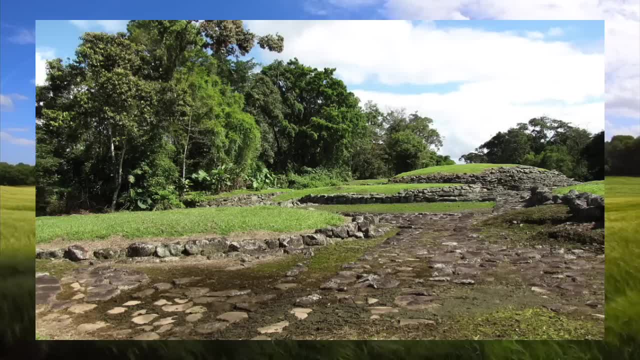 architectural features showcasing advanced engineering and planning. the remnants include mounds, staircases and platforms, with a sophisticated water management system, complete with aqueducts and water tanks, attests the ingenuity of its builders. considered a key archaeological discovery in central america, guado cultural significance is reflected in its status. 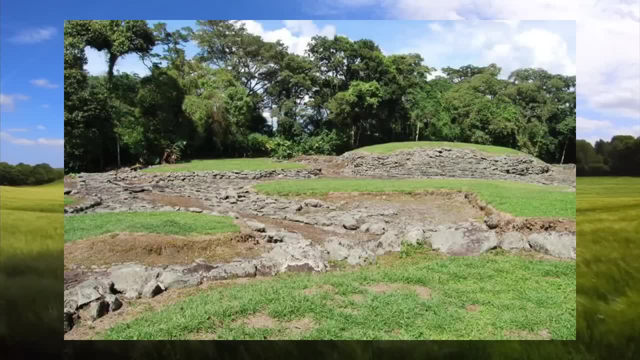 as a central hub for pre-columbian people. despite the site's abandonment, the reasons for which remain elusive, ongoing research and excavations aimed to unravel its history and shed light on the mysteries of its ancient civilization. the guayabo national monument envelops the archaeological site, safeguarding both the remains in the surrounding lush tropical forests. 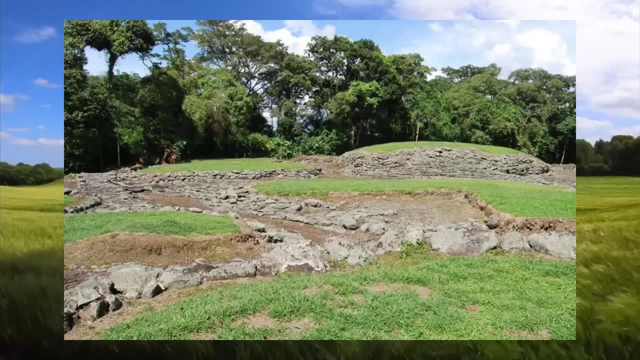 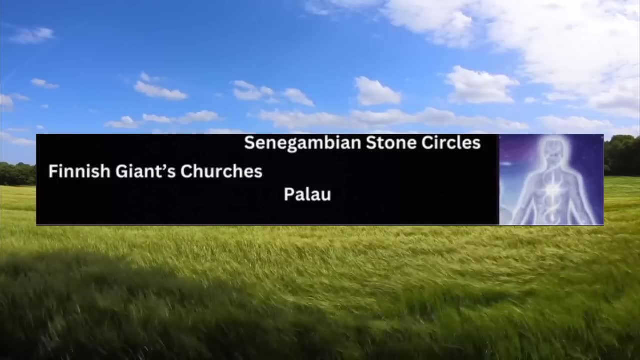 petroglyphs from mysterious rock carvings found at the site add another layer of intrigue, with the meaning and purpose subject to the scholarly interpretation and no one really knows all right. now on to the final tier of the iceberg, tier eight, starting off with sanegamian stone. 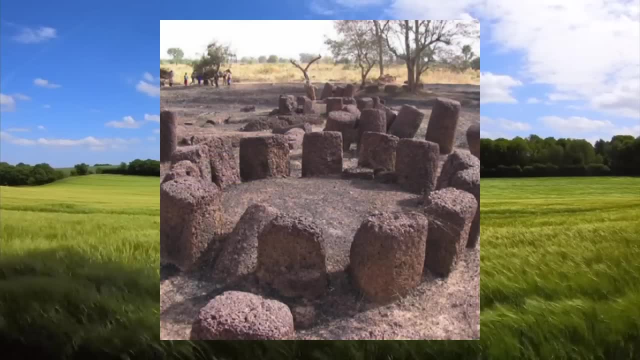 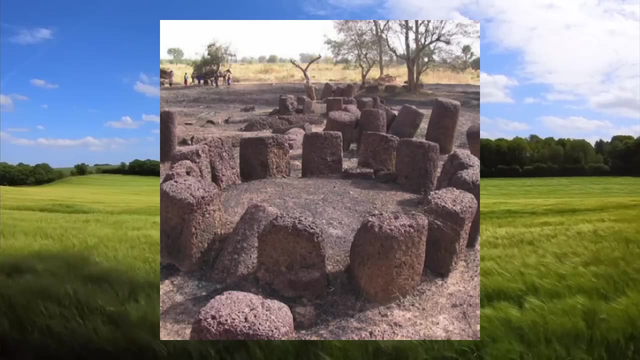 circles. the senegambian stone circles, situated in the senegambian region of west africa, represents a remarkable archaeological landscape dating back to the later part of the neolithic period and extending into the early iron age. scattered across senegal and gambia, these megalith monuments 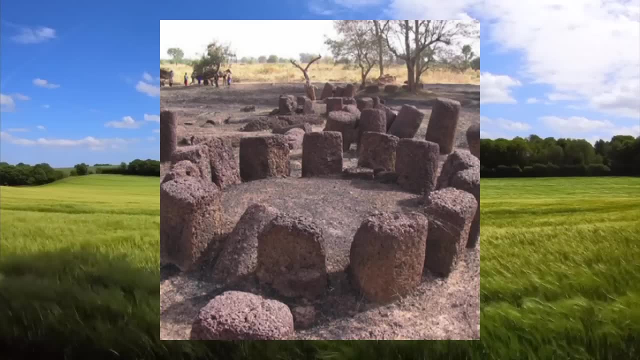 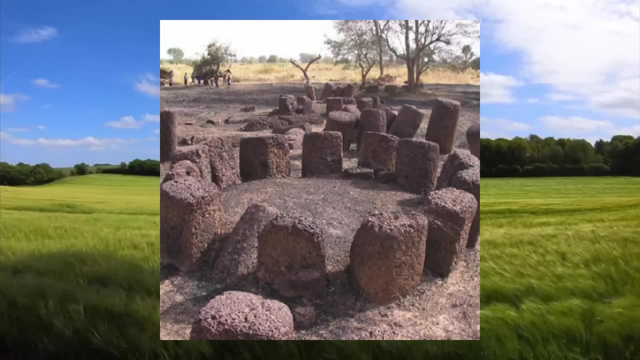 varying size and structure, ranging from small arrangements to extensive circles featuring tall and slender stones. the stones often associated with burial mounds hold cultural and funerary significance, suggesting a link to ancestral worship and ritual practice. the construction of the stone circles spans several centuries, pointing to a substantial cultural tradition and the presence of a diverse ethnic group in the region. 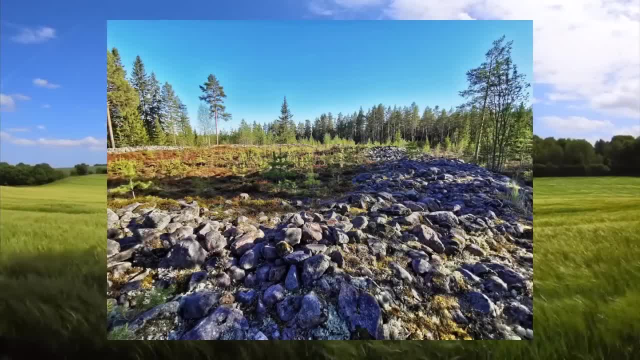 finnish giants churches known as jetin kiriko or jutuno kuriko in finnish, represent a captivating archaeological phenomena along the coast of austro-bothnia and finland. these prehistoric stone enclosures dating all the way back to 3500. 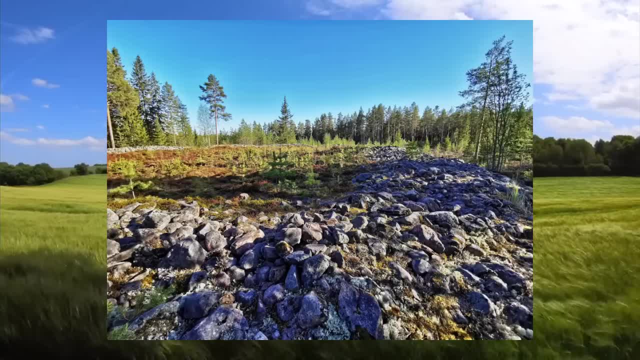 to 10th century. finnish stone enclosures dating all the way back to 3500 to 10th century, 2000 bc, stand as a rare examples of monumental architecture crafted by northern european hunter gatherers scattered across the coast of cocoa to kemi, with a concentration around rahel and olulu. 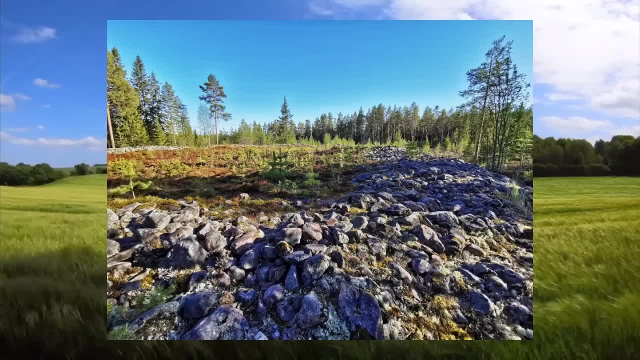 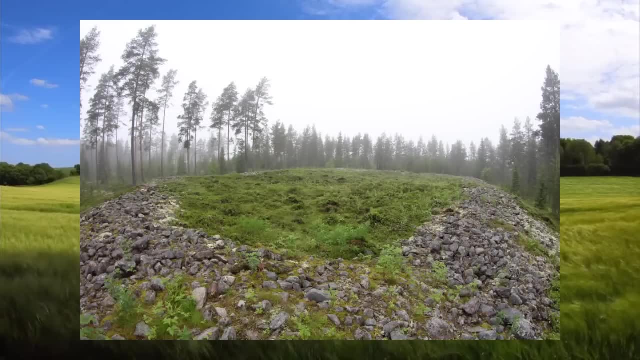 approximately 40 sites are known, forming a dense network of over 400 kilometers strip characterized by rectangular or oval boulder embankments. the giants churches display meticulous planning and construction. originally situated along the shoreline, they are currently found inland, possibly due to changes in the landscape or due to the lack of landings and the natural environment. 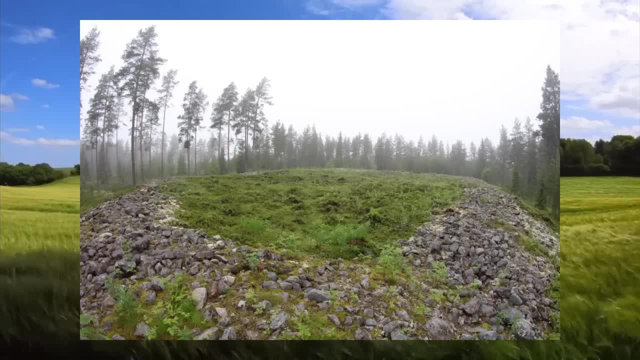 or post-glacial rebound. Despite their prominence, the exact purpose of these stone enclosures remain a mystery, with no hard evidence pointed to their intended use. One hypothesis suggests a practical function, proposing that the Giants' churches may have served as bases for seal hunters or spring. ice. This idea aligns with the notion that these structures accommodated individuals temporarily away from their usual dwelling places. Among the notable sites, the Castelli Giants' church stands out, enclosing an impressive area of 60 by 35 meters, dating back to the sub-Neolithic period. 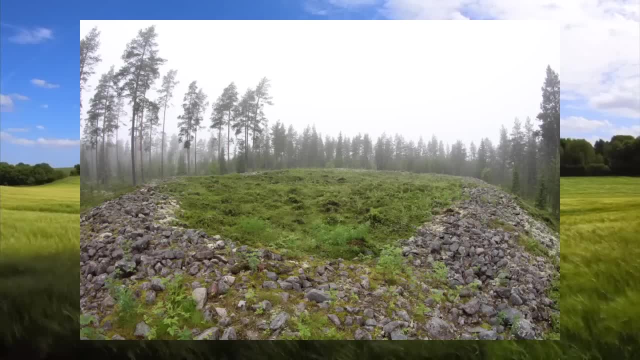 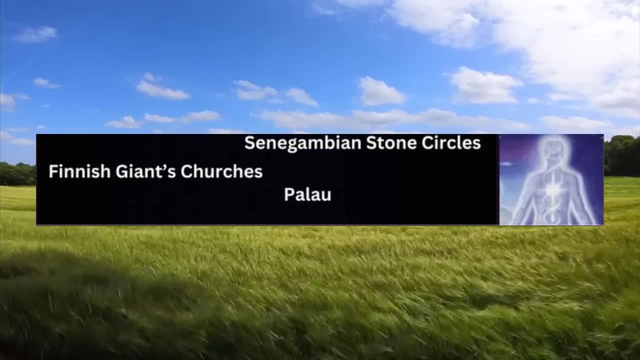 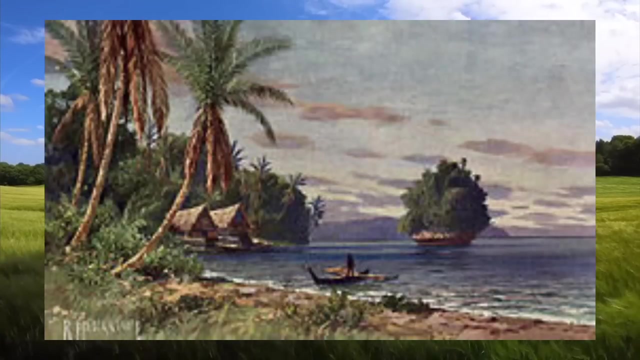 marking the transition from the Mesolithic to the Neolithic eras. The Giants' churches provide a unique window into the lives and activities of prehistoric communities in northern Europe. Palau, Palau, with a history spanning at least 3,000 years, has been home to ancient civilizations. 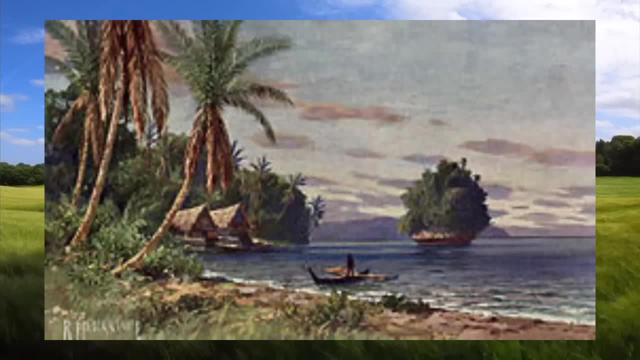 that have left a lasting impact on the cultural identity of the island nation. Early settlers from Southeast Asia navigated the vast Pacific to reach Palau, where they established a society marked by distinctive features such as stone monoliths known as bai. These megalith structures served as communal meeting places. 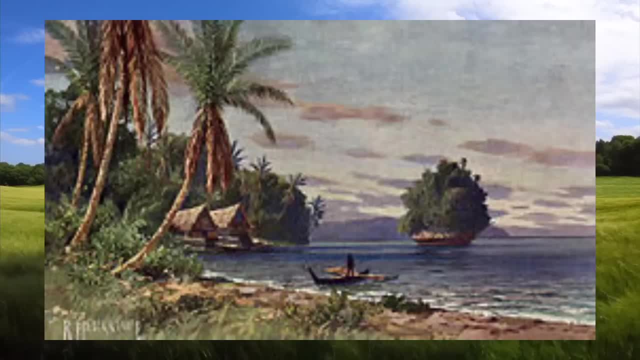 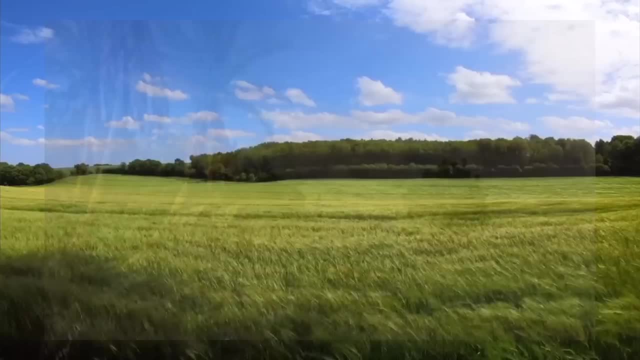 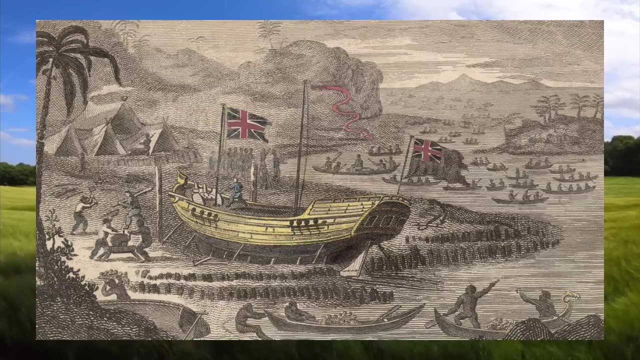 places of worship and venues for important ceremonies, Constructed with large stones adorned with intricate carvings. central to Palau's ancient civilization was a strong emphasis on oral transitions and storytelling, allowing for the transmission of important knowledge and cultural practices through generations. Social organization revolved around clans, each with 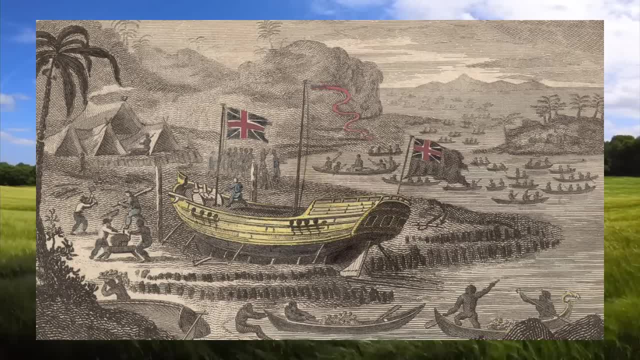 their own chief, reflecting a demographic of the island nation. Palau was a place where the people of Palau were able to interact with each other and interact with each other. Palau was a place where the people of Palau were able to interact with each other and interact with each other. 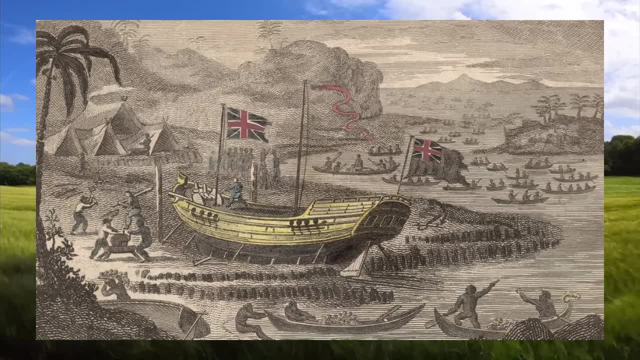 The practice of bull community meetings to discuss and decide on issues underscored the collaborative nature of Palauan society. The ancient Palauans were skilled navigators, utilizing their knowledge of the stars, ocean currents and natural landmarks for sea-faring expeditions. This expertise facilitated trade and cultural interactions with neighboring islands. 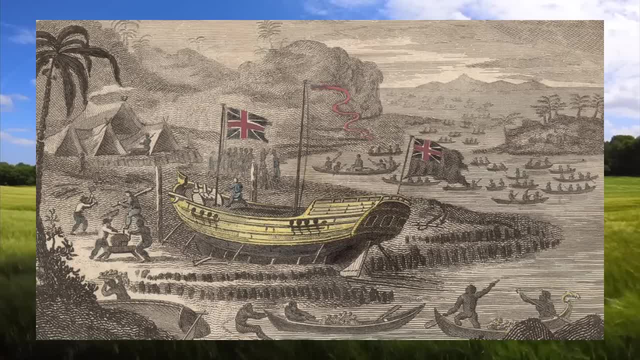 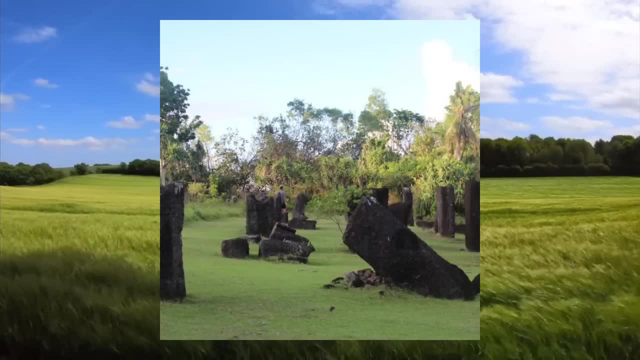 contributing to the broader network in the Pacific. However, encounters with European explorers and colonial powers such as Spain, Germany and Japan brought significant changes to Palauan society, introducing new technologies and industries. Palau was a place where the Palauan IPC mujeres were successful. Palau gained independence in 1994, marking a new chapter in 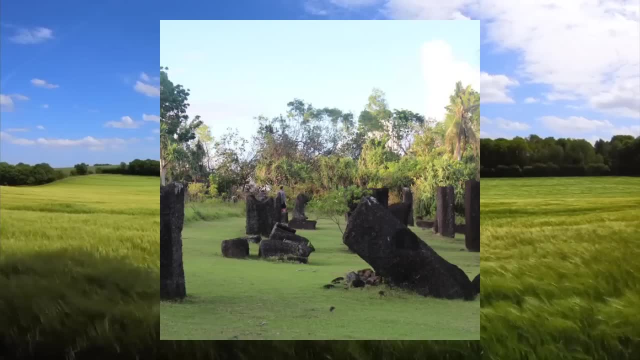 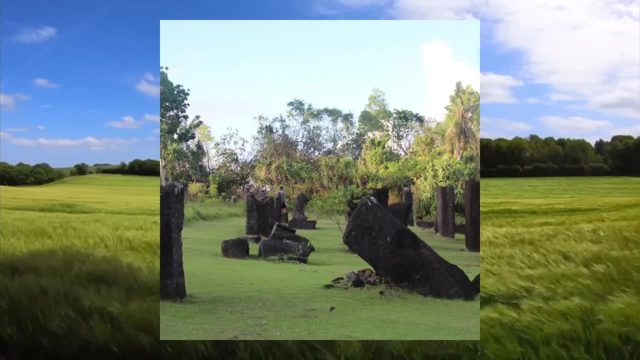 the history as a sovereign nation with its own government and constitution. While much of Palau's ancient history is preserved in oral traditions and archaeological sites, the legacy of its early civilizations remains evident in the stone, monoliths, traditional practices and navigational 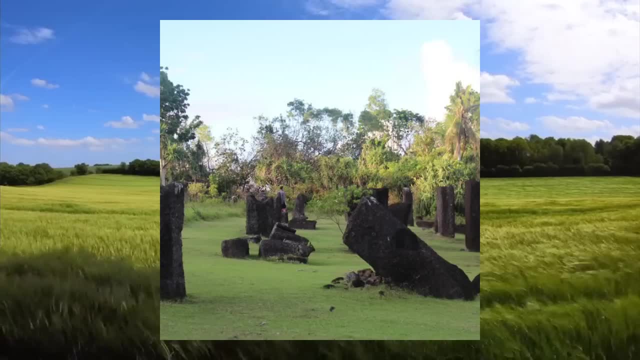 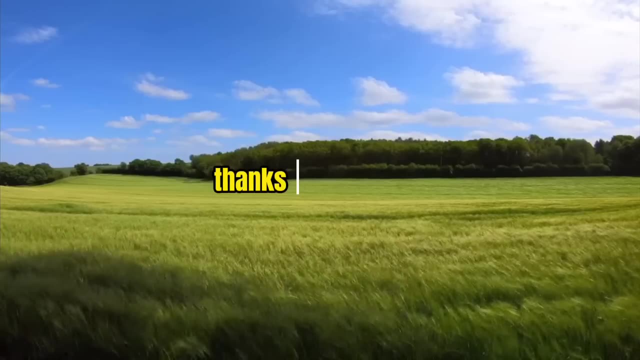 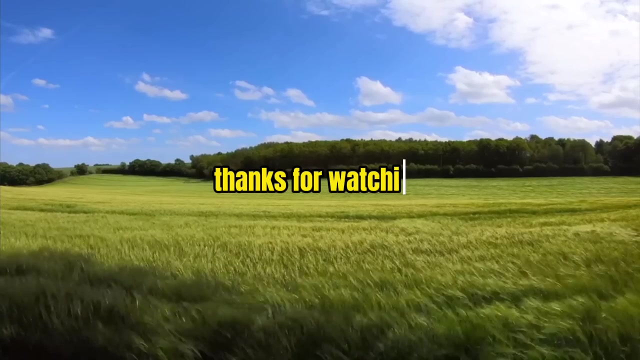 skills that continue to shape the cultural heritage of the Palauan people. thank you guys for watching- if you are still watching, because we're about like two and a half hours in, i think, which is a really long time for ancient civilizations, and i thought this.